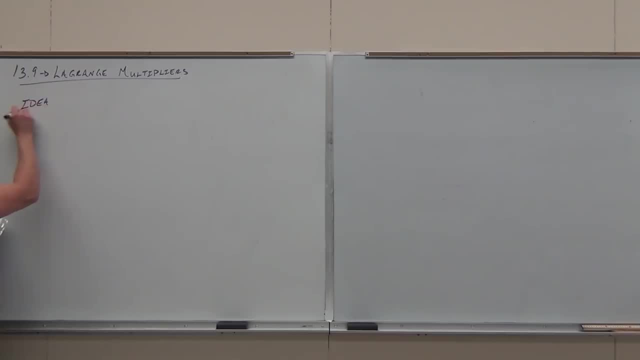 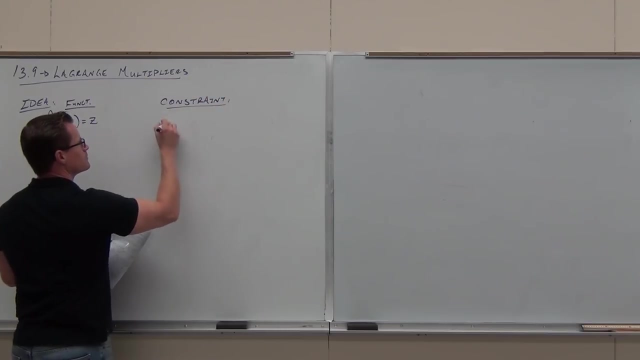 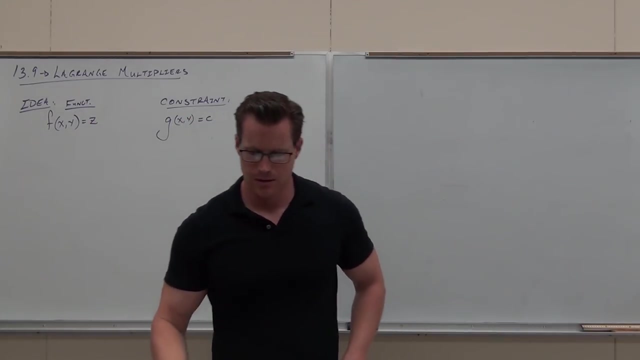 So here's the idea. So take a function, Notice a two-variable function- This is a surface- And take a constraint Where c is a constant. Listen carefully, because I do not want you to miss this. Listen carefully, because I do not want you to miss this. 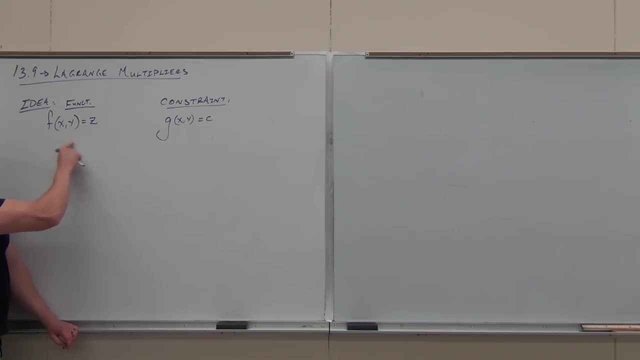 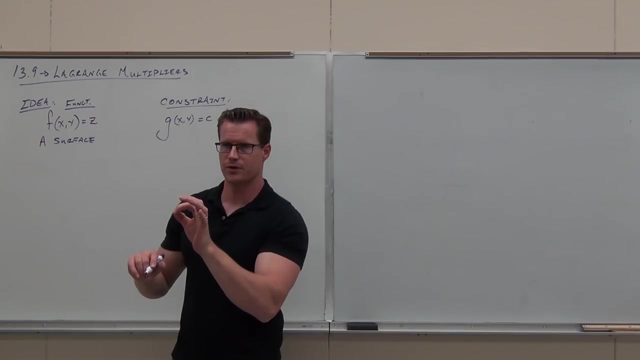 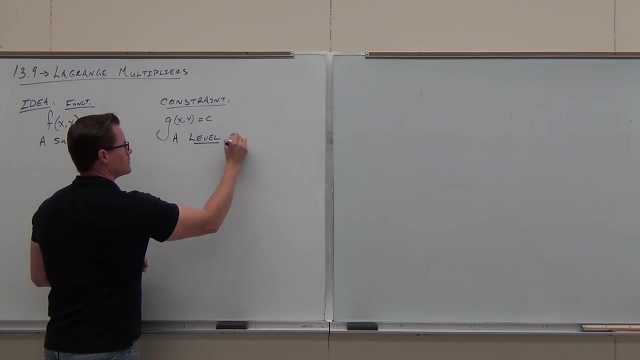 Recognize two independent variables: Two independent variables equal to a dependent variable. This is a surface, correct. Recognize two independent variables equal to a constant. This is a level curve to a surface. Do you see it? This is a level curve to some function. 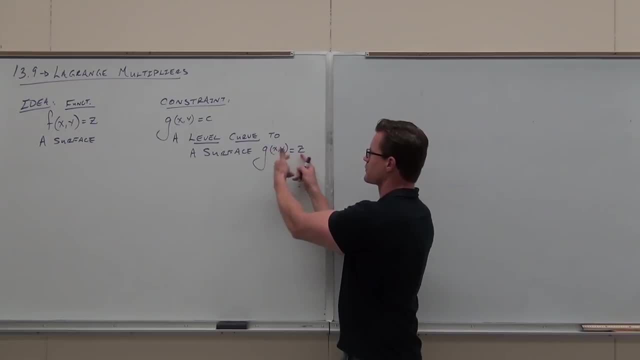 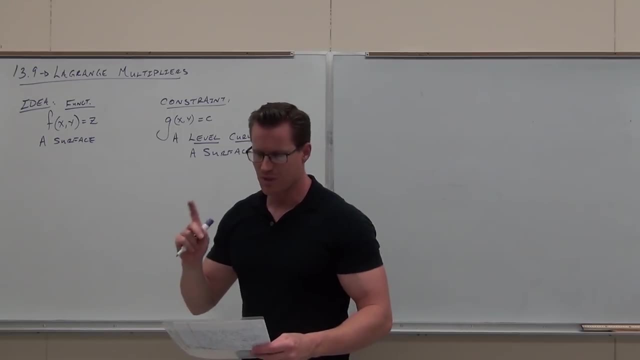 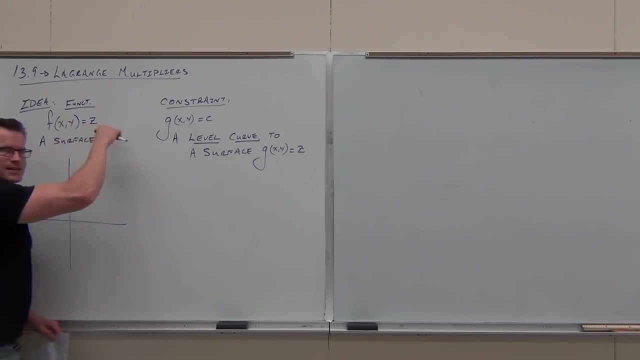 That should make some sense. If that's a surface and I let the surface equal a constant, I get a level curve to the surface. So eventually we're okay with that one. Now consider this. If I set, Please watch carefully. 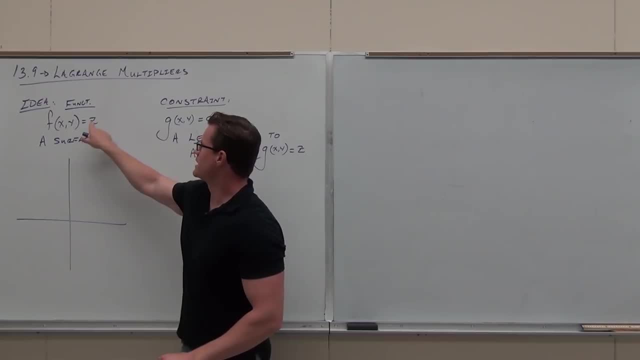 Don't blink, You'll miss it. You'll miss it if you blink. If I start setting This one equal to constants, I'm going to get a whole bunch of level curves. You guys get it. A whole bunch of them. 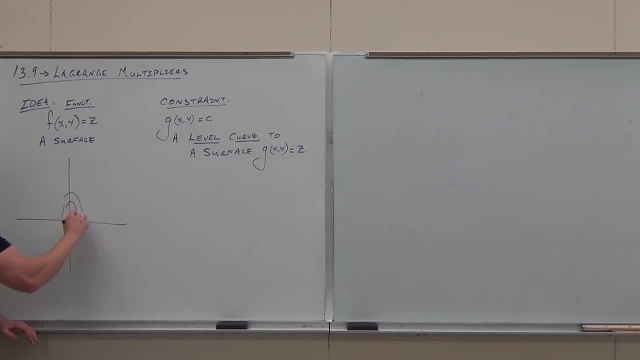 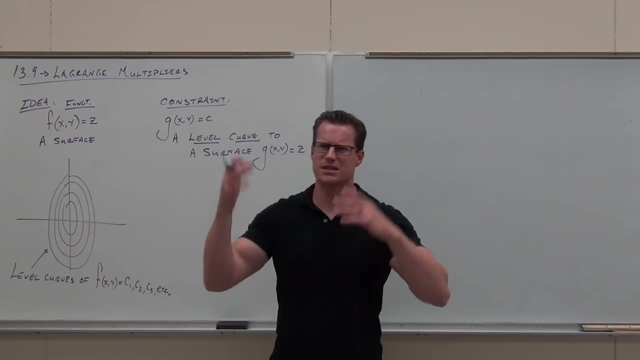 So let's look at some just made-up old level curves. Level curves of f of x equals c1, c2, c3. c3. c3. That doesn't matter, We're getting some level curves on that surface. 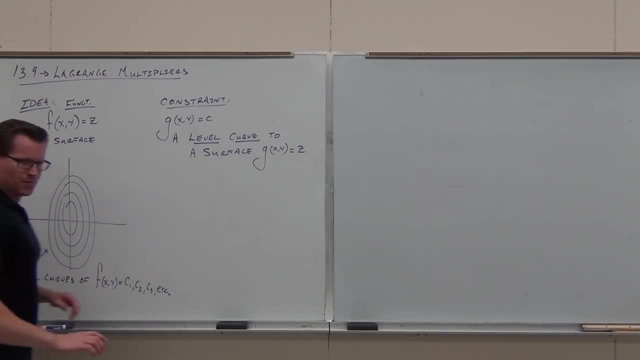 And let's look at this level curve, Check it out, Lost it. If this is a surface, it's going to have a whole bunch of level curves at different values of c. Do you follow me? This is already a level curve. 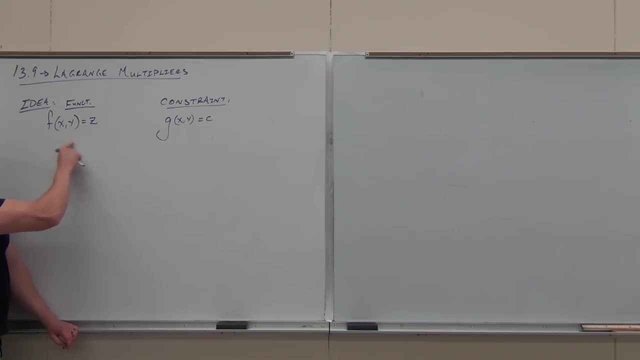 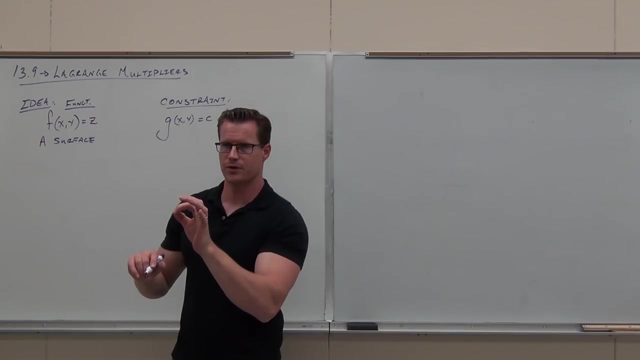 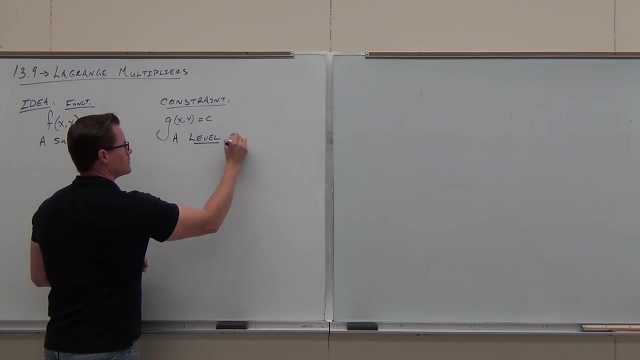 Recognize two independent variables: Two independent variables equal to a dependent variable. This is a surface, correct. Recognize two independent variables equal to a constant. This is a level curve to a surface. Do you see it? This is a level curve to some function. 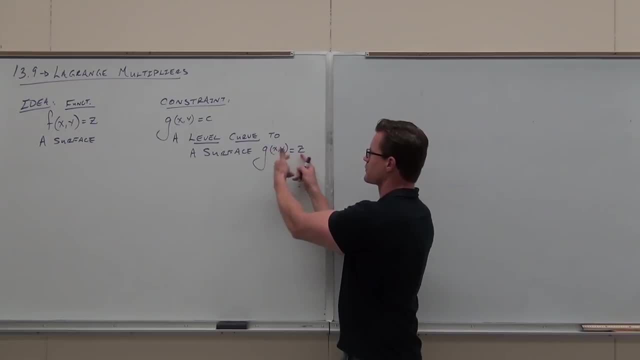 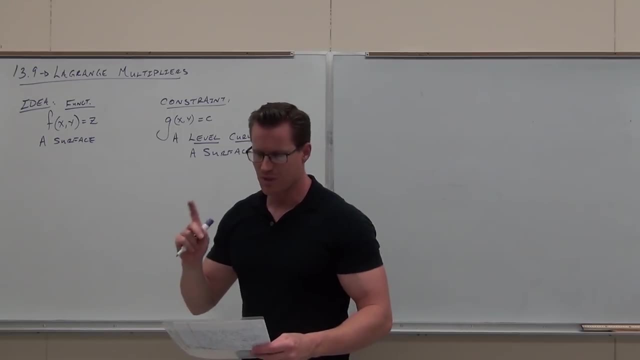 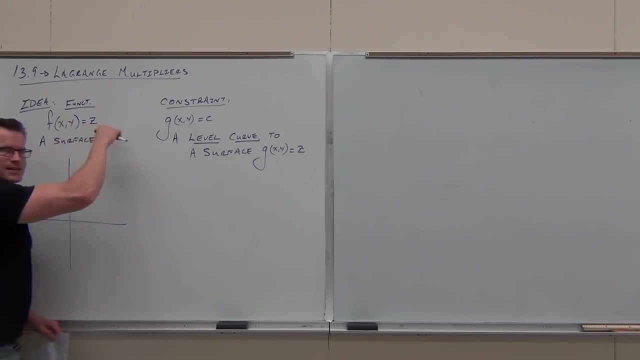 That should make some sense. If that's a surface and I let the surface equal a constant, I get a level curve to the surface. So eventually we're okay with that one. Now consider this. If I set, Please watch carefully. 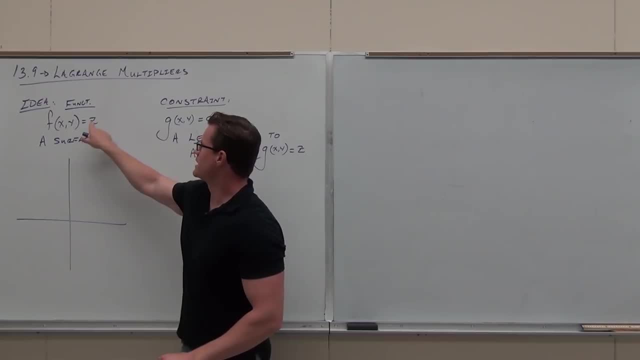 Don't blink, You'll miss it. You'll miss it if you blink. If I start setting This one equal to constants, I'm going to get a whole bunch of level curves. You guys get it. A whole bunch of them. 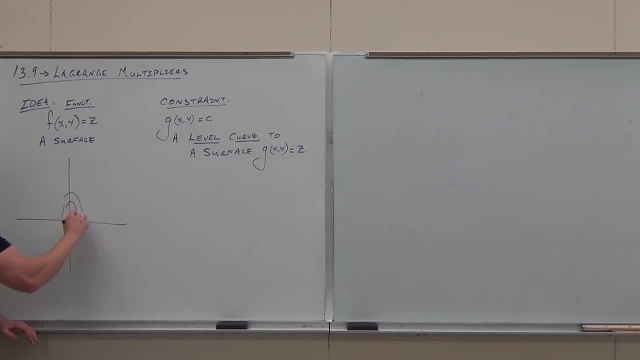 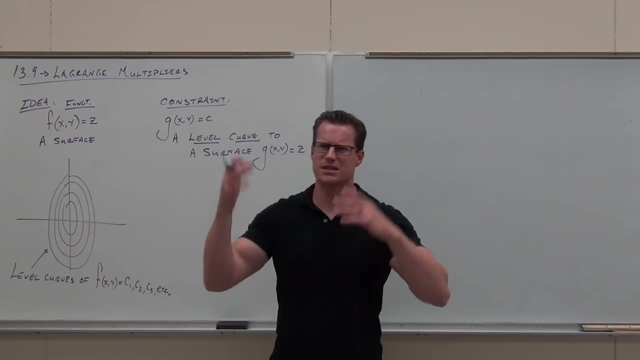 So let's look at some just made-up old level curves. Level curves of f of x equals c1, c2, c3. c3. c3. That doesn't matter, We're getting some level curves on that surface. 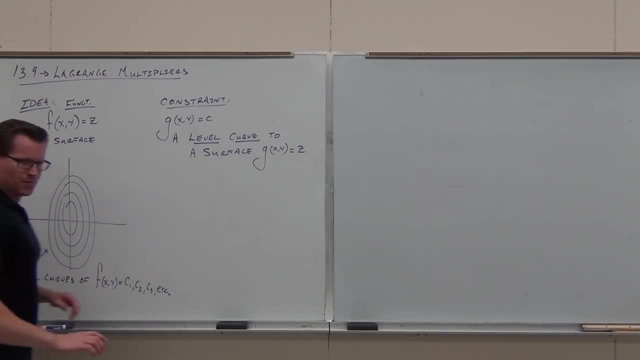 And let's look at this level curve, Check it out, Lost it. If this is a surface, it's going to have a whole bunch of level curves at different values of c. Do you follow me? This is already a level curve. 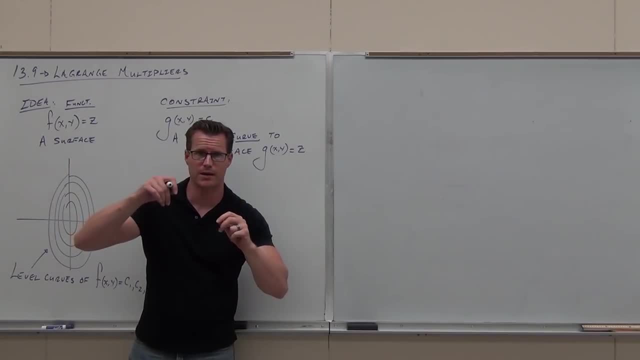 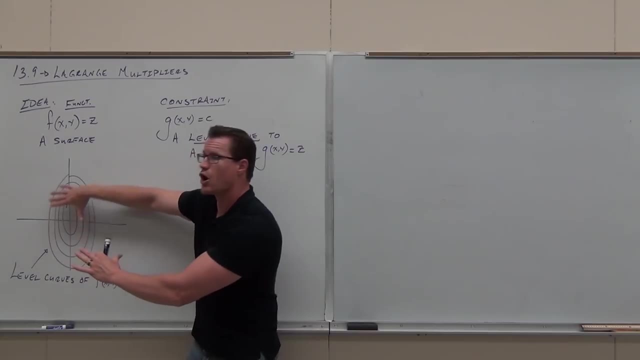 The point is there is going to be an overlay of the level curves of this surface that equal to the different values of c. You're getting different level curves. There's going to be a contour plot. You see all the different level curves we've talked about before. 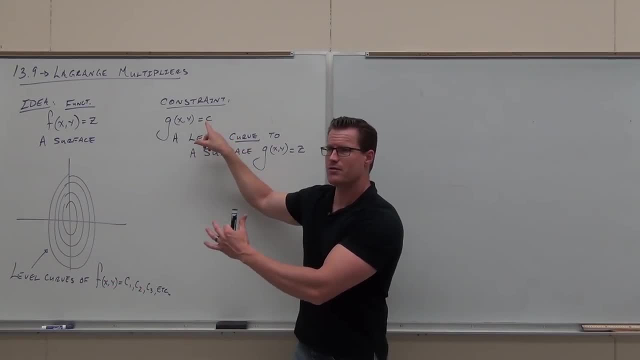 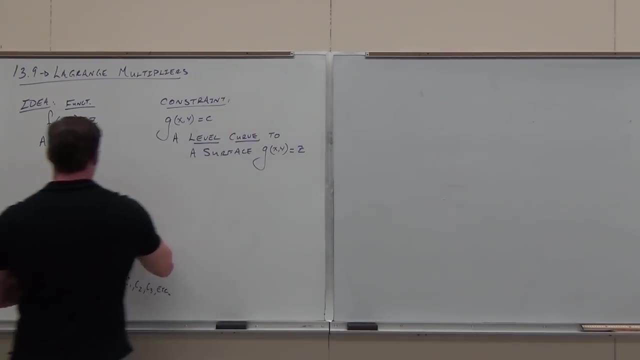 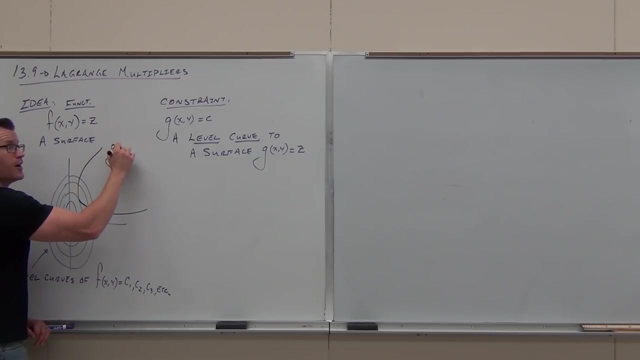 There's a whole bunch of them, But that's also a level curve. Verify something: This and all of these are on the same plane. That means there's going to be some overlay. Let's call this the level curve, This one. 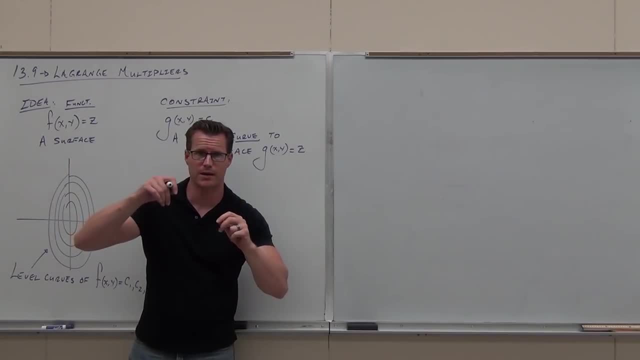 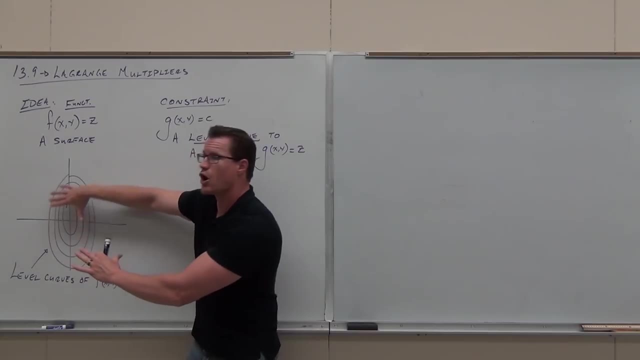 The point is there is going to be an overlay of the level curves of this surface that equal to the different values of c. You're getting different level curves. There's going to be a contour plot. You see all the different level curves we've talked about before. 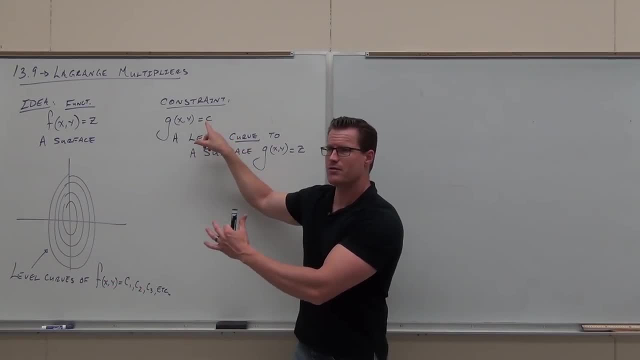 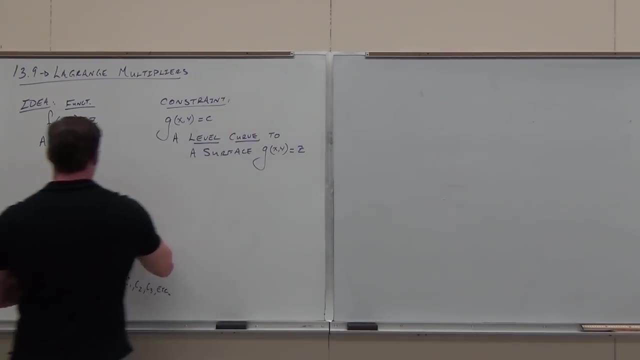 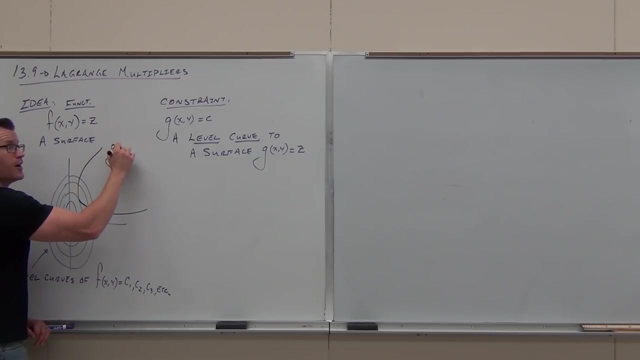 There's a whole bunch of them, But that's also a level curve. Verify something: This and all of these are on the same plane. That means there's going to be some overlay. Let's call this the level curve, This one. 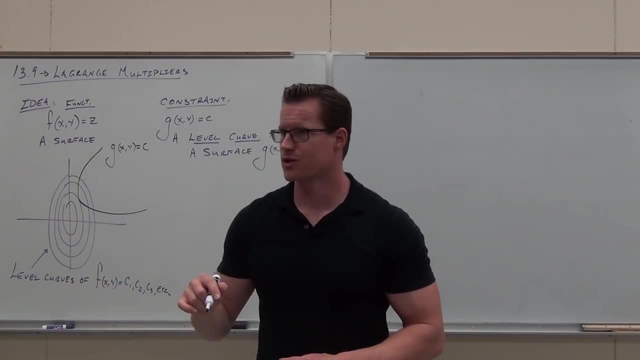 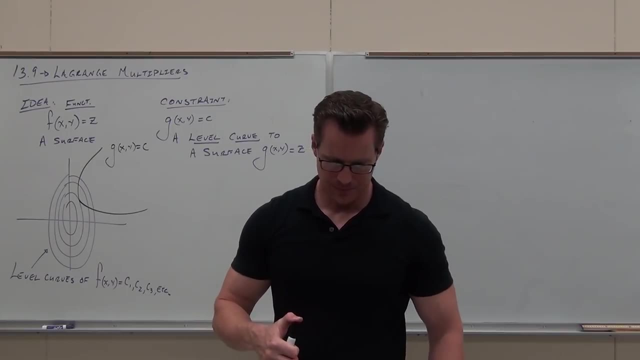 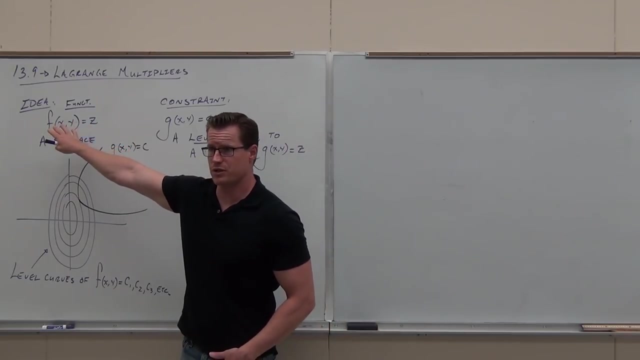 There's going to be an overlay. These level curves are going to intersect. Do you get it? Here's the beautiful thing about it: If we're on a function but we're also given a constraint, Listen carefully, We have to be on the surface. 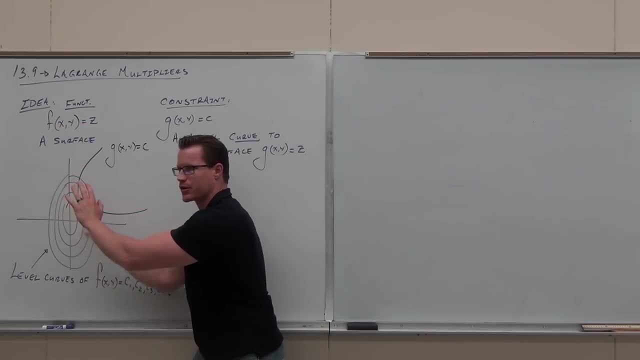 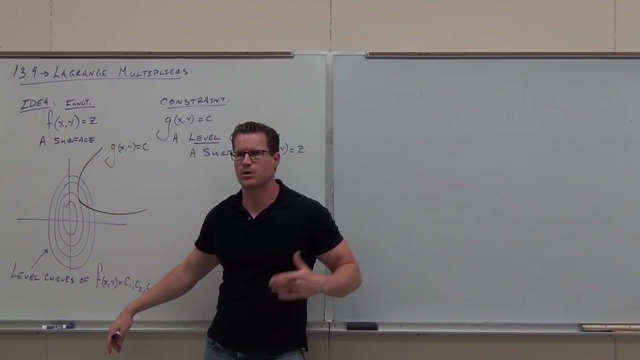 You with me. We have to be on one of these level curves. We also have to be on on this specific level curve where these level curves intersect, this level curve. Do you guys see that we have to be on both? We've got to be on both. 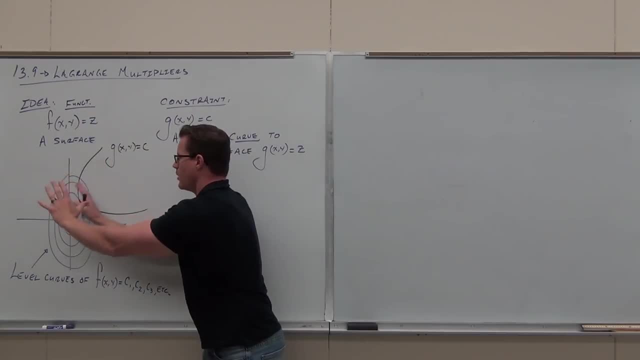 We have a good strength. We have to be on this. We have a function. We have to be on this. We're on all these level curves, but we're bound to this one. This is our constraint. It constrains our outcomes. 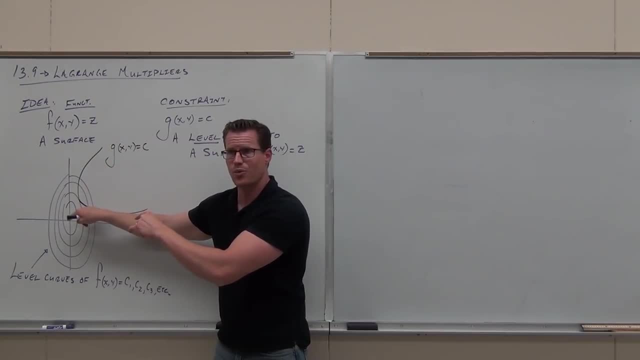 This level curve is going to intersect these level curves Where they do. that's a contour plot. Notice that these level curves are giving different heights, Different heights. I don't know why I said that so intensely. Different heights, We're getting different heights. 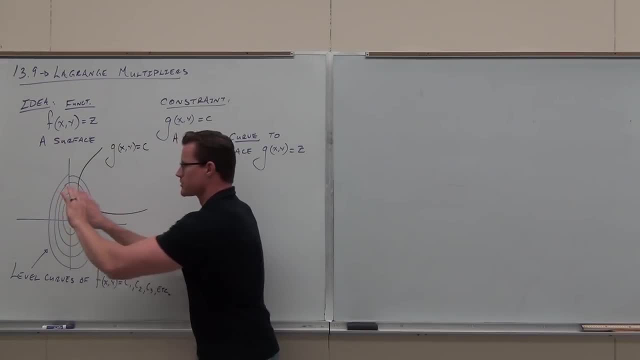 This is either falling. Look carefully, These level curves are either falling away or they're climbing upwards. That means wherever this guy intersects, intersects them. we have different values of our function. Where it bounces off one of them, We will either get a maximum. 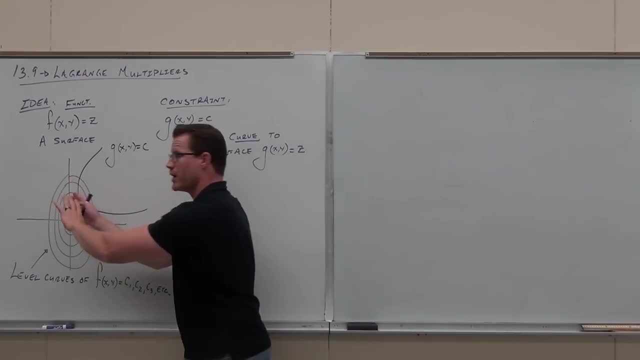 Or a minimum, Because either it's dropping away or it's climbing up. Did you see it? This is what we're looking for. Everything else is going to be higher and or lower. Well, sorry, and either one, It's going to be higher or lower than that point. 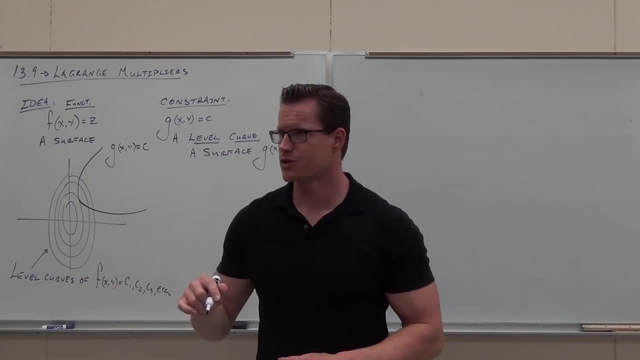 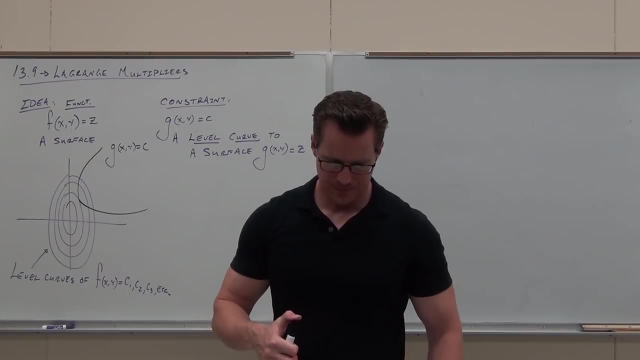 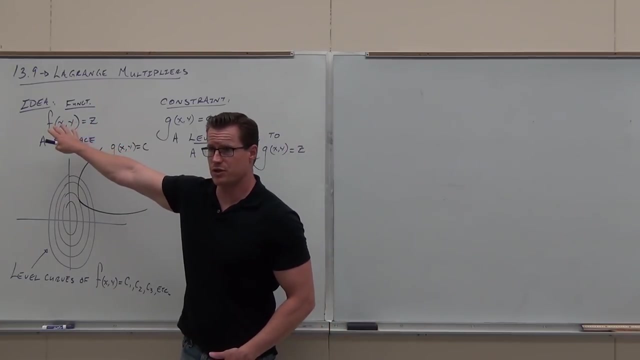 There's going to be an overlay. These level curves are going to intersect. Do you get it? Here's the beautiful thing about it: If we're on a function but we're also given a constraint, Listen carefully, We have to be on the surface. 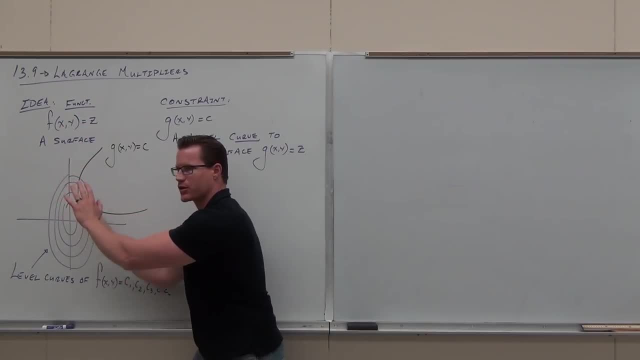 You with me, We have to be on one of these level curves We also have to be on. We have to be on this specific level curve where these level curves intersect, this level curve. Do you guys see that we have to be on both? 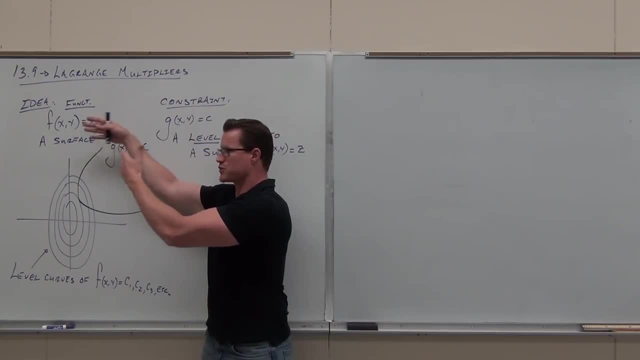 We've got to be on both. We have a good strength. We have to be on this. We have a function. We have to be on this. We're on all these level curves, but we're bound to this one. This is our constraint. 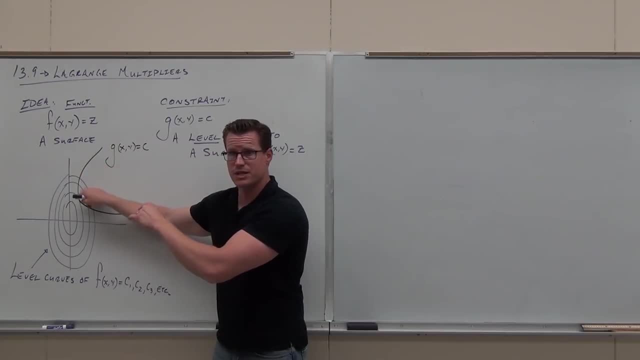 It constrains our outcomes. This level curve is going to intersect these level curves where they do. That's a contour plot. Notice that these level curves are giving different Heights Different heights. I don't know why I said that so intensely. 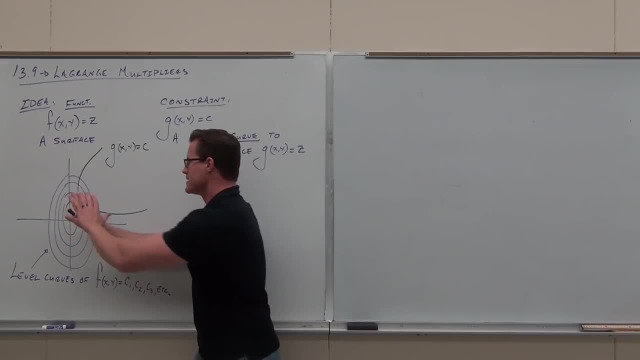 Different heights. We're getting different heights. This is either falling- Look carefully, These level curves are either falling away or they're climbing upwards. That means wherever this guy intersects, Intersects them. we have different values of our function. Where it bounces off one of them, 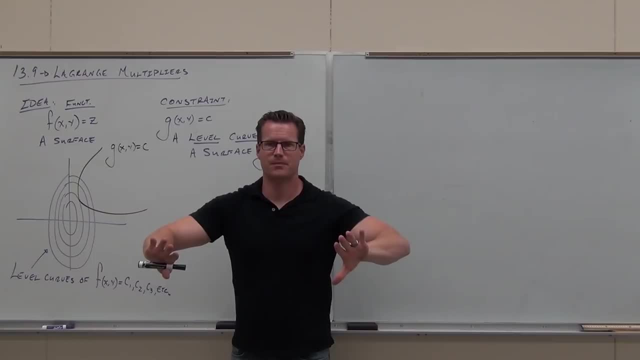 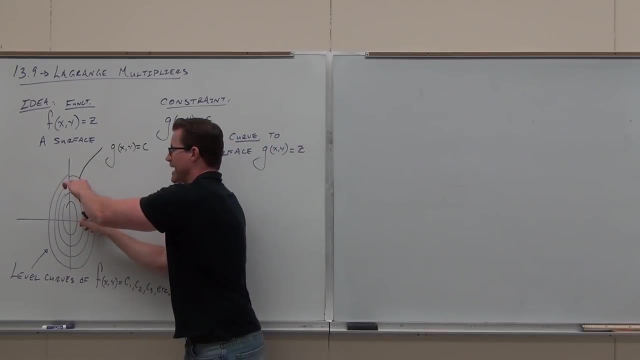 We will either get a maximum Or a minimum, Because either it's dropping away or it's climbing up. Do you see it? This is what we're looking for. Everything else is going to be higher and or lower. Well, sorry. 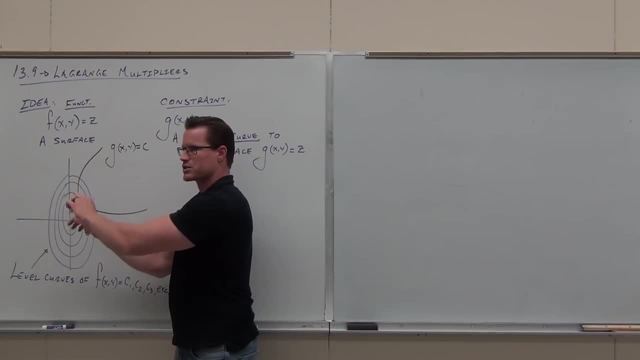 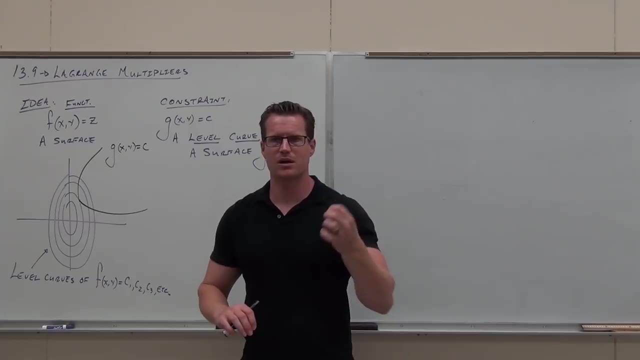 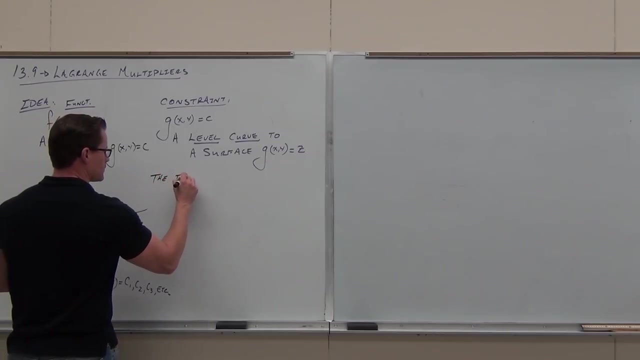 And either one It's going to be higher or lower than that point. So this right here, That right there Gives us Where these things intersect, Give us constrained maximum or constrained minimum. Okay, What you're missing has to be oil seeping in here. 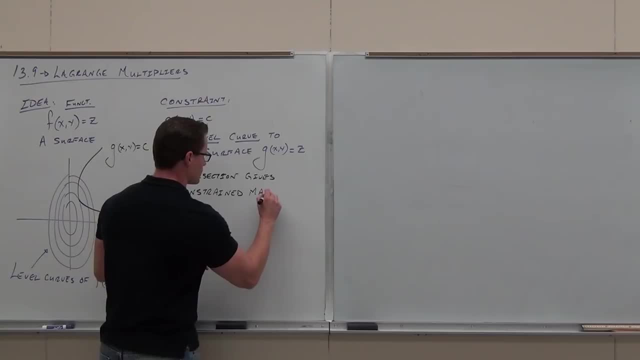 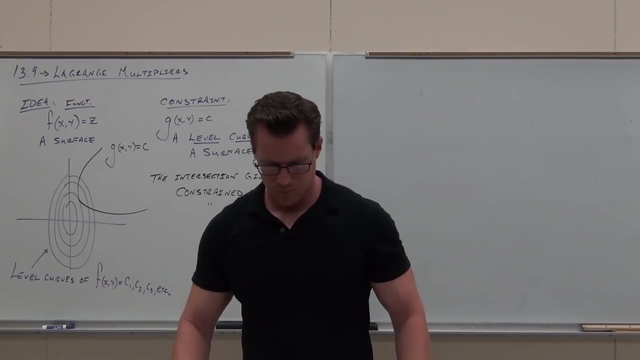 So this is your maximum. What was it? We'll see what it is Okay. So all these vezes, God is making the sun go down the side, fixed something up the pretty part and making that thing comes to sound. This gonna be the end of your afternoon course. 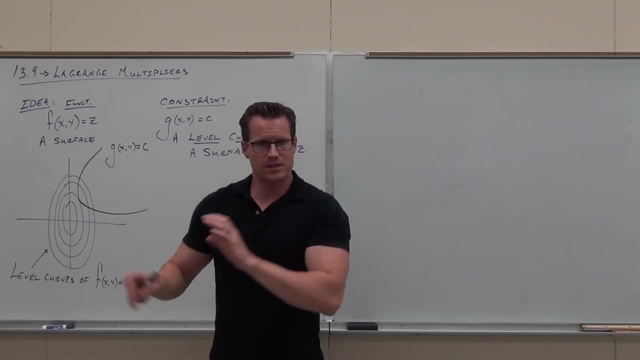 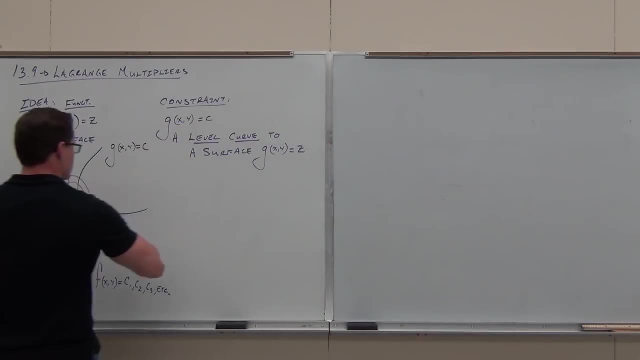 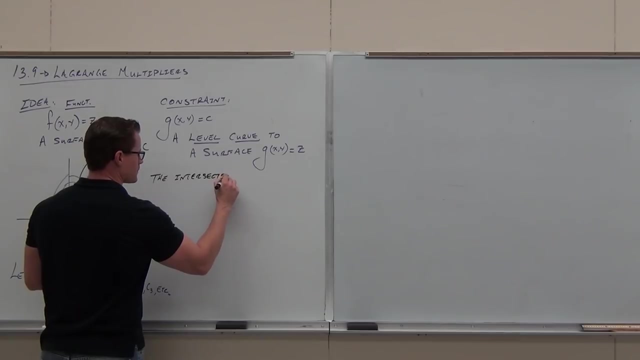 So this right here, that right there gives us where these things intersect, give us constrained maximum or constrained minimum. Let's now go back. We are going to try a little bit more different. Here. we have something in the middle Sighted. 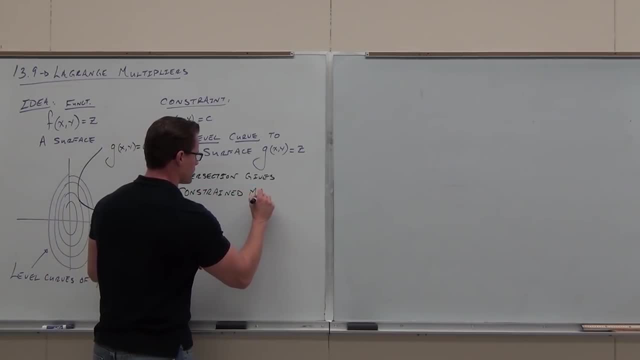 Something like this: right here I'll give you a different angle. See, here It's a little bit lower. Here it's a little bit lower. See, It's a little bit lower. Okay, Let's have a little more of this. 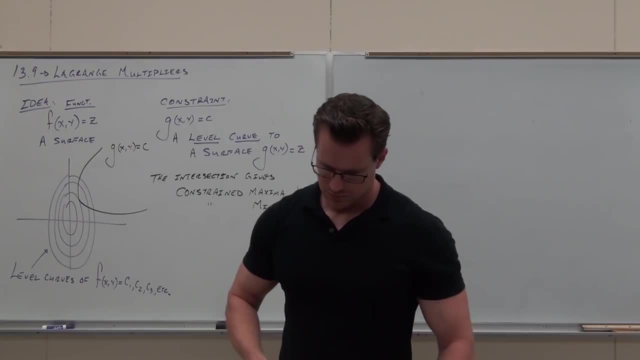 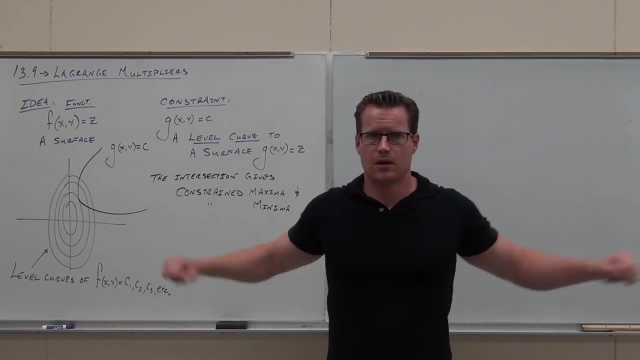 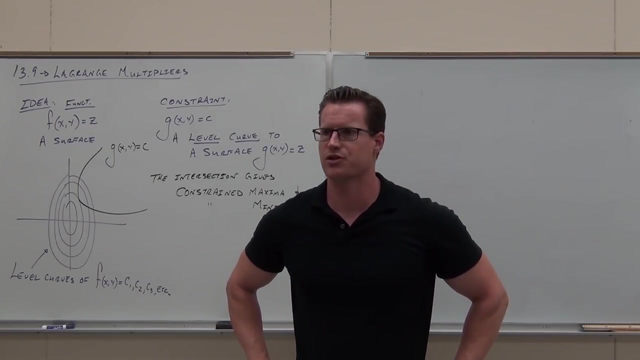 One, Two, Three, Four, Five, Six, Seven, Eight, Nine, Ten, Eleven, Twelve. I'm ready for it. Are you ready for it? This could blow your minds. This blow is going to crush your heads. 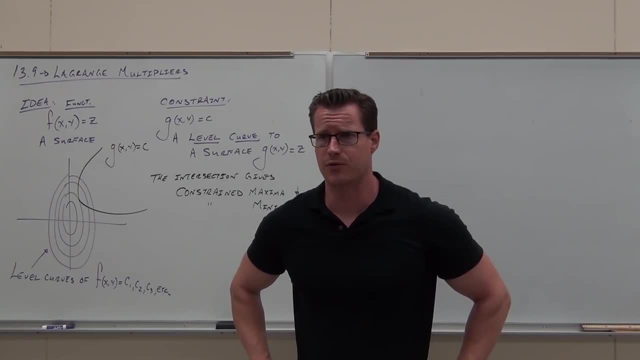 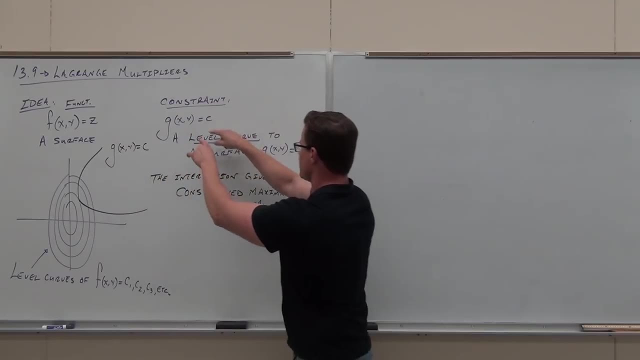 Ready. You're going to love it Because it's going to put all of chapter 13 completely together for you, Promise. You've got to stick with me. Number one: do you guys get the surface level curves? This is a level curve of some surface. 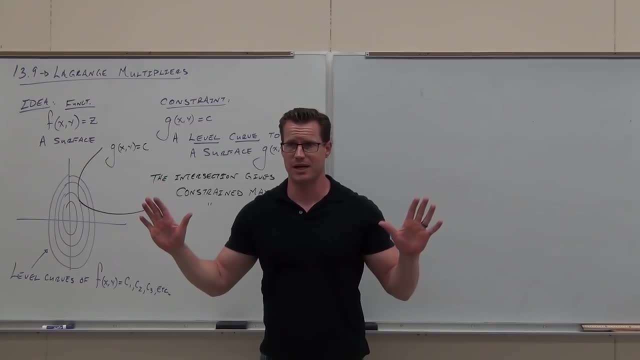 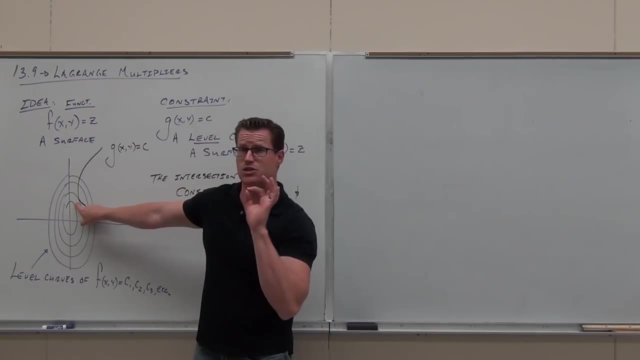 and the level curves are going to intersect if we're going to have any solutions. Do you guys get it? Do you understand the concept that if we bounce off, if these level curves are falling or climbing, that guy right, there is going to be an absolute max or an absolute min for that constraint. 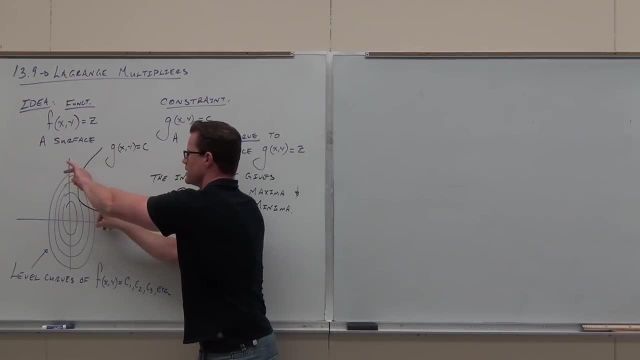 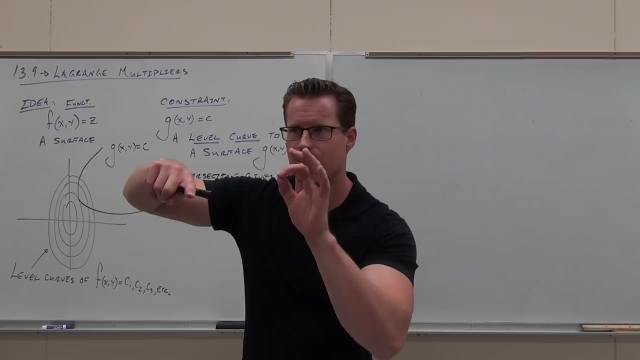 Do you get it? Don't know which one, but these are giving us different intersections, different outcomes. Check it out. We're looking for the one that we bounce off of. Now how about this? If we bounce off, if the level curves, bounce off each other? 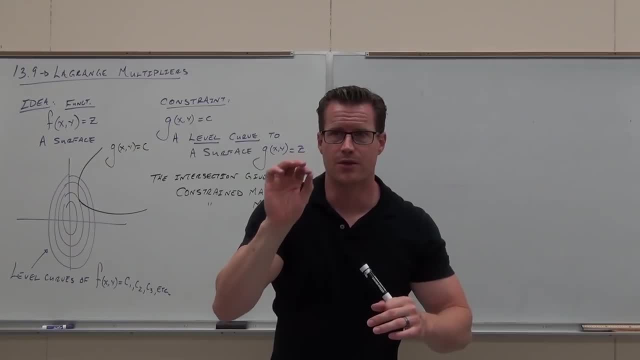 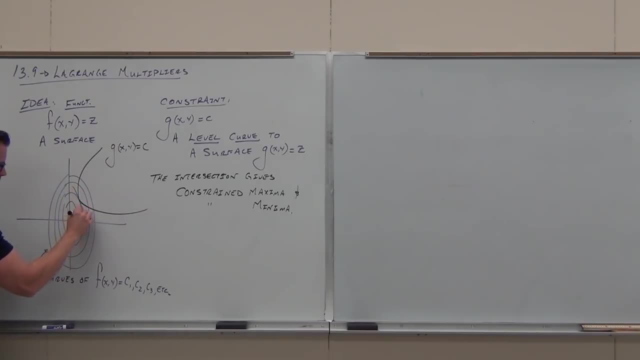 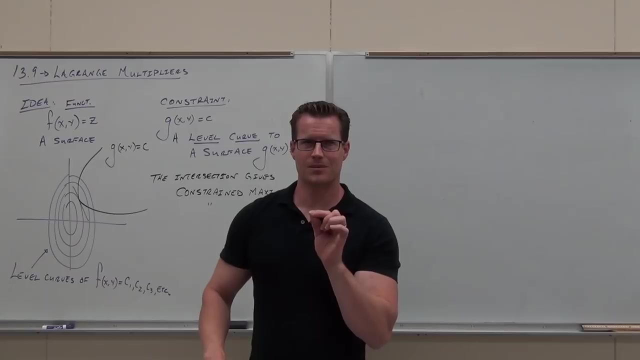 if two curves intersect at one and only one point, they share a common tangent, Or at least at least their tangents are scalar multiples. I'm not writing all this down. You're going to have to listen to it a couple times if you don't catch it. 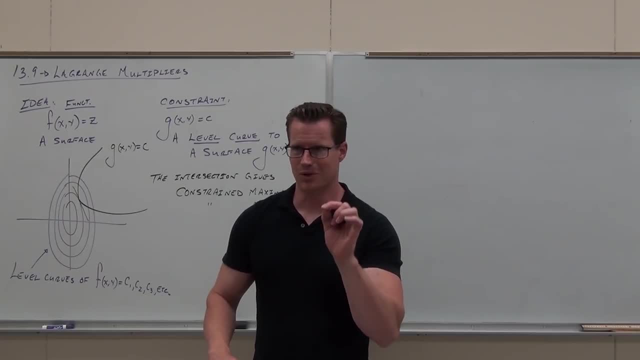 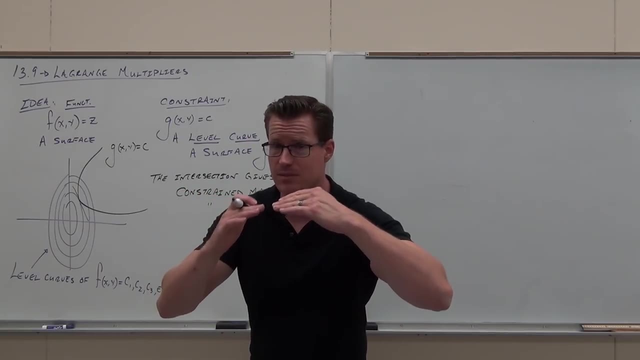 I don't have time. Their tangents are scalar multiples, Do you get it? But here there's more. Oh my gosh, there's more, There's more. If they have the same tangent, tell me something about their normals. 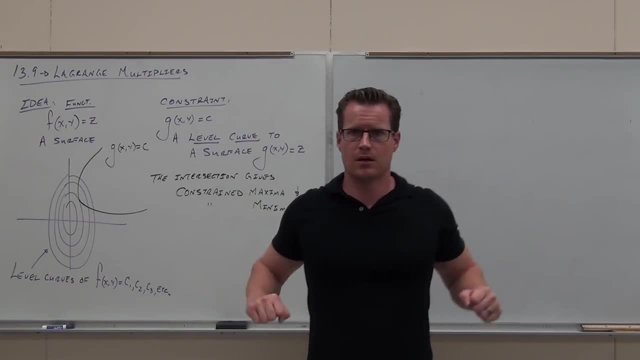 See you guys later. All right, Bye, Let's go. Bye. Thank you. Thank you, Excuse me, Okay, Okay, Bye, Thank you, Bye, I'm ready for it. Are you ready for it? This could blow your minds. 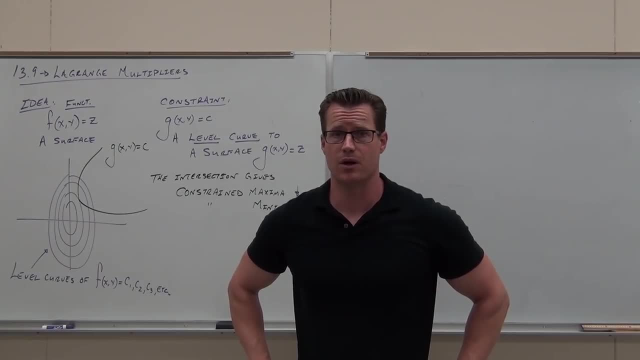 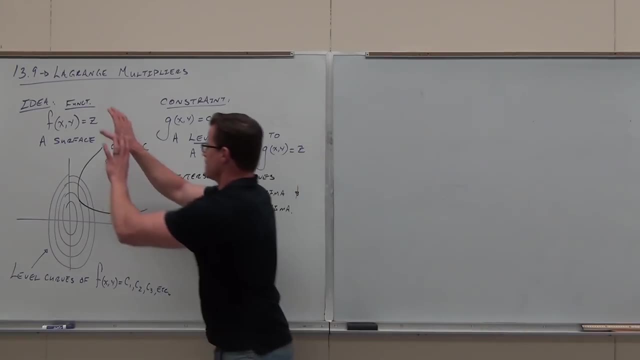 This blow is going to crush your heads Ready. You're going to love it Because it's going to put all of chapter 13 completely together for you Promise. You've got to stick with me. Number one: do you guys get the surface level curves? 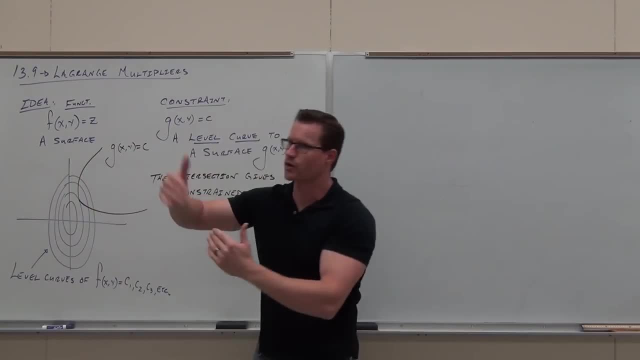 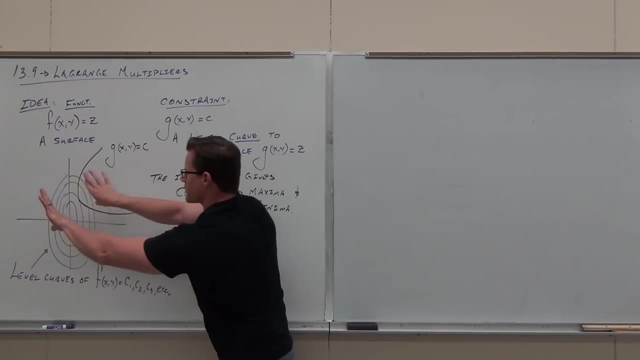 This is a level curve of some surface and the level curves are going to intersect. if we're going to have any solutions, Do you guys get it? Do you understand the concept that if we bounce off, if these level curves are falling or climbing, 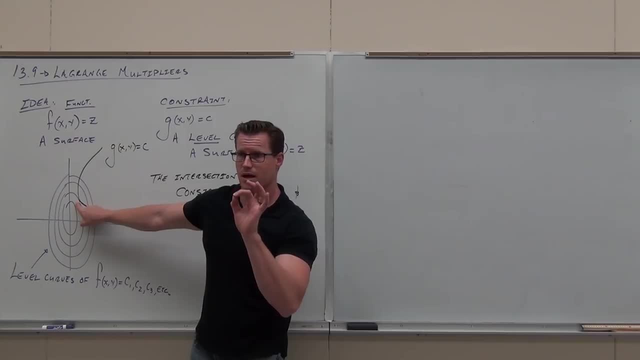 that guy right, there is going to be an absolute max or an absolute min for that constraint. Do you get it? Don't know which one, but these are giving us different intersections, different outcomes. Check it out. We're looking for the one that we bounce off of. 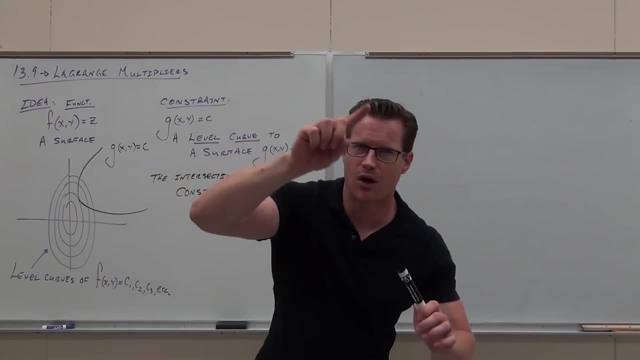 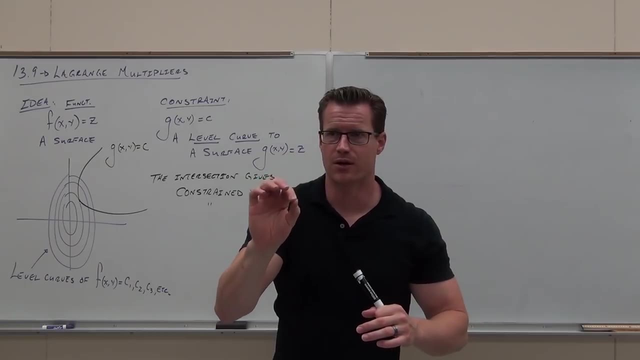 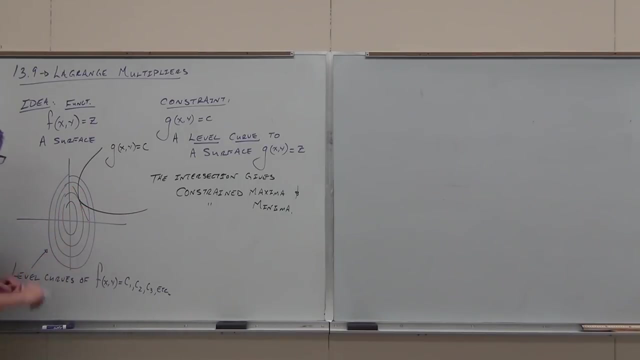 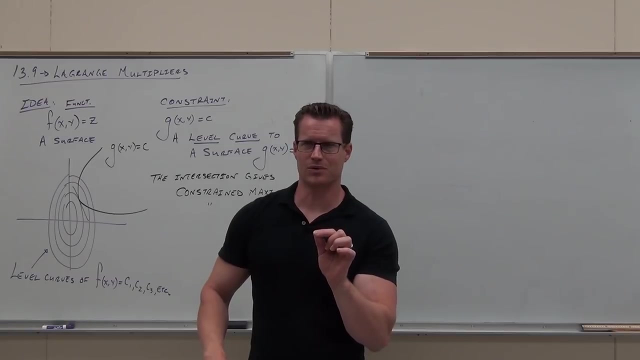 Now, how about this? If we bounce off, if the level curves bounce off each other? if two curves intersect at one and only one point, they share a common tangent, Or at least, at least, their tangents are scalar multiples. 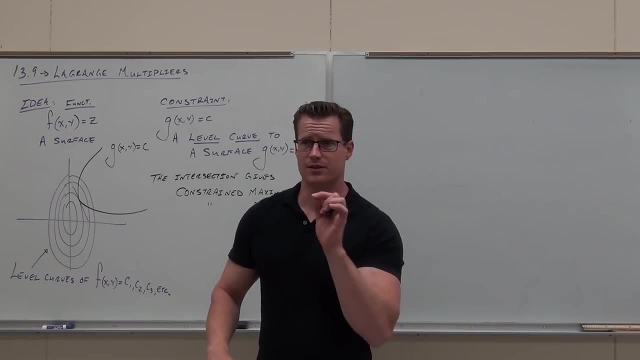 I'm not writing all this down. You're going to have to listen to it a couple times if you don't catch it. I don't have time. Their tangents are scalar multiples, Do you get it? But here there's more. 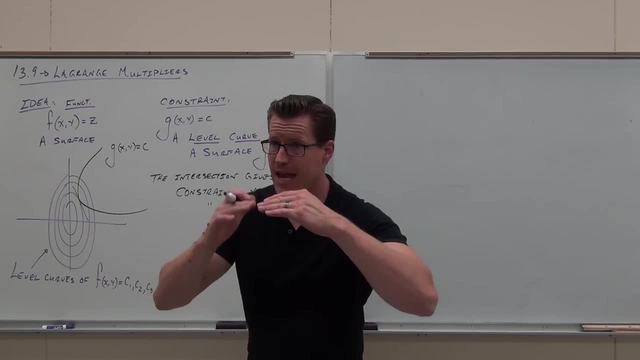 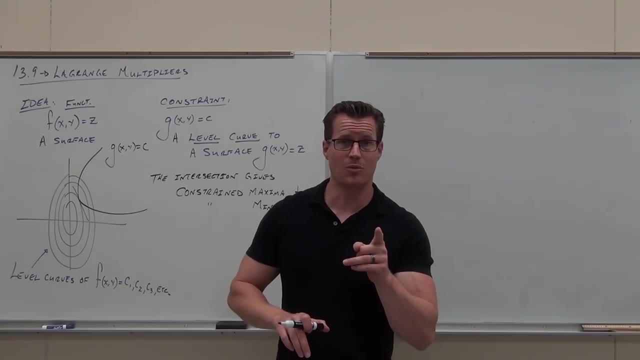 Oh my gosh, there's more. There's more If they have the same tangent. tell me something about their normals. Same normals, Do you get that? if they bounce off each other, they have a common tangent? If they bounce off each other, they also have a common normal. 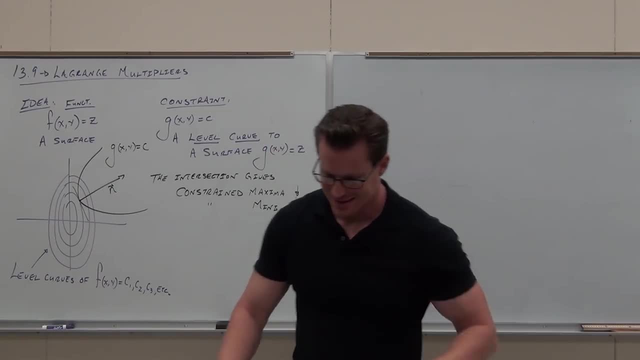 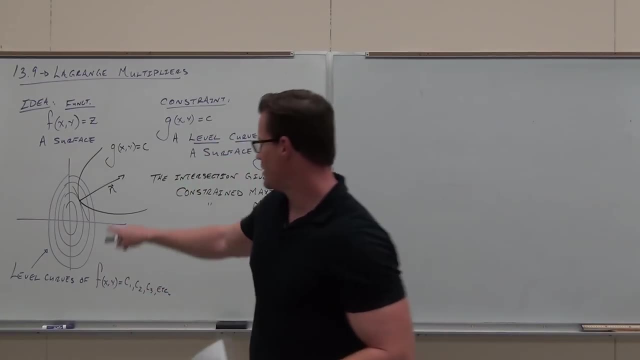 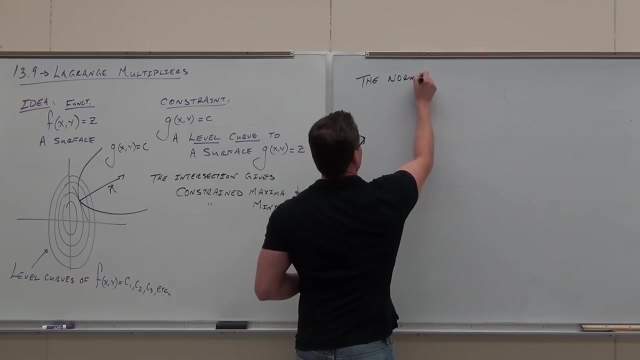 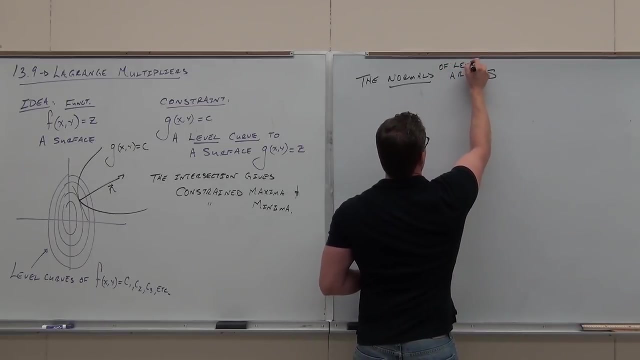 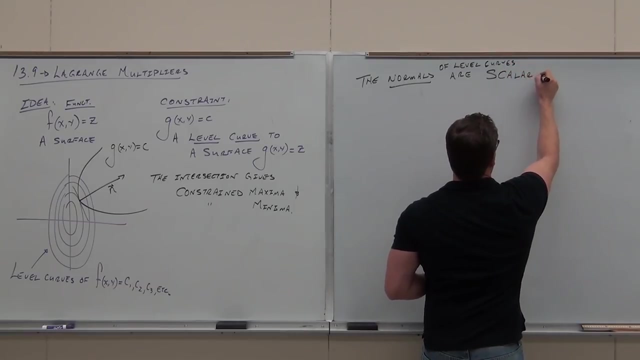 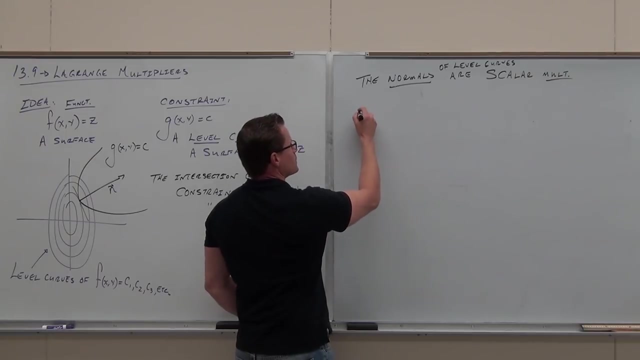 They have a common normal vector, Or at least the normals are scalar multiples. I'm sorry, the normals of the level curves are scalar multiples. Here's the magic. Here's the magic. Keep on saying that. Here it is. So the normals. 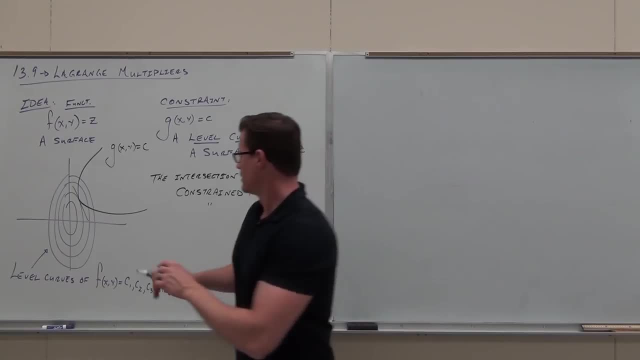 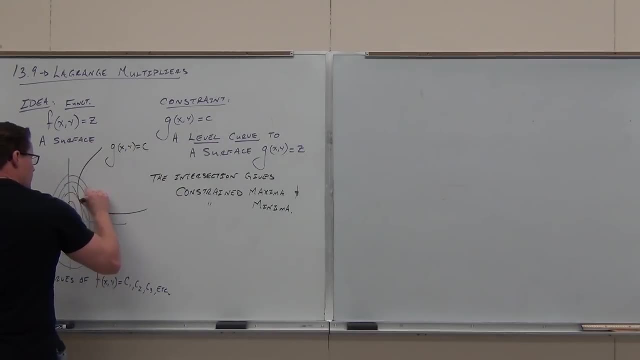 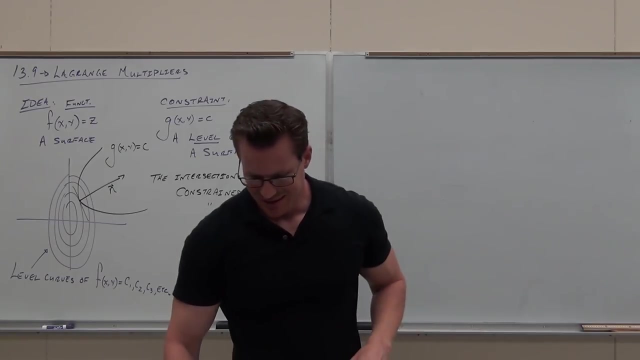 Same normals. Do you get that? if they bounce off each other, they have a common tangent. If they bounce off each other, they also have a common normal. They have a common normal vector, Or at least the normals are scalar multiples. 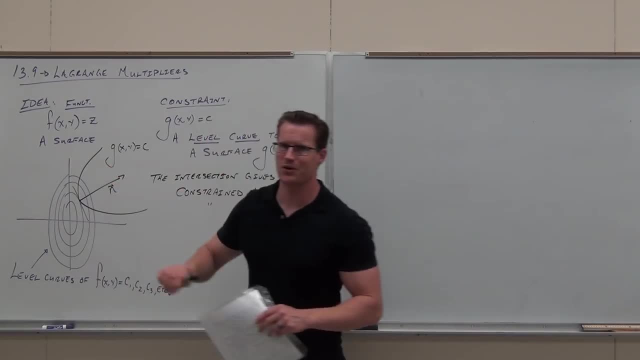 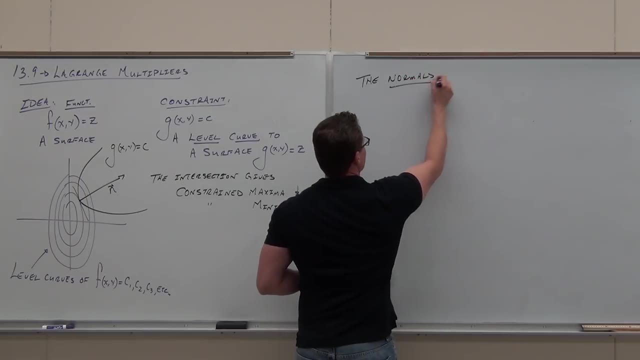 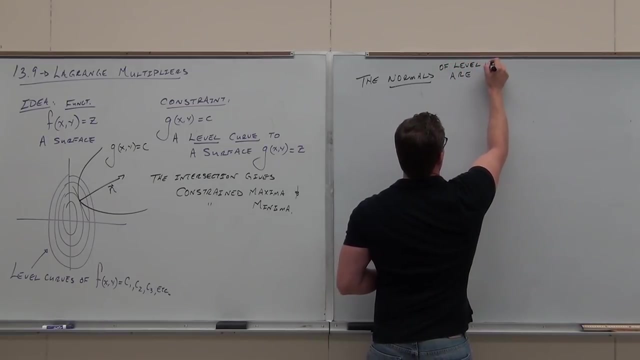 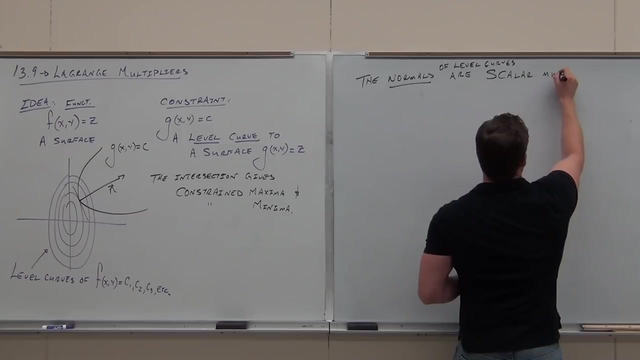 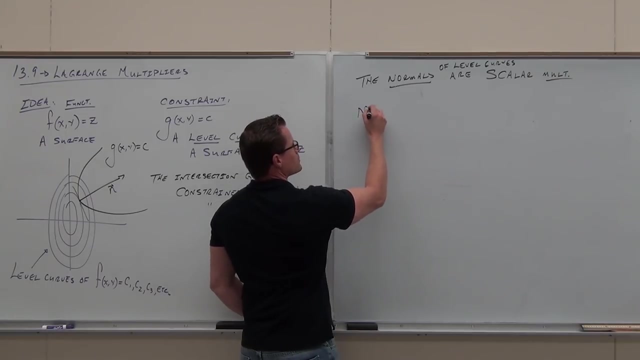 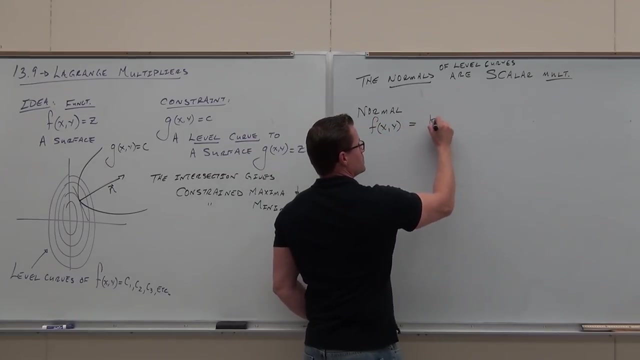 I'm sorry. the normals of the level curves are scalar multiples. Here's the magic. Here's the magic. Keep on saying that. Here it is. So the normals. The normal for this surface is equal to K times. Let's call it a constant, for right now. 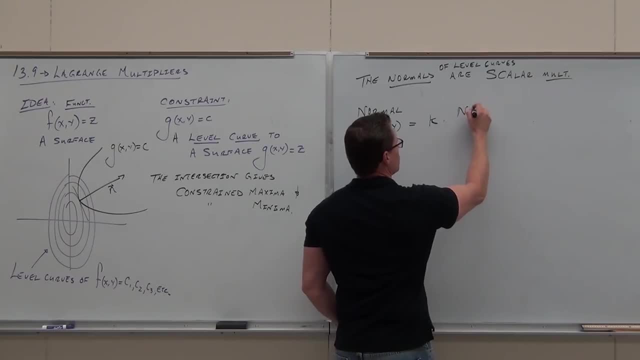 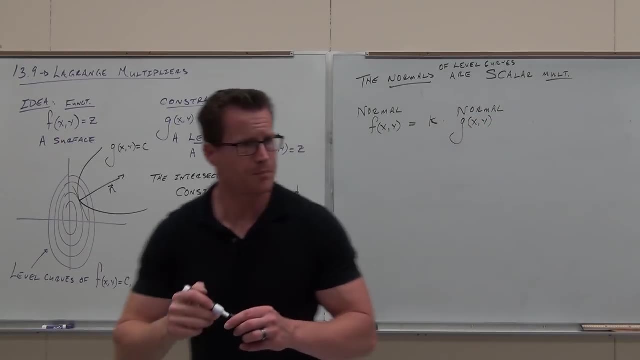 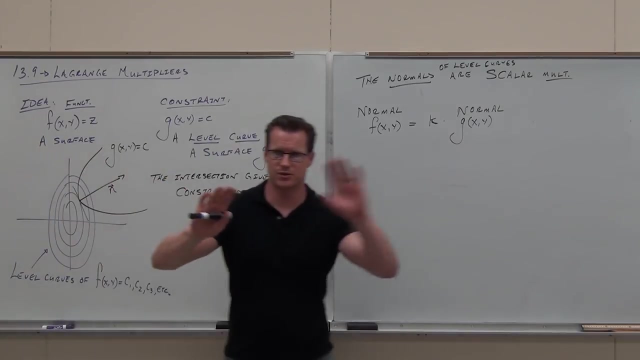 I'm going to change it to a constant in just a second- K times the normal- to this function. Bear with me. Level curves of F. The level curve: Listen, listen, Don't wait for a second before you write that down. 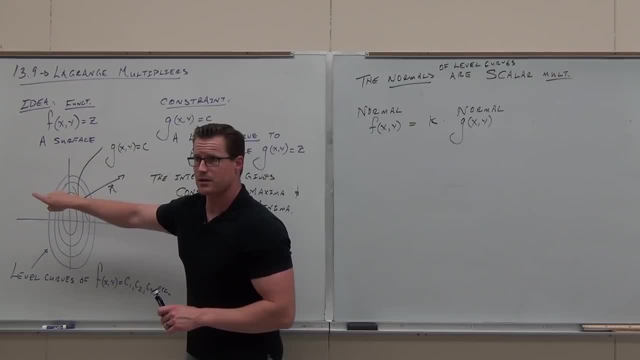 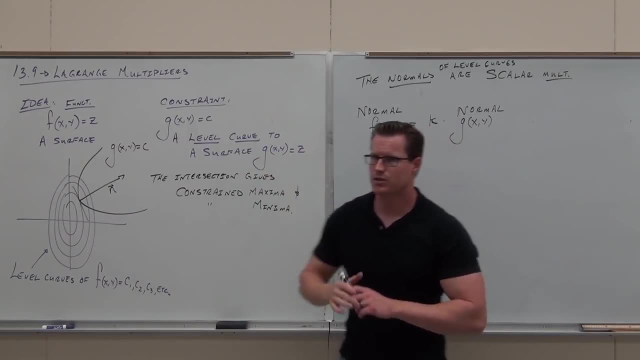 I need your eyes right here. The level curves of F correct The one level curve we care about for G. This level curve Is a level curve of some higher function, So the normals for this function are scalar, multiple, Just K times, just constant. 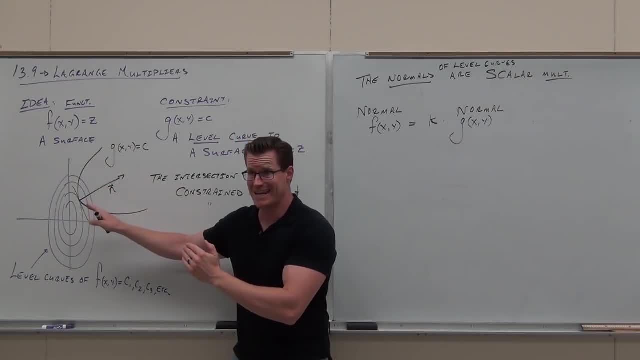 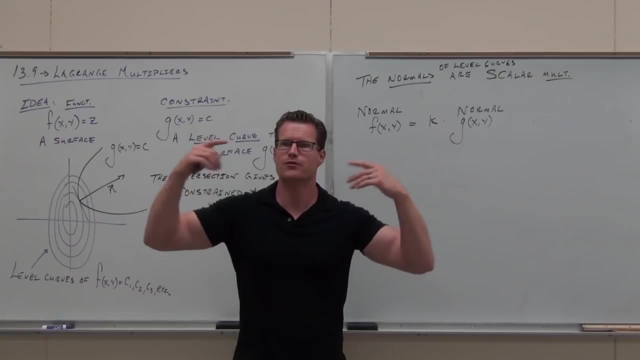 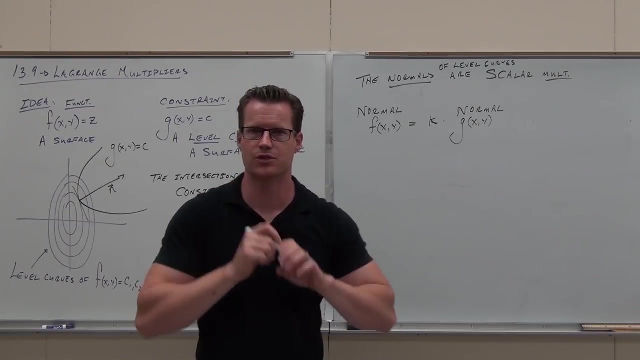 Times the normal to this function. That's saying that their level curves have the same normal, Or scalar multiple the same normal. And now put all of your knowledge of all this chapter together. What gives you normals to level curves, Normals of the level curves. 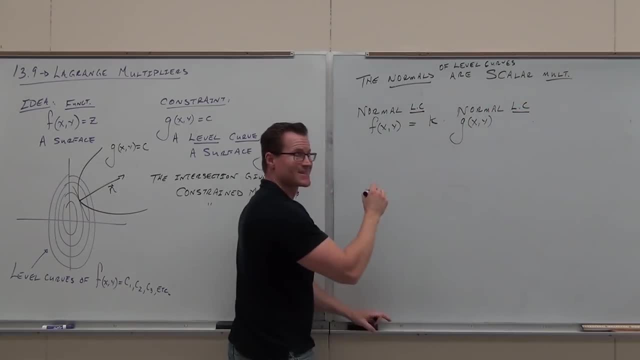 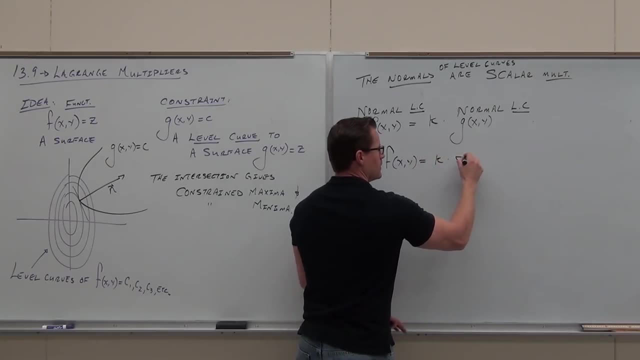 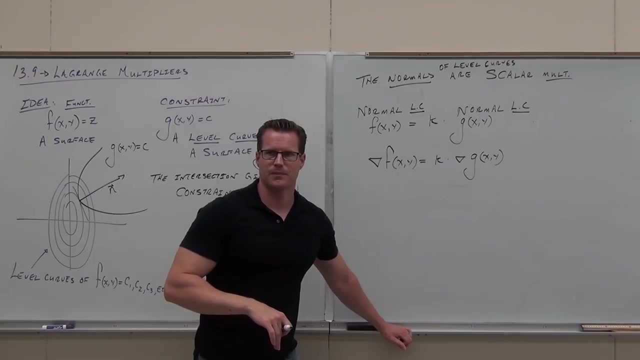 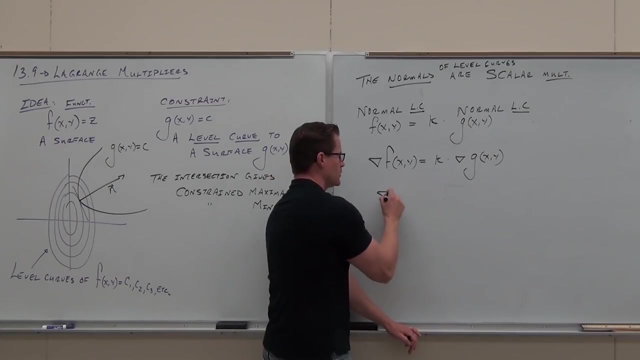 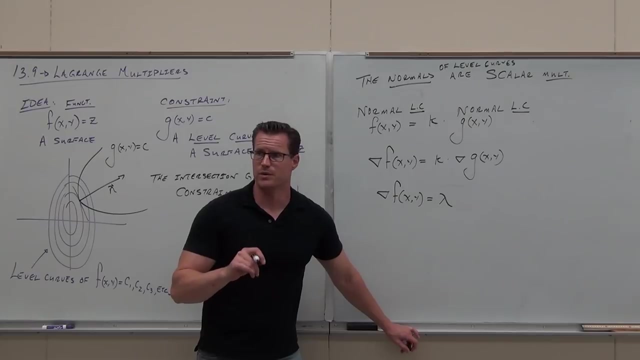 That means the gradient for F must be a scalar multiple of the gradient of G, Has to be. Here's what we call that constant. That scalar multiple has a special name. That scalar multiple is called lambda. And that right, there is what we define as the Lagrange multiplier. 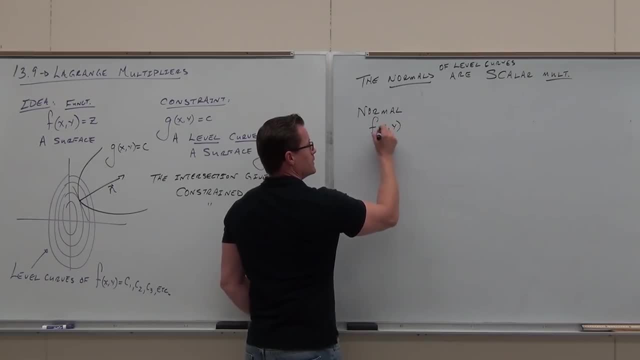 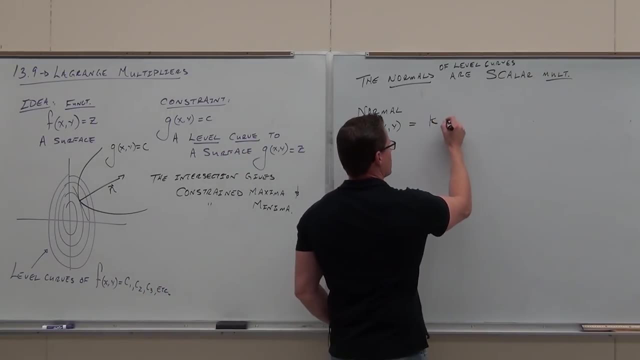 The normal for this surface is equal to K times. Let's call it a constant for right now. I'm going to change it to a constant in just a second. K times the normal to this function. Bear with me. Level curves of F. 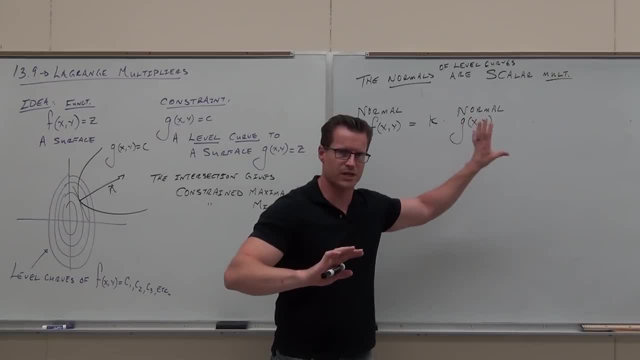 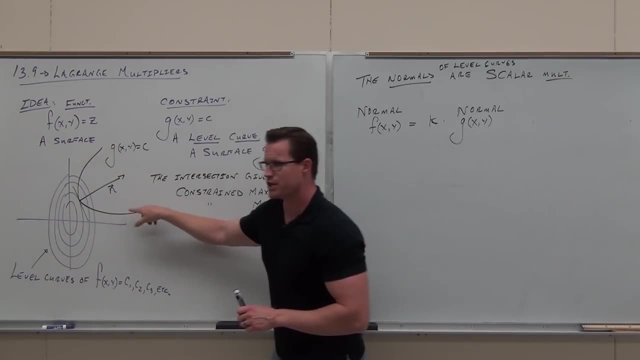 The level curve. Listen, listen, Don't wait for a second before you write that down. I need your eyes right here. The level curves of F correct The one level curve we care about for G. This level curve Is a level curve of some higher function. 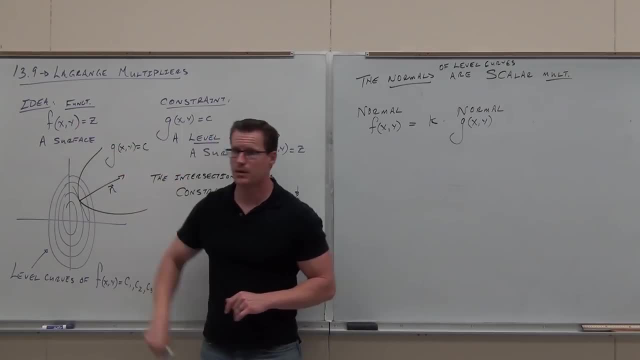 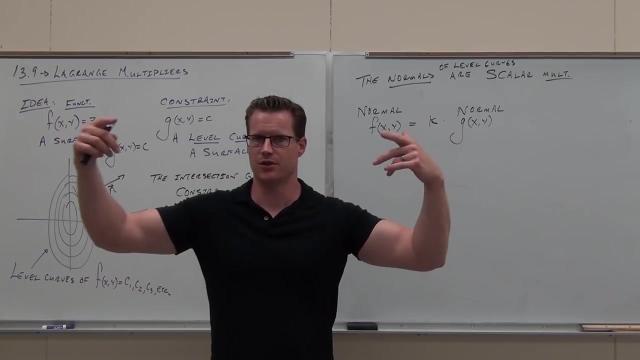 So the normals for this function are scalar multiple- Just K times, just constant Times the normal to this function. That's saying that their level curves have the same normal, Or scalar multiple, the same normal. And now put all of your knowledge of all this chapter together. 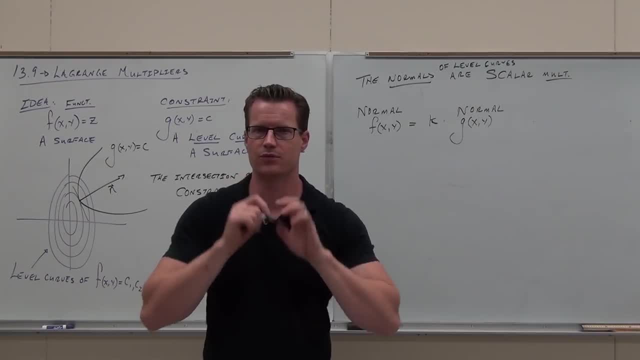 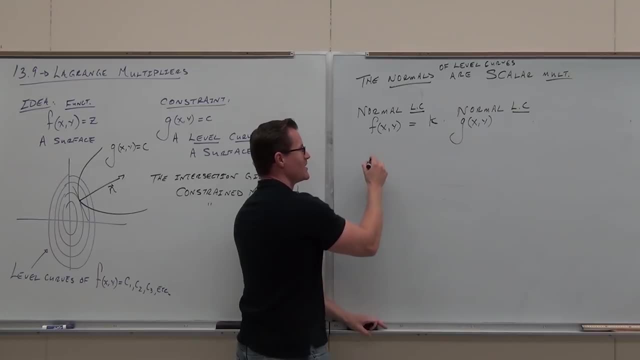 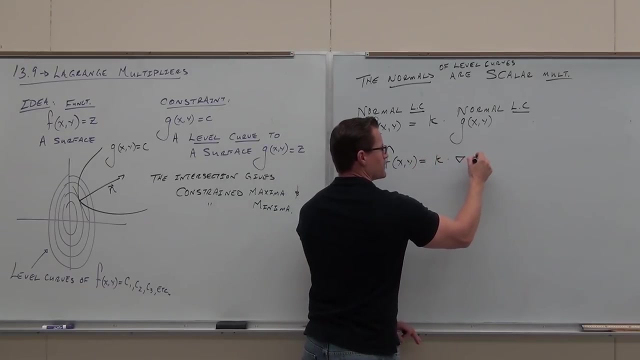 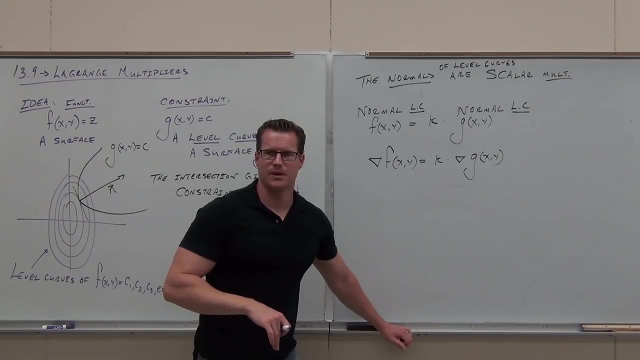 What gives you normals to level curves, Normals of the level curves? That means the gradient for F must be a scalar multiple of the gradient of G, Has to be. Here's what we call that constant. That scalar multiple has a special name. 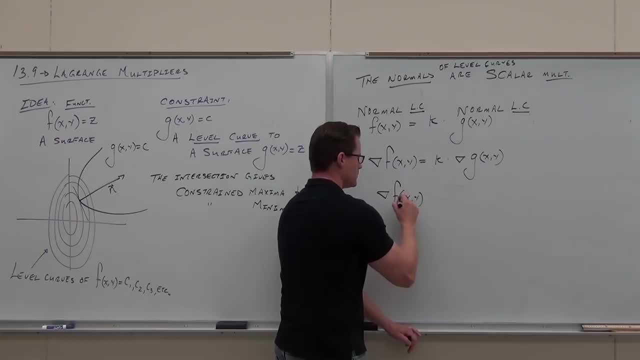 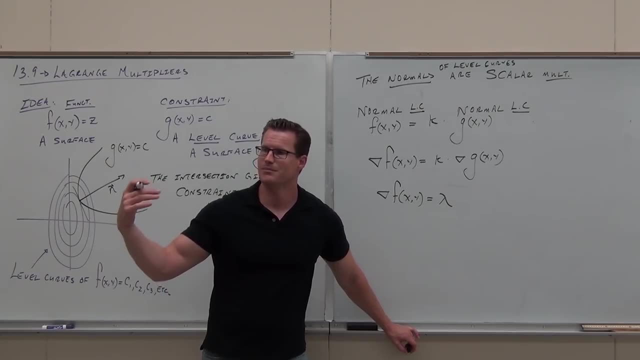 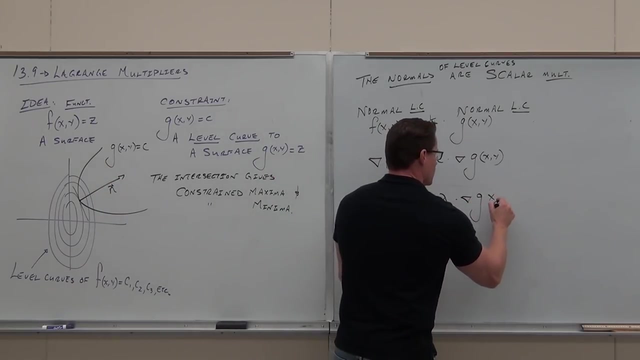 That scalar multiple is called lambda And that right there is what we define as the Lagrange multiplier, Multiplier, Scalar multiple, The Lagrange multiplier- That's what it is. The most important part is that this can be extrapolated for three dimensions. 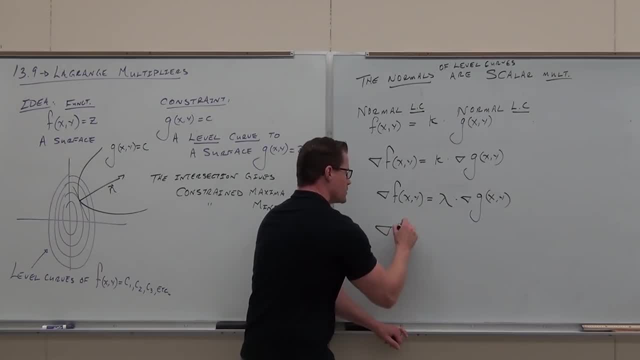 Which means that when you get optimization with three dimensions, you don't have to change a variable anymore, Because gradients work like that. gradients give you normals of level curves or level surfaces And since those normals have to be identical, or at least scalar multiples, 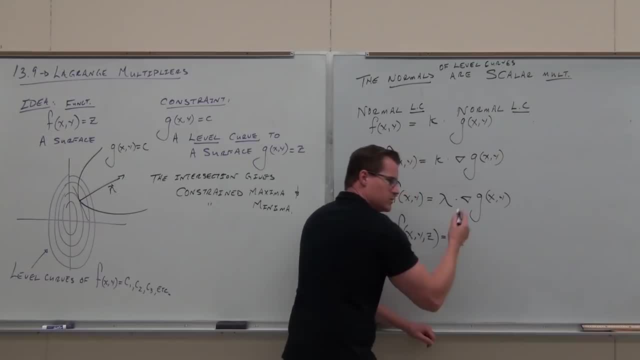 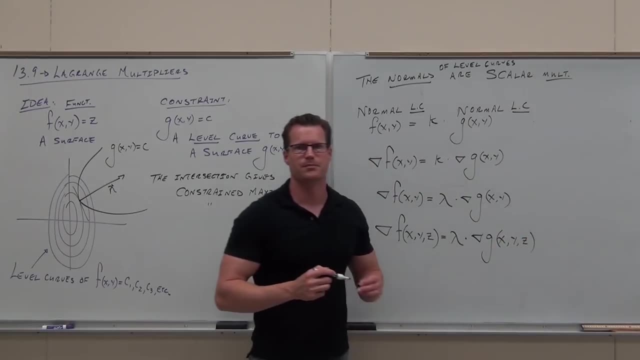 we get. the gradient for F has to be a scalar multiple. We call it Lagrange multiplier For the gradient of G, No matter how many variables I have. That is fantastic. Level curves have to intersect. We're looking for the one that bounces off. 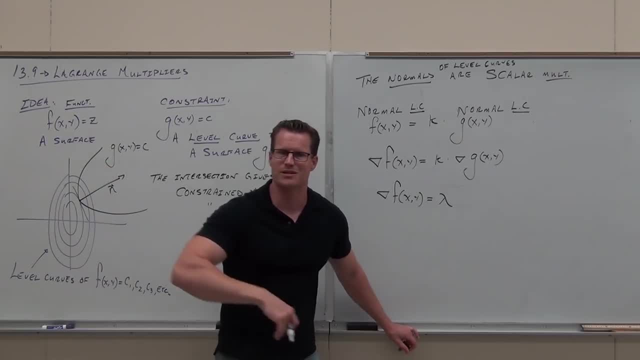 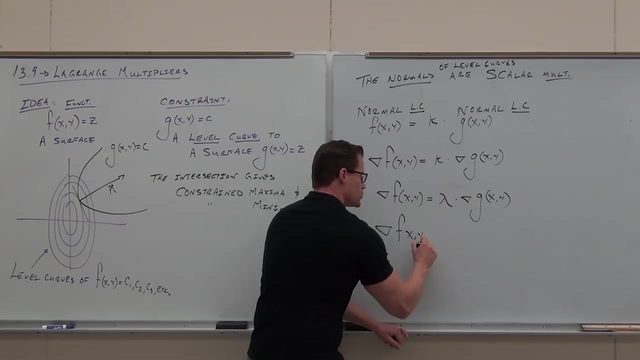 Multiplier- Scalar multiple, The Lagrange multiplier. That's what it is. The most important part is that this can be extrapolated for three dimensions, Which means that when you get optimization with three dimensions, you don't have to change a variable anymore. 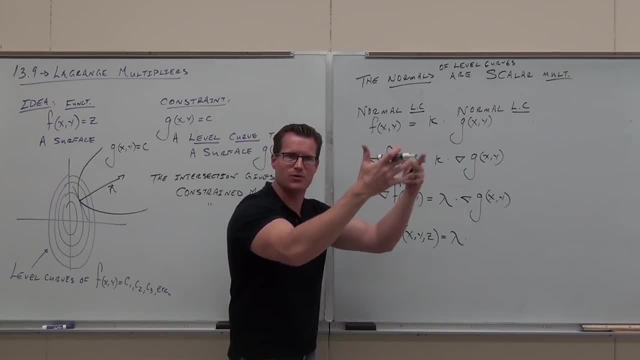 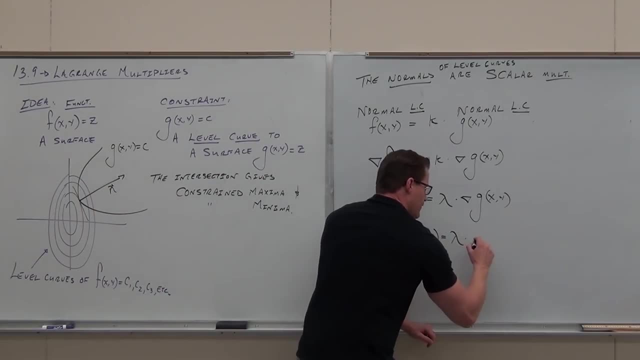 Because gradients work like that. gradients give you normals of level curves or level surfaces And since those normals have to be identical or at least scalar multiples, we get the gradient, for F has to be a scalar multiple, We call it Lagrange multiplier. 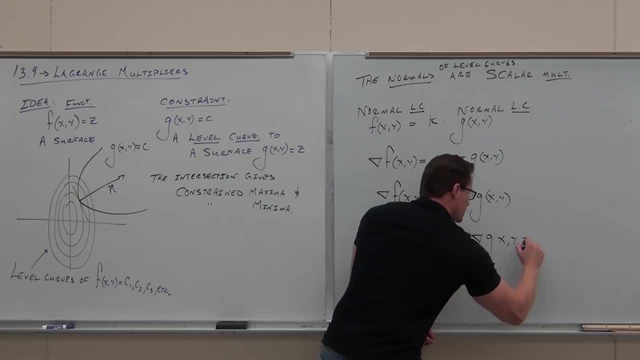 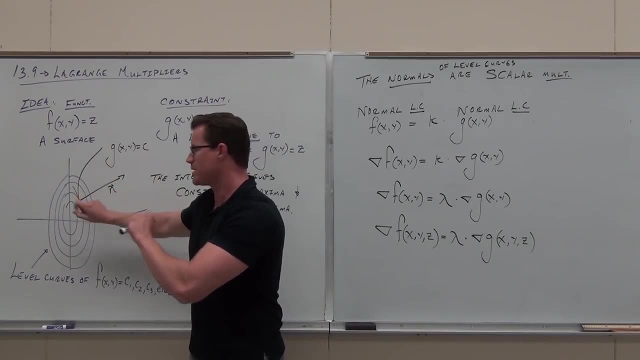 For the gradient of G, No matter how many variables I have. That is fantastic. Level curves have to intersect. We're looking for the one that bounces off. If it bounces off, it has the same tangent, Scalar multiple, Same normal. 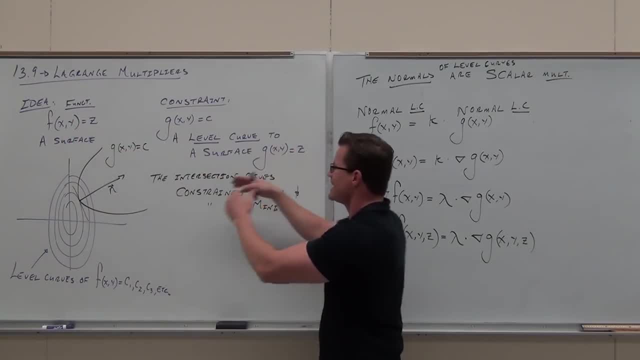 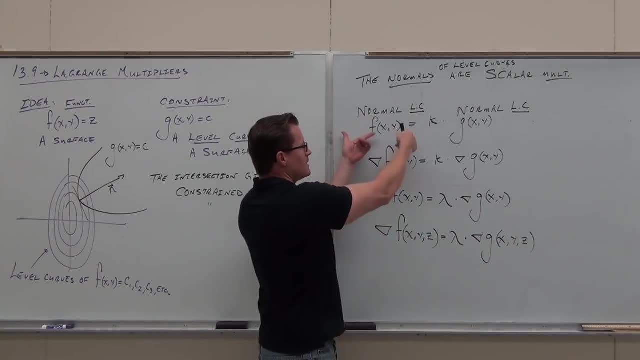 Scalar multiple. So if we go back to the surfaces that created our level curves, the gradient is the same. It gives us the normals to those surfaces. The gradient gives us the normals to the level curves. Gradient gives us normal to the level curves. 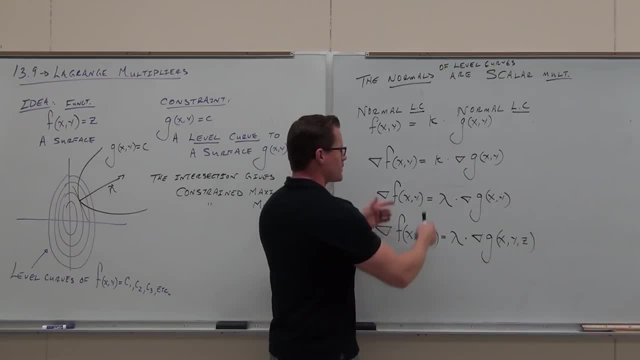 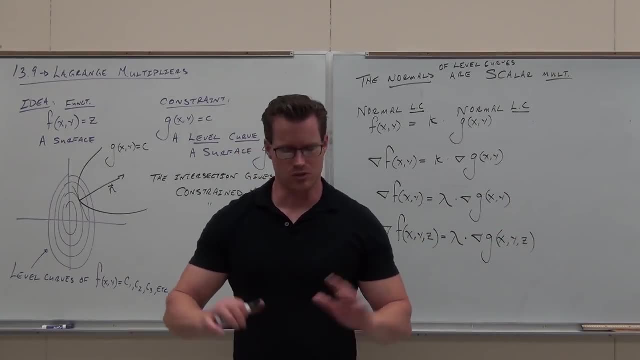 They have to be scalar multiples. We just showed why: Same tangent, same normal. Therefore we call that scalar multiple Lagrange multiplier. Now that's how we're going to start doing constraint optimization. I'll show you exactly how it's done next time. 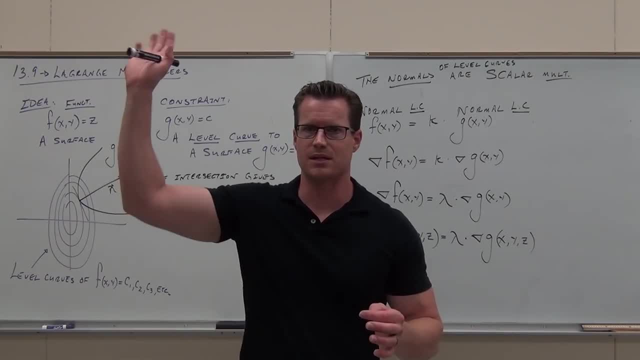 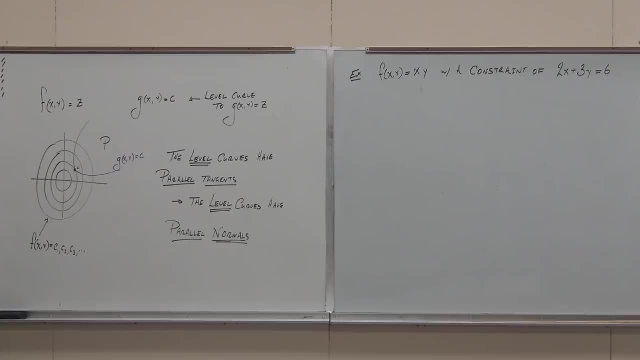 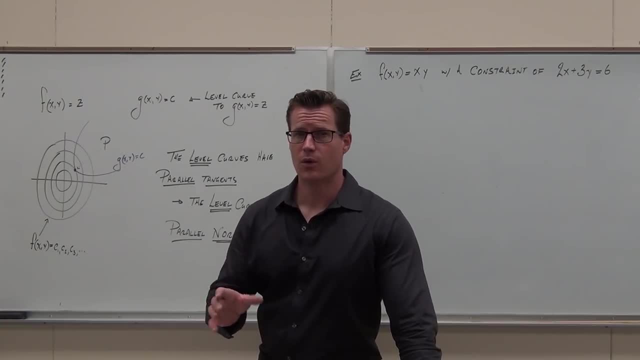 I'm going to do a little recap because I know it's been a few days for us So we're going to come back at it. It's going to be a brief recap, But here's what we're learning about Section 13.9.. 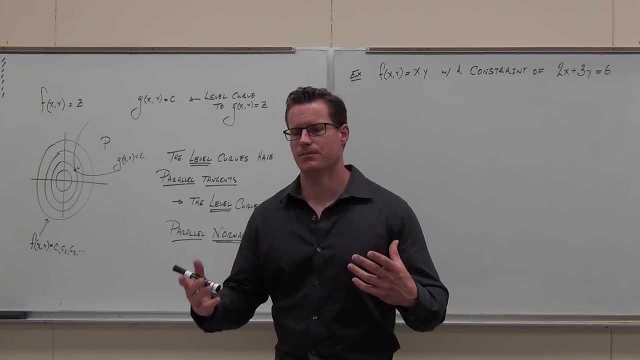 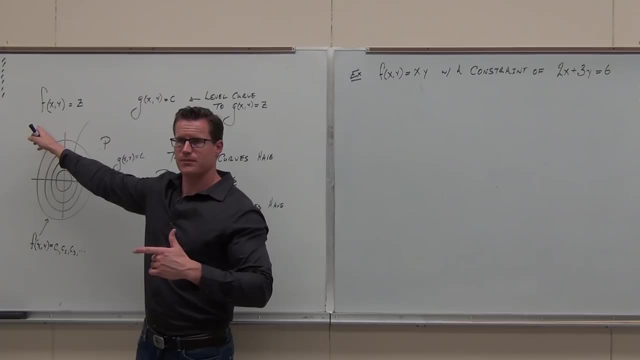 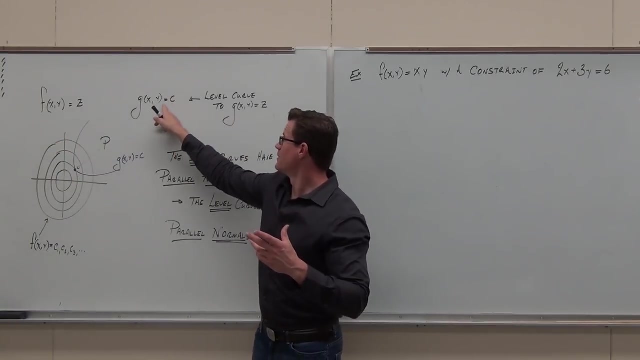 This is just the continuation of that. Here's our idea. Our idea is: suppose I give you some function, verify, it's a surface. Are you doing some lines? Yes, Okay, And suppose I give you a constraint. Well, if I give you a constraint equal to a constant, how our constraints are. 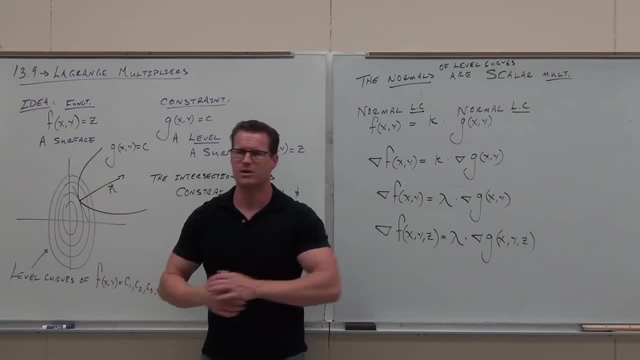 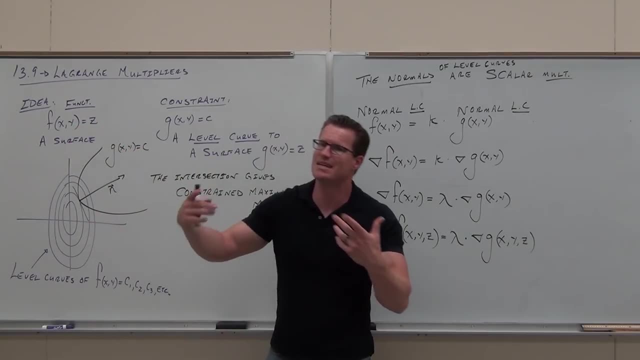 If it bounces off, it has the same tangent Scalar multiple, Same normal Scalar multiple. So if we go back to the surfaces that created our level curves, the gradient is the same. It gives us the normals to those surfaces. The gradient gives us the normals to the level curves. 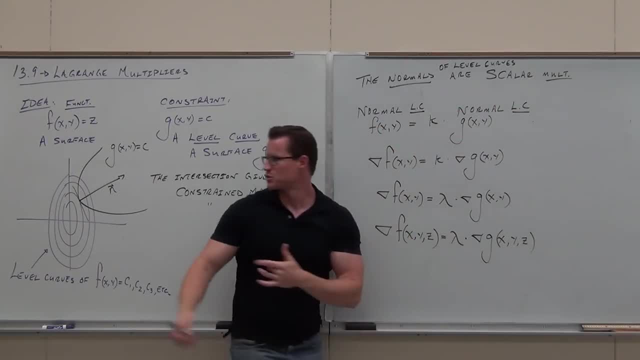 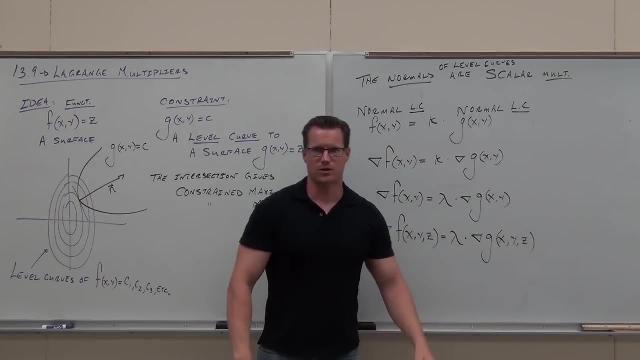 Gradient gives us normal to the level curves. They have to be scalar multiples. We just showed why: Same tangent, same normal. Therefore we call that scalar multiple Lagrange multiplier. Now that's how we're going to start doing constraint optimization. 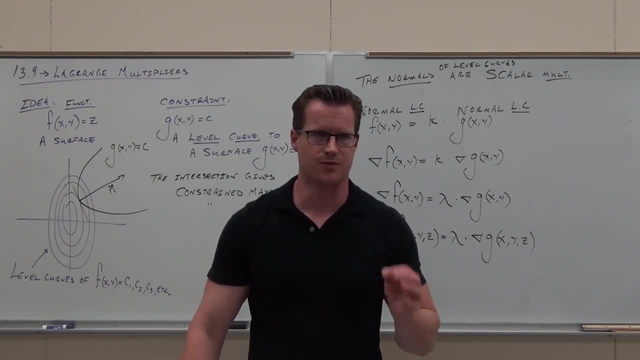 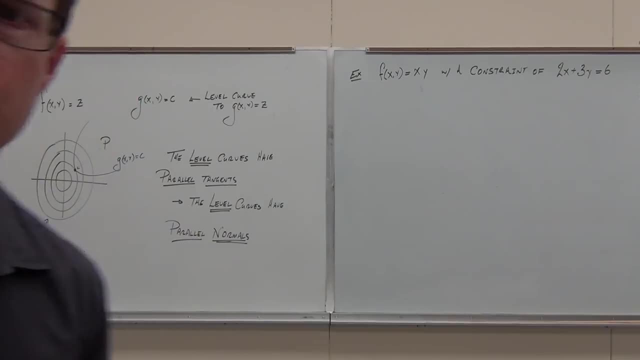 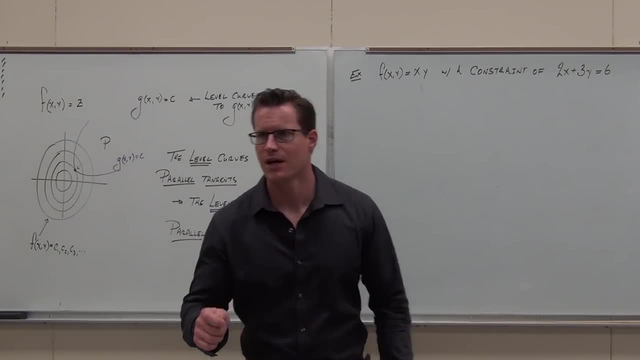 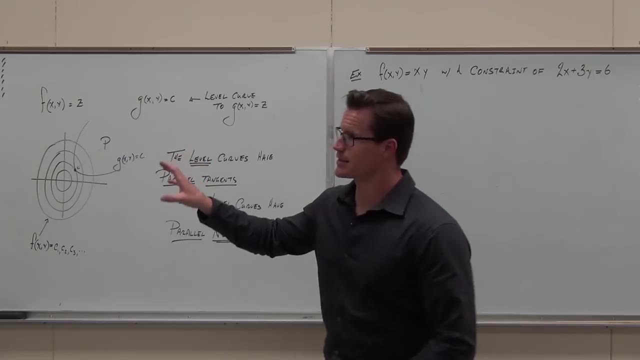 Okay, So welcome back to Lagrange multipliers and constraint optimization. I'm going to do a little recap because I know it's been a few days for us, So we're going to come back at it. It's going to be a brief recap. 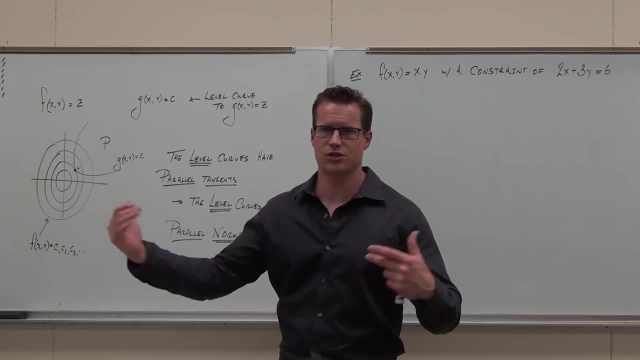 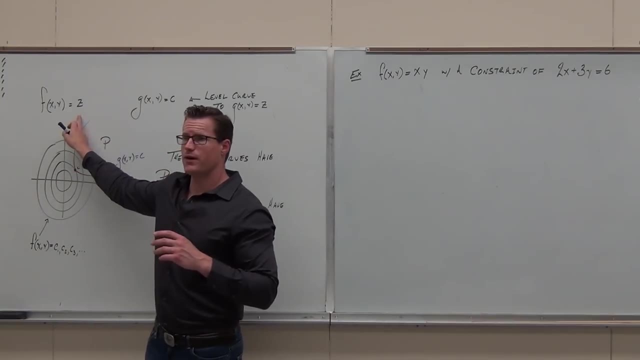 But here's what we're learning about Section 13.9.. This is just the continuation of that. Here's what, here's our idea. Our idea is: suppose I give you some function, Verify it's a surface, A surface, And suppose I give you a constraint. 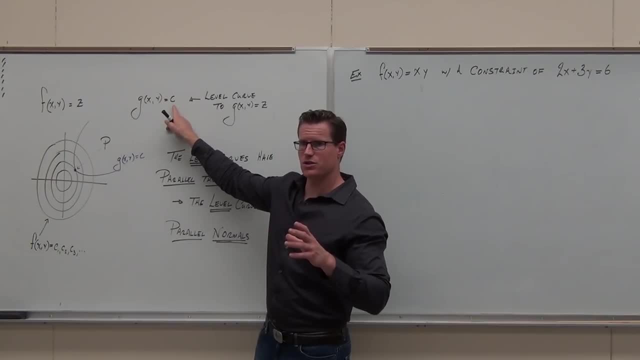 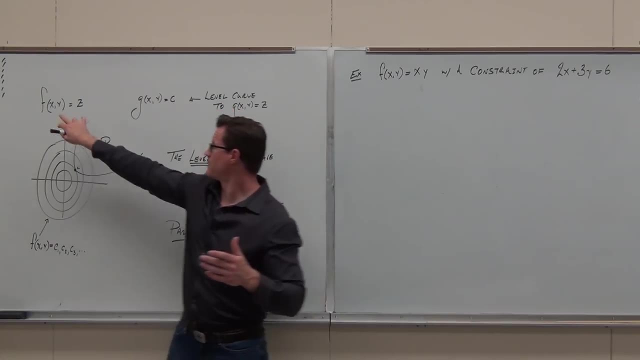 Well, if I give you a constraint equal to a constant, how our constraints are, this is a level curve to some other function, some other surface. So let's check it out. Surface, Yes, Surface, Yes. Is this going to have level curves? 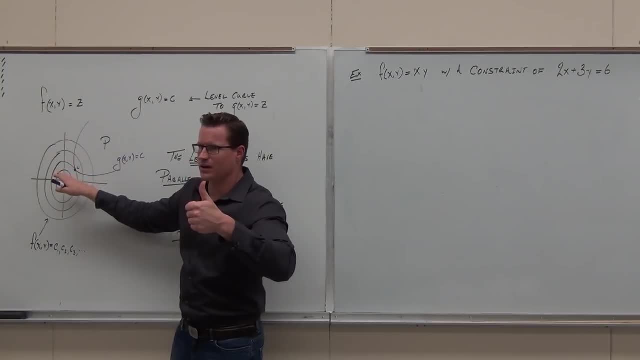 In fact, if I set this equal to a constant, I create a lot of constants. I create a lot of level curves. So take our function, our surface, set it equal to a constant. It's going to create a whole bunch of level curves. 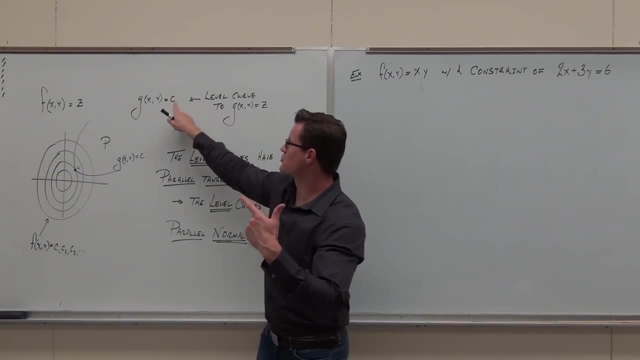 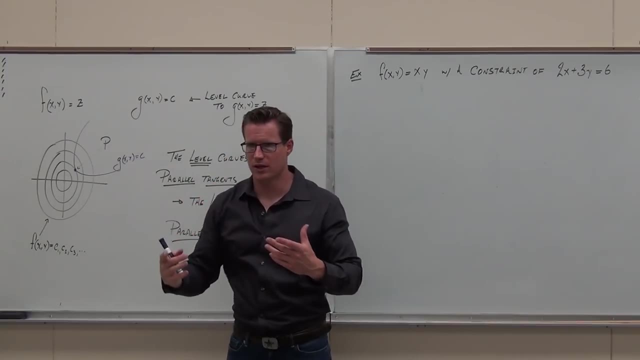 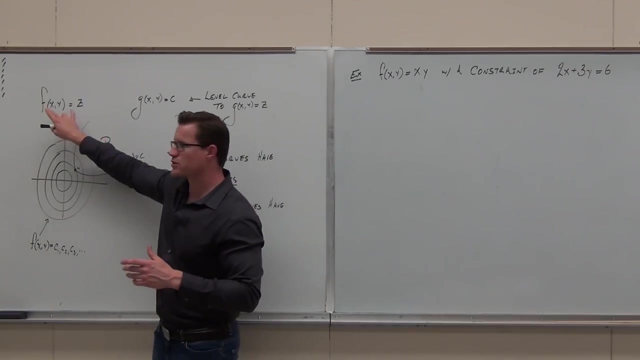 Make sense. Now, this constraint, it's already set equal to a constant. This is a specific level curve. So here's what I'm looking for with our constrained optimization: In constrained optimization, you do have to be on this surface. 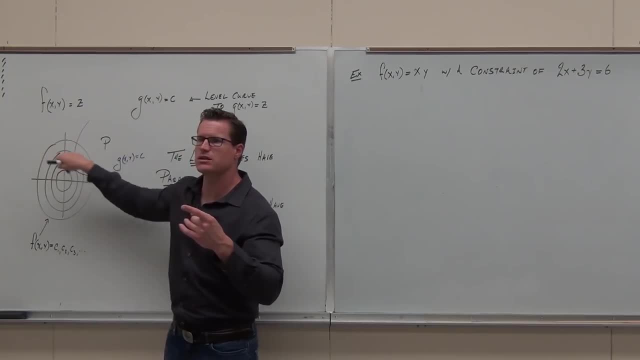 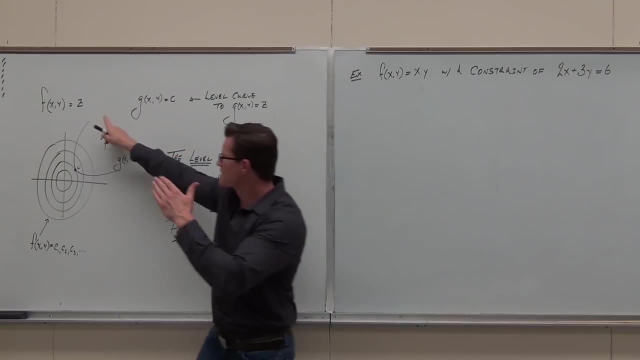 which means you're going to be on these levels, Level curves- does that make sense? But you also have to be on this constraint, So you have to be on this specific level curve. If I were to draw both of them, look, this surface has a whole bunch of level curves. okay, 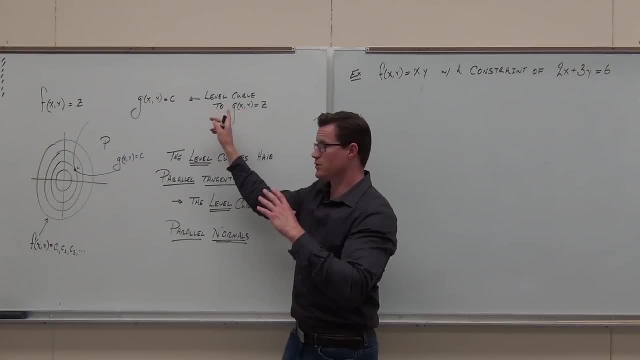 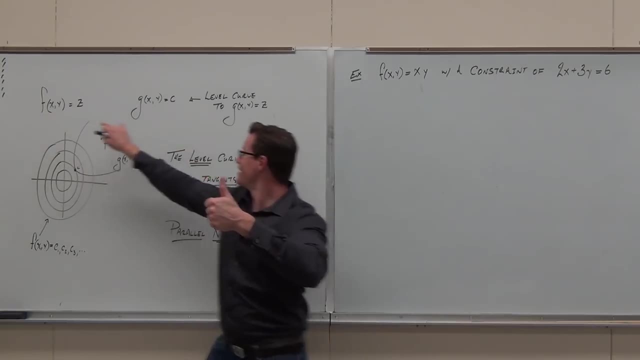 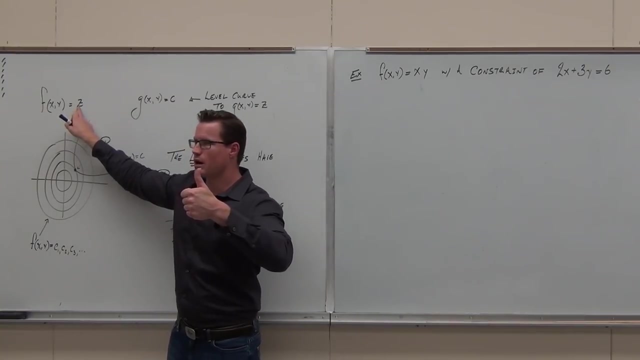 this is a level curve to some other function, some other surface. So let's check it out: Surface, Yes, Surface, Yes. Is this going to have level curves? Yes, In fact, if I set this equal to a constant, I create a lot of constants. 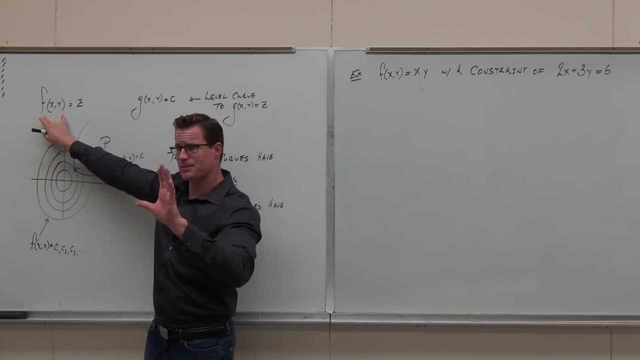 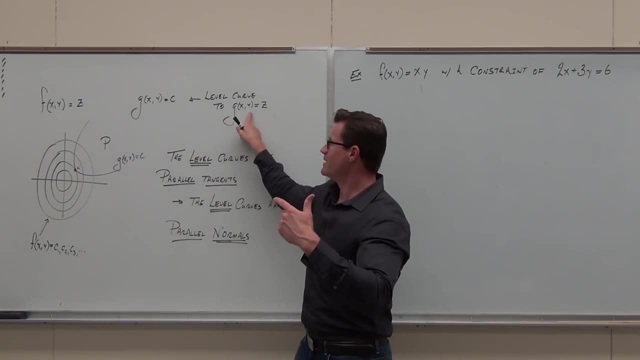 It's going to create a lot of level curves. So take our function, our surface, set it equal to a constant. It's going to create a whole bunch of level curves. Make sense Now this constraint? it's already set equal to a constant. 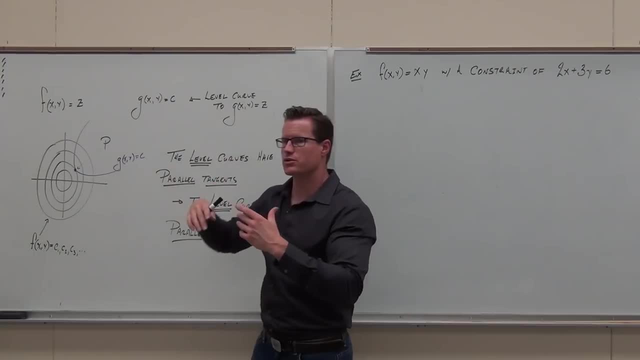 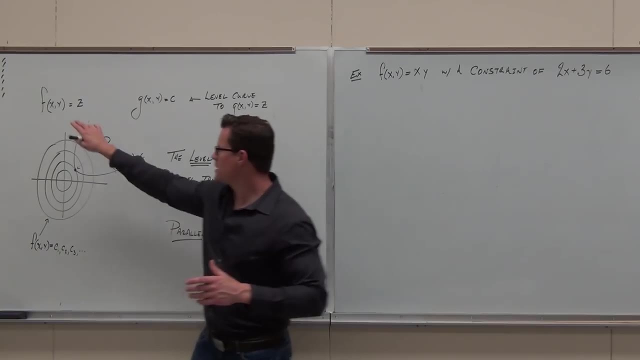 This is a specific level curve. So here's what I'm looking for with our constrained optimization. In constrained optimization, you do have to be on this surface, which means you're going to be on these levels. You have to be on these level curves. 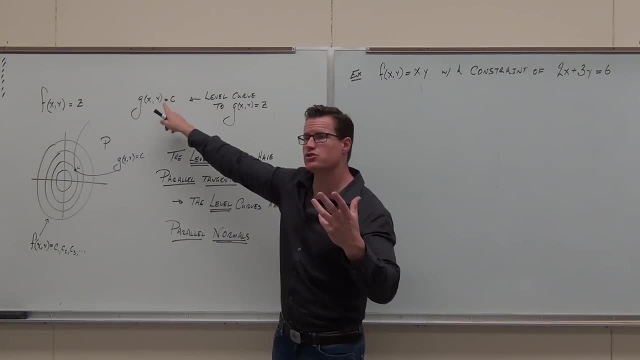 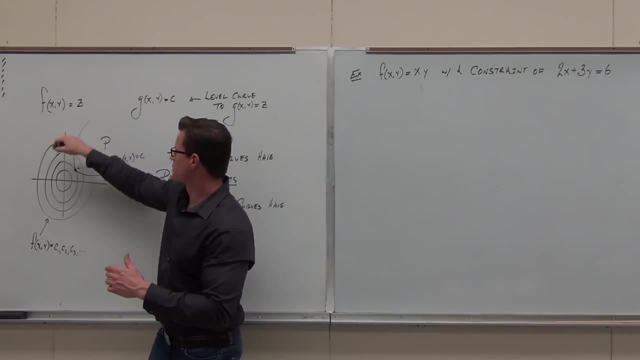 Does that make sense? But you also have to be on this constraint, So you have to be on this specific level curve. If I were to draw both of them, look, this surface has a whole bunch of level curves. This surface has a whole bunch of level curves. 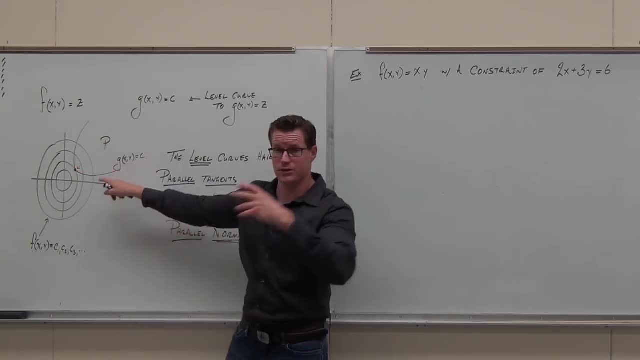 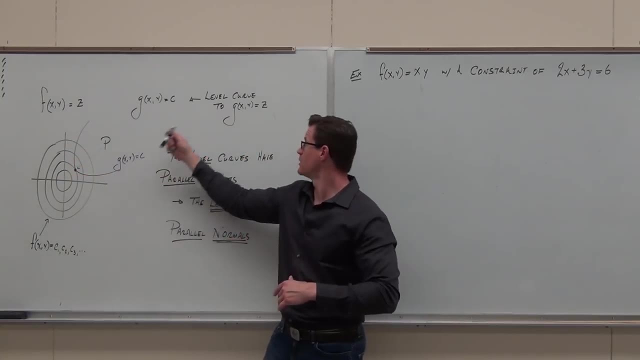 This is one specific level curve, the constraint that we have to be on. Do you guys see the difference? There's a whole bunch of level curves for this, but there's only one that I care about for that surface, The one equal to the constant that gives us that constraint. 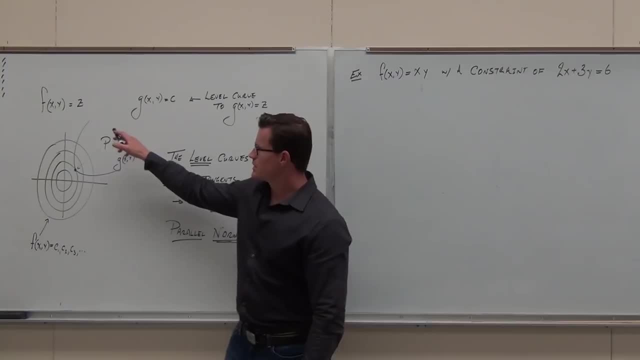 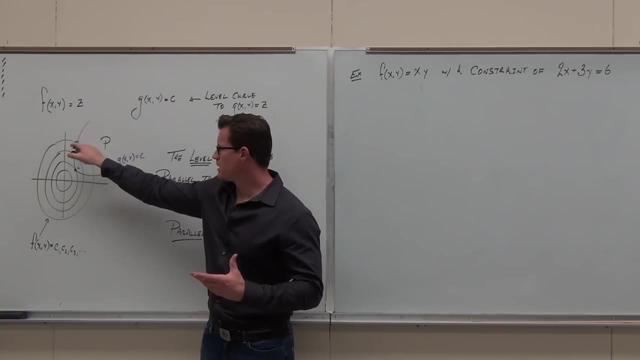 So we go: okay, fantastic, These level curves are going to intersect. If there's going to be a solution, they're going to intersect. So the level curve, this constraint, is going to intersect, a whole bunch of these level curves for that surface. 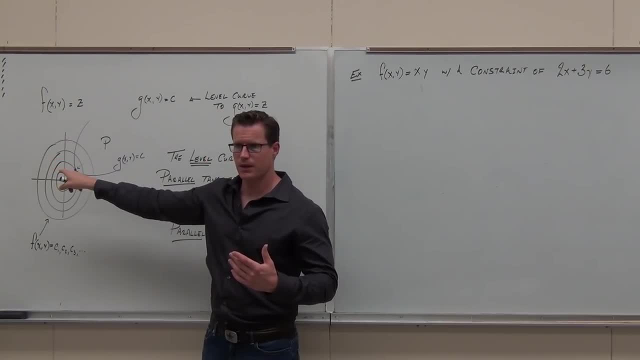 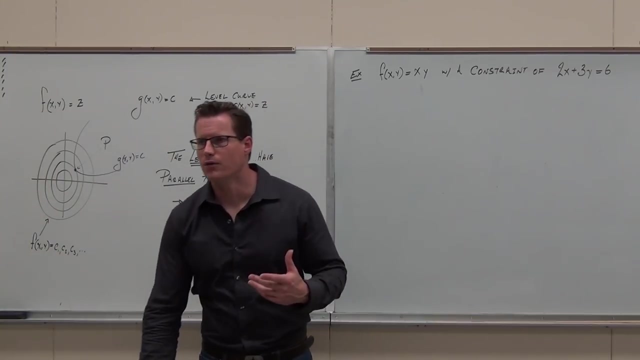 Do you guys get the idea? What we're looking at is for the point where this constraint level curve bounces off one or more of the level curves of the other function. Why we care about them bouncing off, why we care about them intersecting at one point, is this: 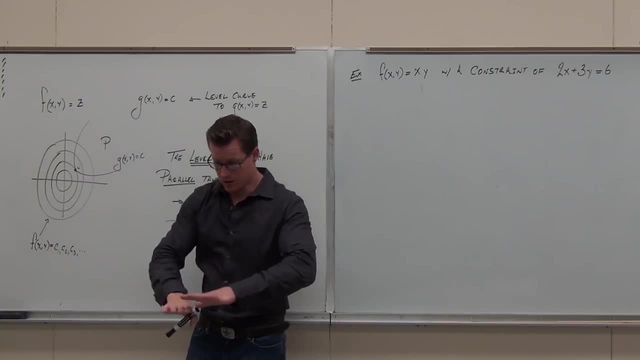 If I'm going to map the level curves of this surface onto a plane, which is exactly what I've done, that's a contour plot, And what that means is that from here- look carefully please- from here to here, and here and here. 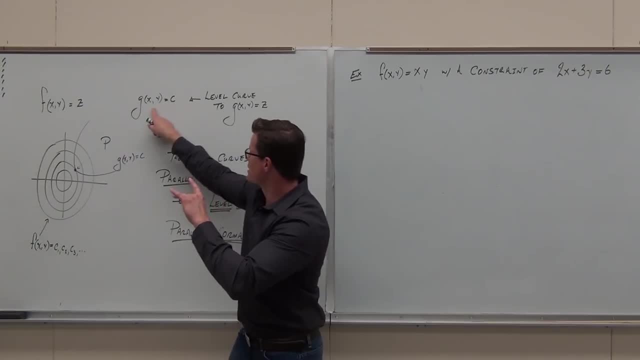 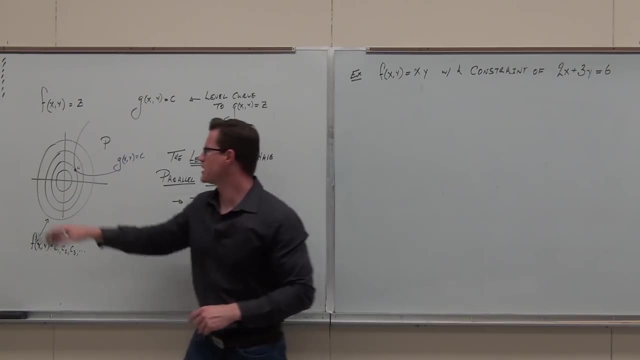 This surface has a whole bunch of level curves. This is one specific level curve, the constraint that we have to be on. Do you guys see the difference? There's a whole bunch of level curves for this, but there's only one that I care about for that surface. 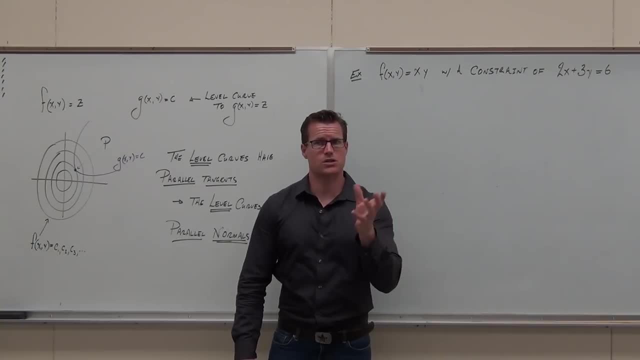 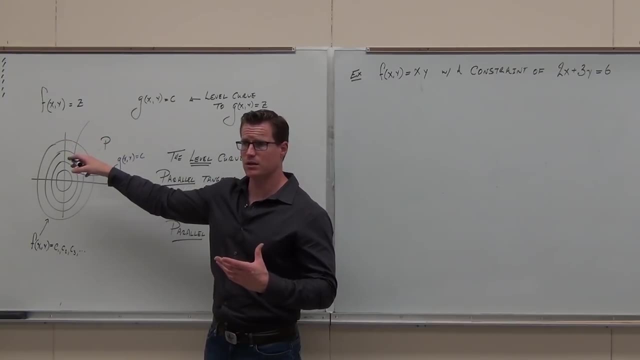 The one equal to the constant. that gives us that constraint. So we go: okay, fantastic, These level curves are going to intersect. If there's going to be a solution, they're going to intersect. So the level curve, this constraint, is going to intersect, a whole bunch of these level curves for that surface. 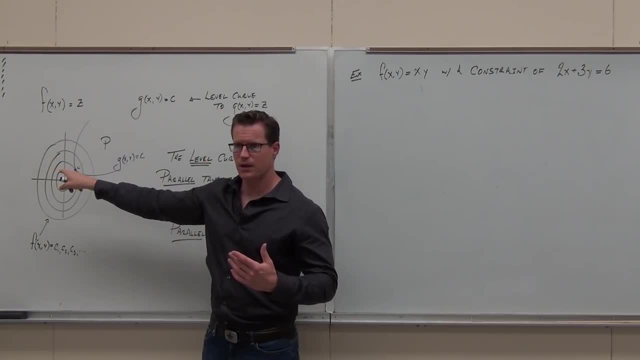 Do you guys get the idea? What we're looking at is for the point where this constraint level curve bounces off one or more of these level curves. Do you guys get the idea? What we're looking at is for the point where this constraint level curve bounces off one or more of these level curves. 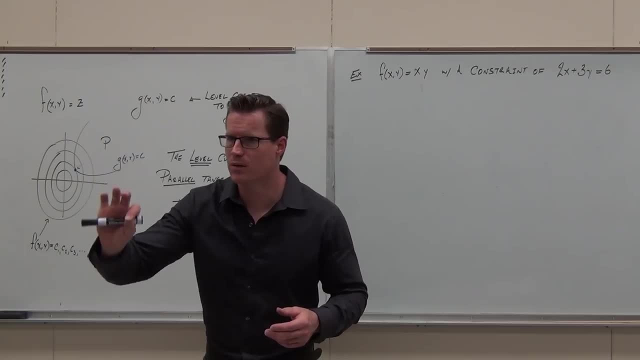 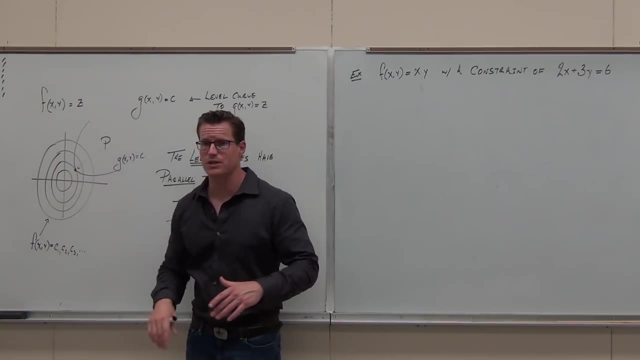 Why we care about them bouncing off, why we care about them intersecting at one point, is this: If I'm going to map the level curves of this surface onto a plane, which is exactly what I've done, that's a contour plot. 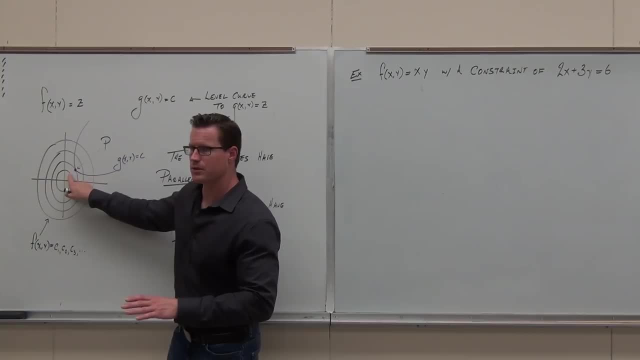 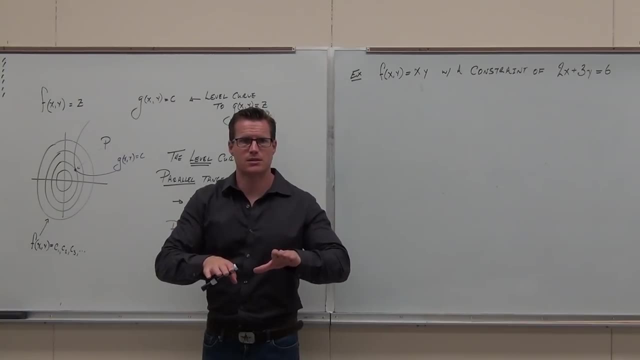 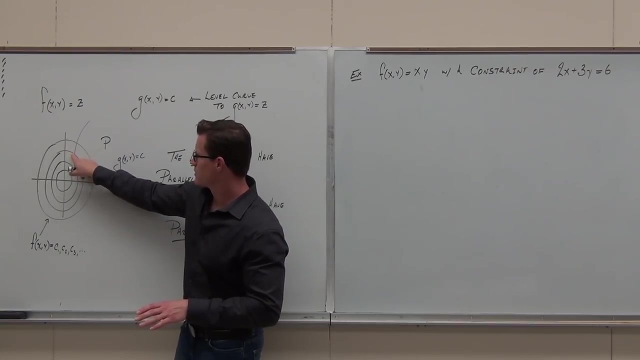 And what that means is that from here- look carefully please- from here to here, and here and here the function is either falling or the function is climbing. Does that make sense? So if I look at here or here, This function right here is either higher or lower than this. 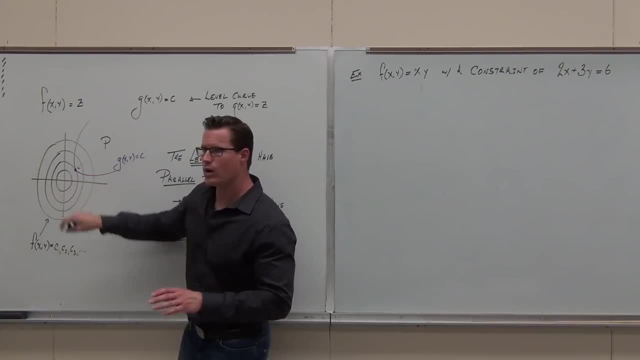 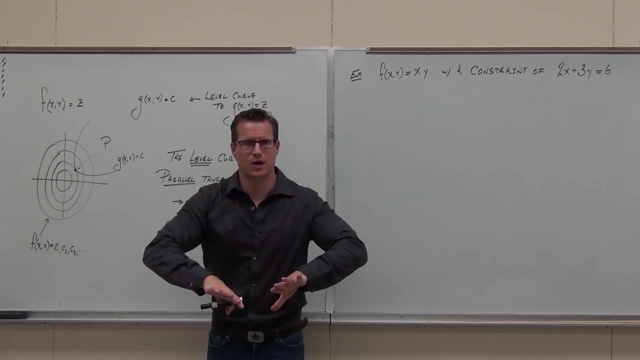 Here is either higher or lower than this. So that one point: if I think about the contour map, this is either going to be a high spot or a low spot. Consider the contour map. These things are either falling away or they're climbing, correct? 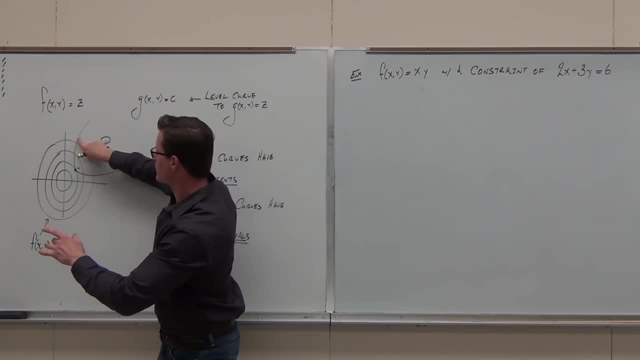 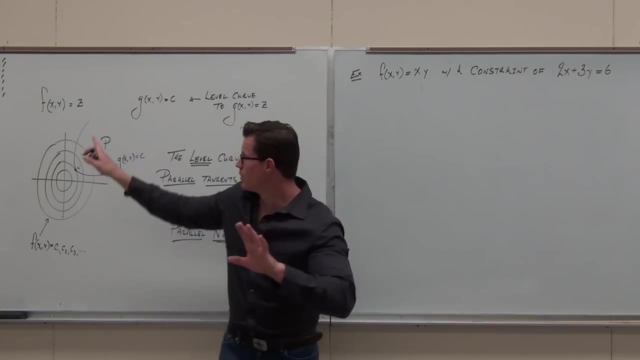 So where they intersect, these points are all higher or lower than that. What that means is that this point where we bounce off, Where one level curve- the one we care about the constraint- intersects a level curve of the other function, the function where we're trying to maximize or minimize 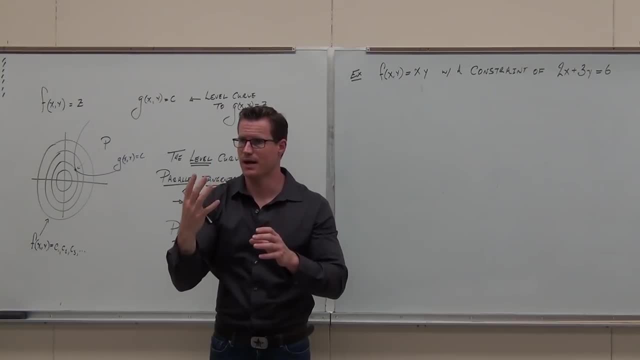 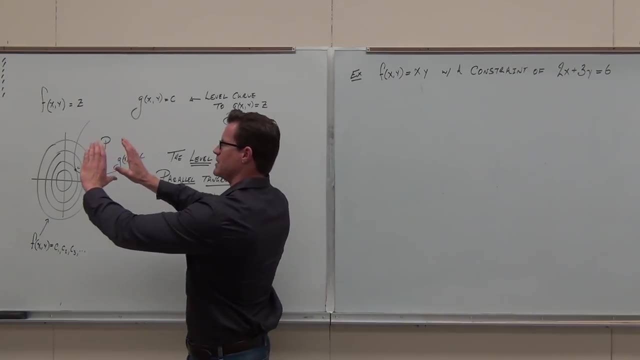 Where they bounce off. we either get a high point- a constrained maximum- or a low point- a constrained minimum. Did you guys get the idea of the contour plot That the contour plot is shaping the surface, showing the shape of the surface? 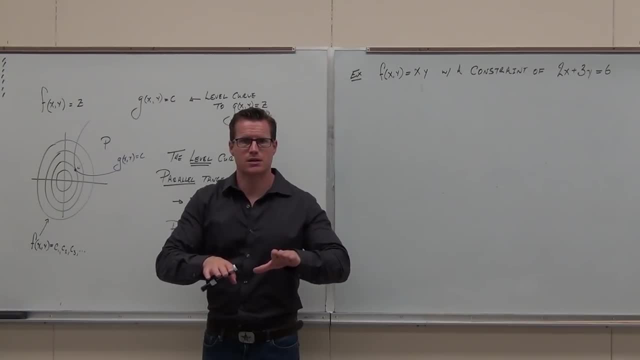 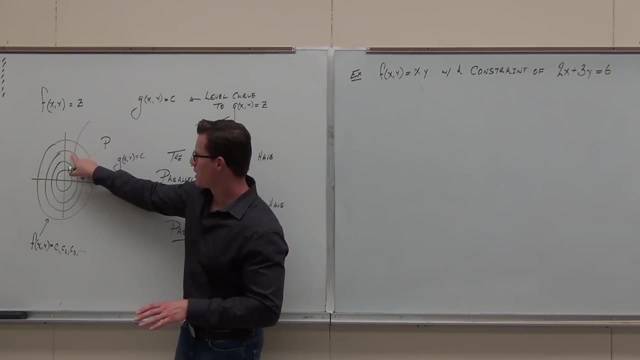 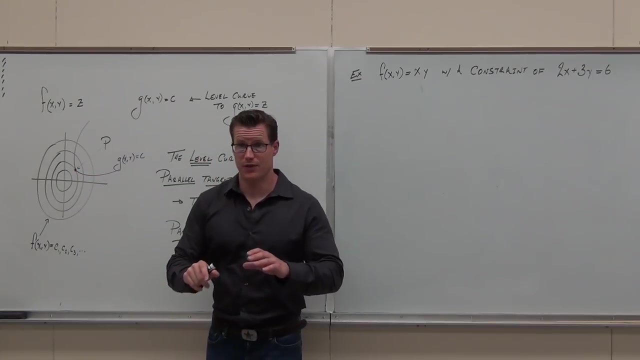 the function is either falling or the function is climbing. Does that make sense? So if I look at here or here or here, this function right here is either higher or lower than this. Here is either higher or lower than this. So that one point. if I think about the contour map, this is either going to be a high spot or a low spot. 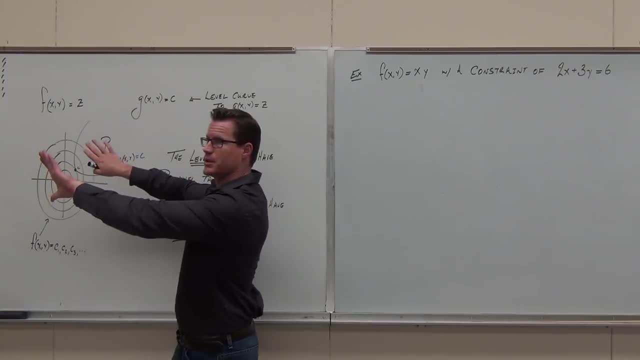 Consider the contour map. These things are either falling away or they're climbing correct. So where they intersect, these points are all higher or lower than that. What that means? What that means is that this point where we bounce off, where one level curve, the one we care about. 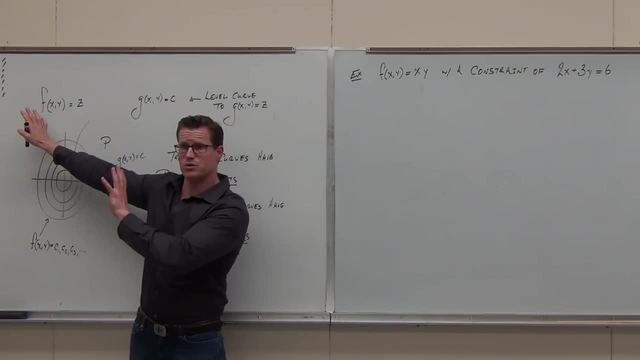 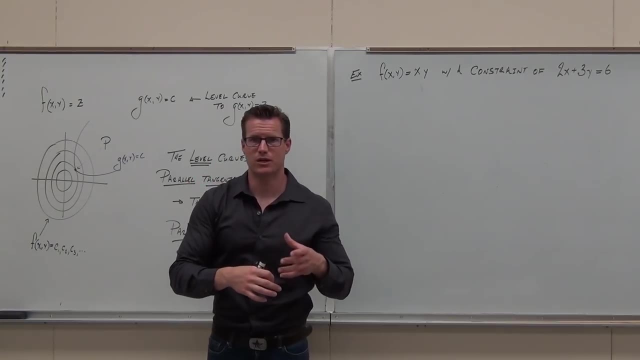 the constraint intersects a level curve of the other function, the function where we're trying to maximize or minimize, where they bounce off. we either get a high point- a constrained maximum- or a low point- a constrained minimum. Did you guys get the idea of the contour plot? 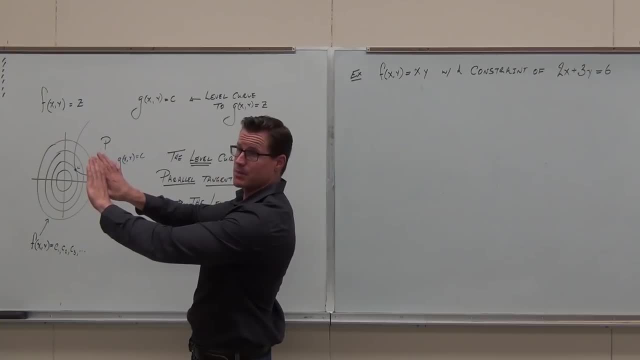 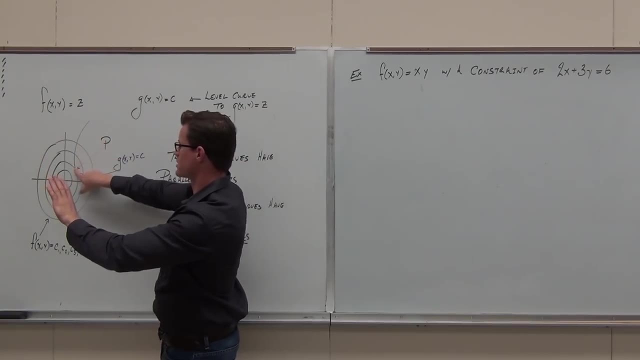 That the contour plot is shaping the surface, showing the shape of the surface. It's either falling away or it's climbing up. Do I know which one? Not really, I don't really care, because what I care about is that it's going to be one of them. 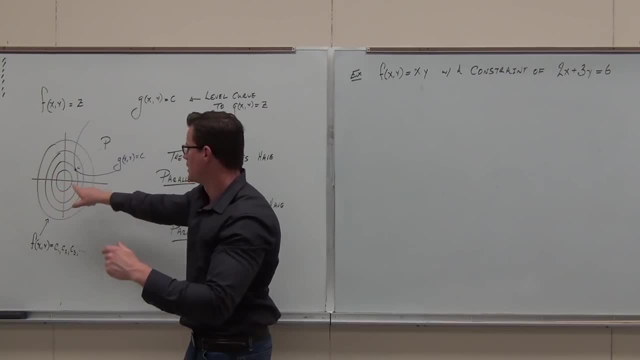 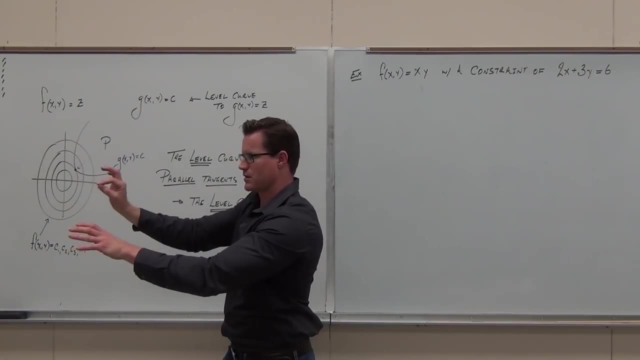 We have other things that we can do to figure out whether it's a maximum. The point is at that one spot where we touch, at one spot that creates a high point of a surface like this or a low point of a surface like that. 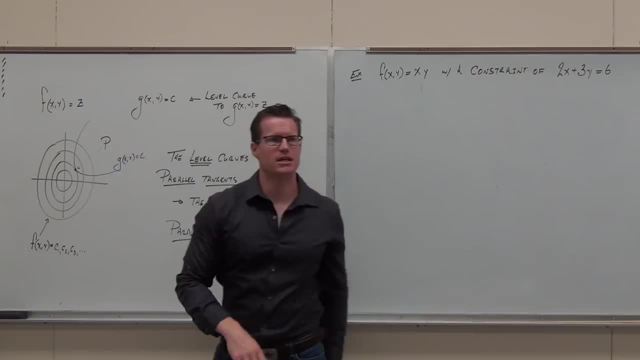 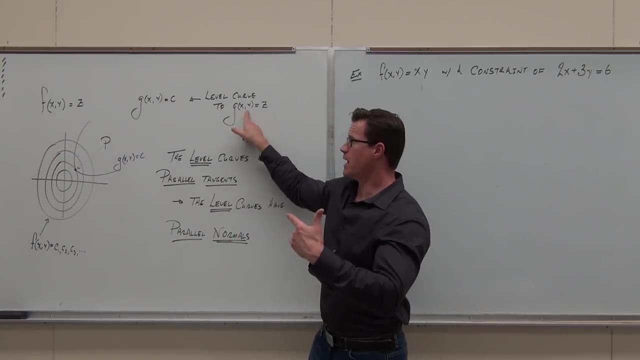 Does that make sense? That's the whole point. Now we start studying it. Surface, yeah, but we set it equal to constants and we get a lot of level curves. Surface, yeah, but we set it equal to a specific constant. a little constraint: that's one specific level curve where they bounce off. 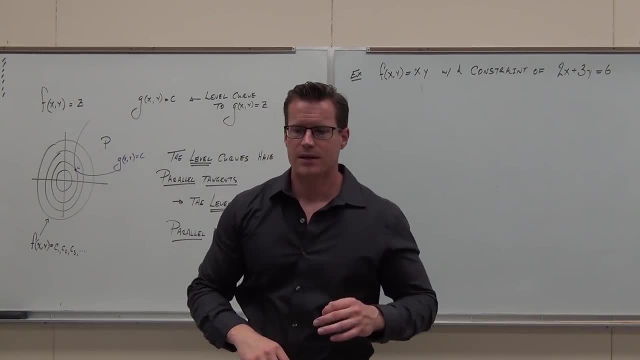 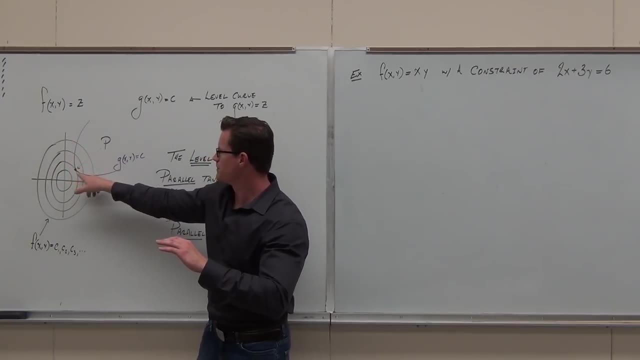 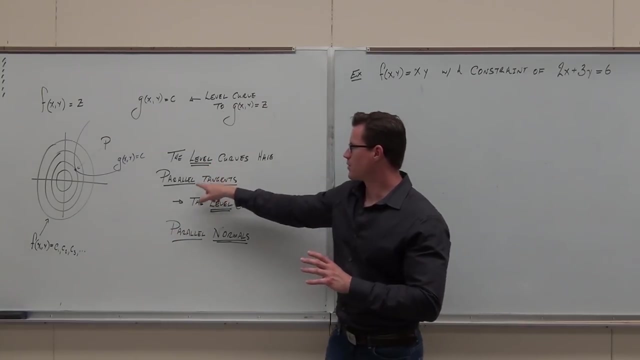 That's what we're looking for: Constraint maximum, Constraint minimum. Now we study the idea of that. If a function intersects another function at one point, they're said to have a common tangent, Or at least their tangents are parallel. So let's put this into perspective here. 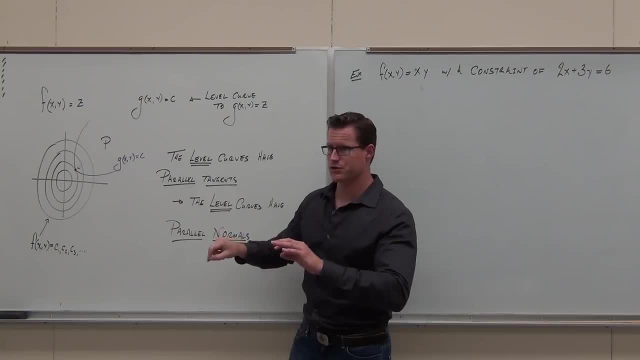 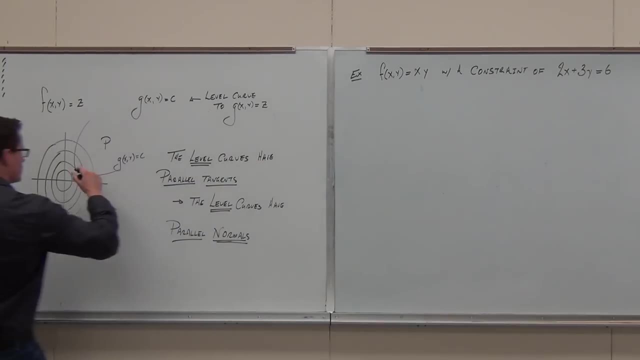 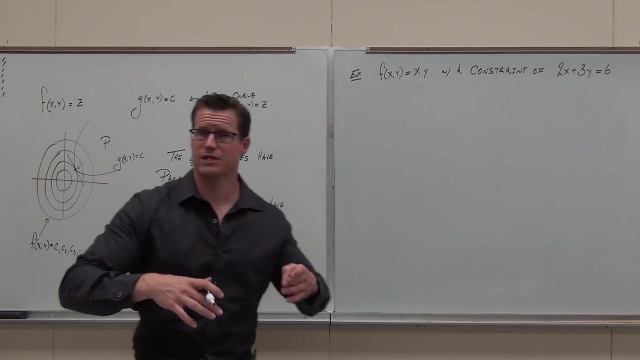 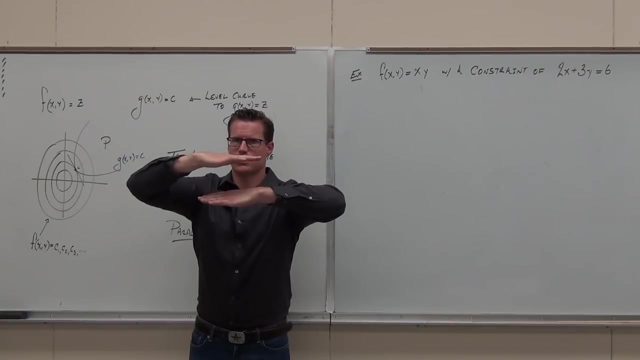 Please listen carefully. The level curves- level curve, level curve- have parallel tangents. Do you follow that? Okay, You say common tangent or parallel tangents. However, if the level curves have parallel tangents, think about this: If you have parallel tangents that are like this, parallel tangents, are your normals also parallel? 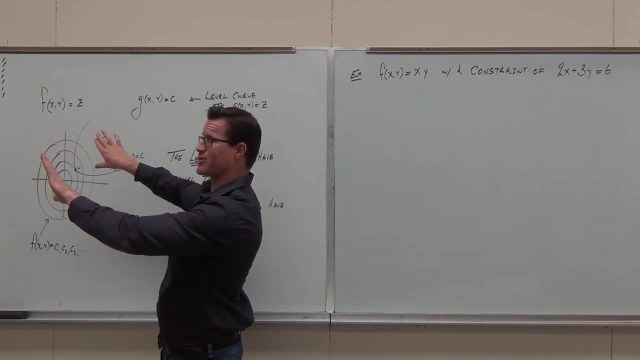 It's either falling away or it's climbing up. Do I know which one? Not really, I don't really care, Because what I care about is that it's going to be one of them. We have other things that we can do to figure out whether it's a maximum or minimum. 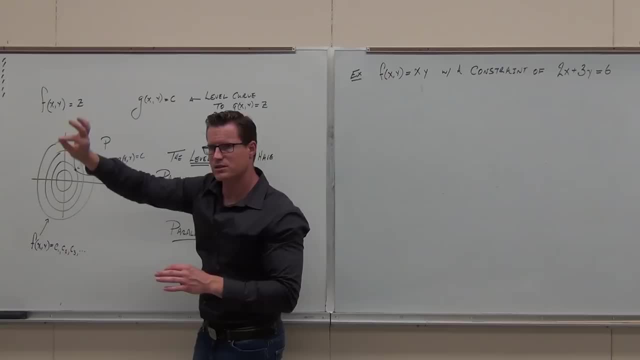 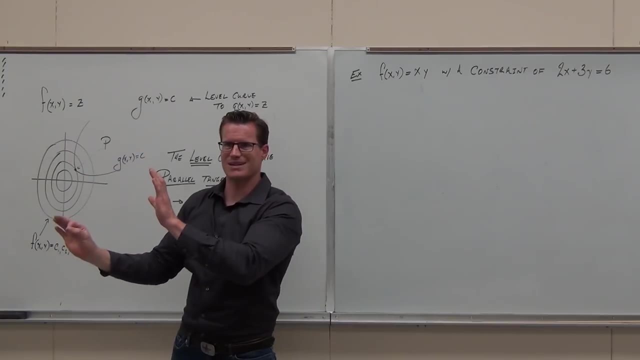 The point is at that one spot, where we touch at one spot that creates a high point of a surface like this or a low point of a surface like that. Does that make sense? That's the whole point. Now we start studying it. 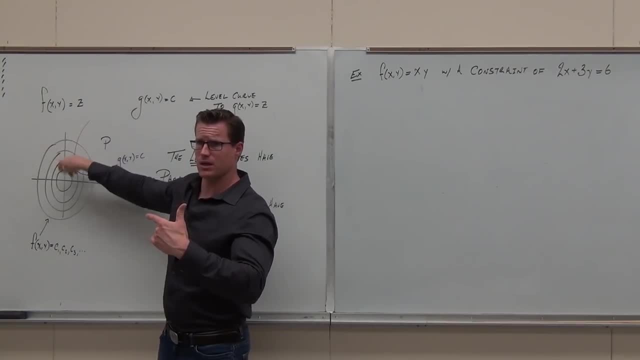 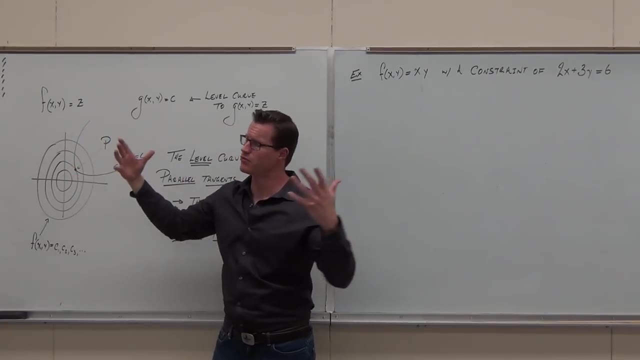 Surface: yeah, But we set it equal to constants and we get a lot of level curves. Surface, yeah, But we set it equal to a specific constant and a constraint, that's, one specific level curve where they bounce off. That's what we're looking for. 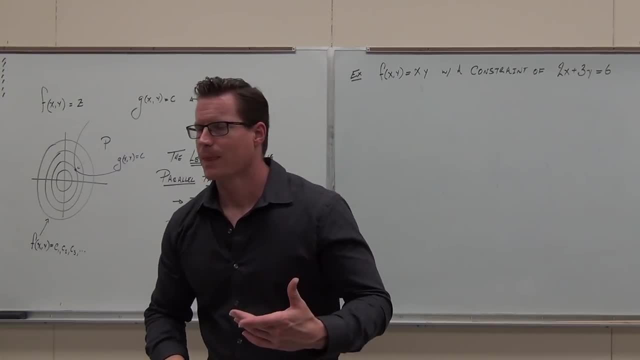 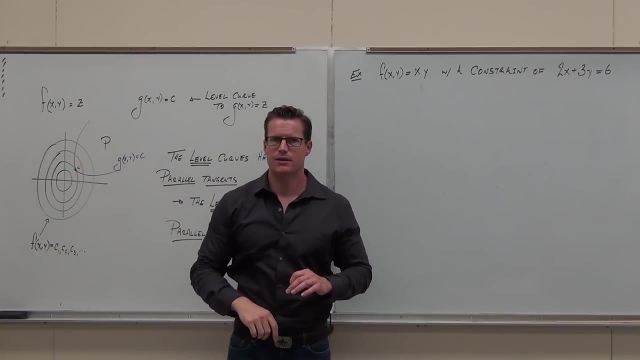 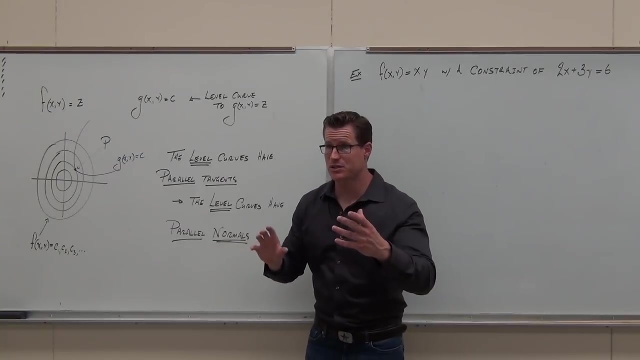 Constraint max or constraint min. We studied the idea of that. If a function intersects another function at one point, they're said to have a common tangent, Or at least their tangents are parallel. So let's put this into perspective here. Please listen carefully. 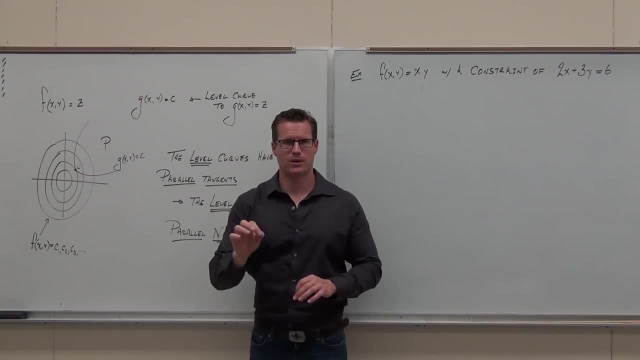 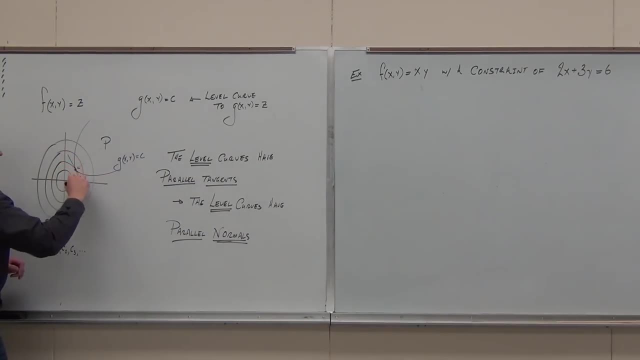 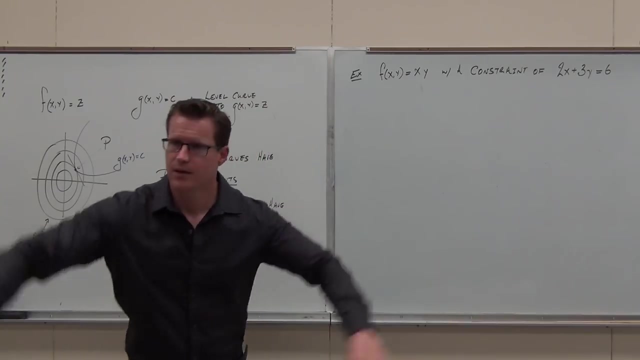 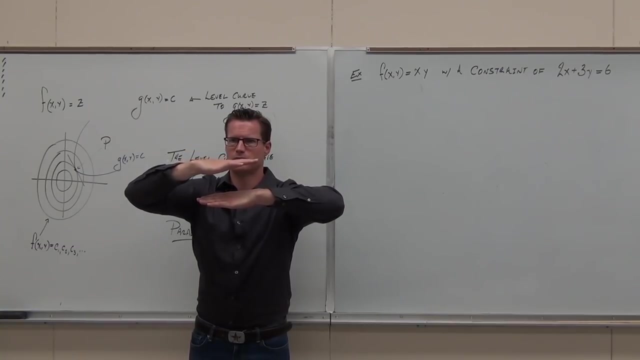 The level curves- level curve, level curve- have parallel tangents. Do you follow that? Okay, Let's say common tangent or parallel tangents. However, if the level curves have parallel tangents, think about this: If you have parallel tangents that are like this, parallel tangents, are your normals also parallel? 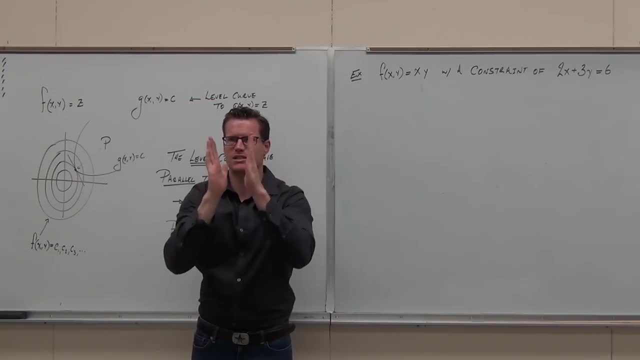 Yes, Yeah, I feel like a mind. I'm in a box of emotion. So if your tangents are parallel, the level curves also have normals that are parallel. Level curves have parallel tangents. Check Level curves have parallel normals. 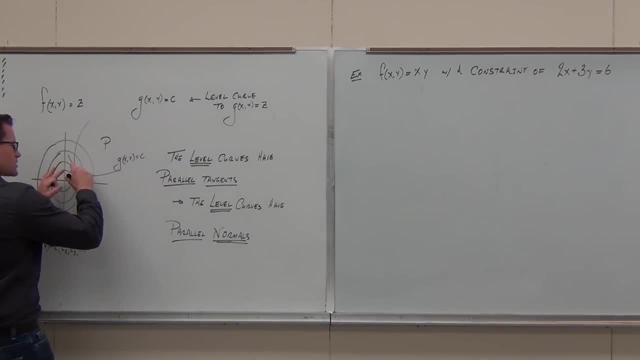 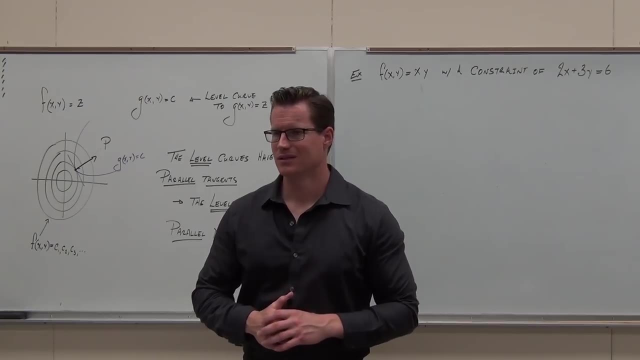 Check. That's what we're talking about. The normals to these curves at that point is common, Or at least they're parallel. Hey, now that you're with me. Now, normals are vectors. Tell me something you know about vectors if they're parallel. 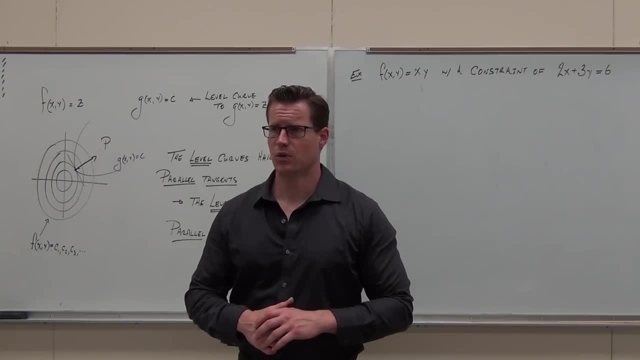 Tell me something about that. Scalar multiples, Scalar multiples: So if our normals listen as we're putting together, okay, so the equation I gave you last time actually makes sense to you now. If the normals are parallel, the normals of these level curves must be scalar multiples. 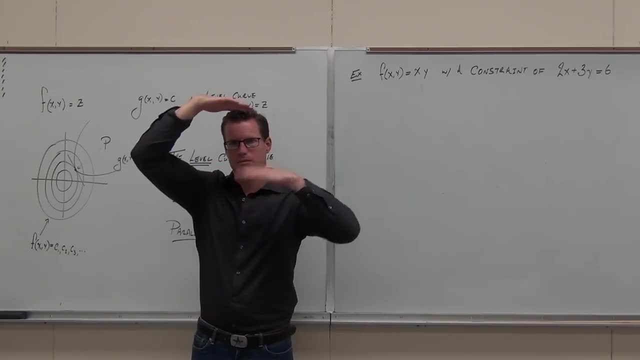 Yes, Yeah, I feel like a mind. I'm in a box of emotion. So if your tangents are parallel, the level curves also have normals that are parallel. Level curves have parallel tangents. check. Level curves have parallel normals. check. 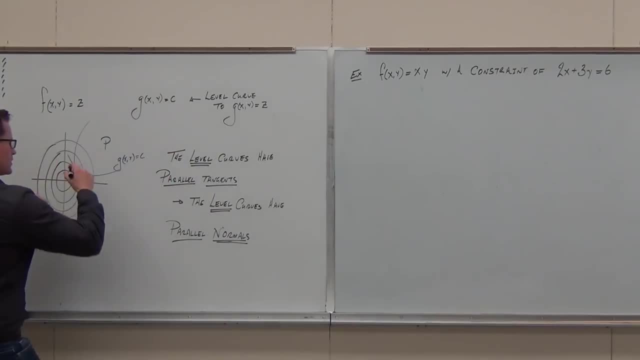 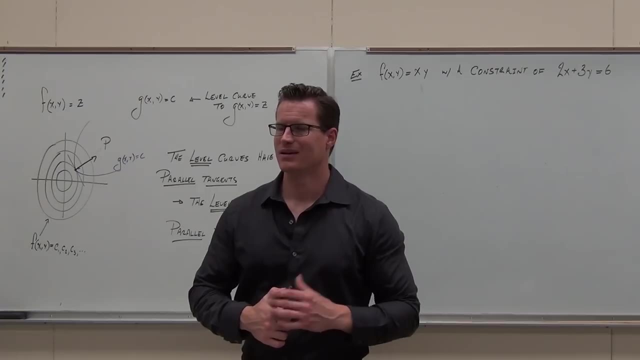 That's what we're talking about. The normals to these curves at that point is common, or at least they're parallel. Hey, now that you're with me. Now, normals are vectors. Tell me something you know about vectors if they're parallel. 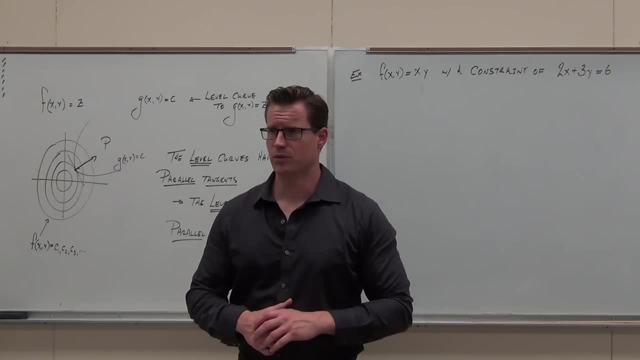 Tell me something about that. Scalar multiples, Scalar multiples: So if our normals listen as we're putting together, okay, so the equation I gave you last time actually makes sense to you now. If the normals are parallel, the normals of these level curves must be scalar multiples. 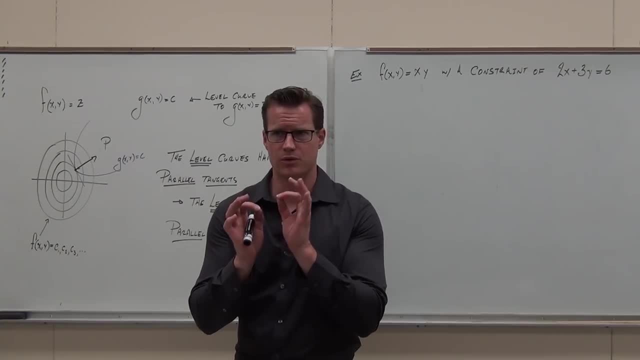 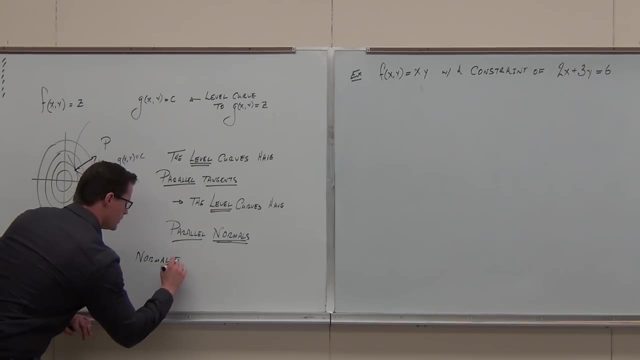 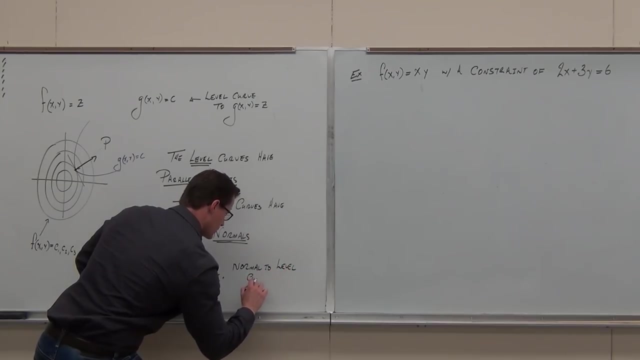 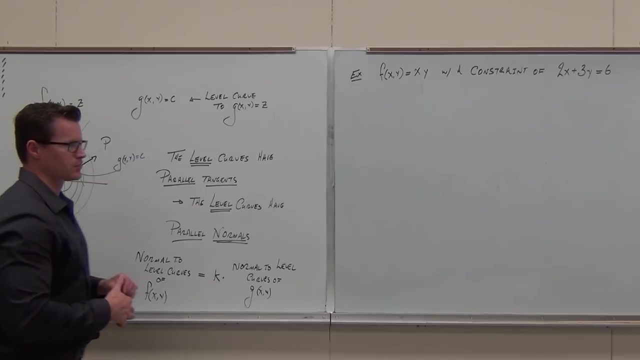 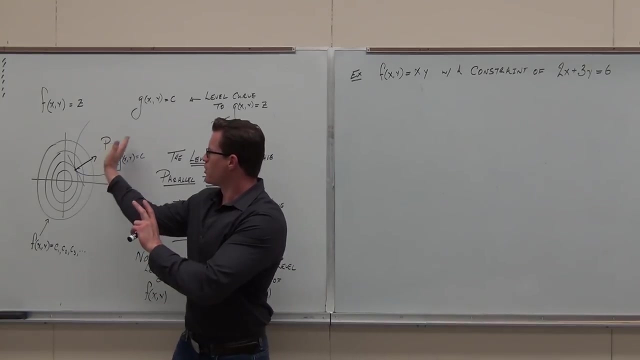 Do you guys get that idea? So the normals must be scalar, multiples: Level curves of F- yep. Level curve of G- yep. What I know is that the normals to those levels, to those level curves at that point, at that one point. 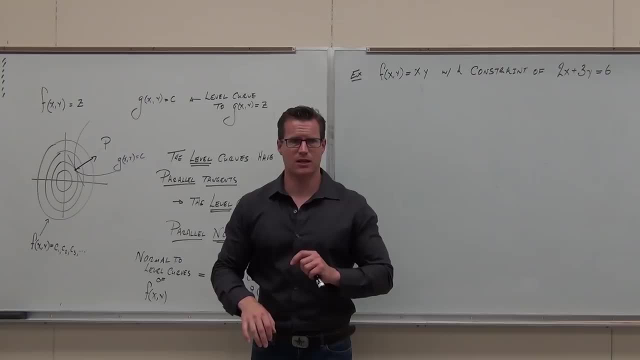 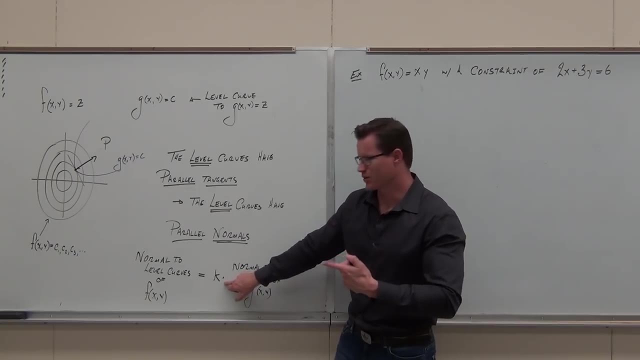 the normals to those level curves have to be scalar multiples. So the normals to level curves of F of X, Y is K times. let's call that a constant, just some scalar, a scalar multiple to the normals of the level curves of G of X, Y. 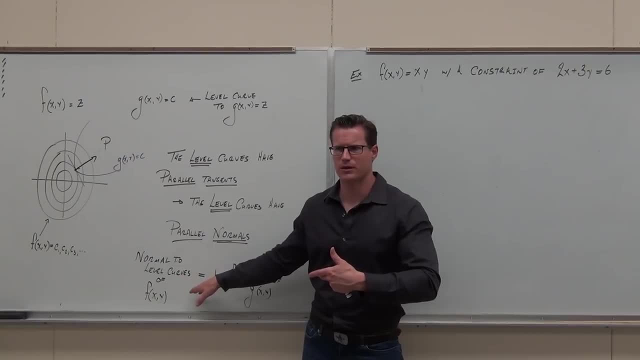 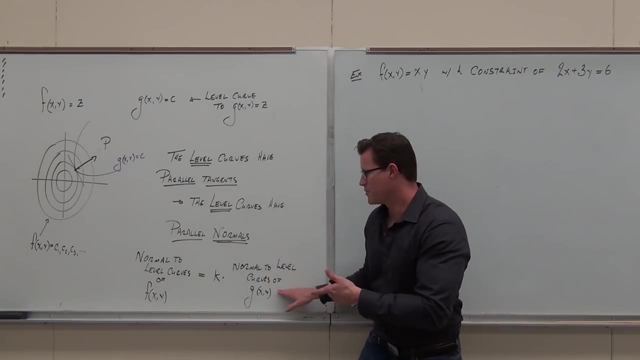 Do you guys see that what we just spoke about is written down in this kind of verbal model here? If we said this: the level curves have parallel normals. The level curves have parallel normals. Oh, they're scalar multiples of each other. Should our parents feel okay with the idea for real? 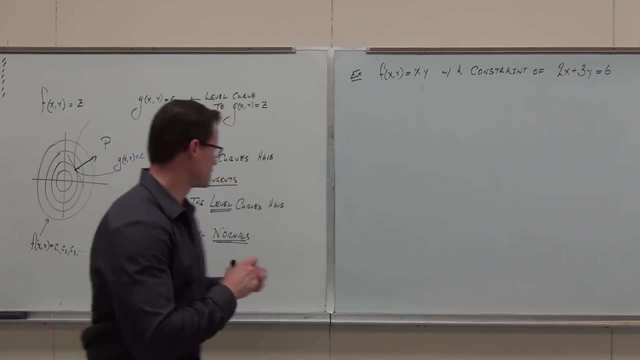 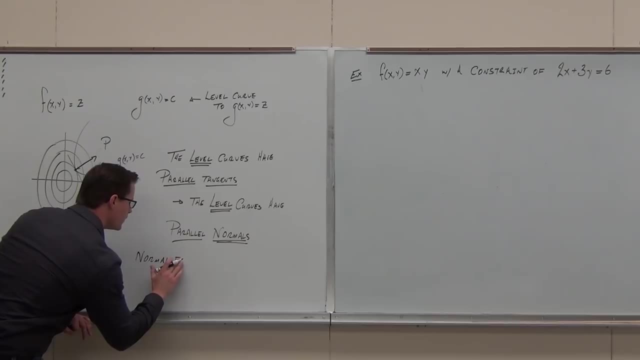 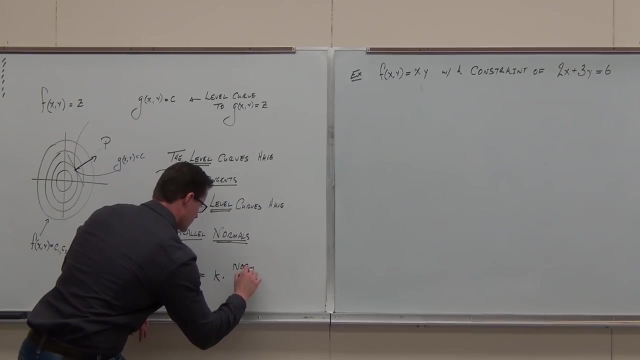 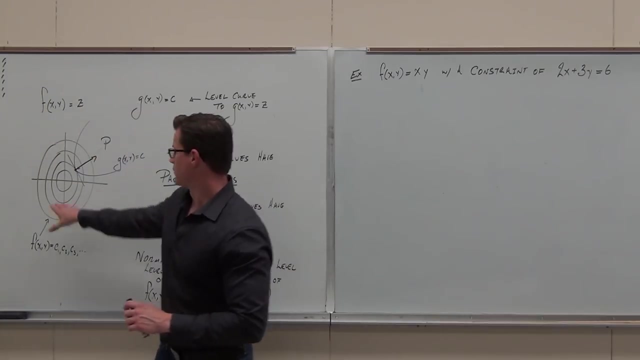 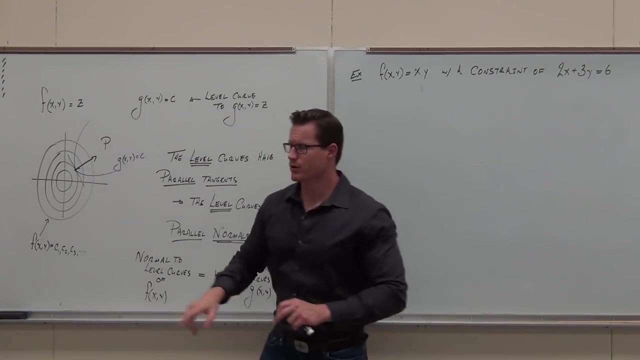 Do you guys get that idea? So the normals must be scalar multiples: Level curves of F- Yep. Level curve of G- Yep. What I know is that the normals to those level curves at that point are parallel. The normals to those level curves at that point, at that one point, the normals to those. 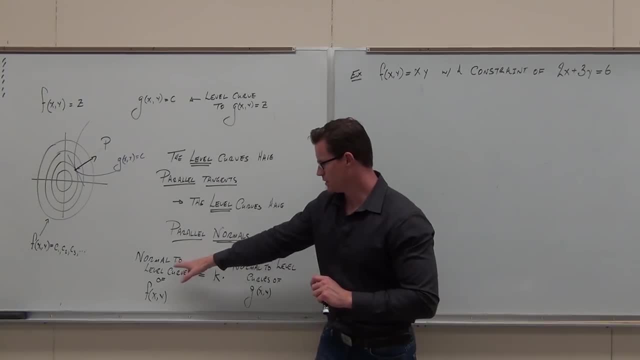 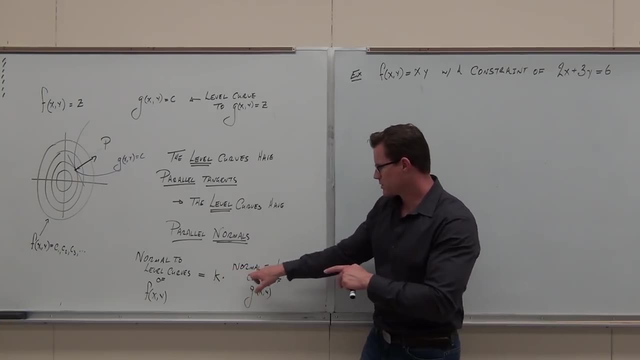 level curves have to be scalar multiples. So the normals to level curves of F of X, Y is K times. let's call that a constant, just some scalar, a scalar multiple to the normals of the level curves of G of X, Y. 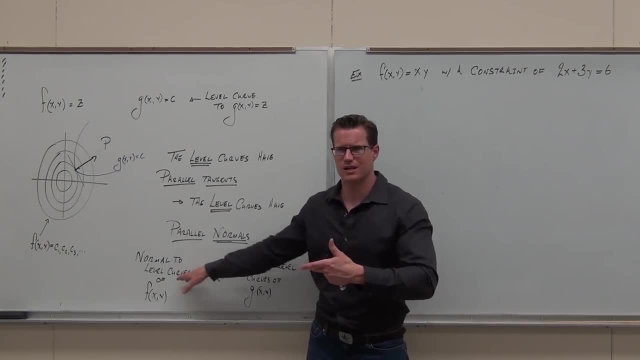 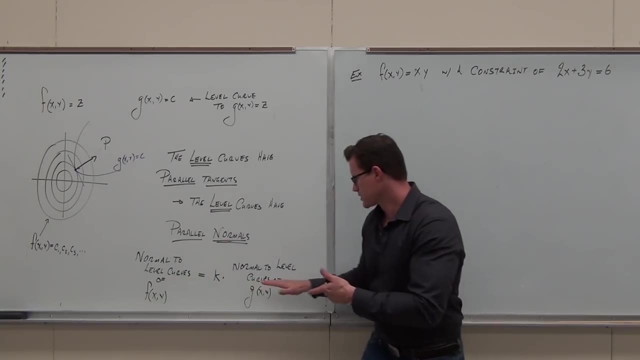 Do you guys see that what we just spoke about is written down in this kind of verbal model here? If we said this: the level curves have parallel normals. The level curves have parallel normals. Oh, they're scalar multiples of each other. Show of hands if you feel okay with the idea for real. 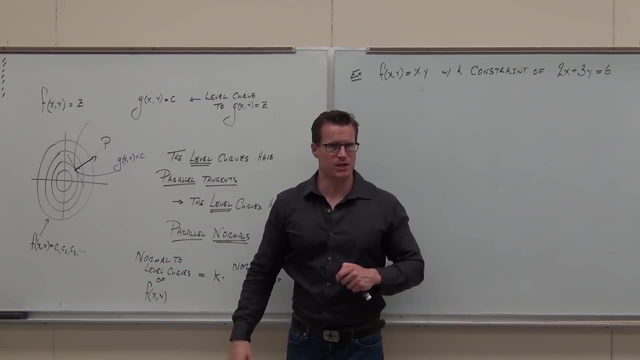 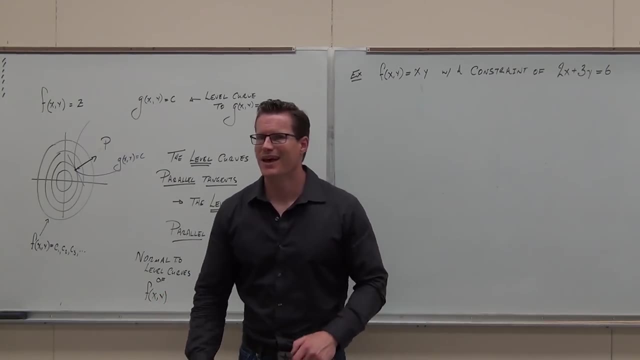 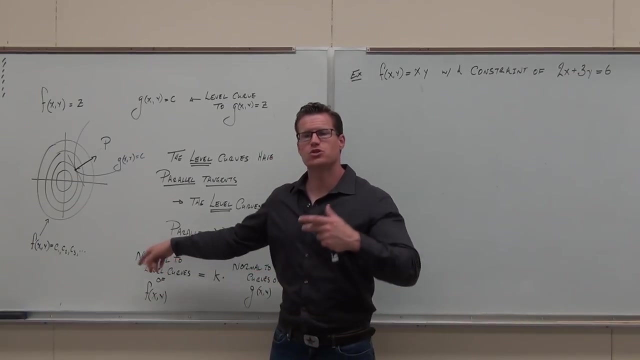 This is the idea of constraint optimization. This is the idea of something called the Lagrange multiplier. What we do is we think back a little bit. Hey, everybody, what gives us look? what gives us normals to level curves? What gives us normals to level curves? 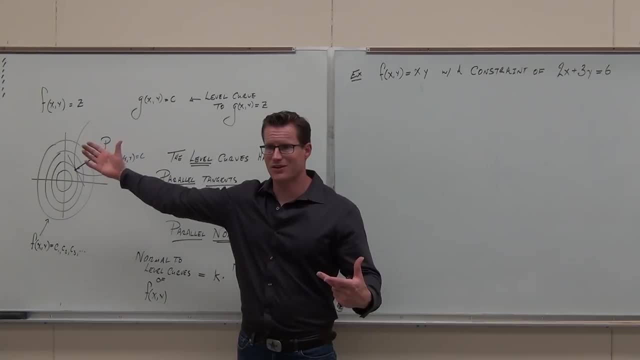 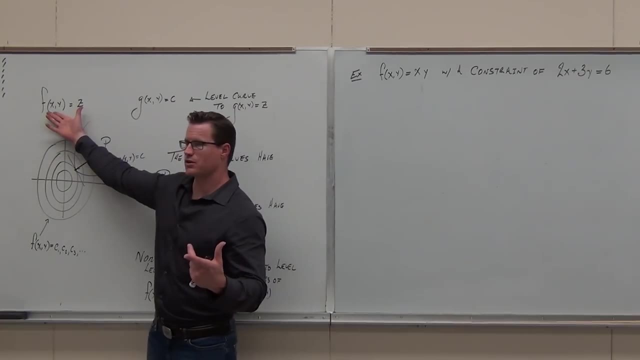 To level curves of a surface. What gives us that we've been doing for the gradient? Did you follow this? Here's a function, right, It's a surface. If I find the gradient, the gradient gives me normals to the level curves. 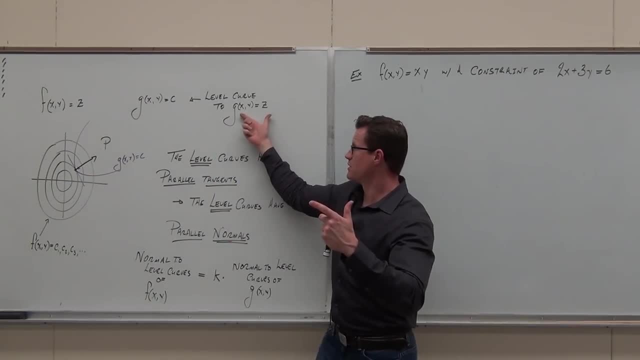 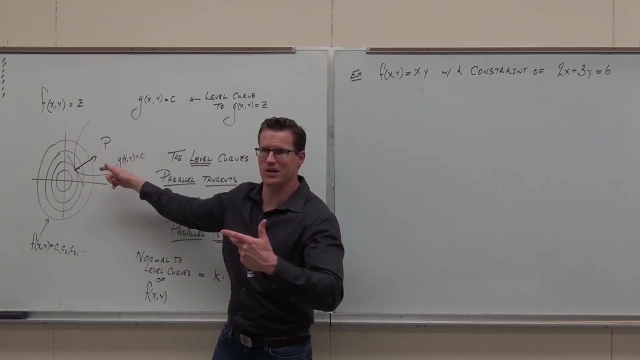 Do you get me? Here's a function. It's a surface but it's a level curve. The gradient would give me the normal to this specific level curve, the one I really care about. I want to know that those normals have to be scalar multiples. 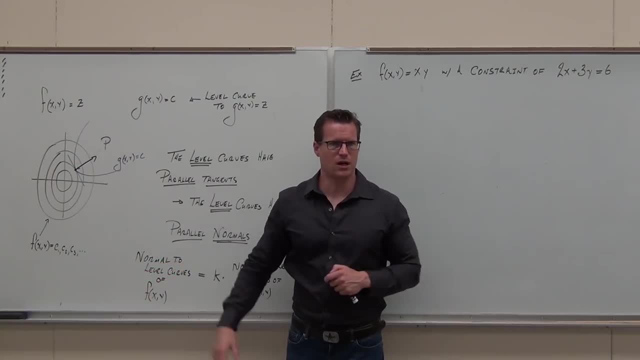 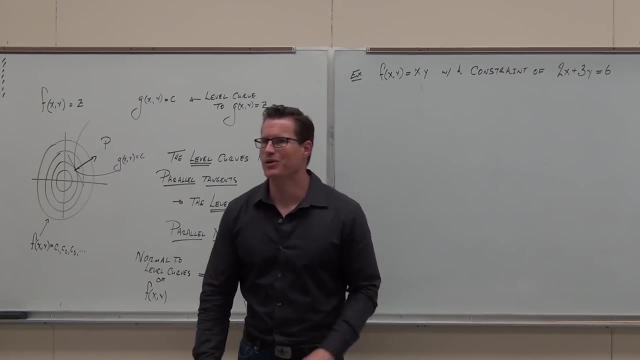 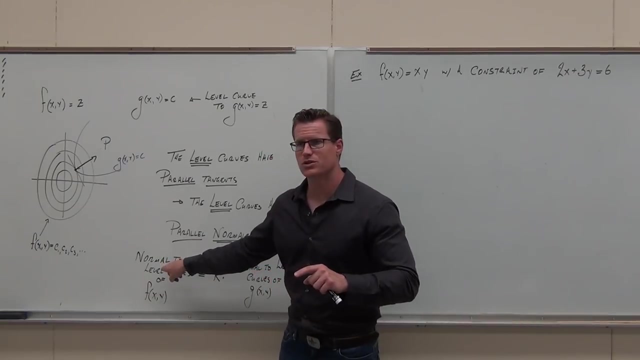 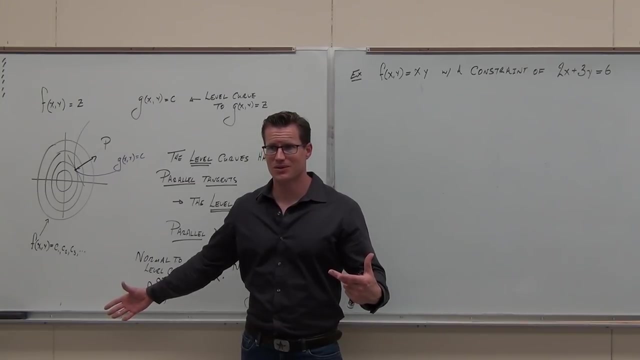 This is the idea of constraint optimization. This is the idea of something called the Lagrange multiplier. What we do is we think back a little bit. Hey, everybody, what gives us look? what gives us normals to level curves? What gives us normals to level curves? 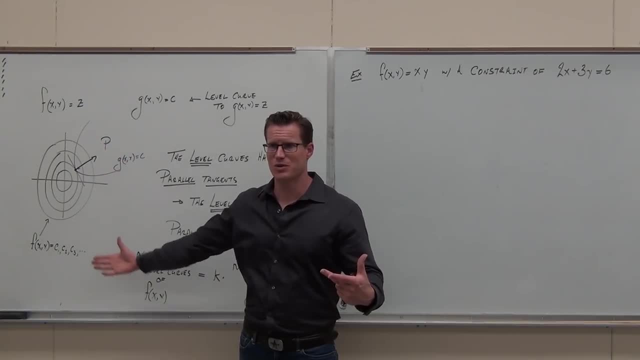 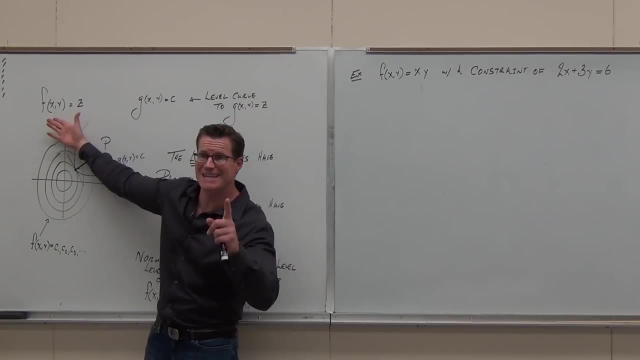 The level curves of a surface. What gives us that we've been doing for the gradient? Did you follow this? Here's a function, right, It's a surface. If I find the gradient, the gradient gives me normals to the level curves. 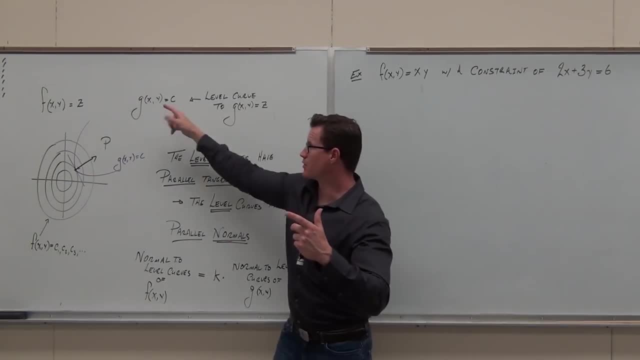 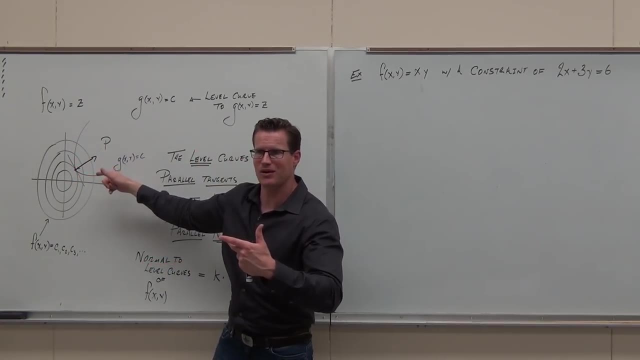 You get me. Here's a function. It's a surface but it's a level curve. The gradient would give me the normal to this specific level curve, the one I really care about. I know that those normals have to be scalar multiples. 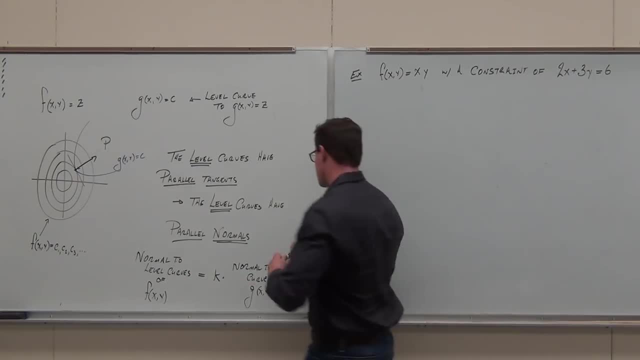 The gradient gives me normals to level curves. The gradient gives me normals to level curves, So we go. okay, so the gradient of F must be a scalar multiple of the gradient of G. Did you catch on to that? I said the same thing twice. 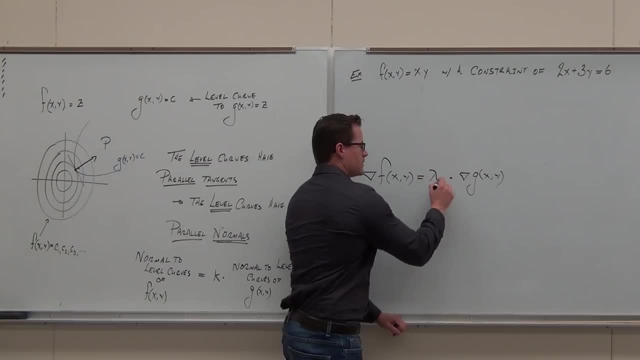 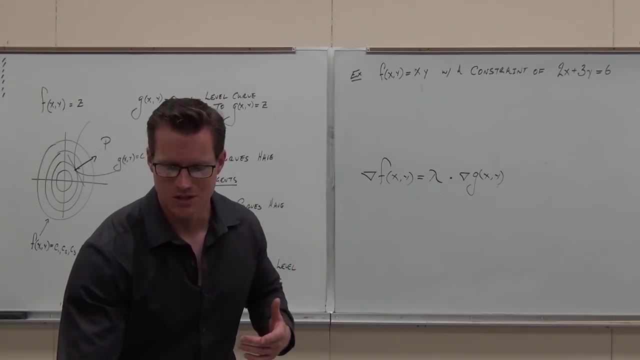 Here's the deal. We just don't call it K, We call it lambda, It's called the Lagrange multiplier and it's a scalar. This is all I'm trying to say. It's how constraint optimization works. Here's what it says. 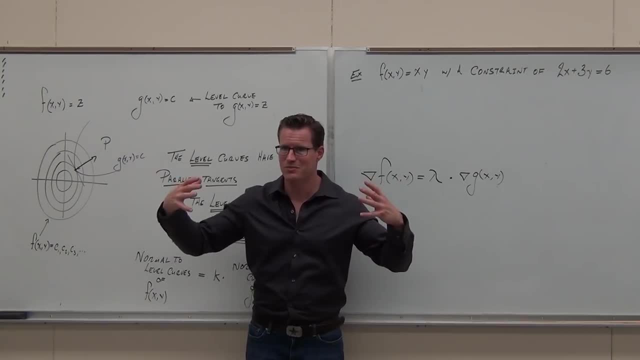 Here's what it says. One last time. okay, Check it out. So you should bear with me because examples are coming. We only have 30 minutes. We're going to get them done in about 25 minutes, But that's it. 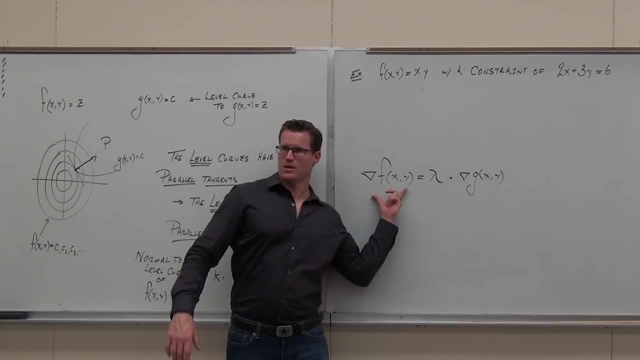 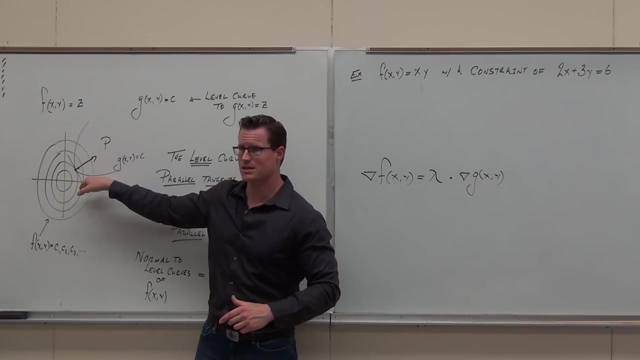 So here we go. This gives us normals to level curves. correct The normals to these things I'm looking at. This gives us normals to level curves. The normals to this one that I'm looking at Make sense If they touch at one point. if they touch at one point, they will. 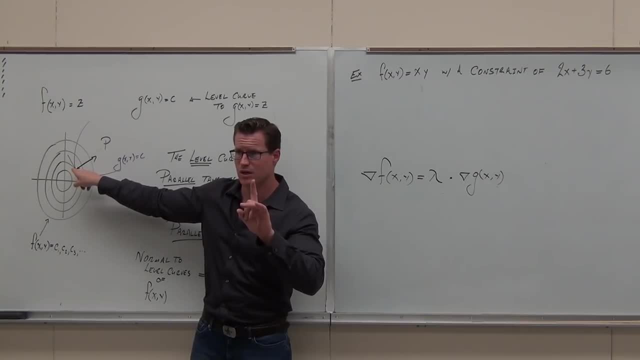 If they touch at one point, their normals have to be scalar multiples. So by making our normals scalar multiples we find the point. So we're going to find the one point or more points where we have normals that are scalar multiples. 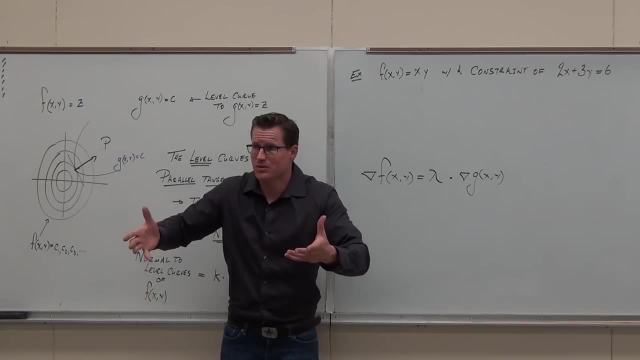 You guys get it At that point. our normals are going to be scalar multiples. So make our normals scalar multiples and we can find the point. We're kind of working backwards here. Does that make sense? Kind of cool right. 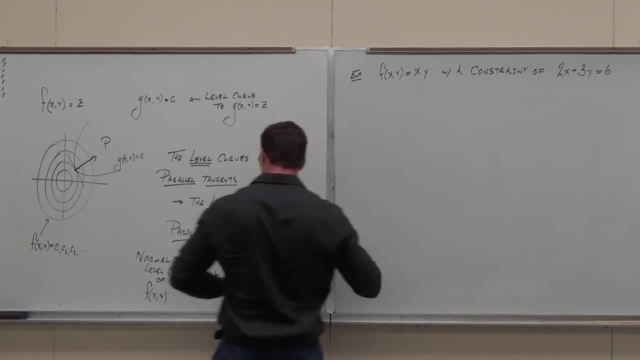 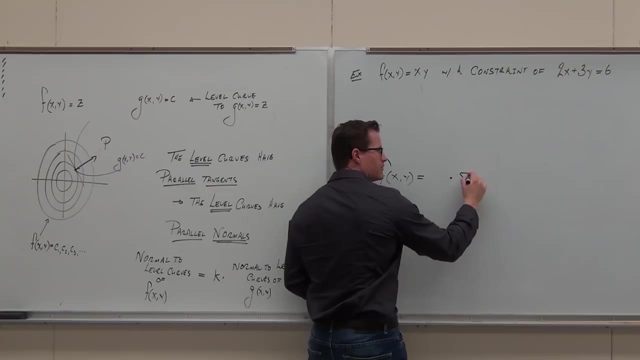 The gradient gives me normals to level curves. The gradient gives me normals to level curves, So we go. okay, so the gradient of F must be a scalar multiple of the gradient of G. Did you catch on to that? I said the same thing twice. 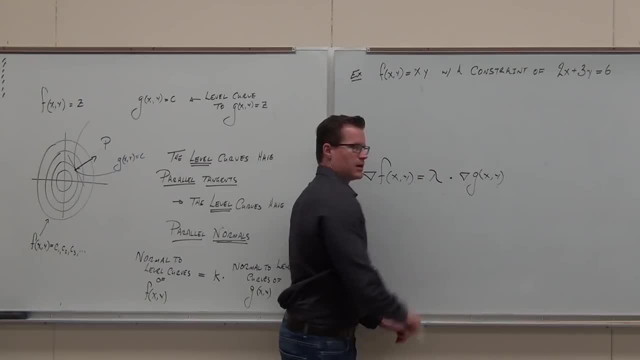 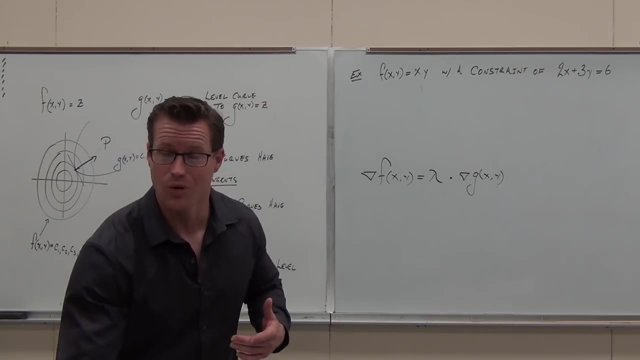 Here's the deal. We just don't call it K, We call it lambda, It's called the Lagrange multiplier and it's a scalar. This is all I'm trying to say. This is how constrained optimization works. Here's what it says. 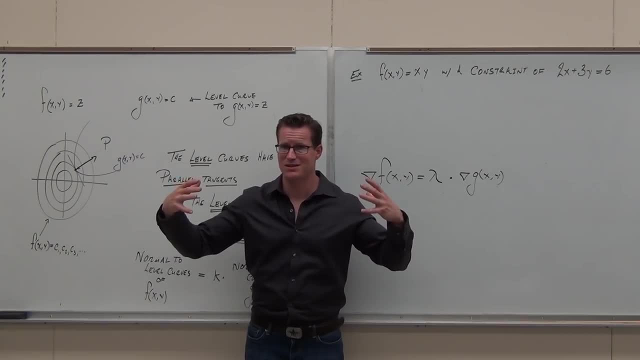 Here's what it says. One last time. okay, Check it out. So you should bear with me because examples are coming. We only have 30 minutes. We're going to be done in about 25 minutes, but that's it. 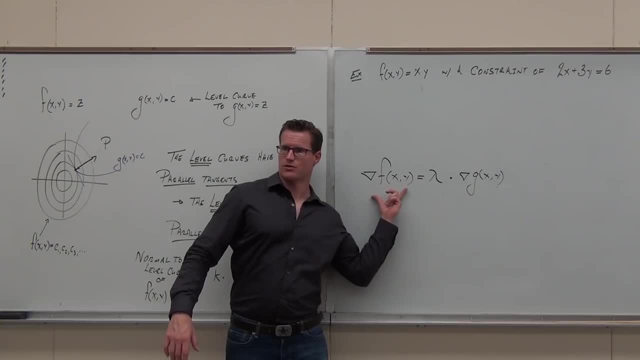 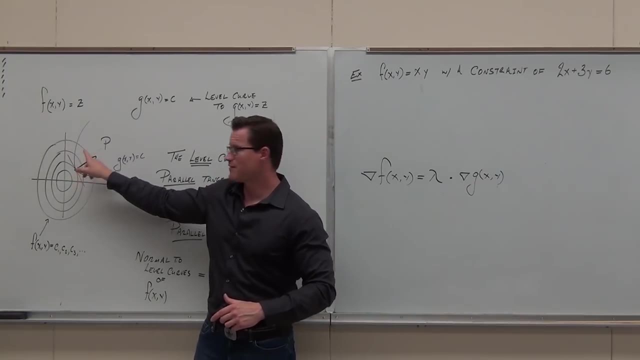 So here we go. This gives us normals to level curves. correct The normals to these things I'm looking at. This gives us normals to level curves. the normal to this one that I'm looking at Make sense If they touch at one point. if they touch at one point, they will. 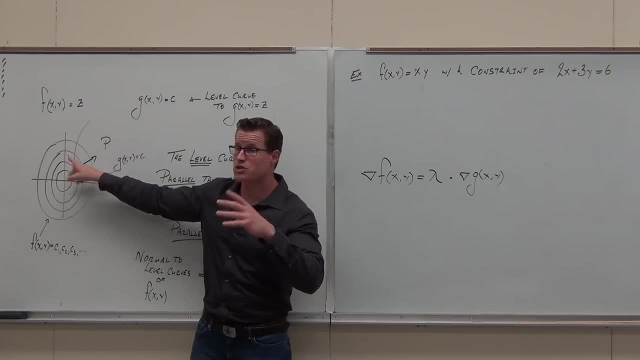 If they touch at one point, their normals have to be scalar multiples. So by making our normals scalar multiples we find the point. So we're going to find the one point or more points where we have normals that are scalar multiples. You guys get it. 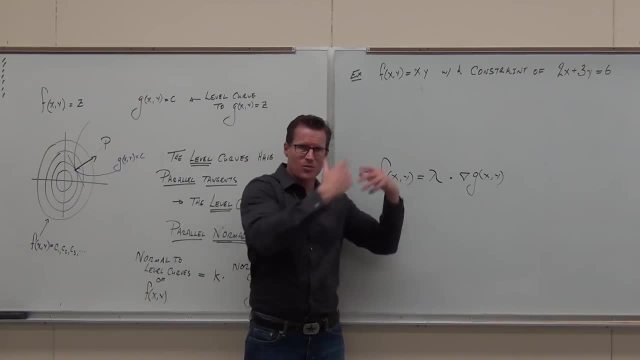 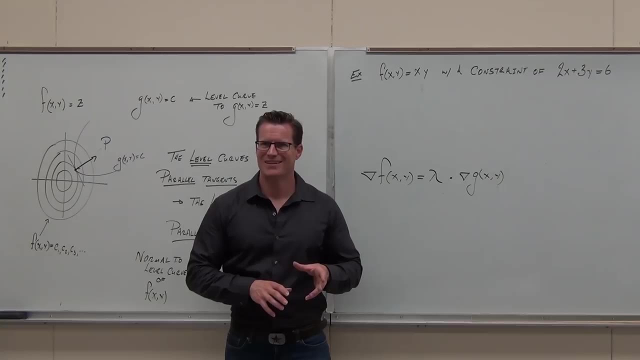 At that point our normals can be scalar multiples. So make our normals scalar multiples and we can find the point. We're kind of working backwards here. Does that make sense? Kind of cool, right. You know the gradient means normals to level curves, so we use that. 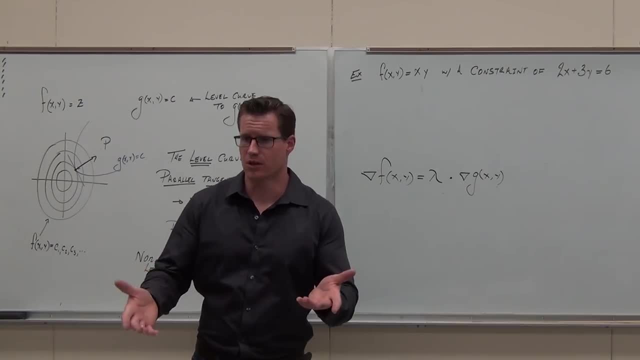 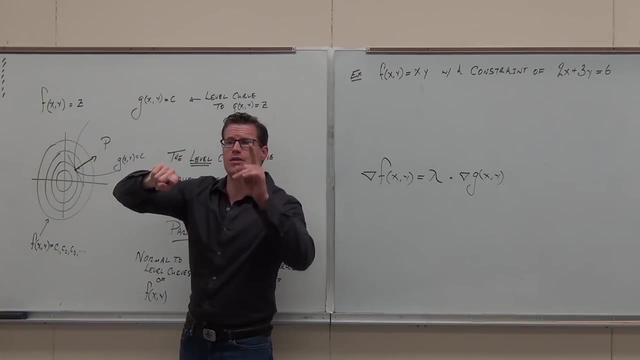 We say we want to find the point where the normals point, Where they are scalar, multiples, Where they are parallel, Where they have basically the same normal. That's where our one level curve constraint intersects another level curve over surface, the function. Let's try an example with this. 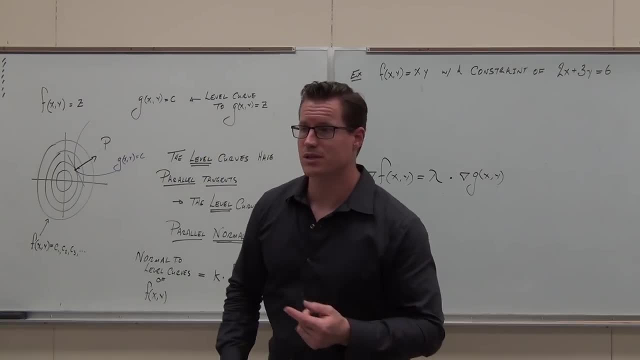 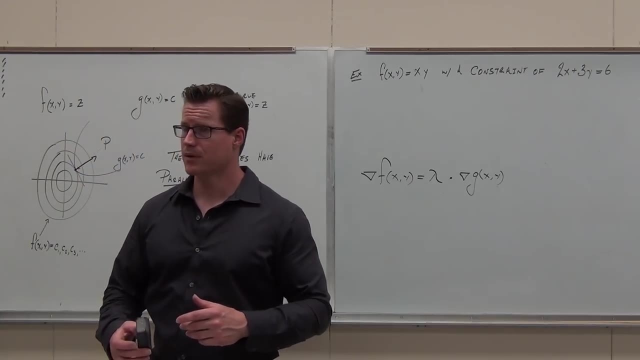 I'll show you how it's done. I've got to tell you right now we're not going to be focusing on word problems because they take a long time. I'm focused on setup and the operations behind them. Word problems do happen. 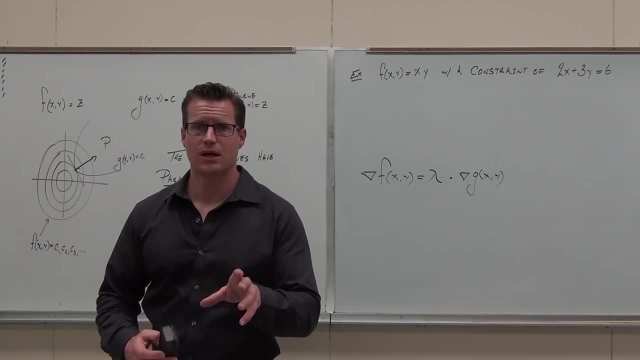 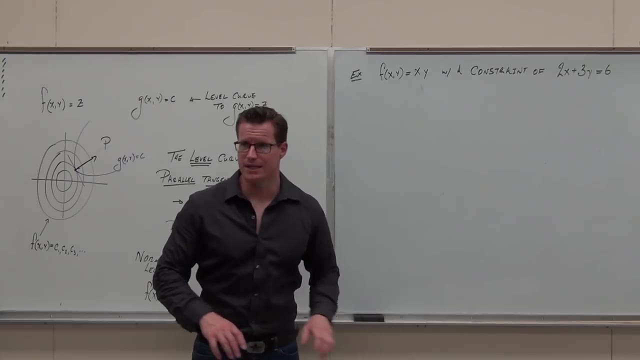 I'm not going to be super concerned about it. I think that you guys can manage it. What I do care about is you going about doing these problems. Head nod if you're okay with the idea before we go any further. Okay, so how do we do it? 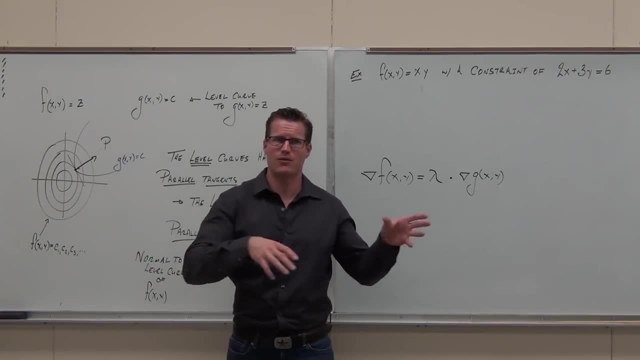 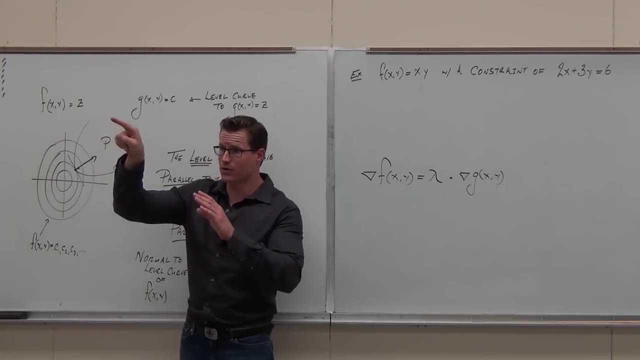 You know, the gradient means normals to level curves. So we use that. We say we want to find the point where the normals are scalar multiples, where they are parallel, where they have basically the same normals, Right? So that's where our one-level curve constraint intersects another level curve. 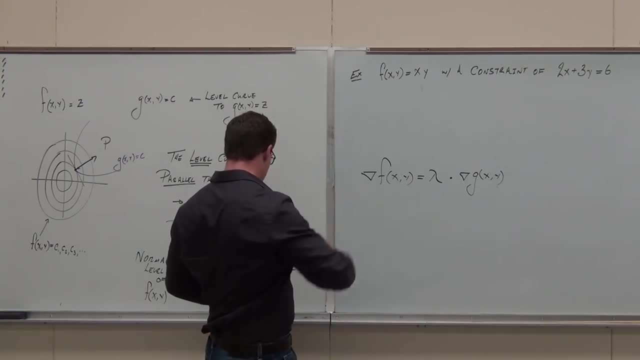 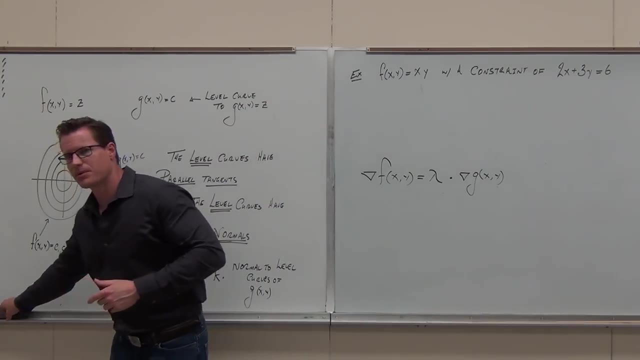 over surface the function. Let's try an example with this. I'll show you how it's done. I've got to tell you right now we're not going to be focusing on word problems because it will take a long time. I'm focused on setup and the operations behind them. 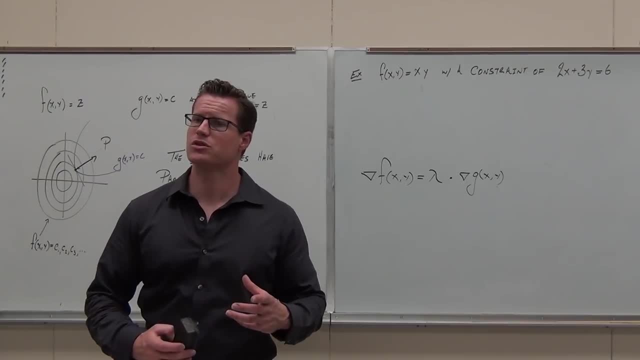 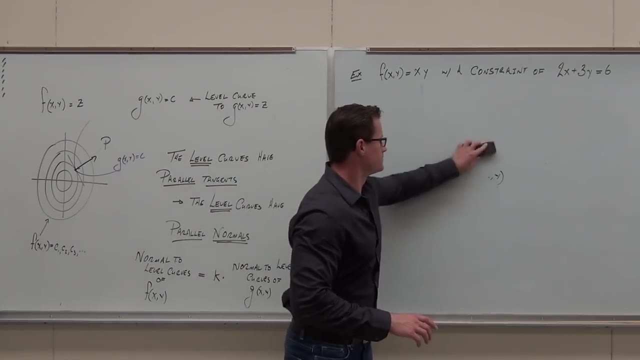 Word problems do happen. I'm not going to be super concerned about it. I think that you guys can manage it. What I do care about is you going about doing these problems. Head nod if you're okay with that. Okay, I'm going to give you an idea before we go any further. 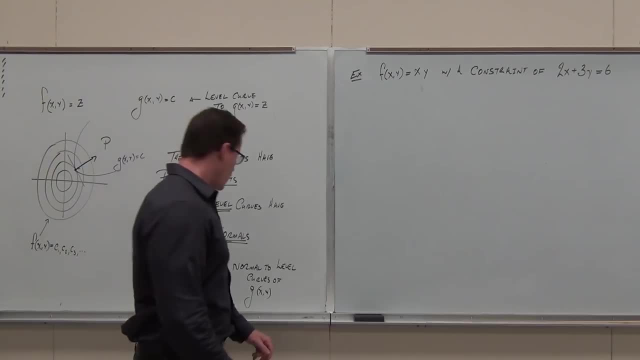 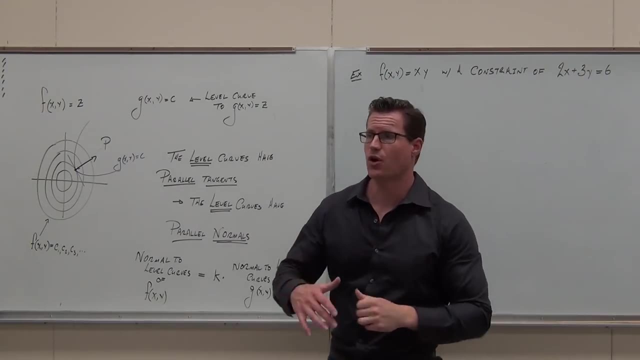 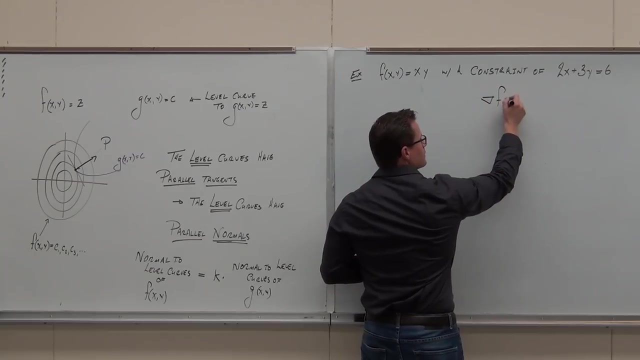 Okay. So how do we do it? Well, the first thing I want you to do is recognize that I'm giving you a surface here and a constraint here. Here's what I want you to do first, The whole goal- where my pants go, the whole goal is to find lambda. 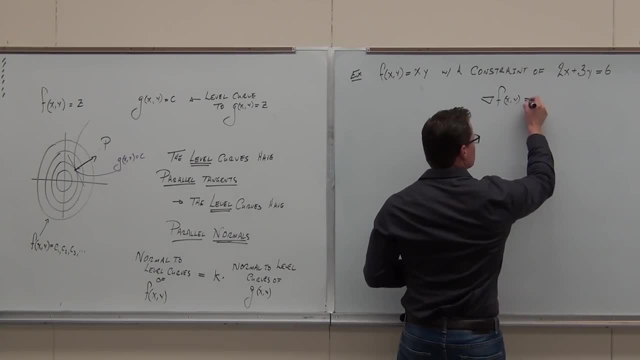 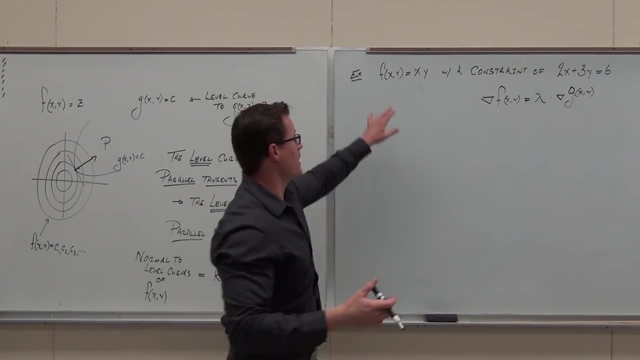 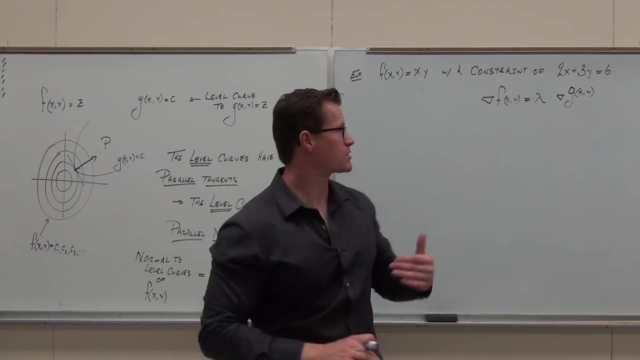 That's a horrible lambda. Horrible to find lambda. So now, here's what's kind of nice. We already have a function f. Do you remember? You remember? You remember a while back, when I gave you like 2x plus 3y equals 6,? 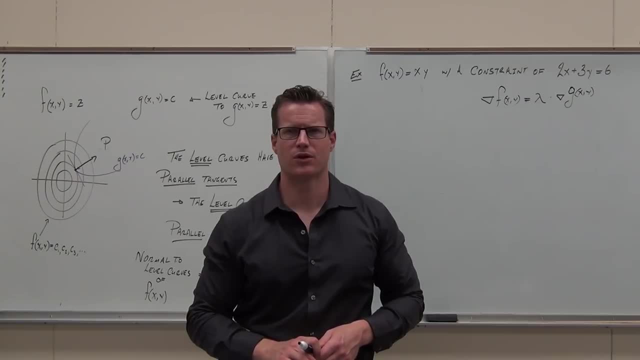 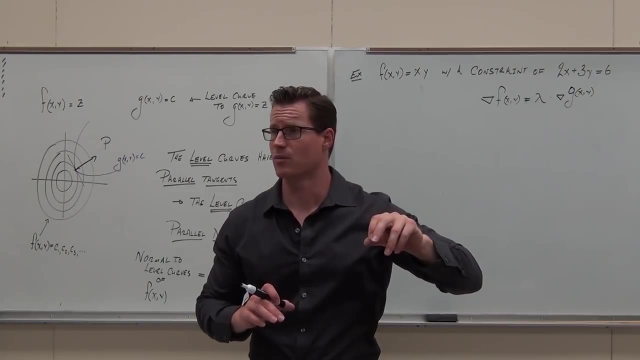 and I said: hey, I want you to pretend that's a level curve, So you're going to find the function higher. That way the gradient gives me the normal to that. Do you remember doing that? It was when we found tangent planes, normal lines, all that sort of stuff. 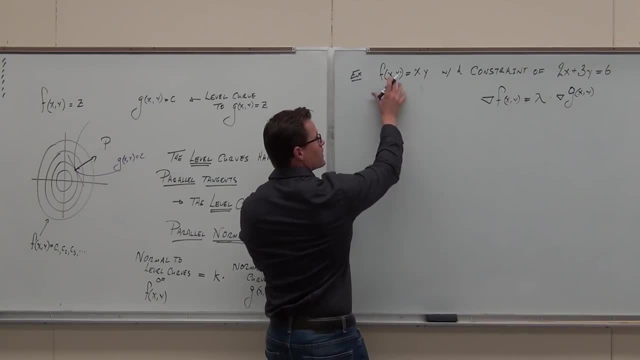 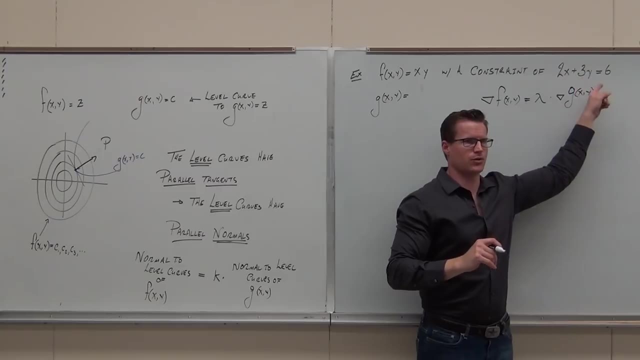 That's what we're going to do, So let's do that here real quick. I already have a function f, but I'm going to create a function g, such that that is a level curve. It's not hard, It's not hard. 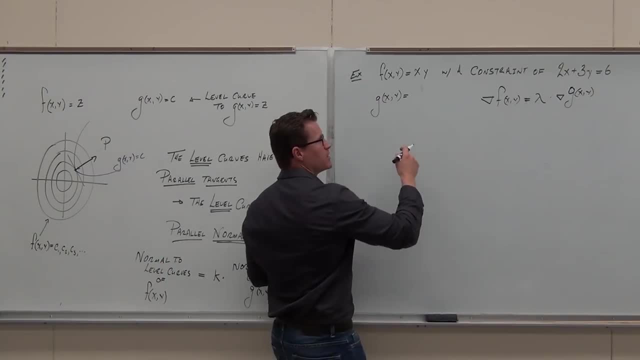 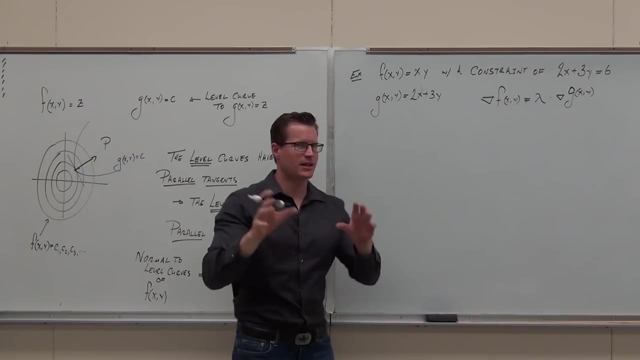 All you got to do is put the function without the constant. So what's g of xy going to be? everybody, please, Yep, Okay. So bear with me here for a second. Is this one specific level curve of this function? 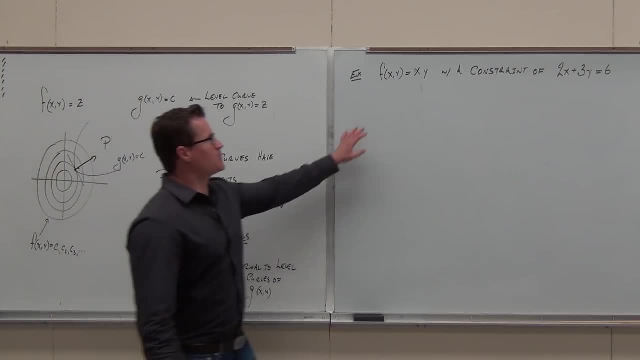 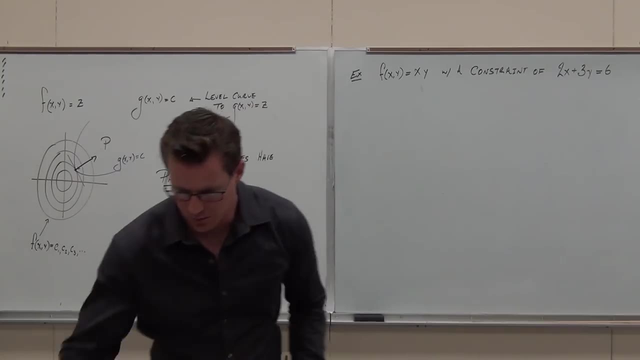 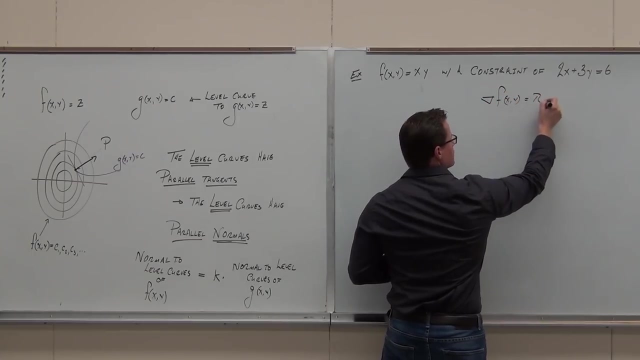 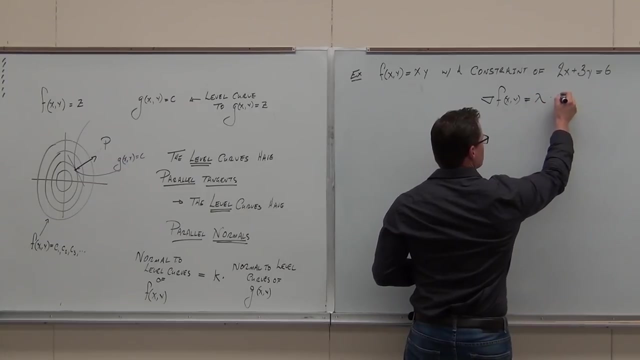 Well, the first thing I want you to do is recognize that I'm giving you a surface here and a constraint here. Here's what I want you to do. first, The whole goal is to find lambda. That's a horrible lambda, Horrible. 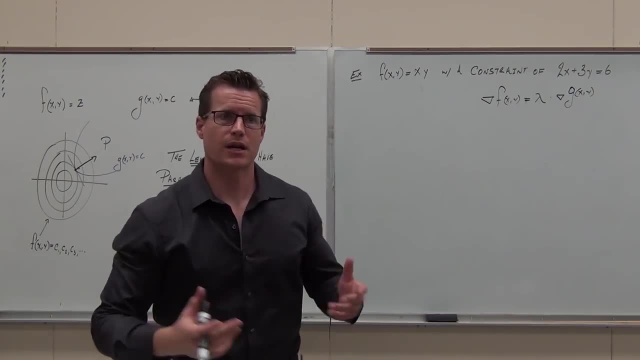 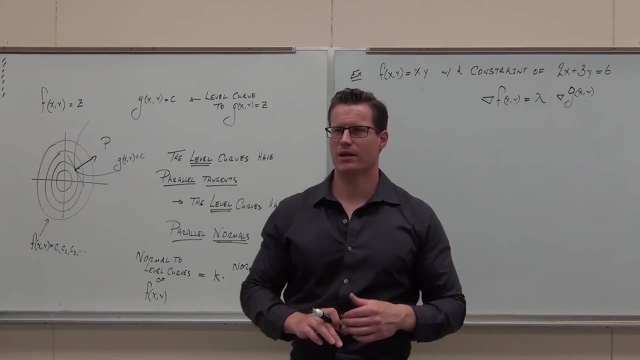 Define lambda. So now here's what's kind of nice: We already have a function f. Do you remember? You remember, You remember a while back, when I gave you like 2x plus 3y equals 6 and I said, hey, I want you to pretend that's a level curve. 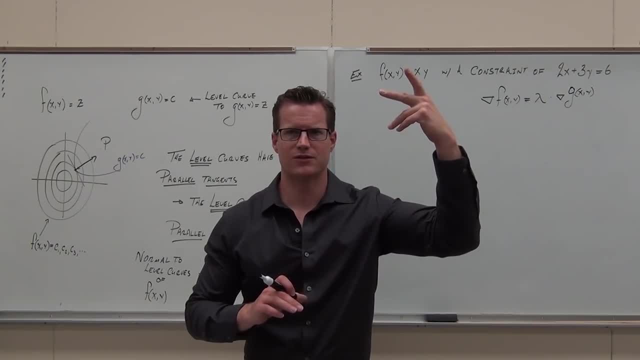 So you're going to find the function higher. That way, the gradient gives me the normal to that. Do you remember doing that? It was when we found tangent planes, normal lines, all that sort of stuff. That's what we're going to do. 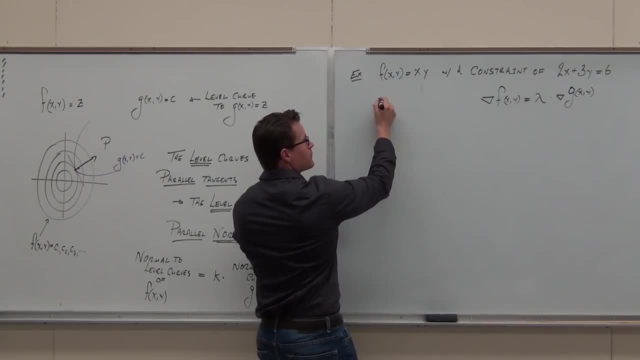 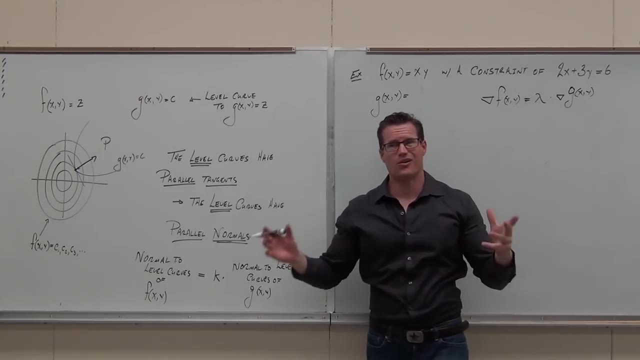 So let's do that here real quick. I already have a function f, But I'm going to create a function g, such that that is a level curve. It's not hard. It's not hard. All you got to do is put the function without the constant. 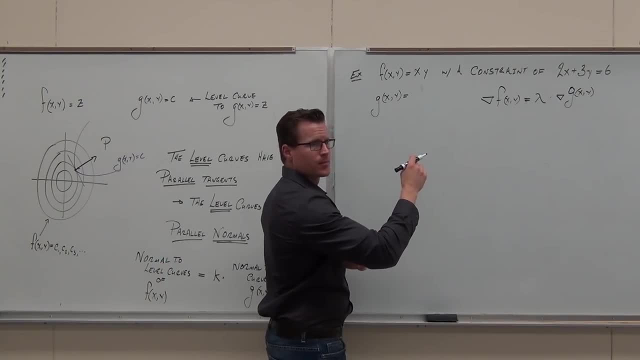 So what's g of xy going to be? everybody, please, 3y, Yep. Okay, let's just bear with me here for a second. Is this one specific level curve of this function? Yeah, namely the one I said- equals 6.. 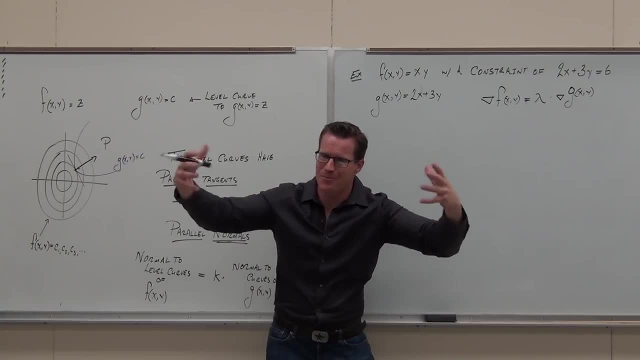 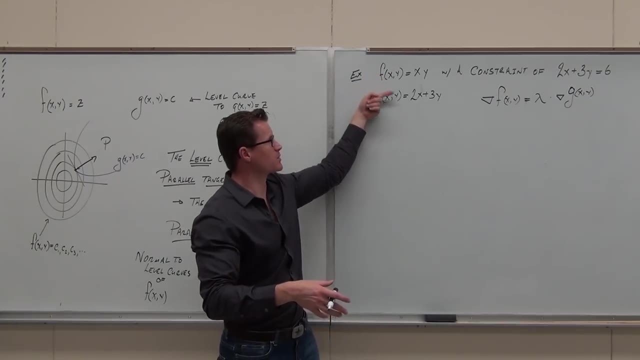 That's a level curve. That's what we're doing. Now, come on, put it together. What gives us normals to level curves? Gradients. So now that I have a function of two variables and a function of two variables, all we got to do is find the gradient, because the gradient is going to give us the normals to that function: level curves. 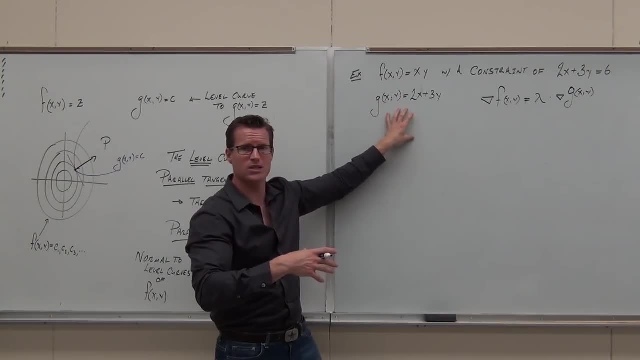 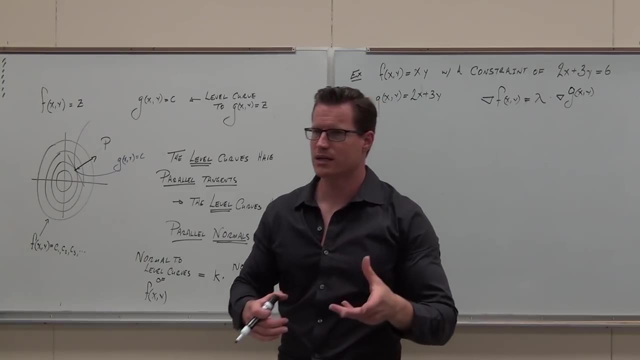 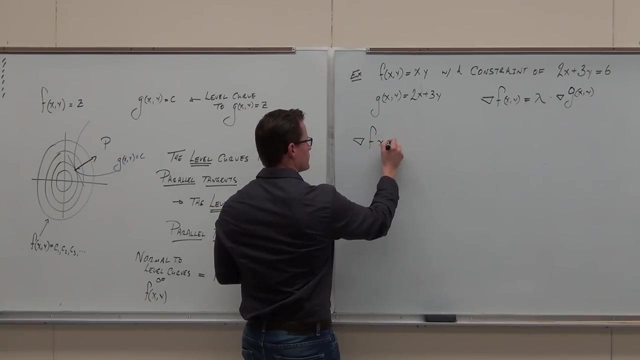 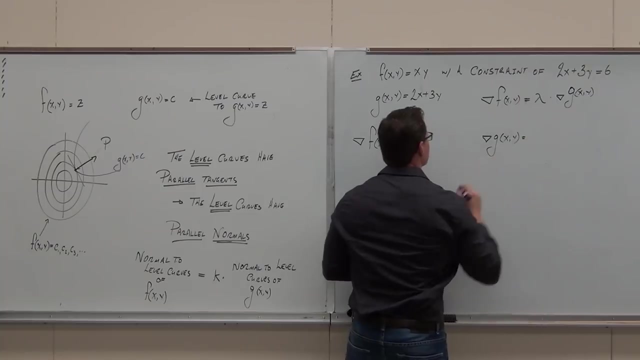 And the gradient is going to give us the normals to that function's level curves, including that one, the one I care about. So let's go ahead and do this right now. Can you find gradient of f and gradient of g? Do you remember how to do the gradient? 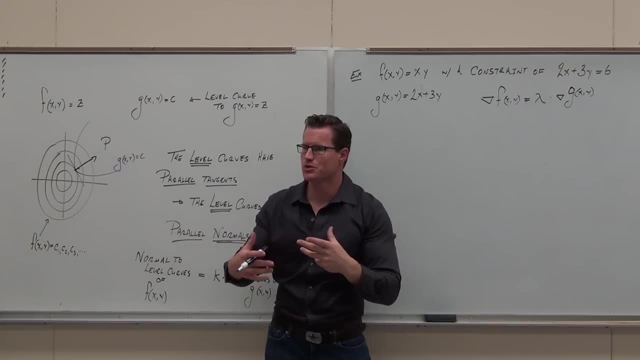 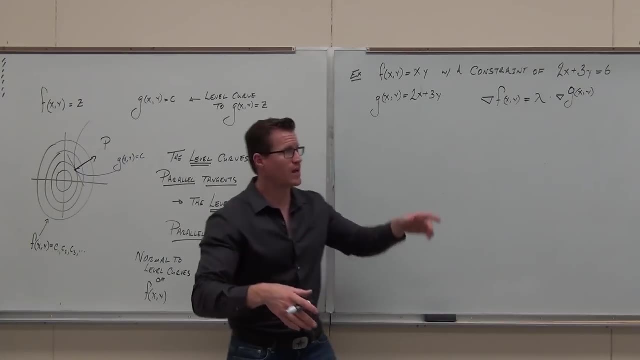 Yes, Yeah, namely the one I said, equals 6.. That's a level curve. That's what we're doing Now. come on, put it together. What gives us normals to level curves? Gradients. So now that I have a function of two variables and a function of two variables, 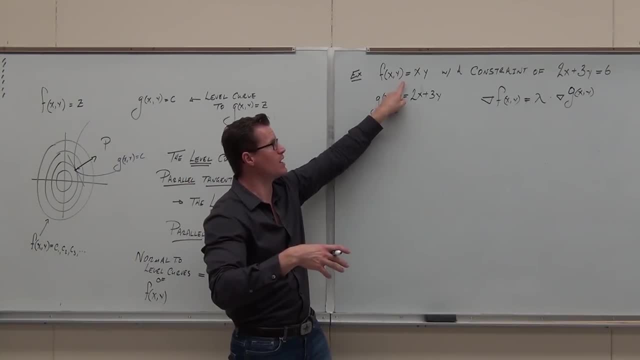 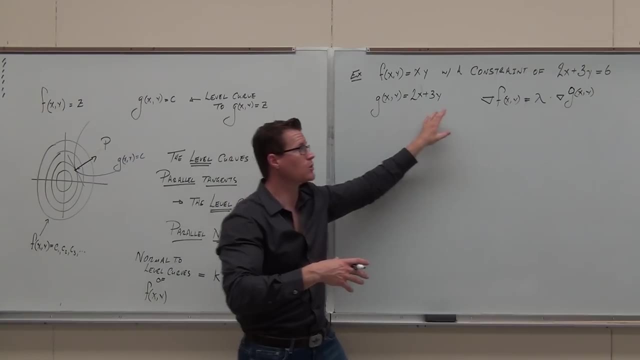 all we got to do is find the gradient, because the gradient is going to give us the normals to that function's level curves, and the gradient is going to give us the normals to that function's level curves, including that one, the one I care about. 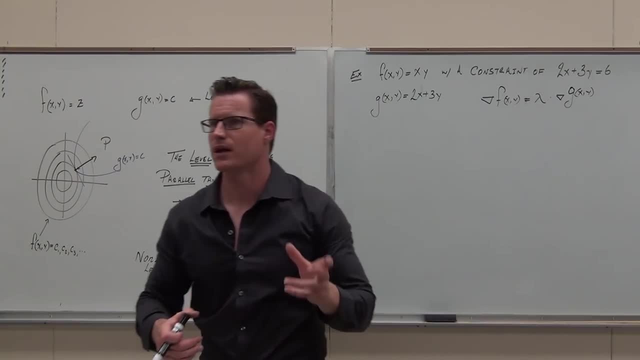 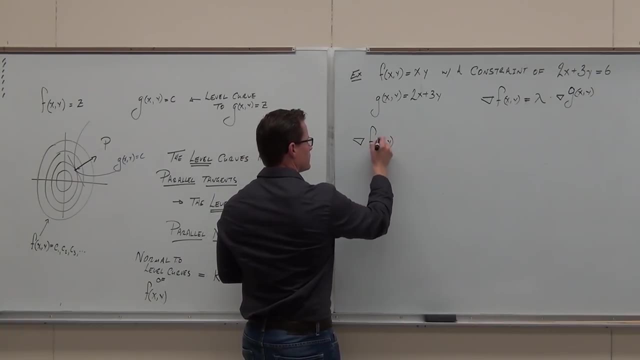 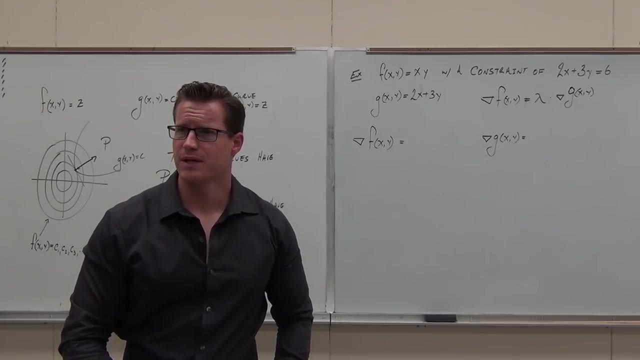 So let's go ahead and do this right now. Can you find gradient of f and gradient of g? Do you remember how to do the gradient? It's been a while. You take the partial derivative with respect to xi plus the partial derivative with respect to yj. 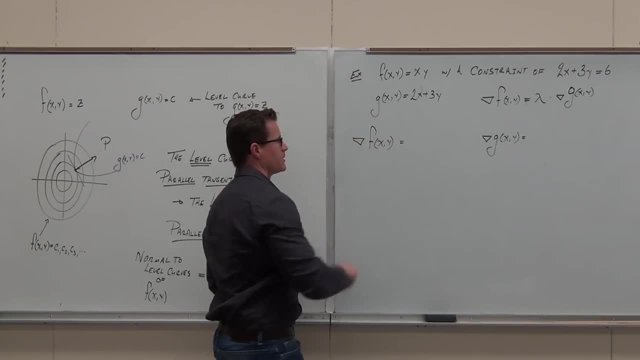 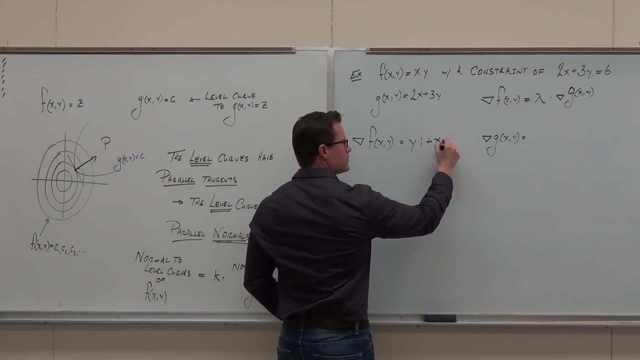 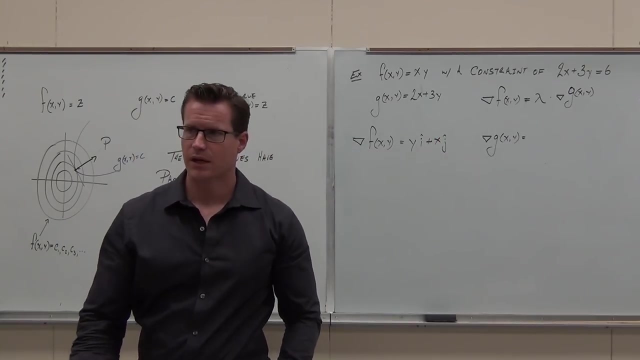 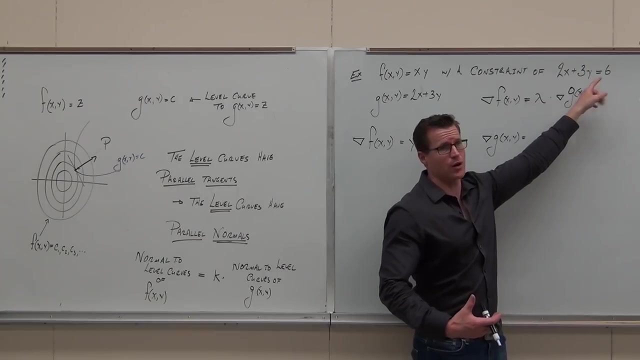 That's all you got to do. So for f, the gradient of f is yi plus xj. I don't know if you're okay with that one. How about for the g? Do I take the gradient of this one? So I'm going to get rid of the level curve. 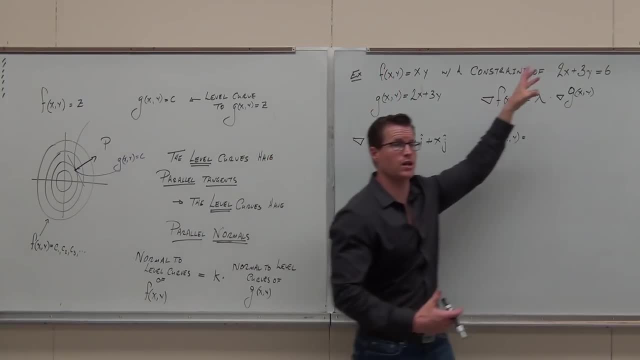 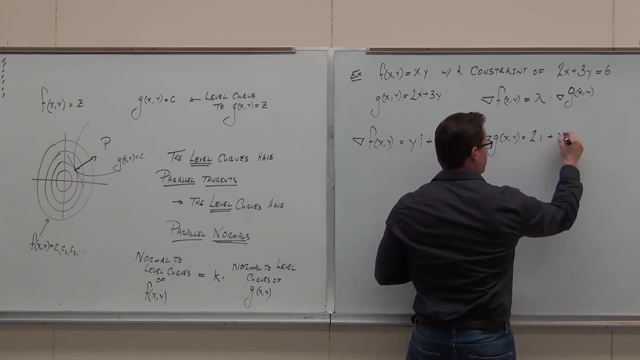 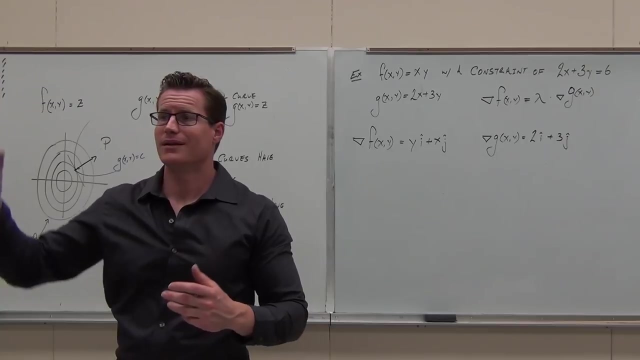 I want to take the gradient of the higher function. That way it gives me the normals to the level curve that I'm looking for. So the gradient of this gives us come on quickly. So thanks for being okay with that, It's not hard. 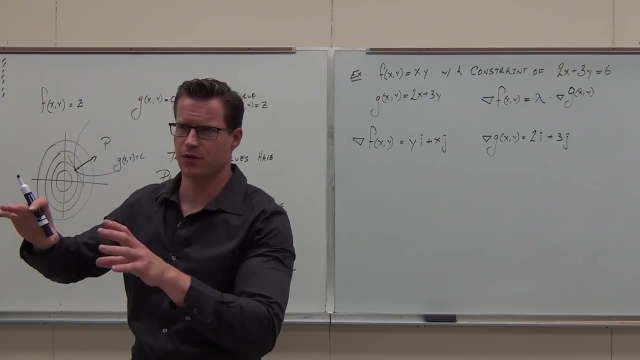 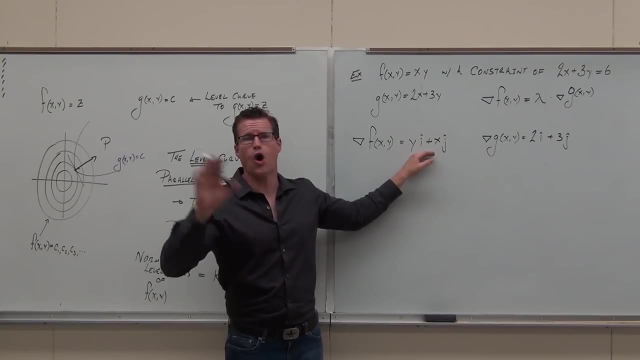 We spent a whole lot of time. so you get the understanding. Here's what we've done so far. Please look carefully. Here's what we've done. We've found an equation that will give us the normals- normals to all of the level curves of that surface. 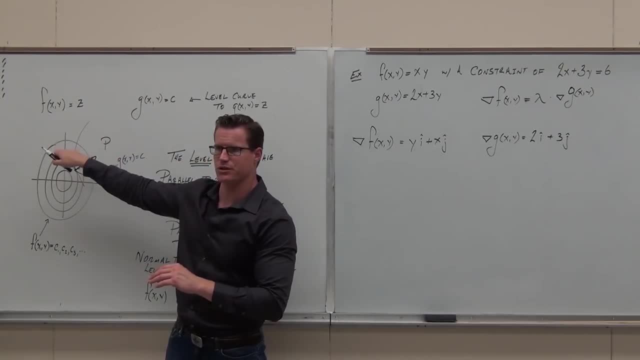 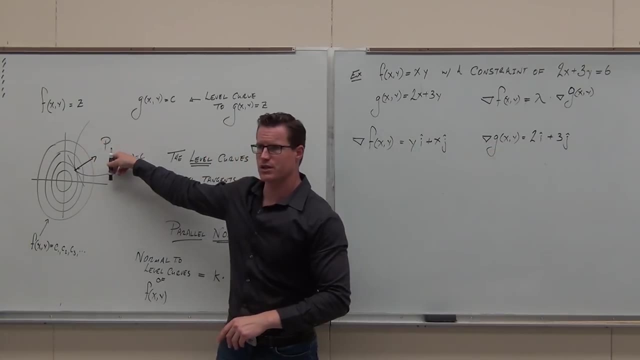 Basically, we found the equation is going to give us the normals to all of these little black circles here. Does that make sense? We've also found the equation that's going to give us the normal to anything on this level curve itself. What we're looking for is the place where they're equal. 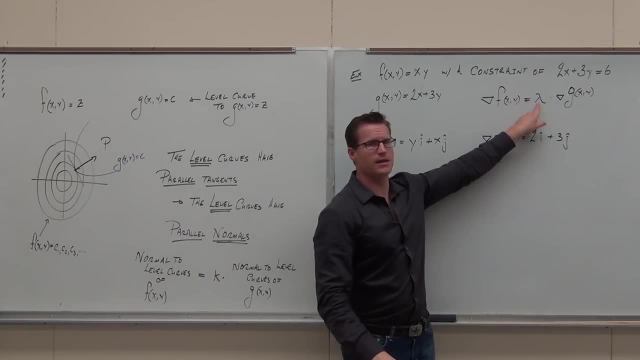 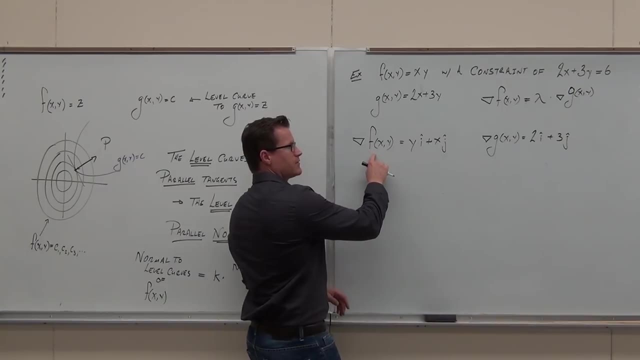 or at least scalar multiples. That's what this says. Find the scalar multiple and we've solved the problem. Does that make sense? So we go okay. well, now the gradient of F is equal to lambda, the Lagrange multiplier times the gradient of G. So 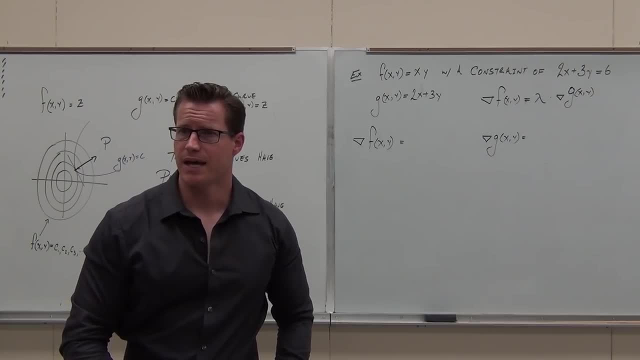 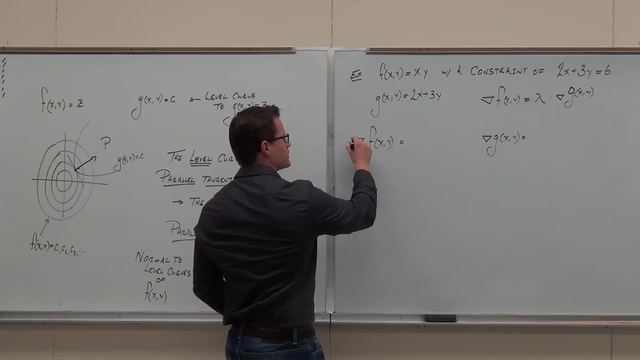 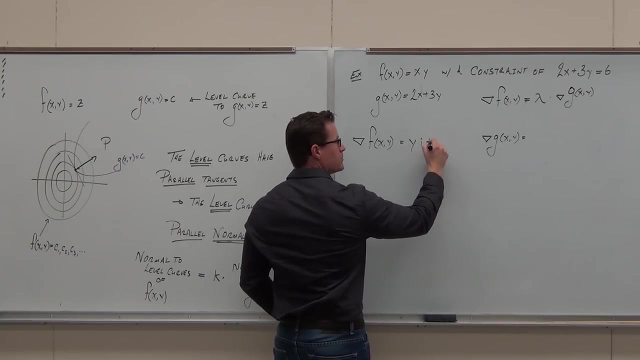 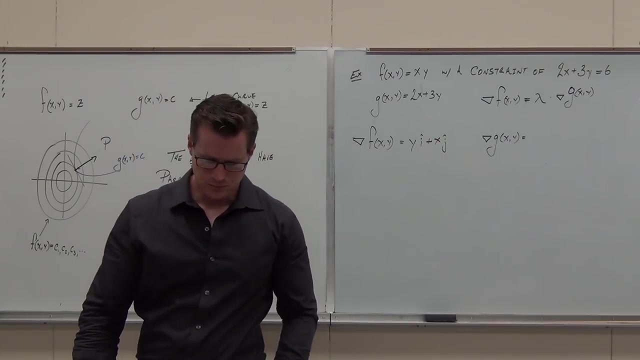 You take the partial derivative with respect to xi plus the partial derivative with respect to yj, That's all you got to do. So for f, the gradient of f is yi plus xj. I don't know if you're okay with that one. 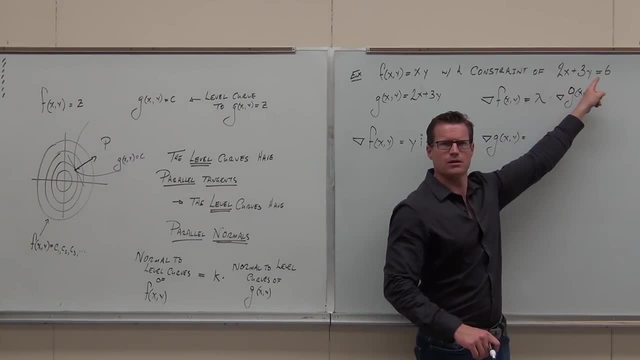 How about for the g? Do I take the gradient of this one? That's already a level curve. I want to take the gradient of the higher function. That way it gives me the normals to the level curve that I'm looking for. 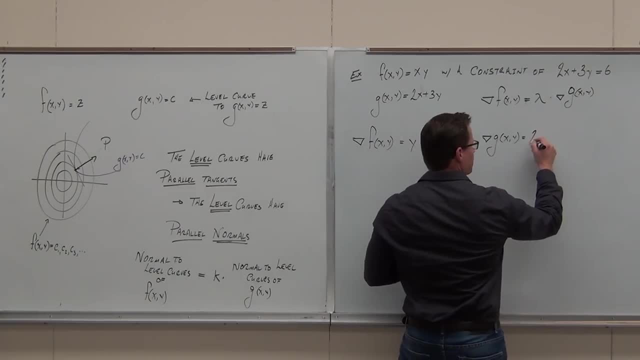 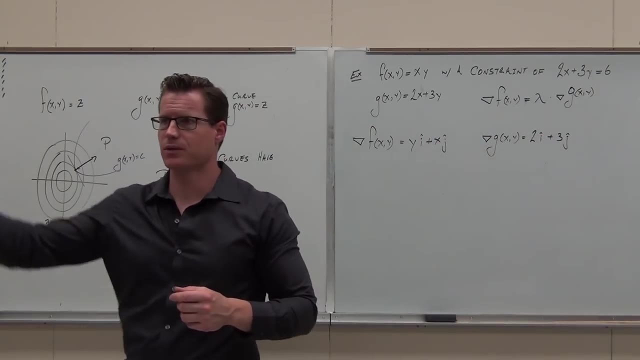 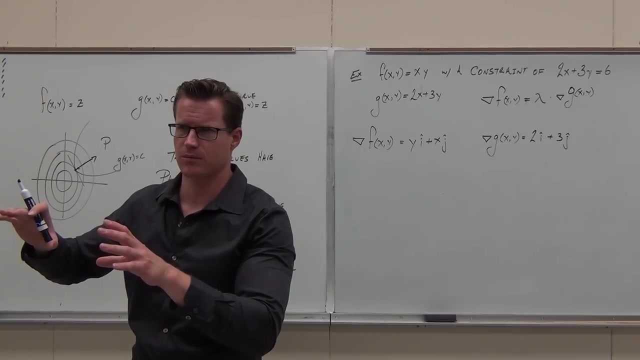 So the gradient of this gives us come on quickly So you guys feel okay with that. It's not hard. We spent a whole lot of time so you get the understanding. Here's what we've done so far. Please look carefully. 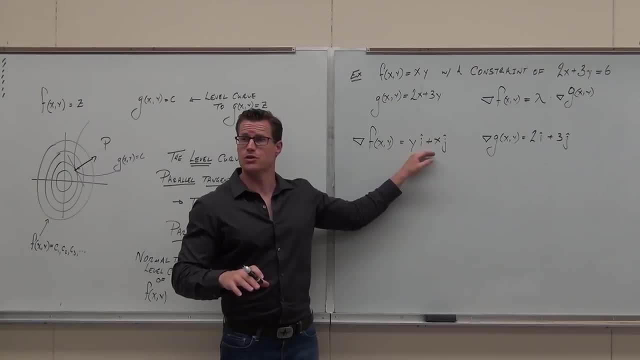 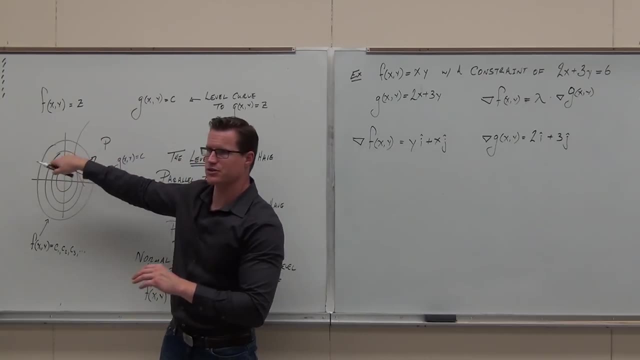 Here's what we've done: We've found an equation that will give us the normals to all of the level curves of that surface. Basically, we've found the equation that's going to give us the normals to all of these little black circles here. 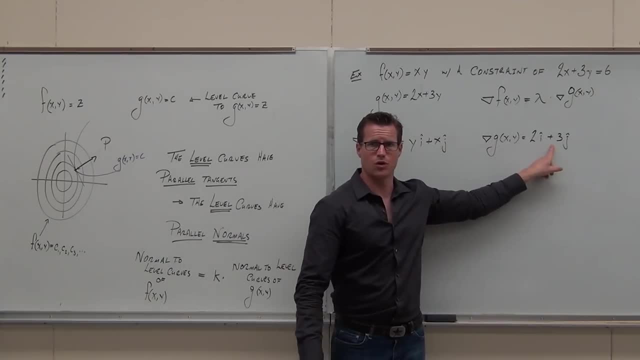 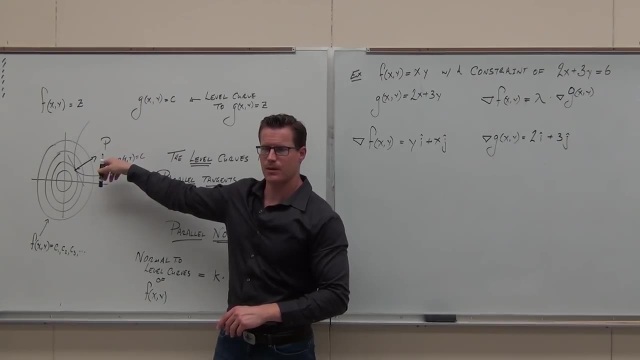 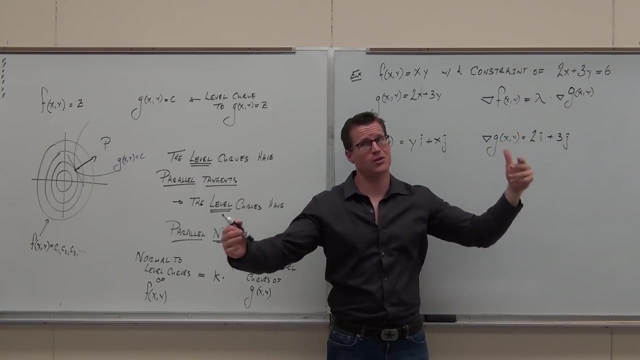 Make sense. We've also found the equation that's going to give us the normal to anything on this level curve itself. What we're looking for is the place where they're equal, or at least scalar multiples. That's what this says. Find the scalar multiple and we've solved the problem. 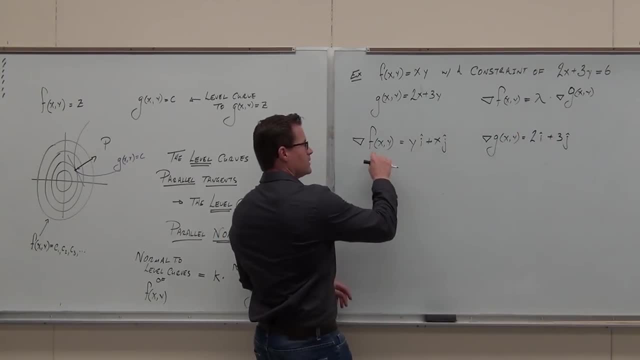 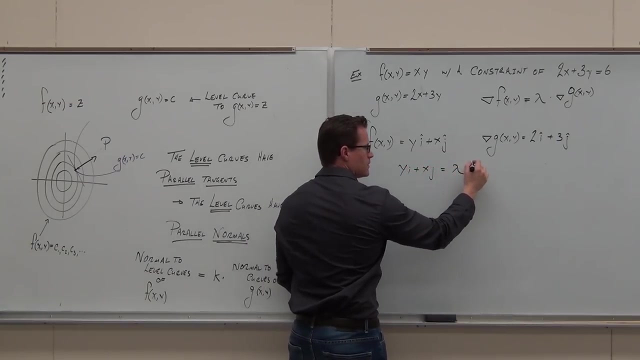 Does that make sense? So we go okay. Well, now the gradient of f is equal to lambda, the Lagrange multiplier times the gradient of g. So here's the gradient of f, Equal to a scalar multiple the Lagrange multiplier. 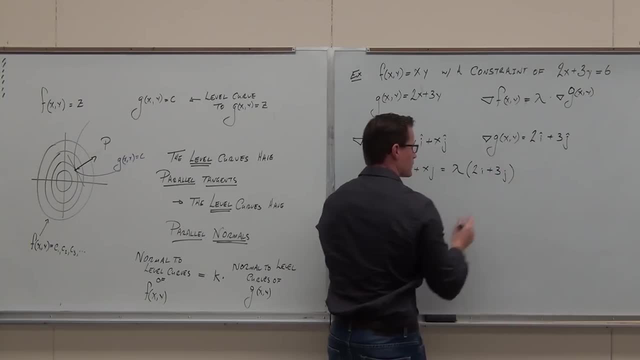 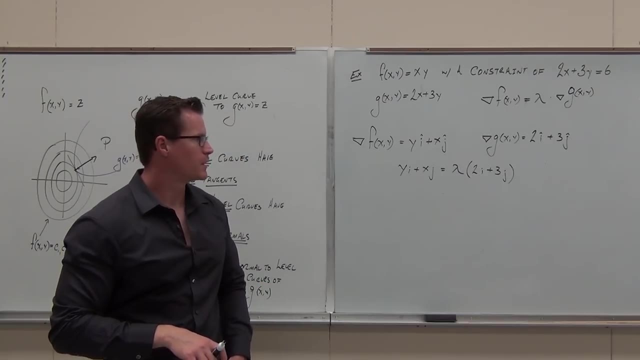 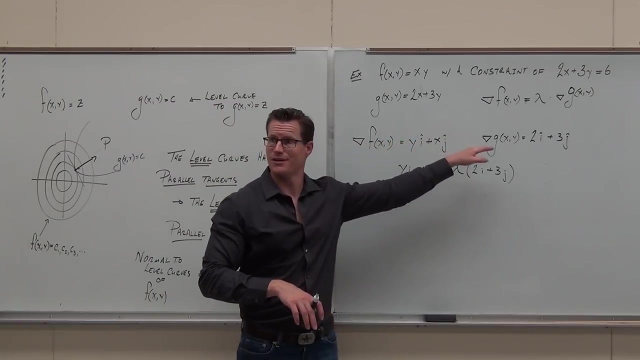 Ladies and gentlemen, do you see where that came from? I don't want to lose you now. You've learned too much. Can you do the gradients? Okay, It's easy. after that Said: this gradient equal to lambda times the other one. 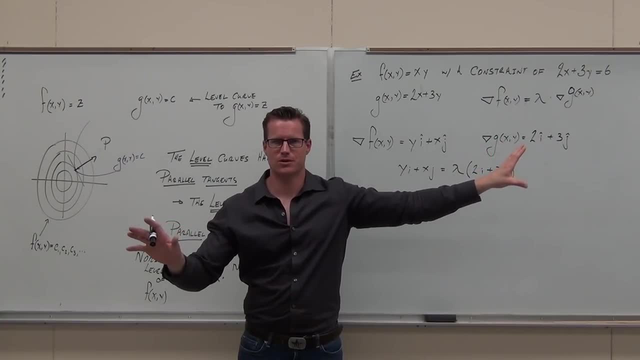 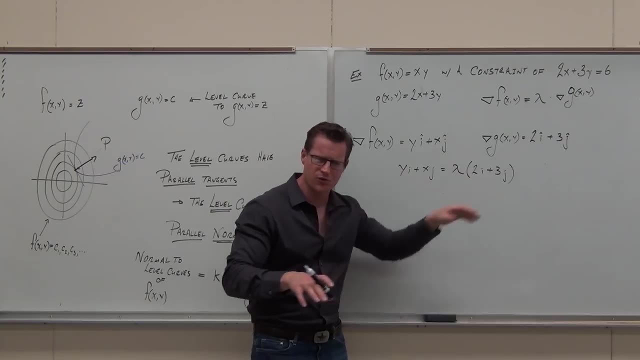 That's all I'm asking for You with me. Now let's use some logic here. Can you distribute the lambda? Yes, Do you understand that for two vectors to be equal- and these are for sure vectors that each component has? 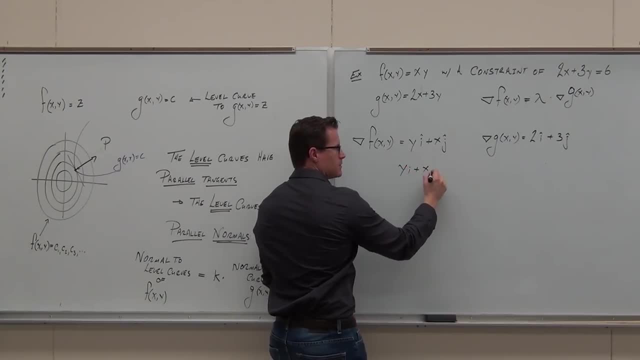 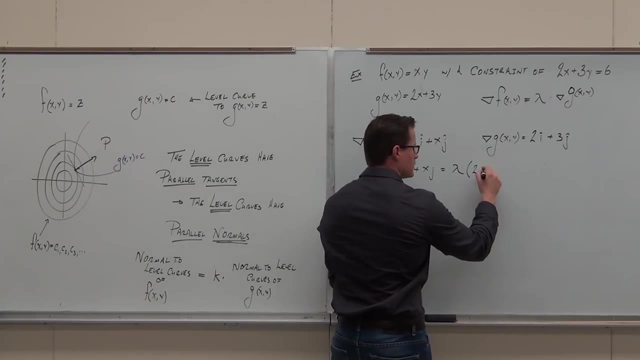 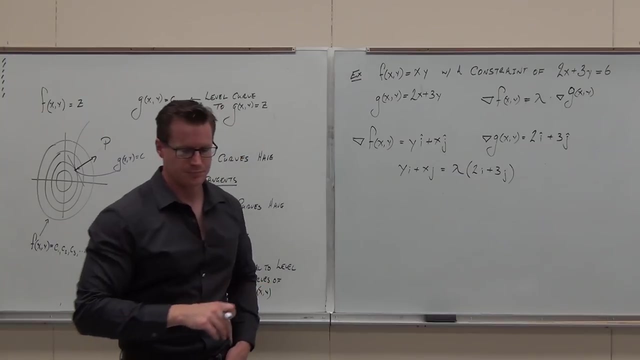 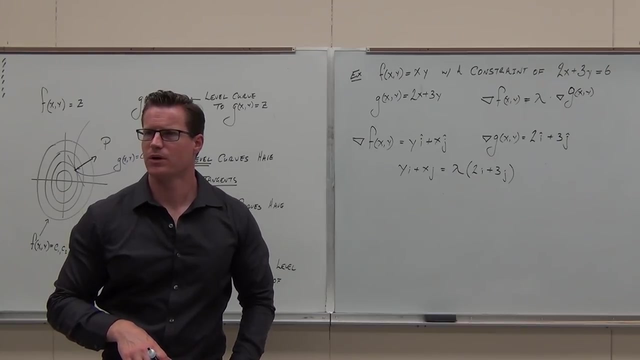 here's the gradient of F, equal to a scalar multiple, the Lagrange multiplier times the gradient of G. Ladies and gentlemen, do you see where that came from? I don't want to lose you now. You've learned too much. Can you do the gradients? 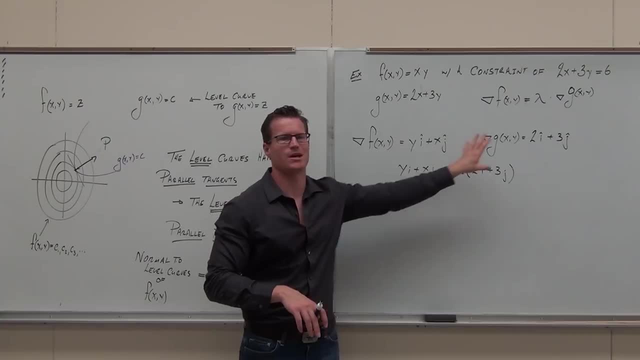 Okay, It's easy. after that, Said this: gradient equal to lambda times the other one. That's all I'm asking for You with me. Now let's use some logic here. Can you distribute the lambda? Yes, Do you understand that for two vectors to be equal, 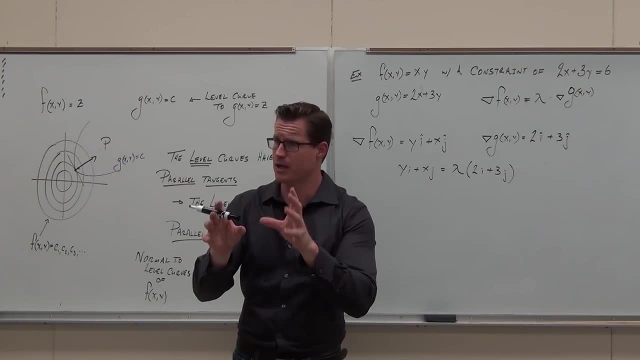 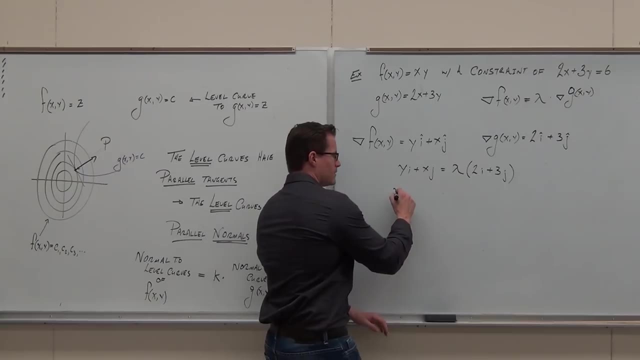 and these are for sure vectors that each component has to be equal. So let's use that. Here's what I'm going to do, You with me. Here's what I know. This Y has to be equal to 2 lambda. 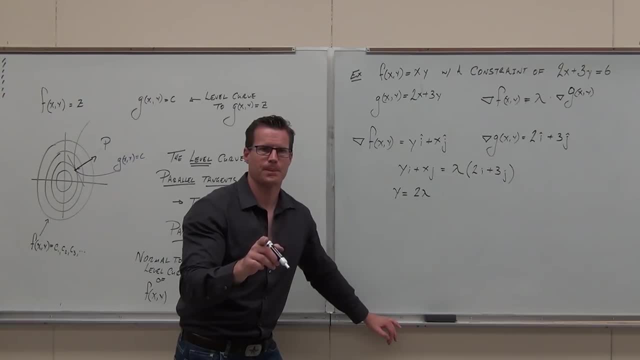 Do you see Y? Do you see? I'm going to have to stick my tongue out forever, Do you see? Do you see Y? Do you see Y? I felt like Michael Jordan there for a second doing math. No, No. 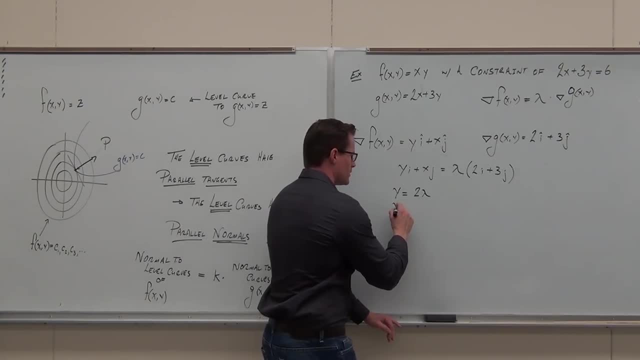 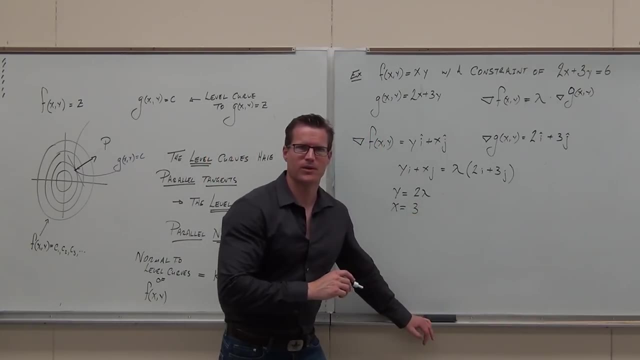 No, I can't jump that high. Okay, If you do see it. what's X equal to 3.. All I heard was rah, rah, rah, But I imagine that you said 3 lambda. Is that what you said? 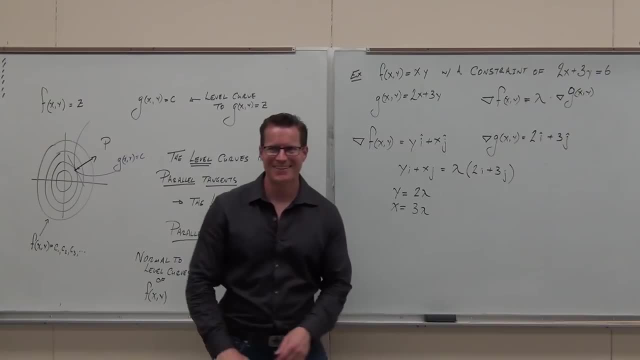 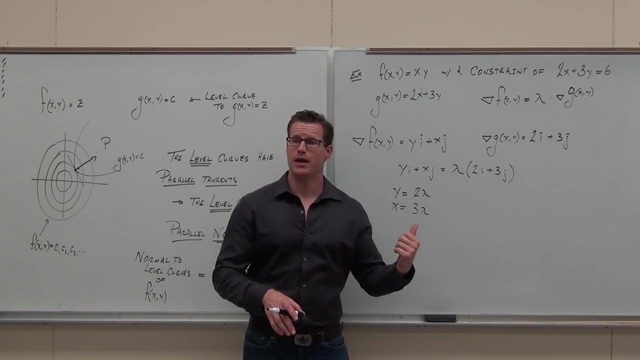 Yeah, This class is fun, This class. Seriously, though, do you guys see what this is? So set this X component equal to this X component, This Y component equal to this Y component, Are you with me? And then write down the constraint. 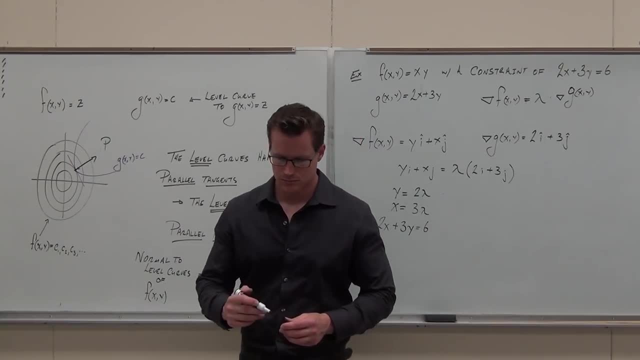 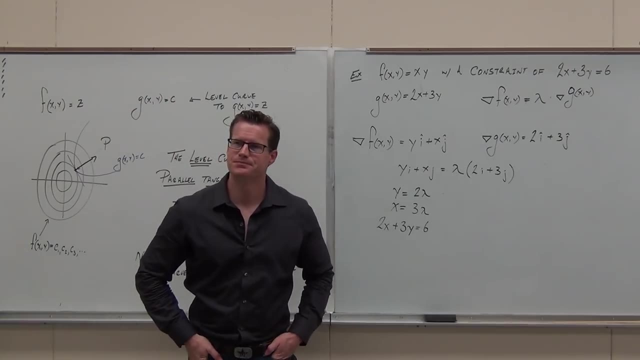 Let's go ahead and write down how many times this dot head was equal to 1 lambda. Ready, Ready, Ready, Ready, Ready. I'm about to tell you your goal in life. Here's your mission in life, in this section of this class. 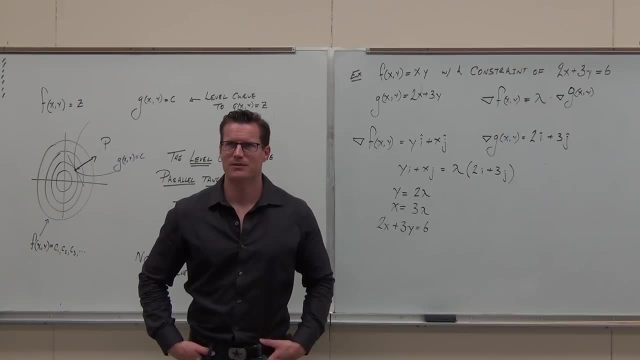 It better not be your mission in life. that would suck Right or what. Oh wait, it's basically my life Doing math. I love it, though It's great. I do math all the time. Ha ha, It's a fantastic job. 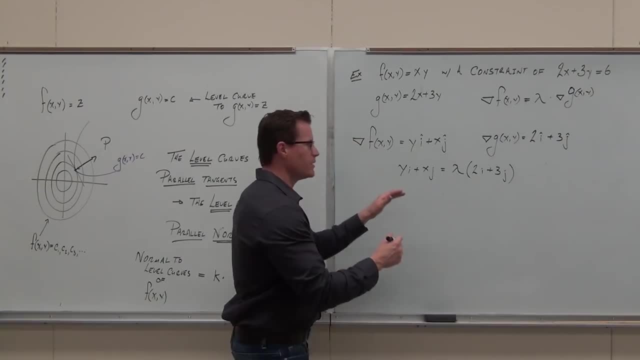 to be equal. So let's use that. Here's what I know, You with me, Here's what I know. This y has to be equal to 2 lambda. Do you see? why? Do you see, I'm going to stick my tongue out forever. 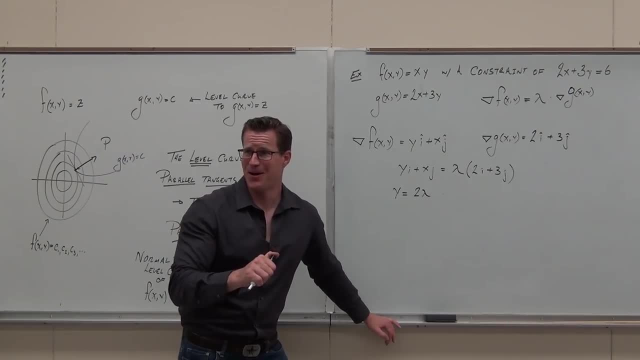 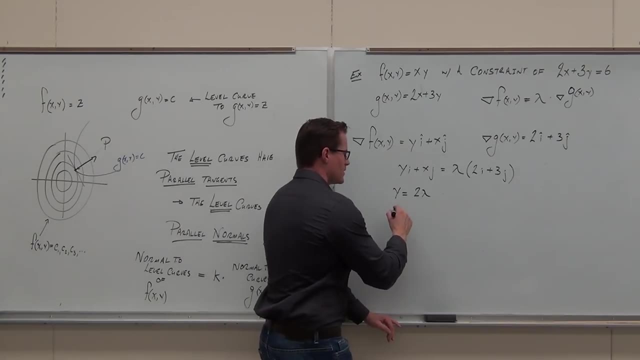 Do you see? Do you see why? Do you see why I felt like Michael Jordan there for a second doing math. No, No, I can't jump that high. Okay, If you do see it, what's x equal to? 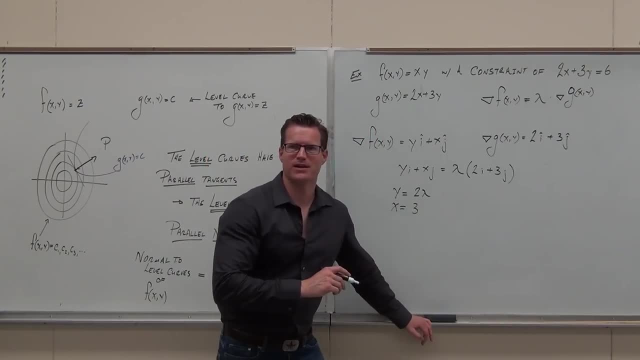 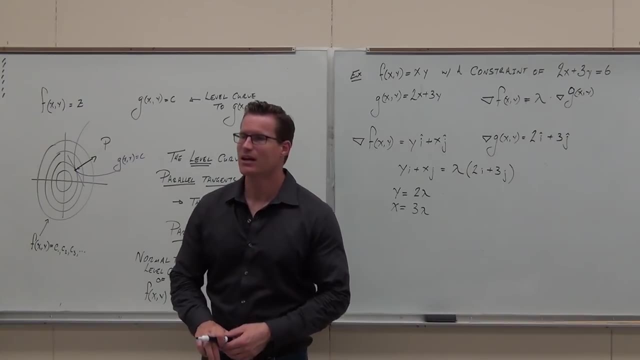 3. All I heard was rah, rah, rah, But I imagine that you said 3 lambda. Is that what you said? Yeah, This class is fun, This class. Seriously, though, do you guys see what this is? 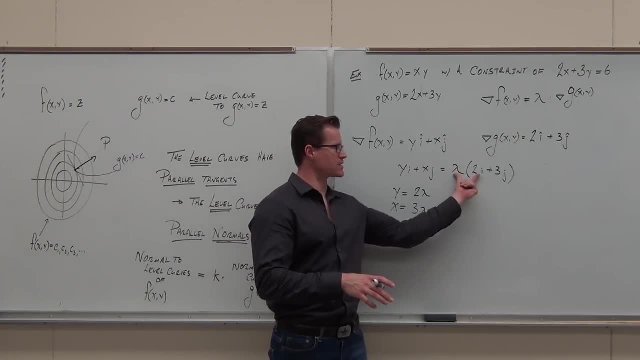 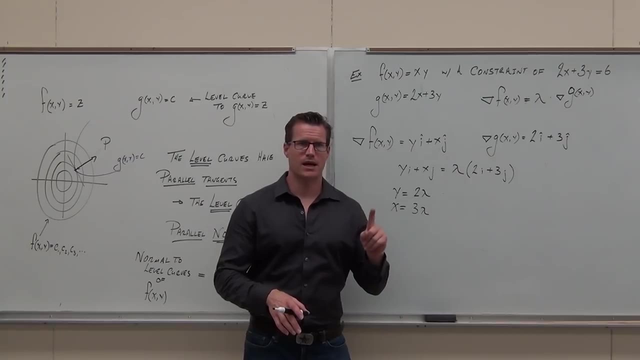 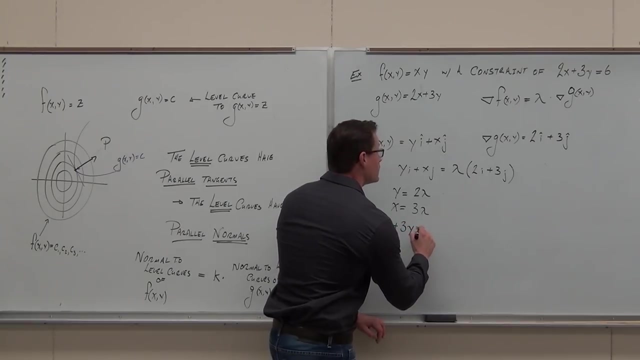 So set this x component equal to this x component, This y component equal to this y component. Are you with me? And then write down the constraint. So if I was at x and I'm at y and I'm at y, I could write down y. 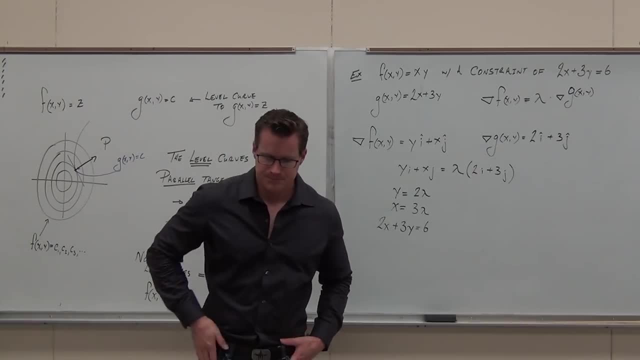 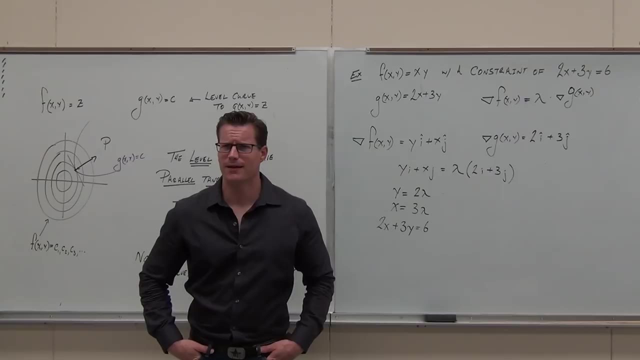 Like I do, that I could write down. you know, my x is equal to y. Ready, Ready, Ready, Ready, Ready. I'm about to tell you your goal in life. Here's your mission in life, in this section, in this class. 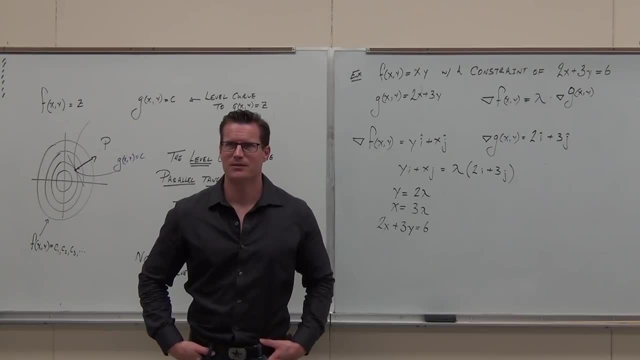 It better not be your mission in life. That would suck Or what. Oh wait, It's basically my life: Do math all the time. I love it, though. It's great You can do math all the time. It's a fantastic job. you should all do it. 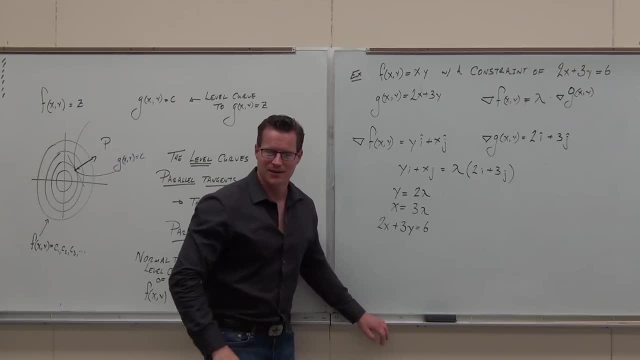 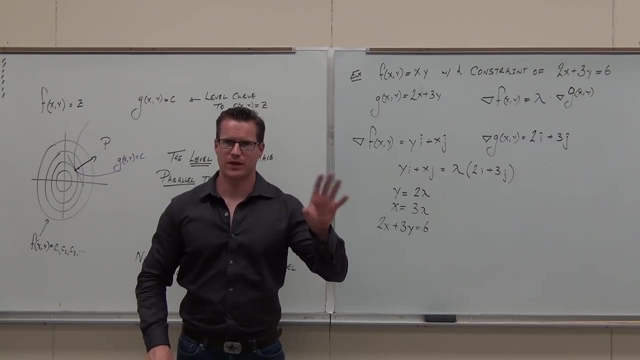 No, wait, that's I need job security. You all find something else to do, okay. Okay, so I'm a math teacher. Here's your main goal in life: solve lambda. Do whatever it takes to solve for lambda and then plug it in. 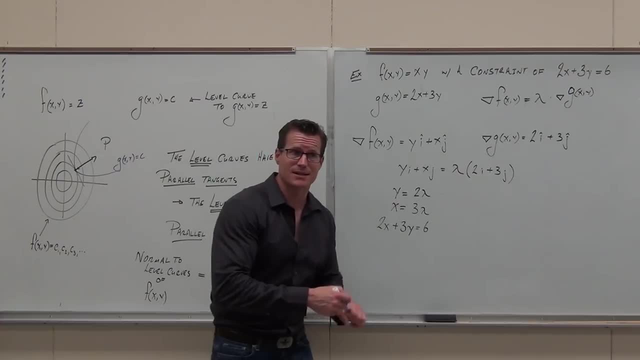 That's your main goal in life. It can be really really easy like this one. Look, look, I have an equation correct. Can I substitute something in for x and y? that lets me solve for lambda. This is the easiest type where you have a direct substitution. 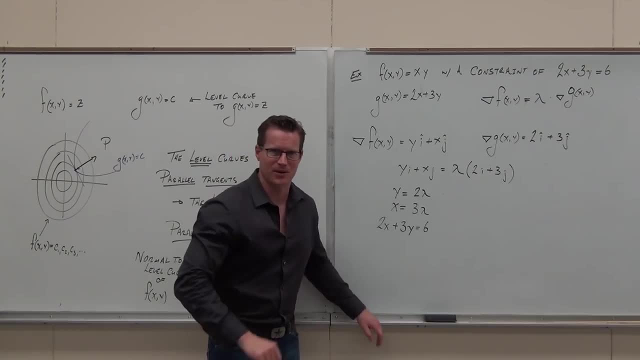 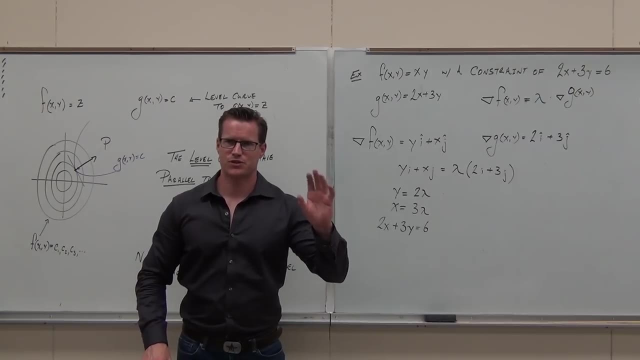 You should all do it. No, wait, I need job security. You all find something else to do, okay. Okay, So I'm a math teacher. Here's your main goal in life: Solve lambda, Do whatever it takes to solve for lambda and then plug it in. 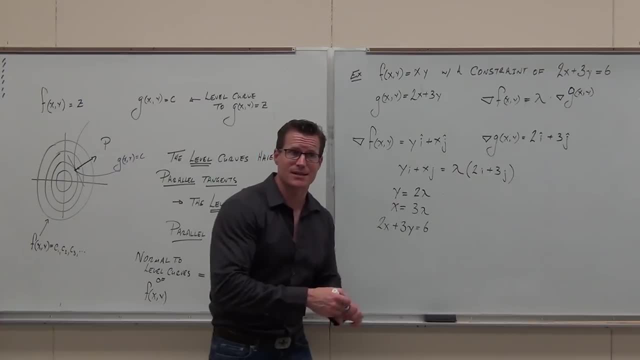 That's your main goal in life. It can be really really easy like this one. Look, look, I have an equation correct. Can I substitute something in for x and y? that lets me solve for lambda. This is the easiest type where you have a direct substitution. 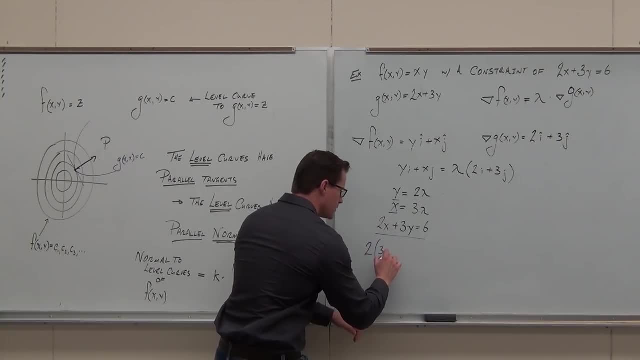 You go: oh hey, here's 2 times 3 lambda plus 3 times 2 lambda equals 6.. So take y Got it, Take x Got it. Make your substitution Solve for lambda. Your main goal in life right now in this section is solving for that Lagrange multiplier. 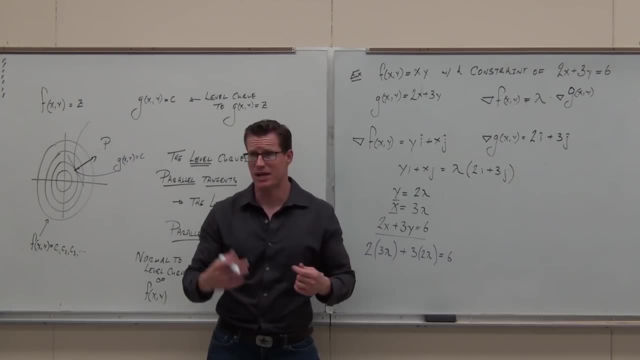 It's basically like what you do on, like direct variation or inverse variation. You have that constant. You've got to find the constant first. That's what we're doing. So here we have- oh well how much- 12 lambda. 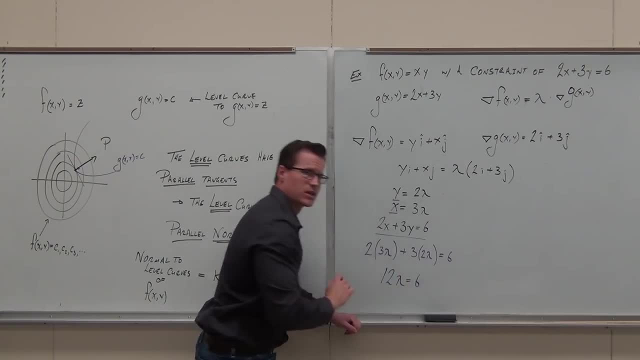 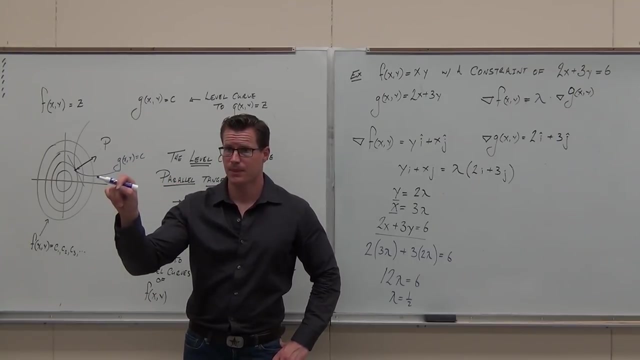 How much is lambda? 12 and a half Perfect, Perfect. Now wait a second. Do you know how to solve for lambda? Do you have something up here that would map lambda back to values of x and y? Yes, Yeah. 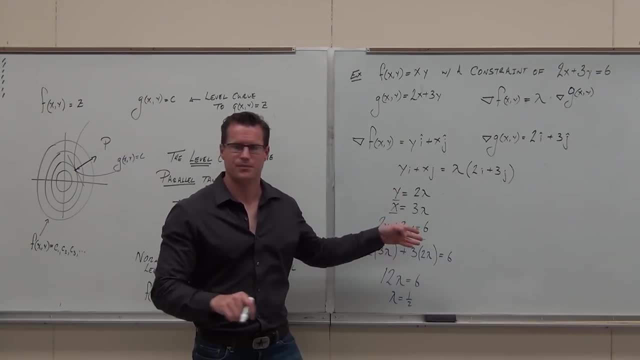 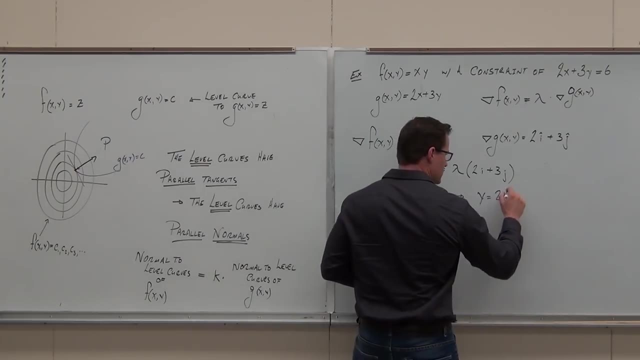 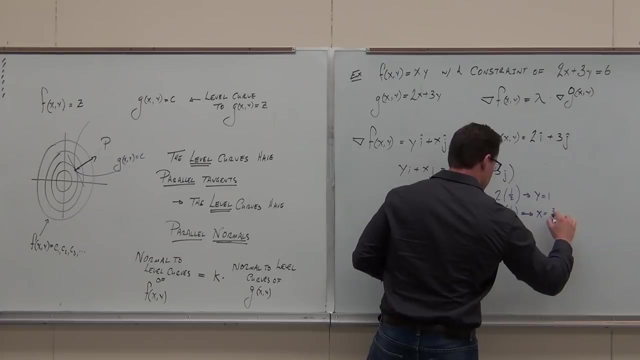 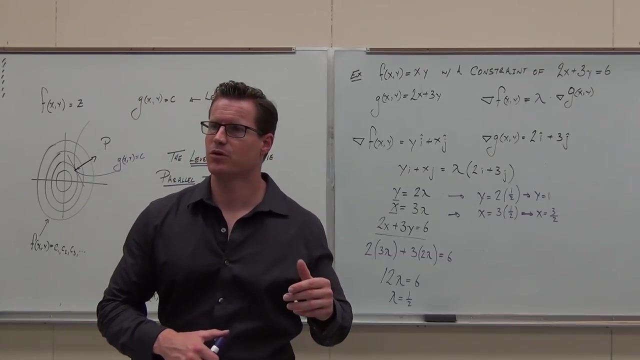 These two We use in concert, all three of them. So y equals 2 lambda, x equals 3 lambda. Here's what it tells us. Remember how we found critical points and all that stuff and then we had to plug in the n values and all that stuff? 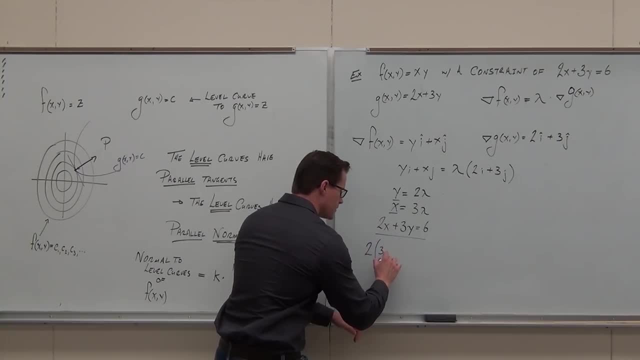 You go: oh hey, here's 2 times 3 lambda plus 3 times 2 lambda equals 6.. So take y got it, take x got it, Make your substitution. solve for lambda, your main goal in life right now. 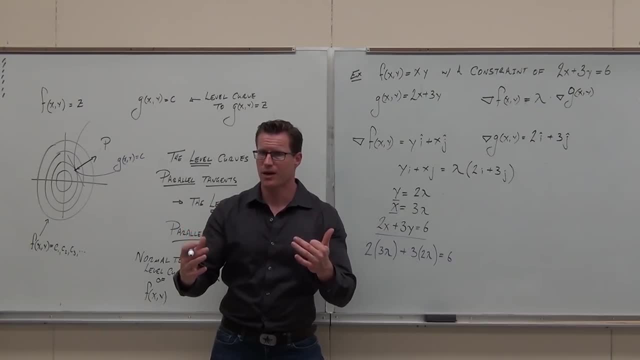 And this section is solving for that- that Lagrange multiplier. It's basically like what you do on, like direct variation or inverse variation. You have that constant. you got to find the constant first. That's what we're doing. So here we have- oh well how much. 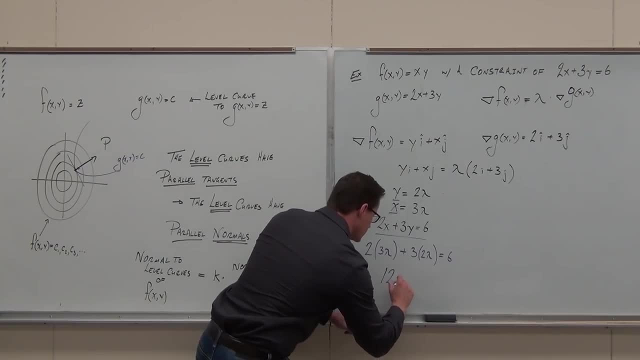 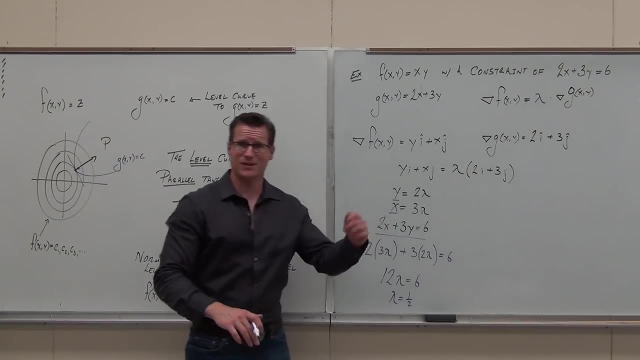 12 lambda, 12 lambda. How much is lambda? 12 and a half Perfect, perfect. Now wait a second. Do you have something up here that would map Lambda back to values of x and y? Yes, Yeah, these two. 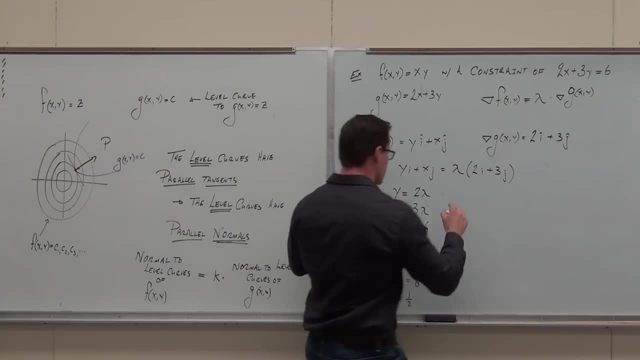 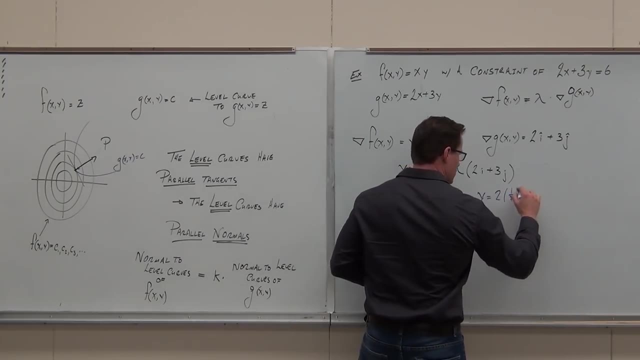 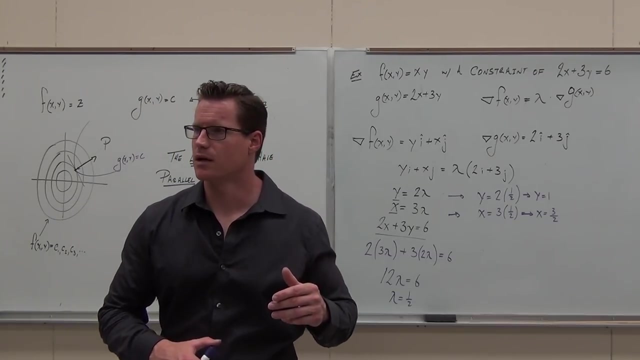 We use in concert all three of them. So y equals 2 lambda, x equals 3 lambda. Here's what it tells us. Remember how we found critical points and all that stuff and then we had to plug in the n values and all that stuff? 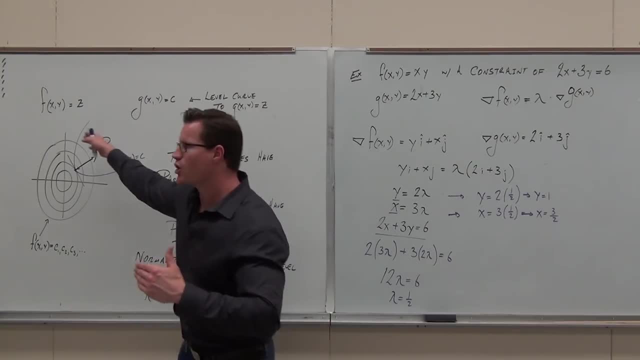 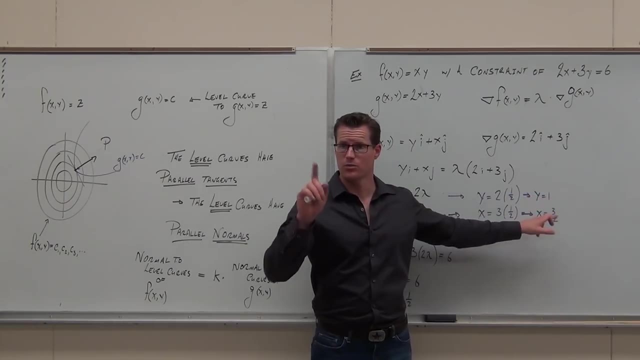 This right here does everything for you Because we based it on a contour plot. I know that. this right here. how many critical points do you have? One, One critical point. Tell me specifically. Tell me specifically. Tell me what it is. 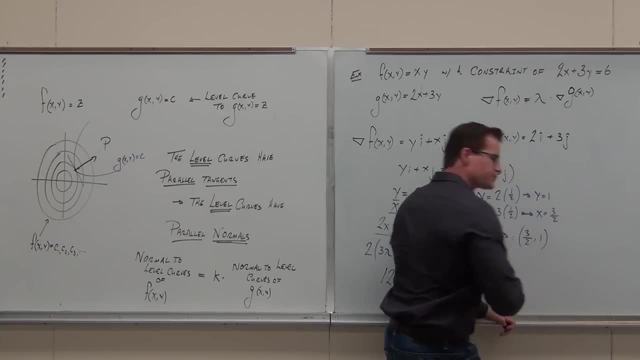 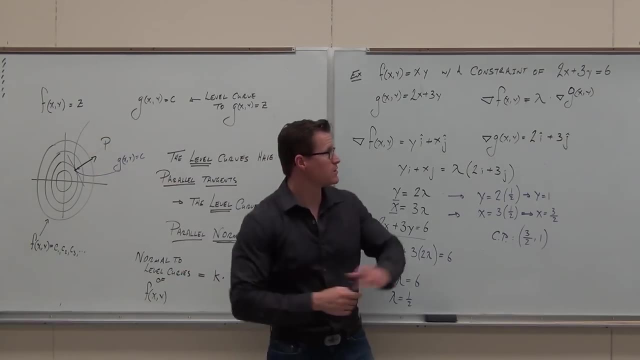 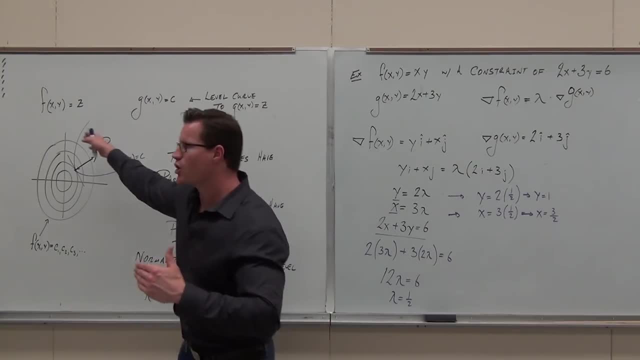 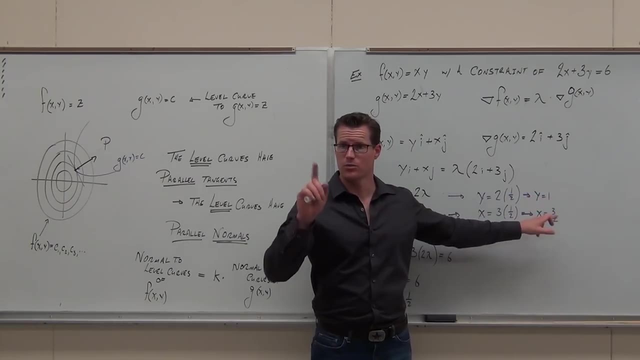 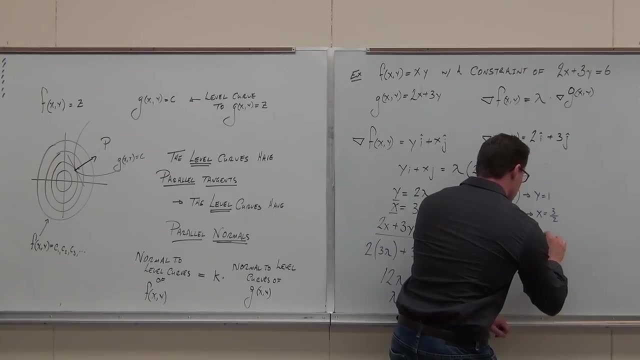 This right here does everything for you Because we based it on a contour plot. I know that. this right here. how many critical points do you have? One, One critical point. Tell me specifically what it is: 3 epsilon, 3 halfs and 3 plus 1.. 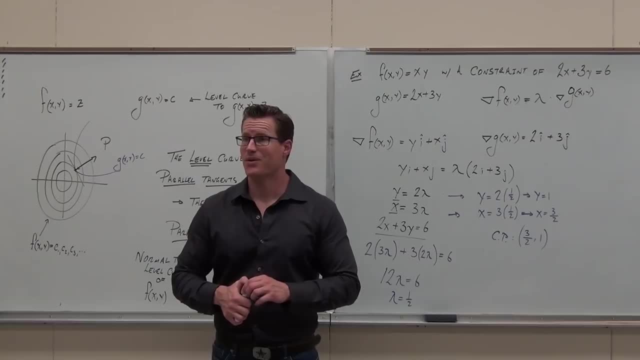 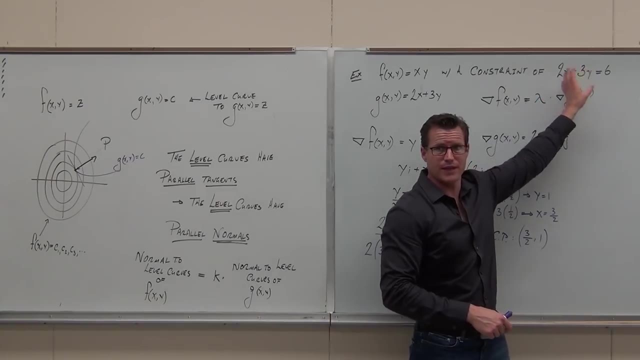 3 halfs and 1.. That right, there is the one critical point. we have That right. there is the one point that this constraint, it's a level curve, That level curve, that constraint is going to bounce off and intersect at one point. 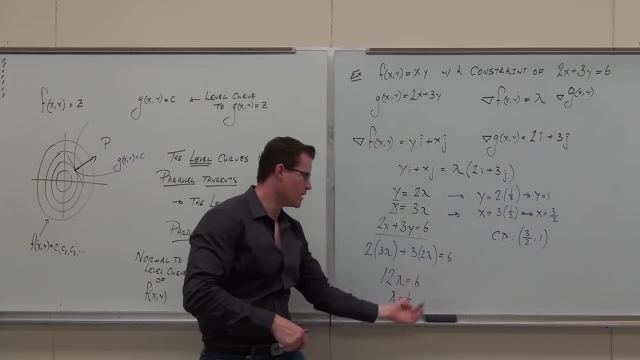 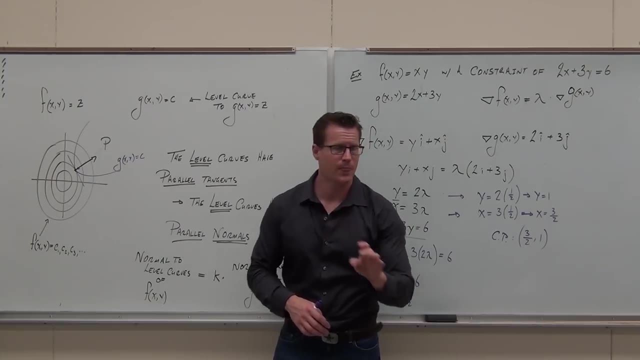 one of these level curves, the one where our lambda happens to be 1 half, We plug it in. We find that one specific point. Here's the last piece of information that I need you to know: All Constraint, maxima and minima will be found at those points. 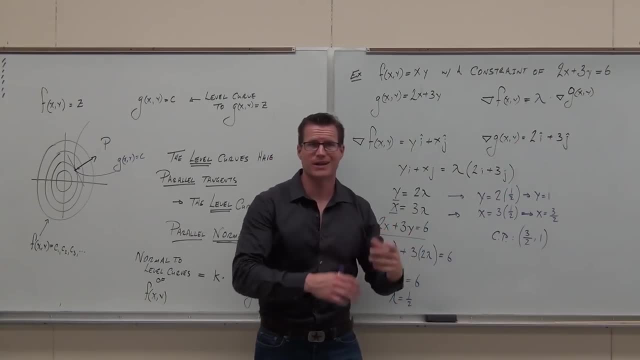 The one where lambda happens to be one half. We plug it in. We find that one specific point. Here's the last piece of information that I need you to know: All constrained maxima and minima will be found at those points. So I know that what these points give us are either maximums or minimums of this function. 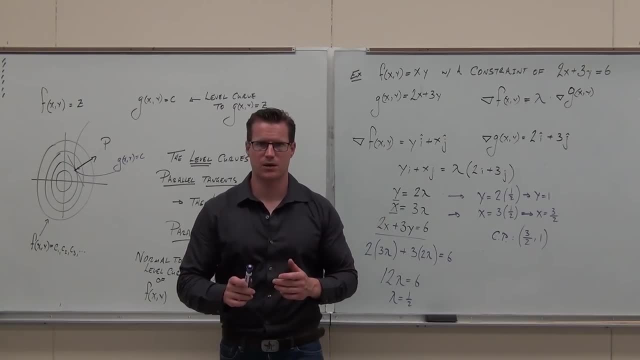 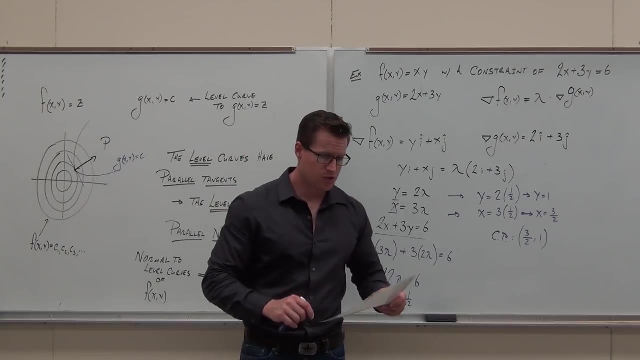 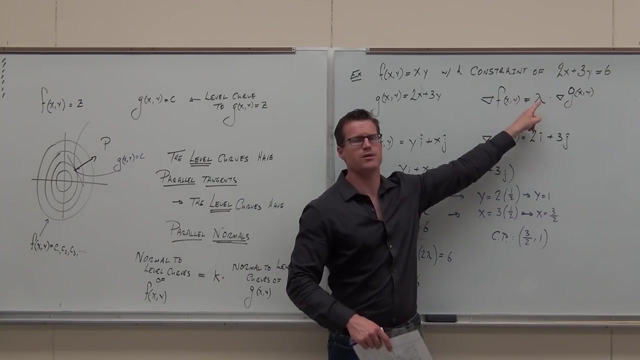 In this case. did you catch that? You might want to write that one down. No, Not constrained. These are absolute with the constraint, So maxima and minima will be found at solutions to this. Maxima and minima will be found at solutions. 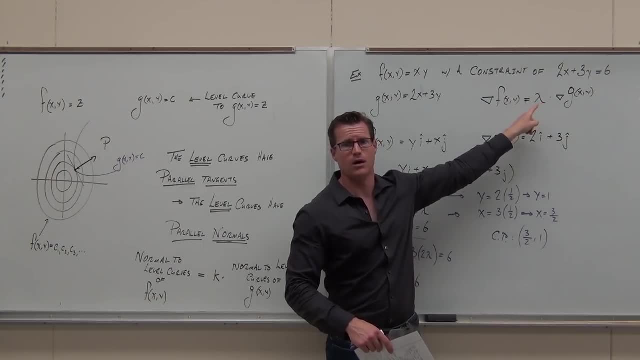 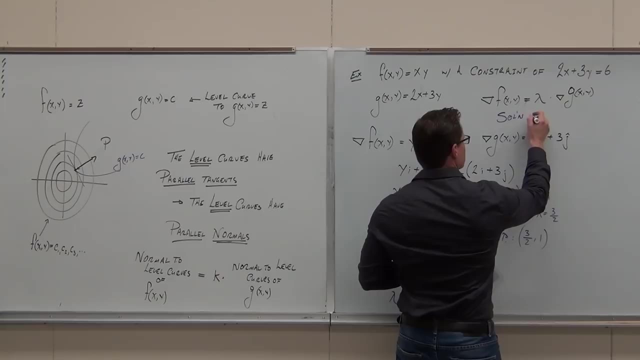 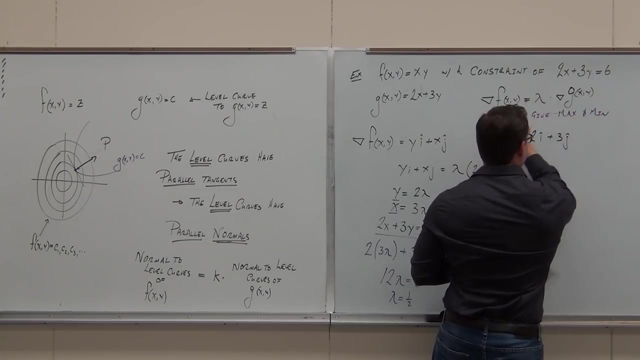 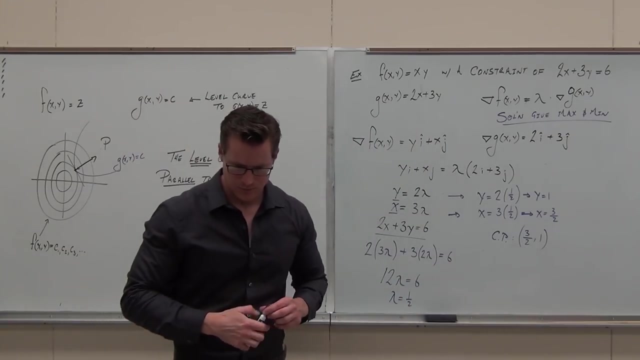 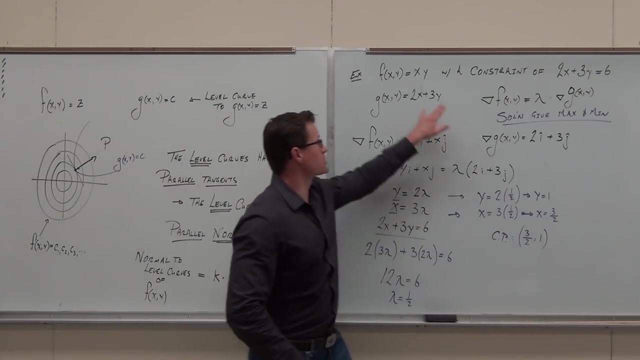 Did you write that down? Write that down. Maxima and minima will be found at solutions to this. Okay, So this is going to be the actual. This is going to be the actual maximum. you take this value just like anything else, plug it in. so what is the? 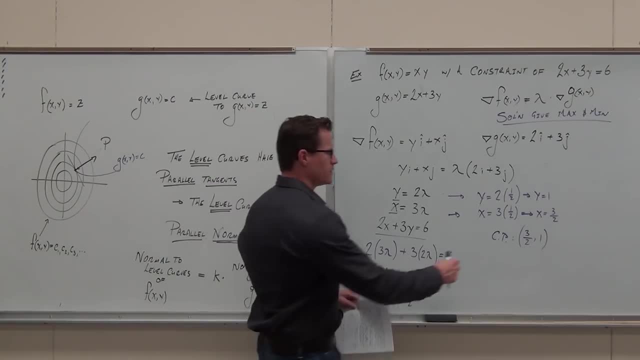 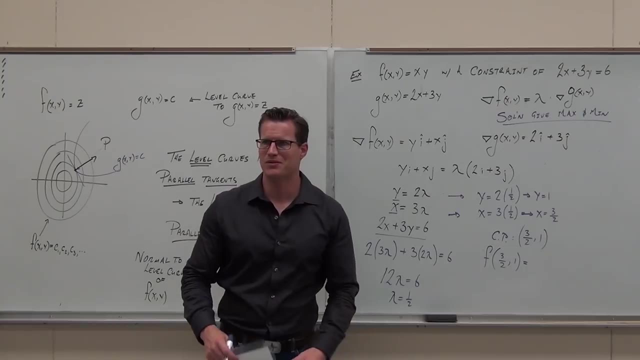 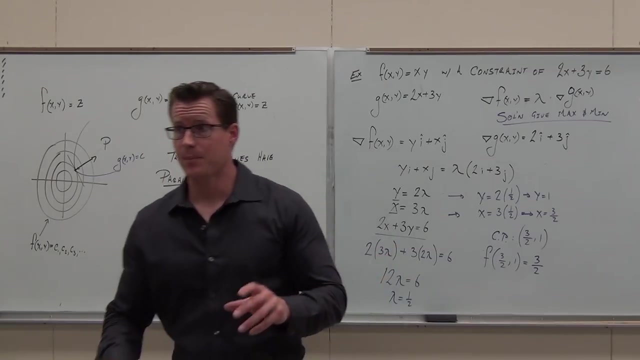 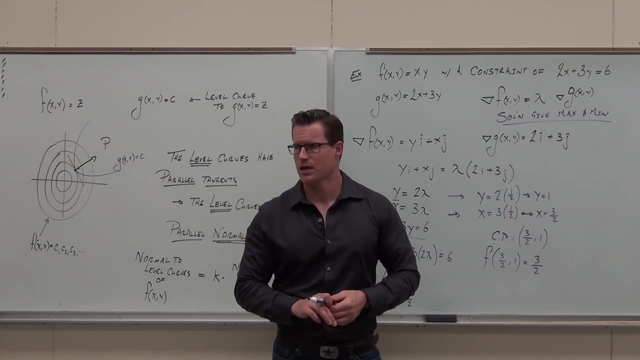 what is the the value when we plug in this? well, that's pretty easy. one, three half times one is three halves. now what is it? I said maximum and minimum happen at that point. but is that a maximum or a minimum? that takes a little bit more work sometimes. if you have two points, it's easier because you can tell one's. 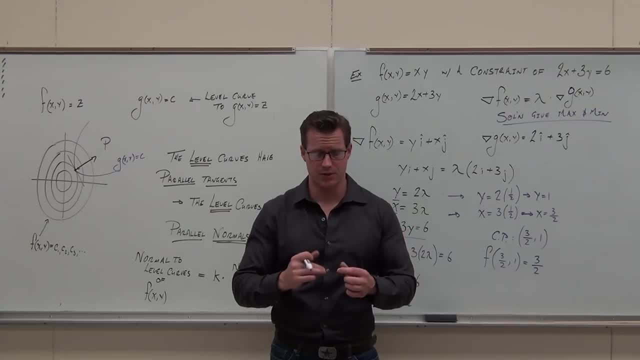 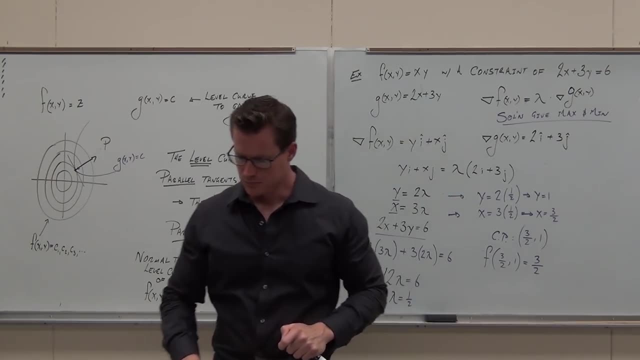 the highest ones, the lowest. you can tell that if you have only one point. here's what's happening. this is either the bottom, a minimum, and everything's climbing higher, or this is top and everything's climbing lower. this particular one is a max, this is a maximum. how I can tell that? I would have 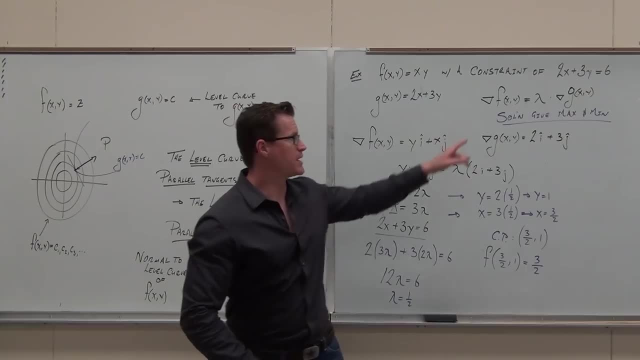 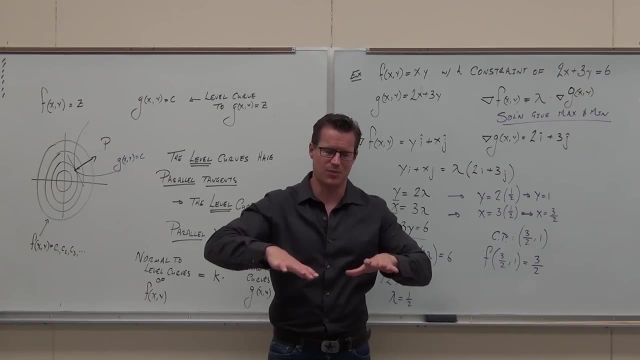 to do the second derivative test. that gives a saddle point and, based on the constraint, what's happening here is for this function, the, the. the saddle point gives this basically some hyperbolic here, where they're going one way along the x-direction below and one way along. 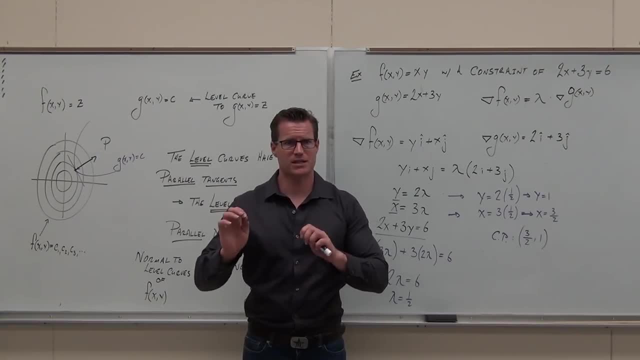 So I know that what these points give us are either maximums or minimums of this function In this case. did you catch that? You might want to write that one down. No, not constraint. These are absolute with the constraint, So maxima and minima will be found at solutions to this. 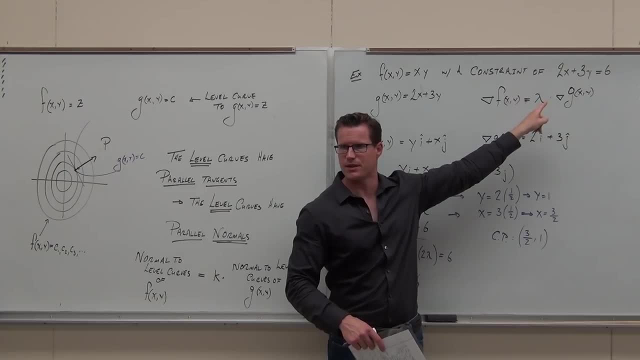 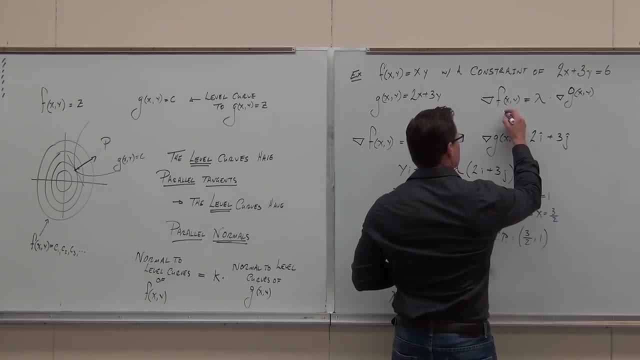 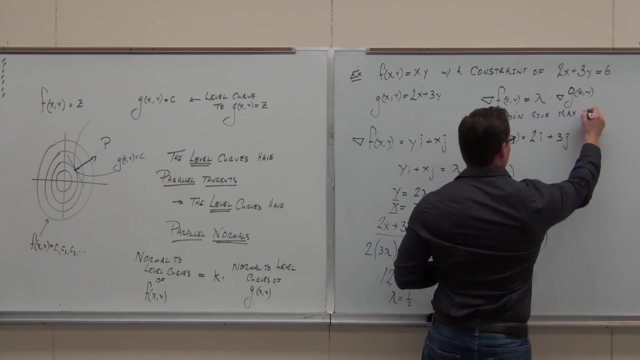 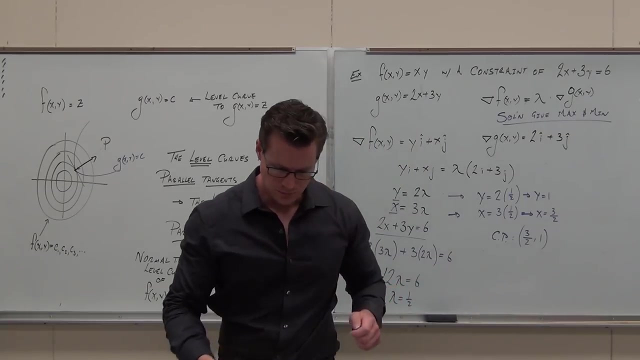 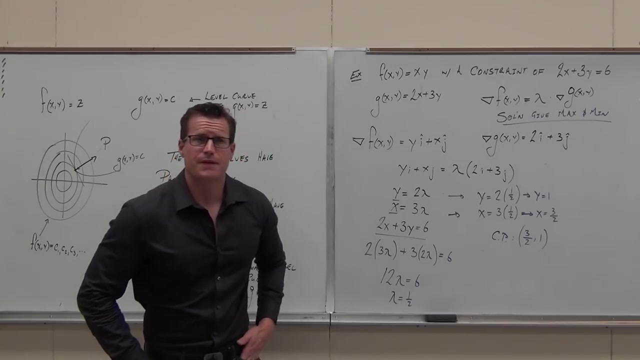 Maxima and minima will be found at solutions to this. Did you write that down? No, Write that down. Maxima and minima will be found at solutions to this. To find the actual maximum, you take this value Just like anything else, plug it in. 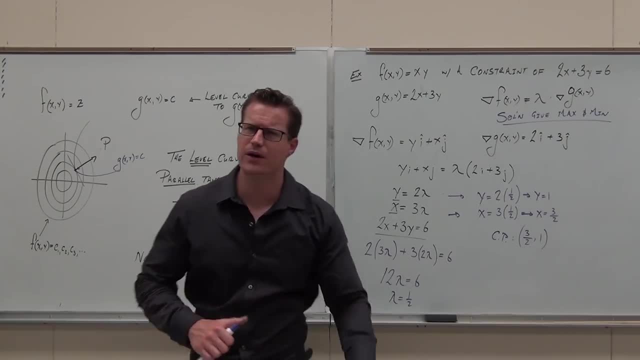 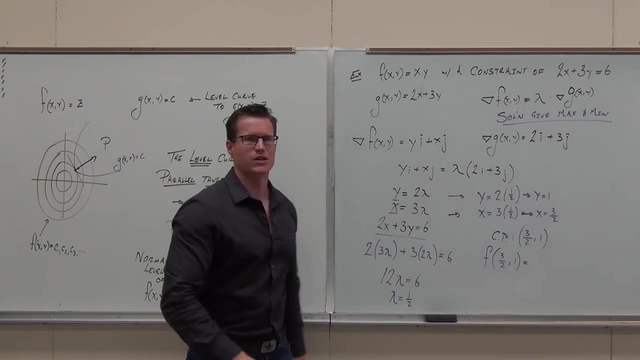 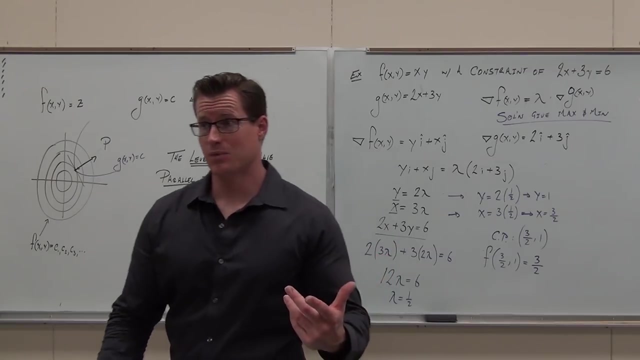 So what is the value when we plug in this? Well, that's a pretty easy one: Three halves times one is three halves. Now what is it? I said maxima and minima happen at that point, but is that a maximum or a minimum? 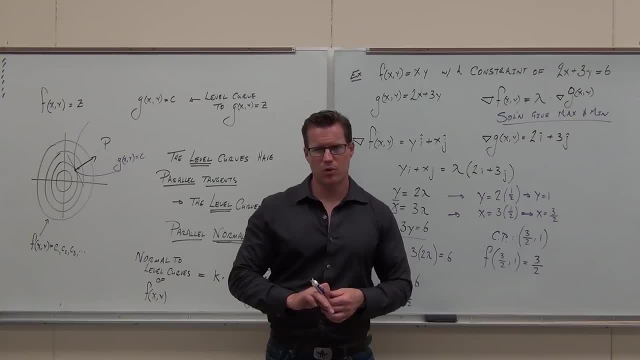 That takes a little bit more work. sometimes If you have two points it's easier Because you can tell one's the highest, one's the lowest. You can tell that If you have only one point. here's what's happening. 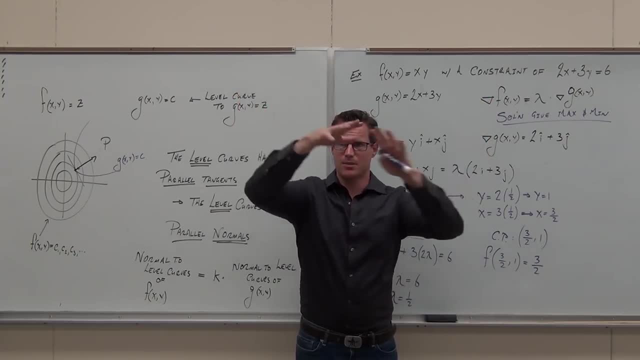 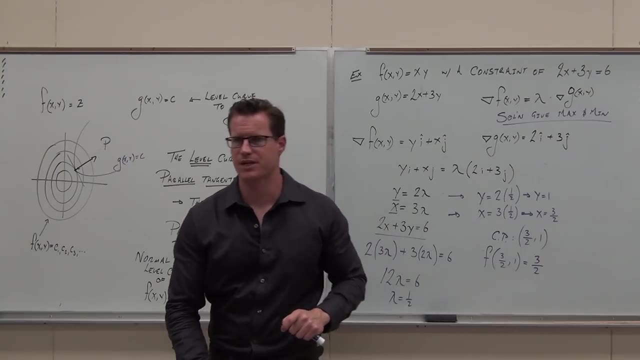 This is either the bottom, a minimum, and everything's climbing higher, or there's a top and everything's climbing lower. This particular one is a max. It's a maximum. How I can tell that I would have to do the second derivative test. 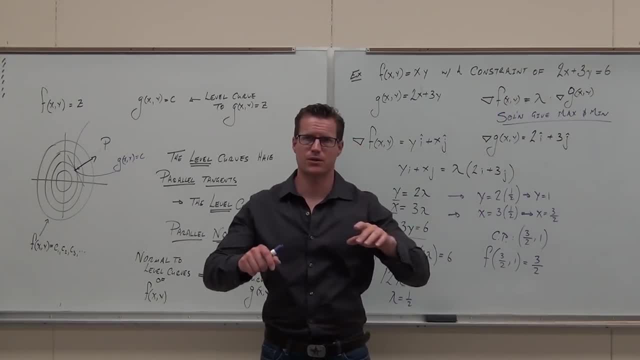 That gives a saddle point And, based on the constraint, what's happening here is for this function. the saddle point gives this basically some hyperbolas here, where they're going one way along the x-direction, One way along the y-direction below and one way along the y-direction above. 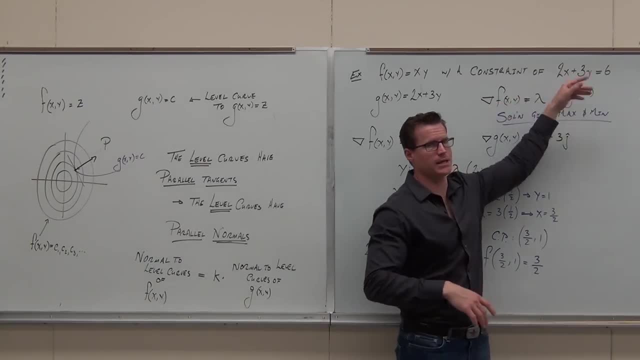 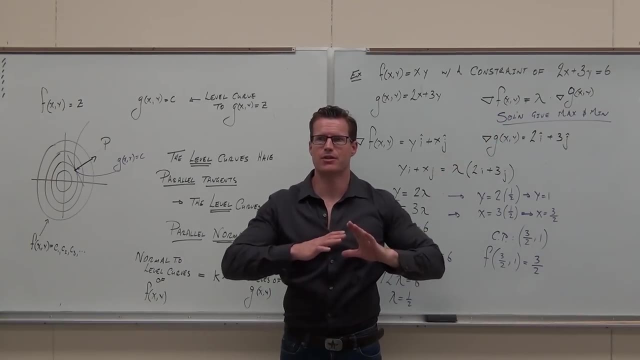 the y-direction above and where that plane intersects that. you see that that's a. that's a plane going up. where that plane intersects those, it's in one region that everything is climbing higher. those, that saddle point is climbing higher. you'd need a second derivative test to tell it, but that. 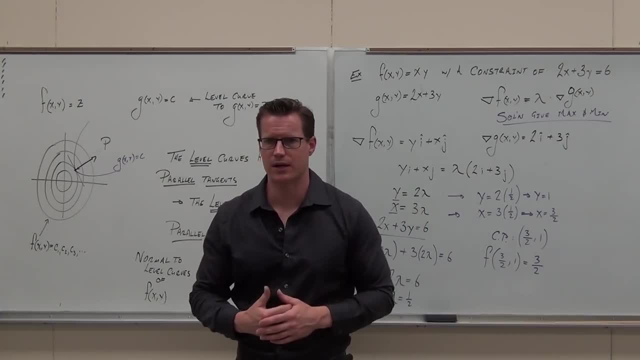 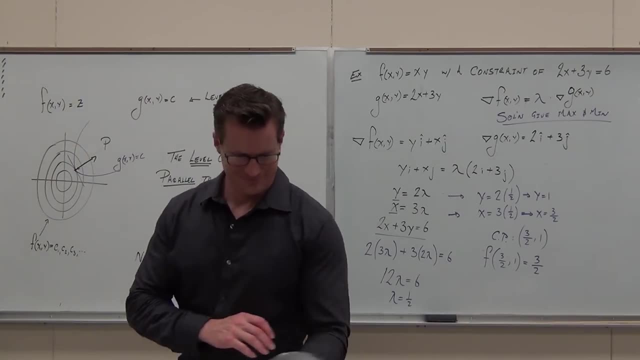 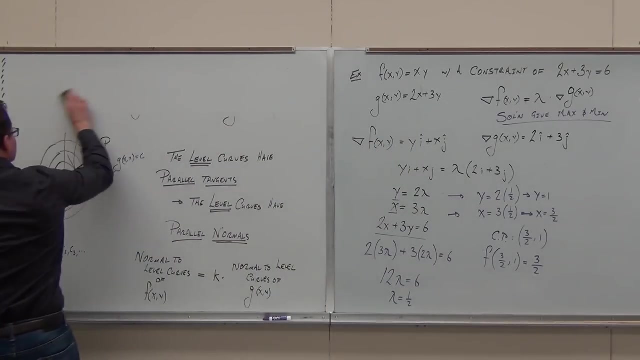 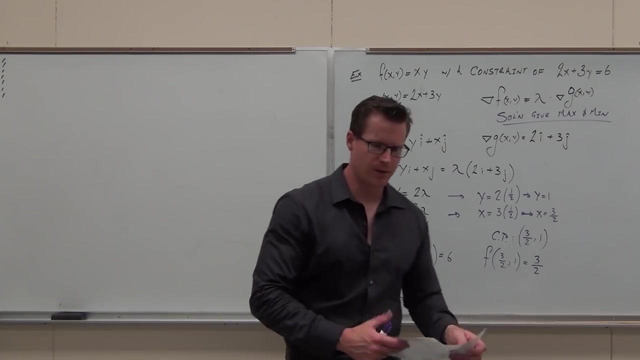 right, there is a maximum value. I think. I'm not going to go into it right now for the sake of time, but that's a max. I want to show you two other ones, one of the one we're going to do. I'm going to skip over. we have an easy, for this was the easy. 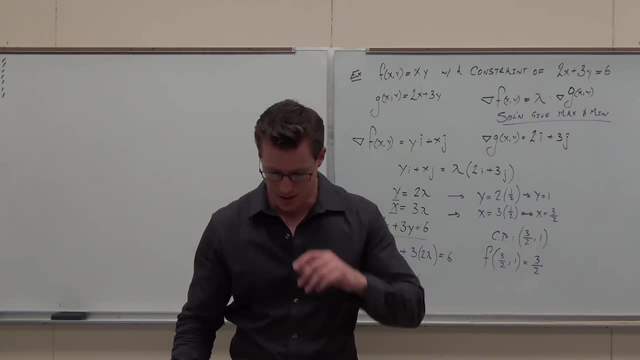 example, we have a really hard one, which I'm going to hold for next time because it takes a little while to explain it, and then I'm going to show you how to do some three variables. so I'm going to do the three variable version. first it's: 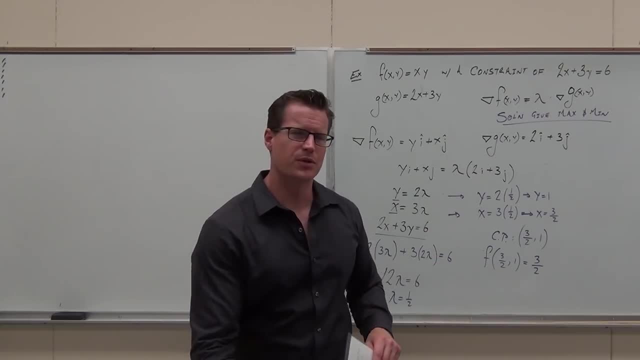 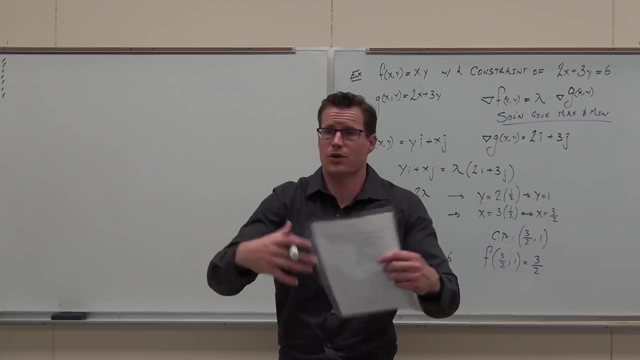 not any harder than this. I just want to show you you can do it. that's one of the beauties about the Lagrange multiplier. the constraint, optimization, is that this stuff- it doesn't matter that you can eliminate a variable. it works with all of this because gradients are easy to find in three variables. so I'm going to. 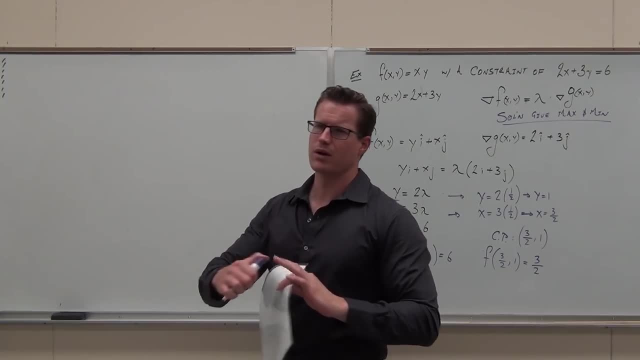 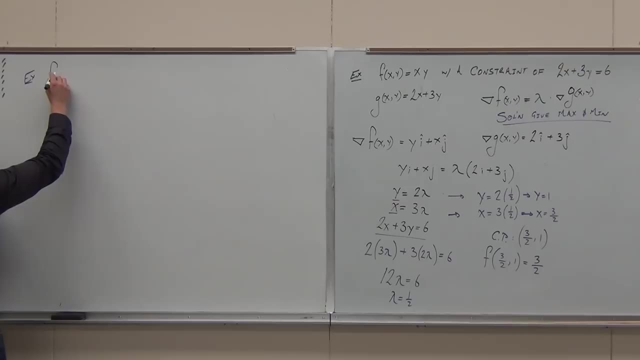 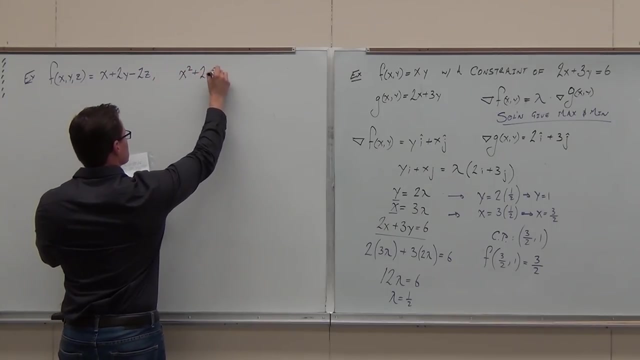 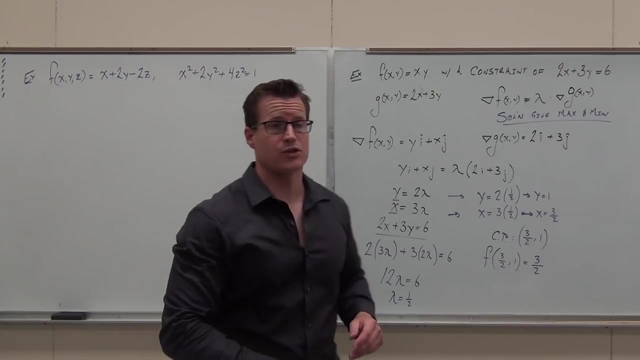 show you that one and then we're going to call it good for now and I'll come back and do one more of these examples next time to really fill it out. okay, so we're going to try to optimize this function with this constraint verified. this is a lot like a surface of 4d. yeah, 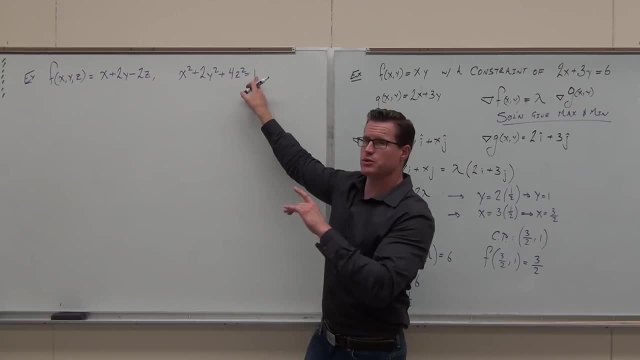 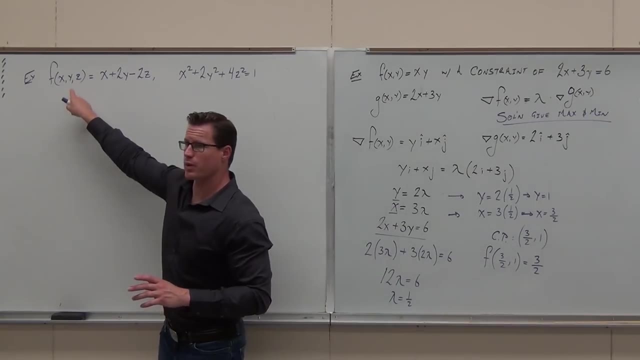 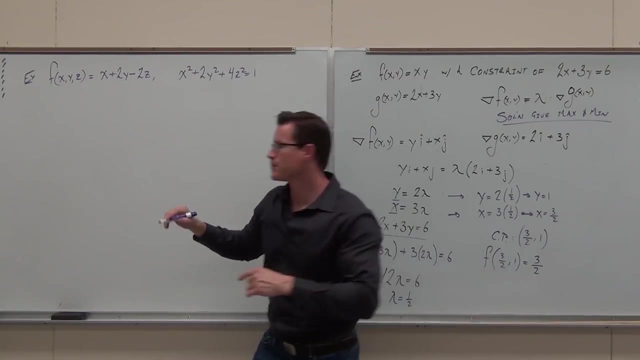 it's crazy. this is a constraint, that's three variables equal to a constant. this is a level surface of some higher function. so what I want to do right now, here's the process: keep this function the way it is. make a function for this such that this is a level surface of some higher function. let's do that now. 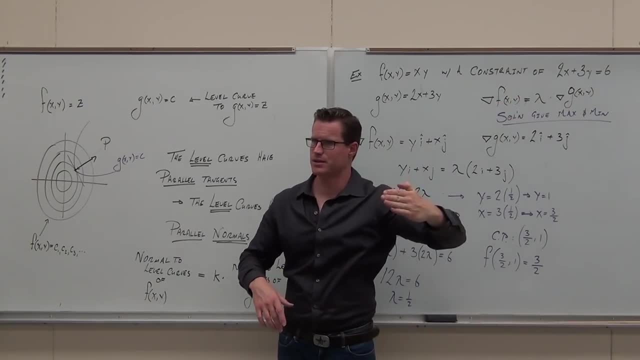 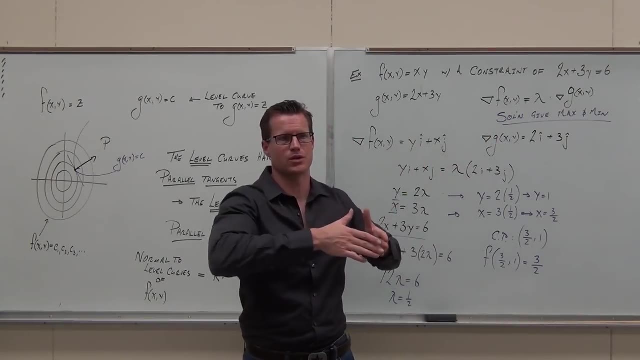 And where that plane intersects that. you see that that's a plane going upward. Where that plane intersects those, it's in one region that everything is climbing higher. That saddle point is climbing higher. You'd need a second derivative test to tell it. but that right, there is a maximum value. 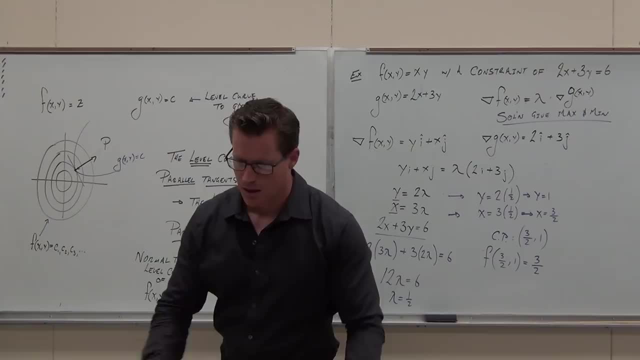 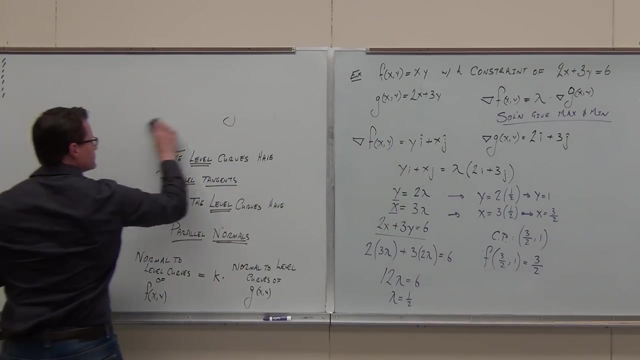 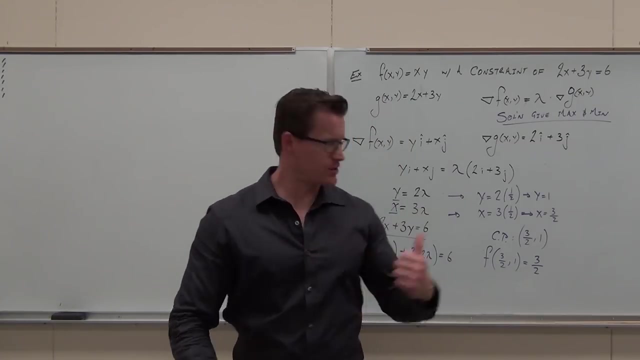 I'm not going to go into it right now for the sake of time, but that's a max. I want to show you two other ones. One other one. What I'm going to do, I'm going to skip over. We have an easy. this was the easy example. 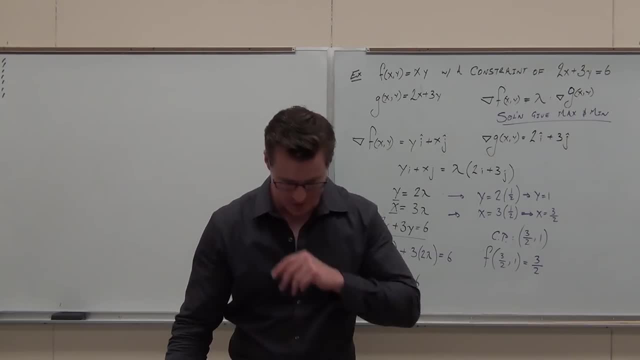 We have a really hard one, which I'm going to hold for next time because it takes a little while to explain it, And then I'm going to show you how to do it. So I'm going to show you how to do it. 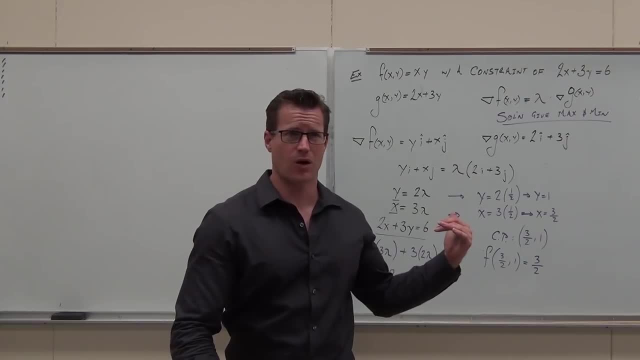 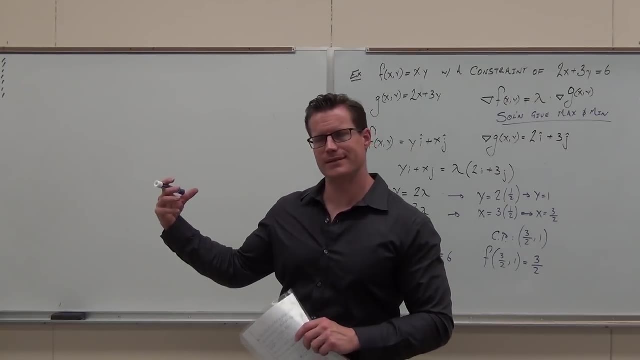 So I'm going to do the three-variable version first. It's not any harder than this. I just want to show you that you can do it. That's one of the beauties about the Lagrange multiplier. the constraint, optimization, is that this stuff. it doesn't matter that you can eliminate a variable. 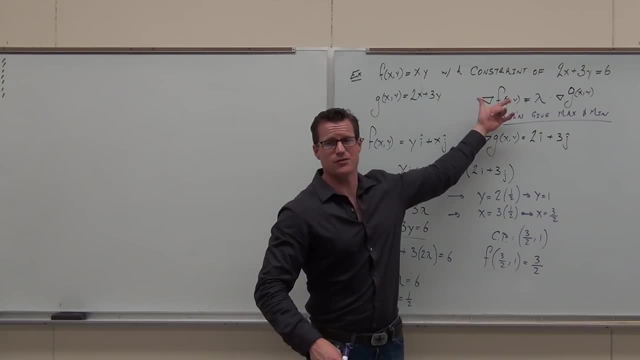 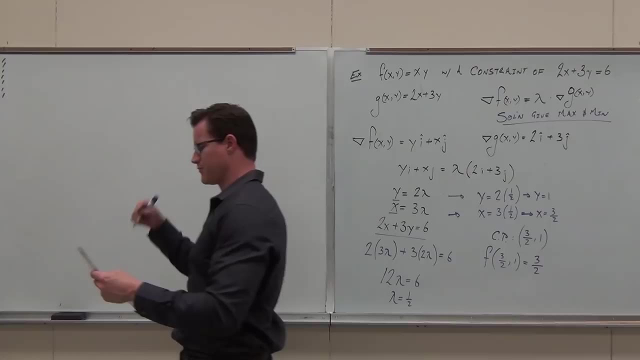 It works with all of this because gradients are easy to find in three variables. So I'm going to show you that one and then we're going to call it good for now And I'll come back and do one more of these examples next time to really fill it out. 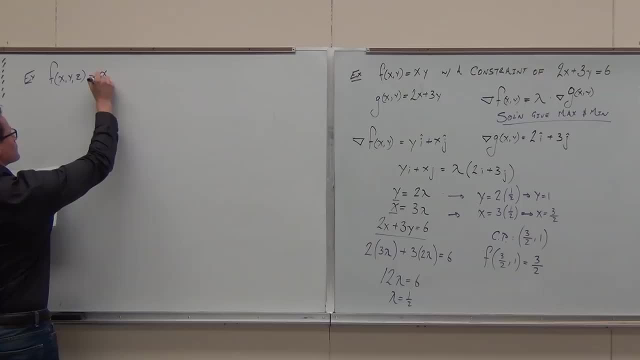 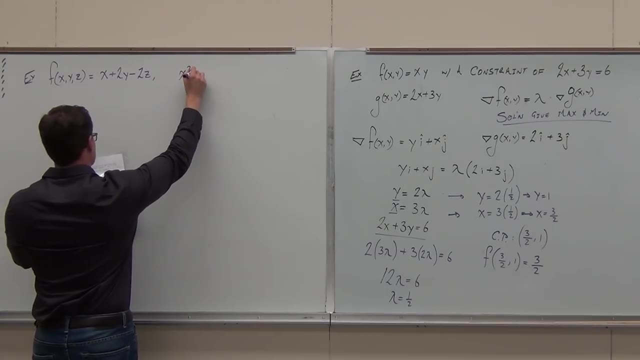 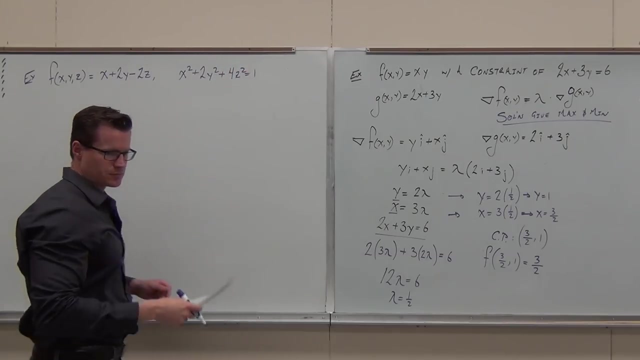 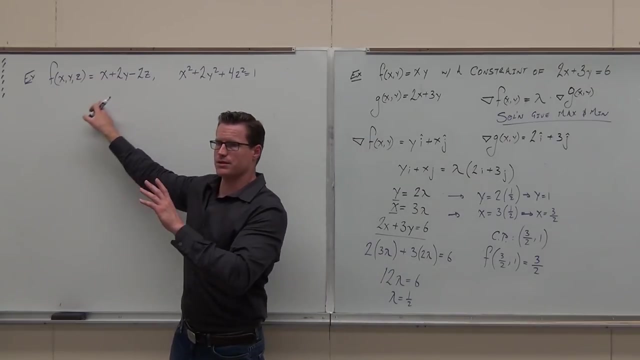 Okay, so we're going to try to optimize this function with this constraint. Verify it. This is a wow. it's like a surface in 4D. yeah, It's crazy. This is a constraint That's three variables. 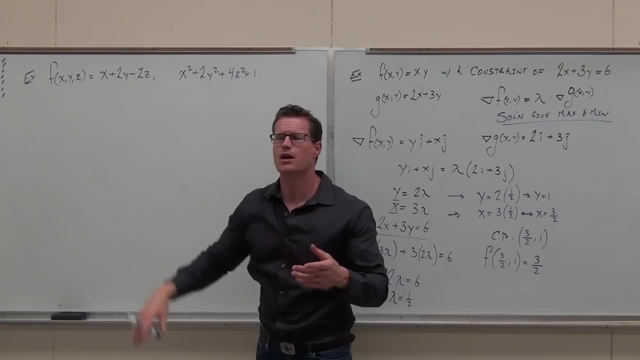 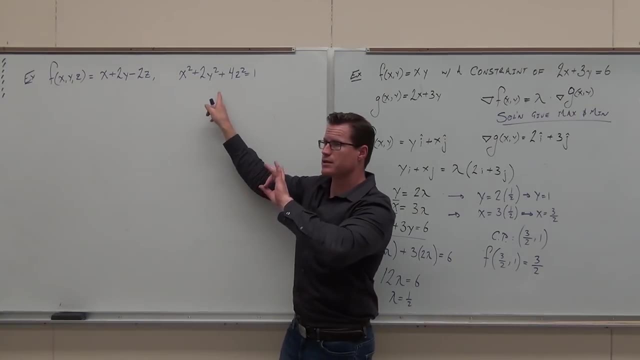 It's equal to a constant. This is a level surface of some higher function. So what I want to do right now, here's the process: Keep this function the way it is, Make a function for this such that this is a level surface of some higher function. 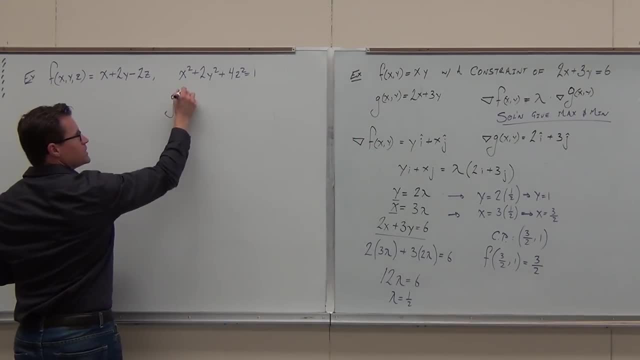 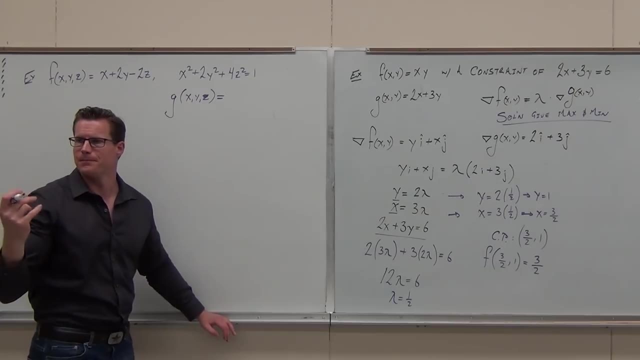 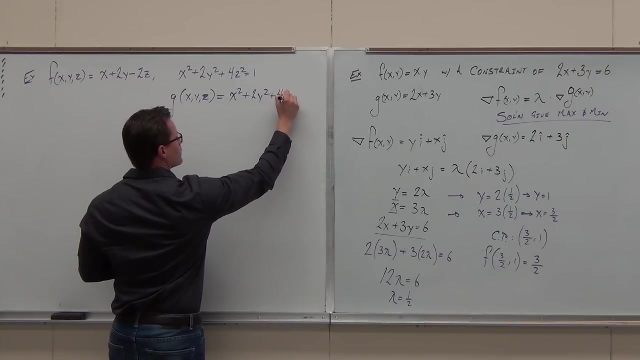 Let's do that now. Call it g. Can you tell me please really quickly what that function's going to be? Come on, Help me, Thank you. Thank you very much, You're welcome. What about the one? Do I need the one? 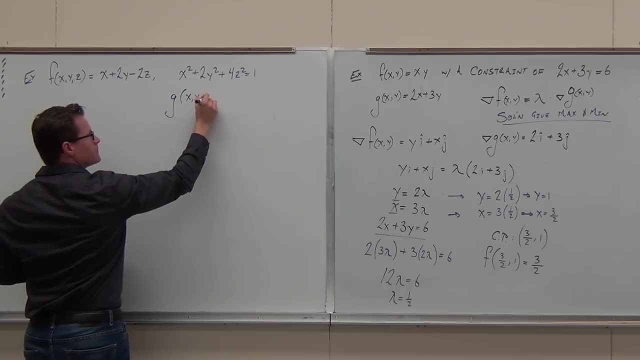 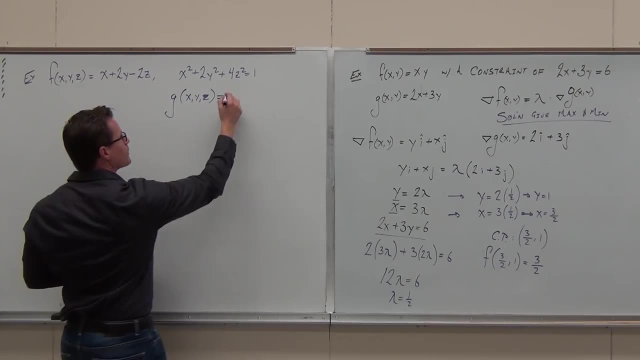 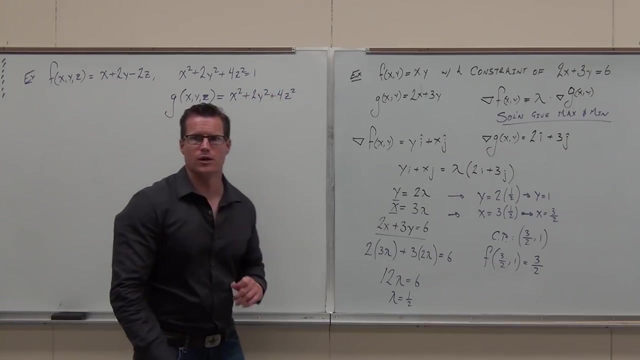 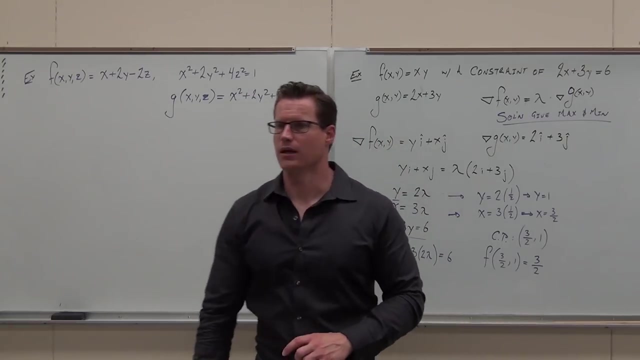 call it G. can you tell me, please really quickly what that function is going to be? come on, what about the one? do any of the one verify that this is a level surface of that piece of junk? okay, cool, now the next thing. whether you get it or not, I 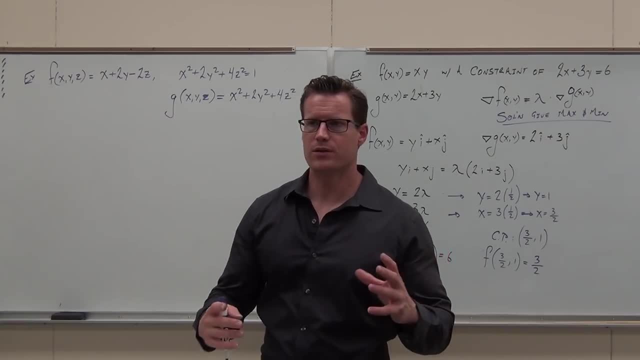 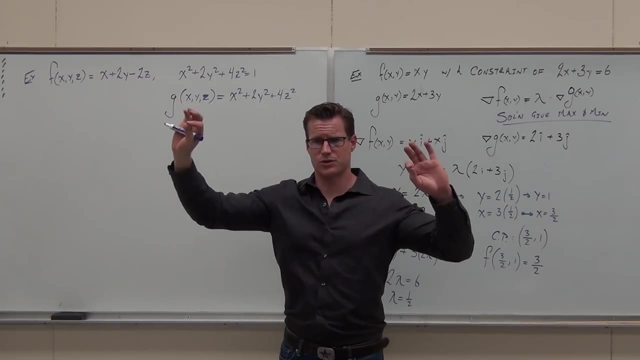 want you to get us. why spend hours talking about this stuff whether you get it or not? the next part is actually pretty easy: find the gradient for this. find the gradient for this because that is so nervous to level services the case and they have to be scalable, so I'm gonna give about 30 seconds to find me a. 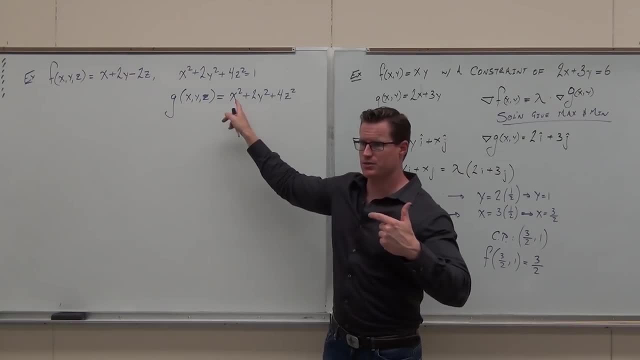 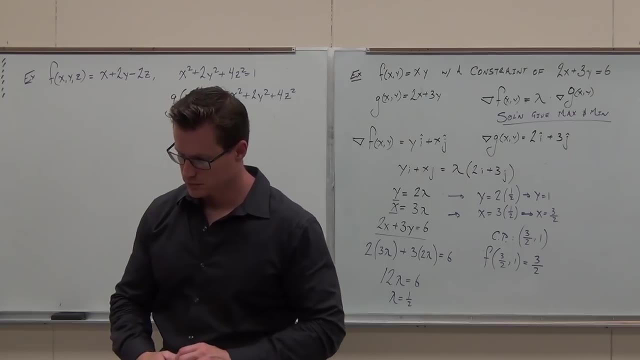 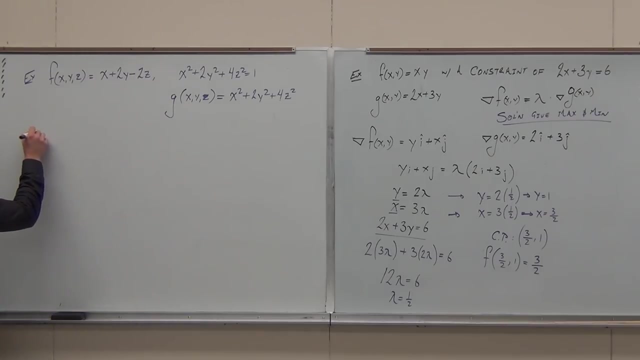 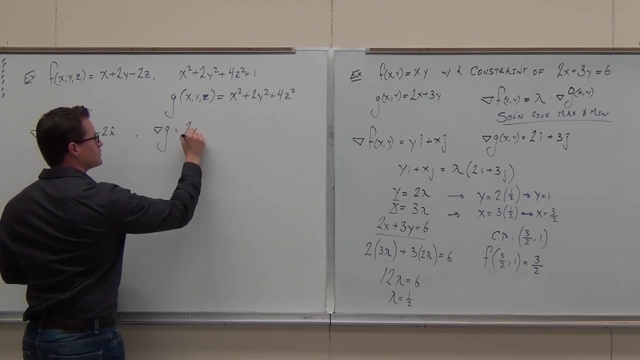 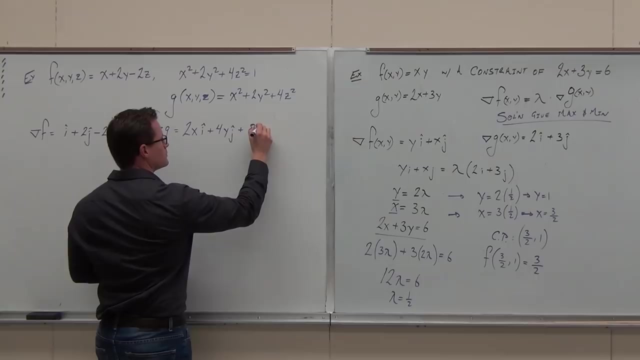 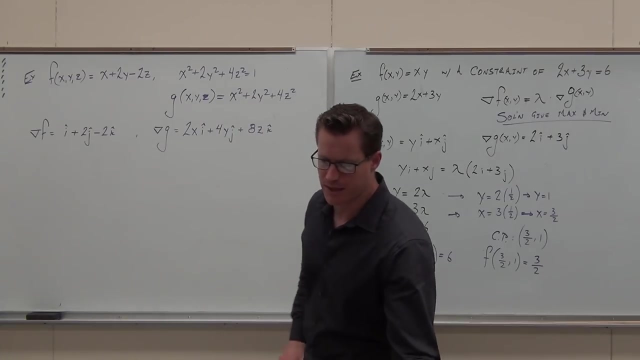 of the gradient is going to have x, y, z i j k. Find me the gradient x, y, z i j k. Set them equal by a scalar multiple called lambda or Lagrange multiplier. Let's double check our gradients here. 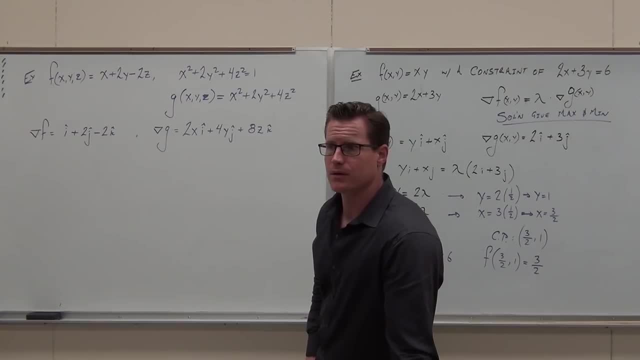 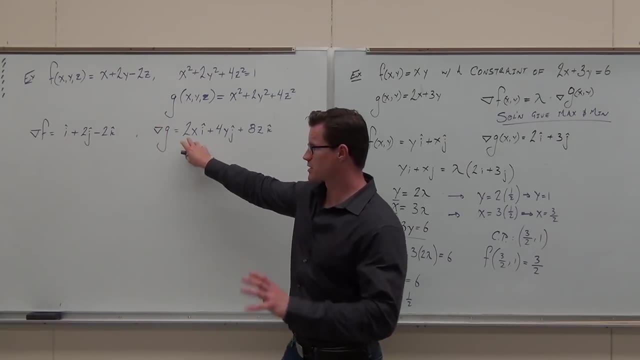 Did you guys get the same gradients that I got? Yeah or no? Yes, yes, no, no, Okay. So if you want to do a shortcut, cut right now and just go x coordinate, lambda x component, that's fine. You really need to build it out and go. well, you know what? 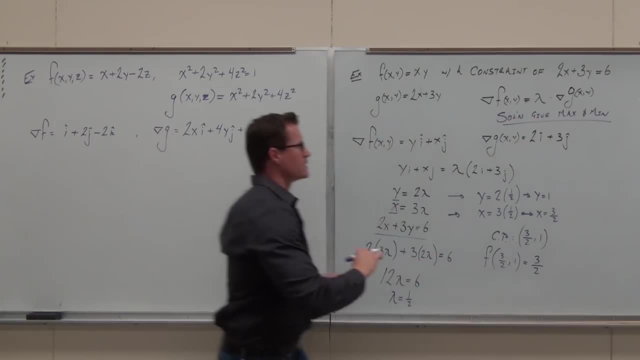 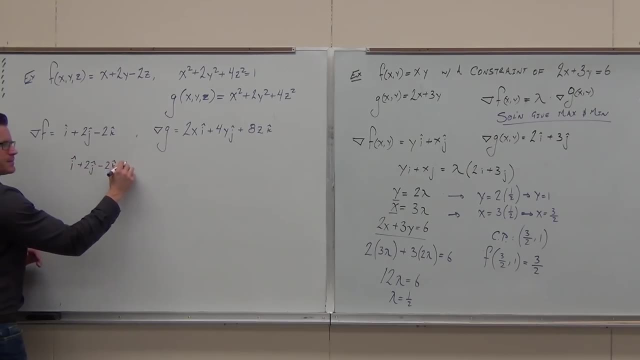 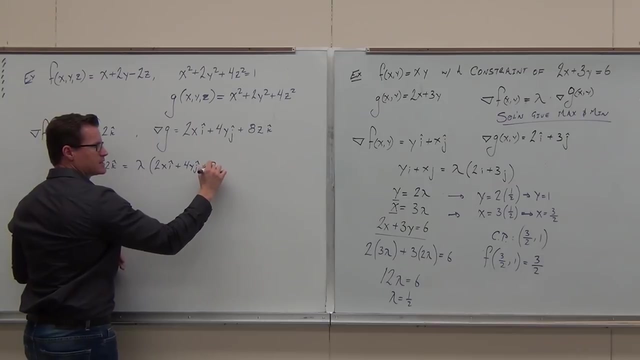 I know that the gradient is equal to lambda times the other gradient. that's fine too. So we have: i plus 2j minus 2k is equal to lambda times 2xi plus 4yj plus 8zk. If you want to build it out like that, that's absolutely fine. 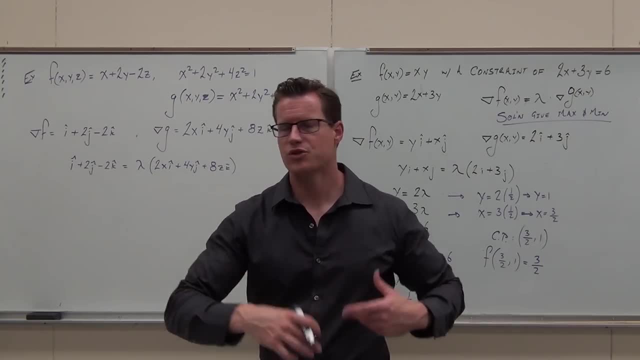 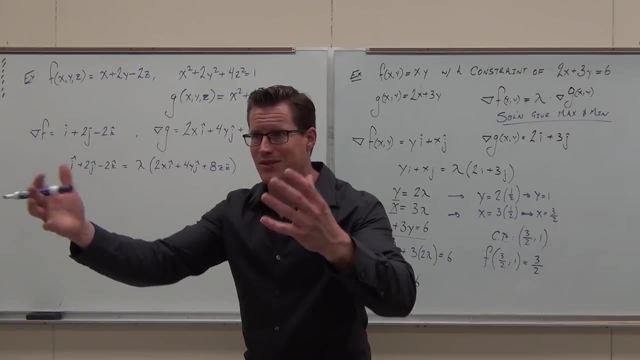 The key point here is: match up your x components, your y components and your z components and get your series of equations. You need to do that, So I want to go really quickly. Come on, I know you're losing focus here. Let me have your focus. 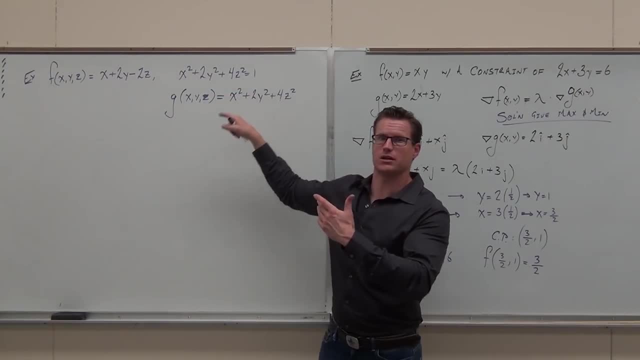 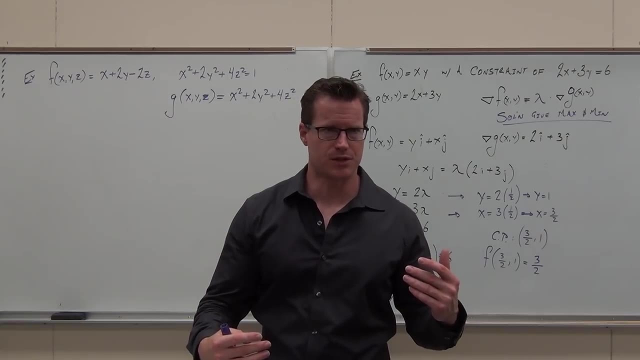 No, Verify that. this is a level surface of that piece of junk. Yeah, Okay, cool. Now the next thing. whether you get it or not, I want you to get it. That's why I spend hours talking about this stuff. 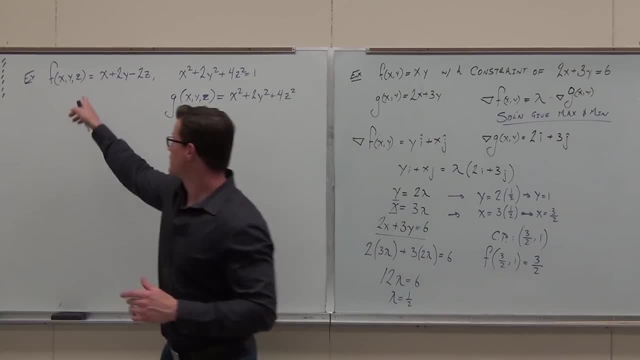 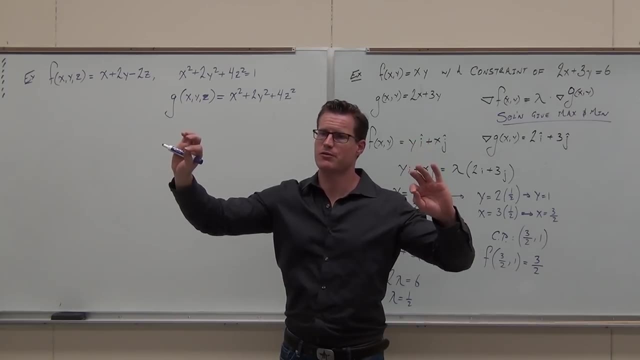 Whether you get it or not, the next part's actually pretty easy. Find the gradient for this. Find the gradient for this, because that gives us our normals Do level surfaces in this case, And they have to be scalar multiples. So I'm going to give you about 30 seconds. 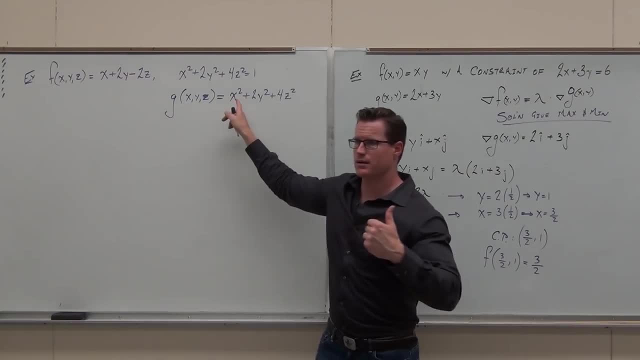 Find me the gradient It's got to have x, y, z, i j k. Find me the gradient. x, y, z i j k. Set them equal by a scalar multiple called lambda or Lagrange multiplier. 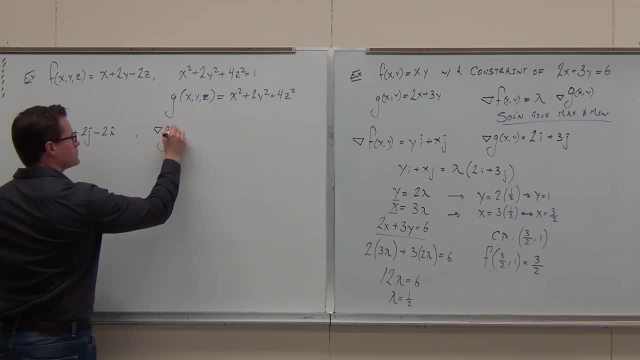 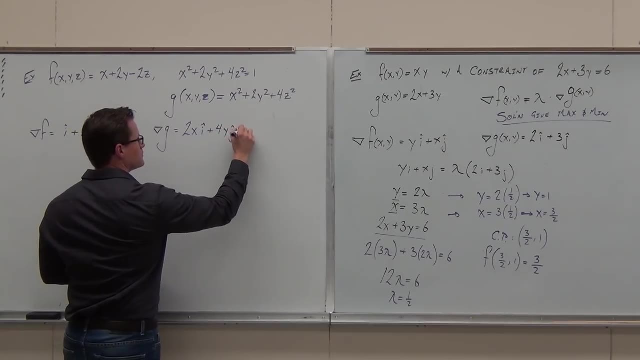 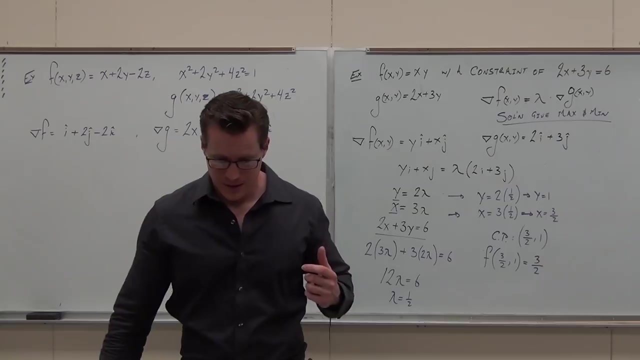 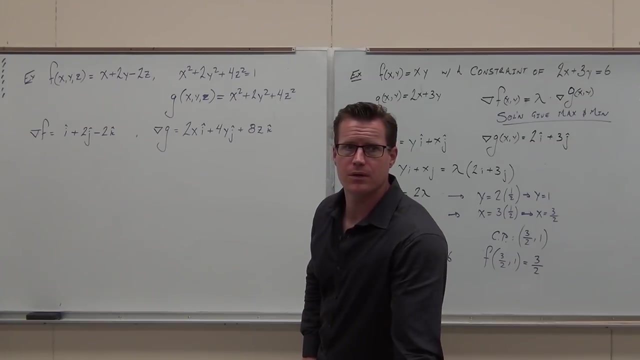 Let's double check our gradients here. Did you guys get the same gradients that I got, Yeah or no? Yes, yes, no, no. Okay. so if you want to do a shortcut right now and just go, x, coordinate lambda x. 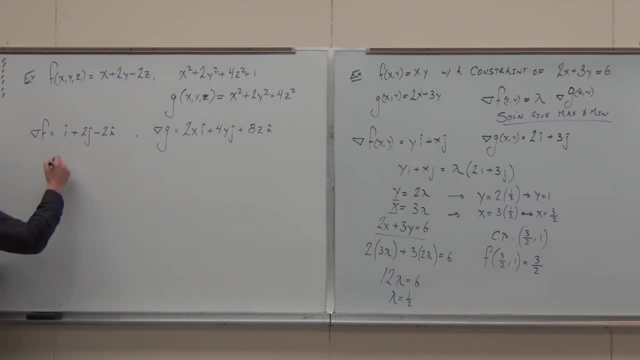 or x component. that's fine. You really need to build it out and go. well, you know what? I know that the gradient is equal to lambda times the other gradient. That's fine too. So we have: i plus 2j minus 2k is equal to lambda times 2xi plus 4yj plus 8zk. 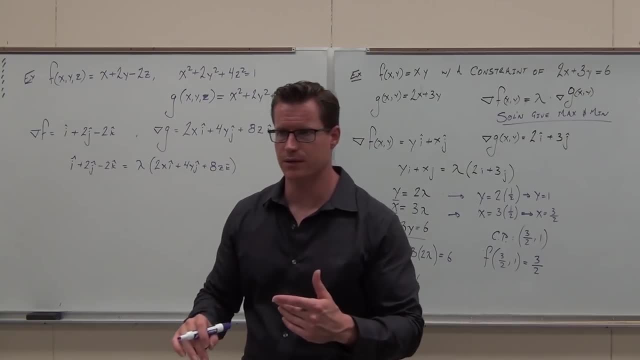 If you want to build it out like that, that's absolutely fine. The key point here is match up your x components, your y components and your z components and get your series of equations. You need to do that, So I want to go really quickly. 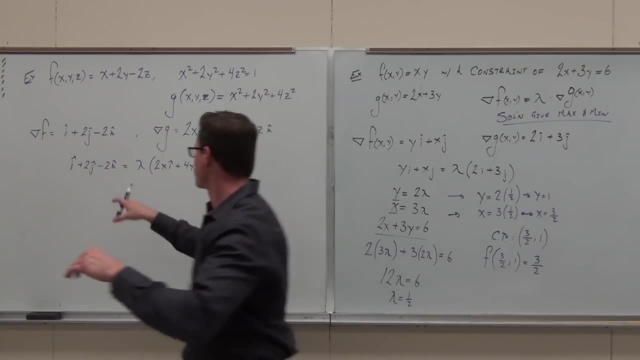 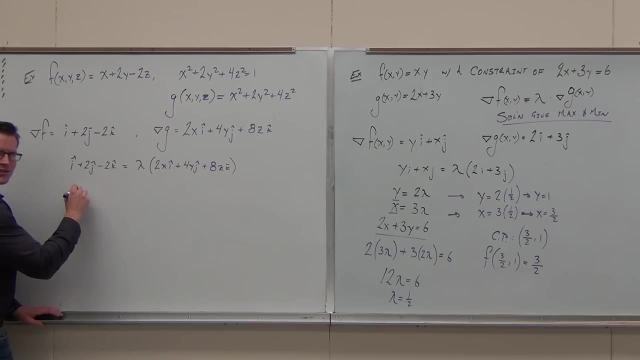 Come on, I know you're losing focus here. Let me have your focus. Can you tell me what the first equation is going to be, please? I didn't hear a word. you said honestly: 2x lambda, equal to what? 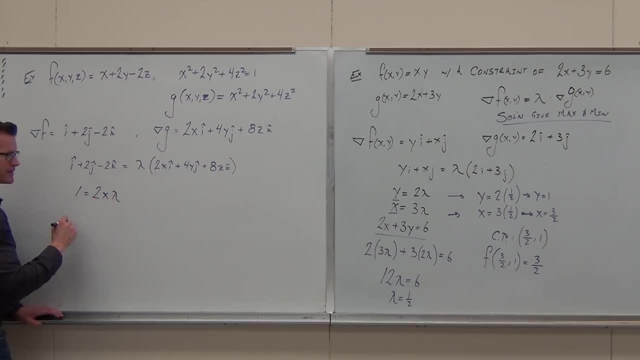 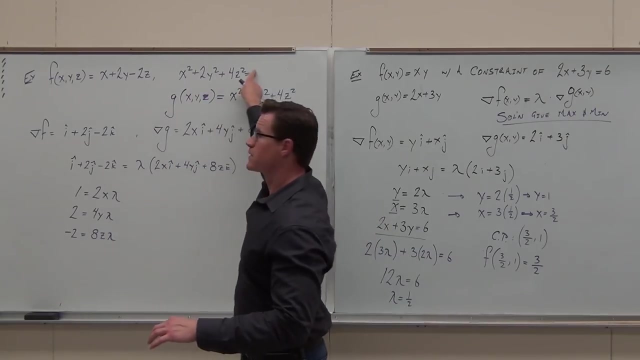 2, what x? Okay, fantastic, Someone else. Come on Quickly. What's the next one? 2. Perfect And lastly, 2. Yeah, fantastic, Now the last one. I want. I want you to write out the constraint. 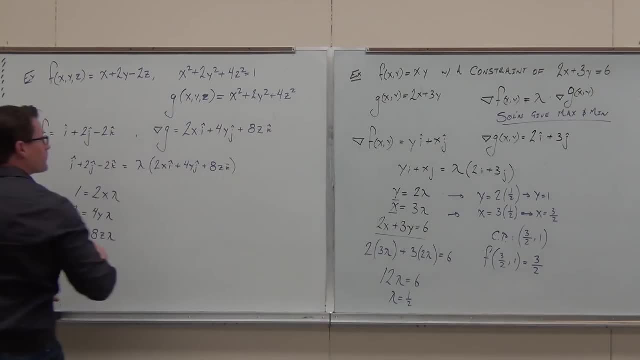 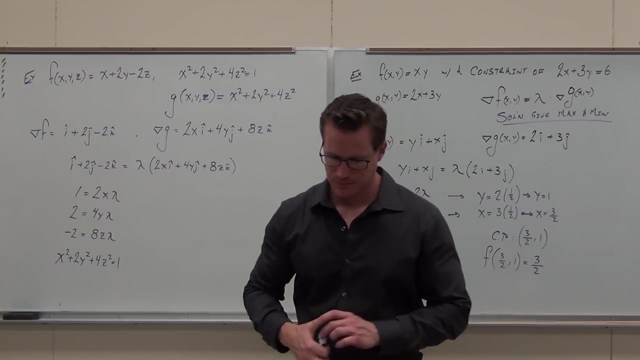 Whatever the constraint is, that's your last equation. That's an important one. You've got to satisfy that. If you're not going to solve it, you've got to solve it in the second equation. So how about this? How about this? 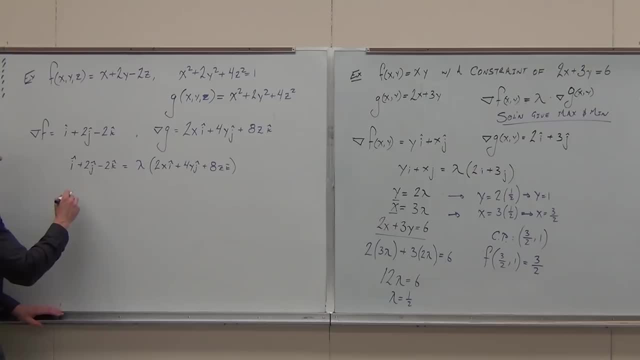 Can you tell me what the first equation is going to be, please? 2x lambda squared. Oh, I didn't hear a word. you said Honestly: 2x lambda equal to what? 2? what x? Okay, fantastic. 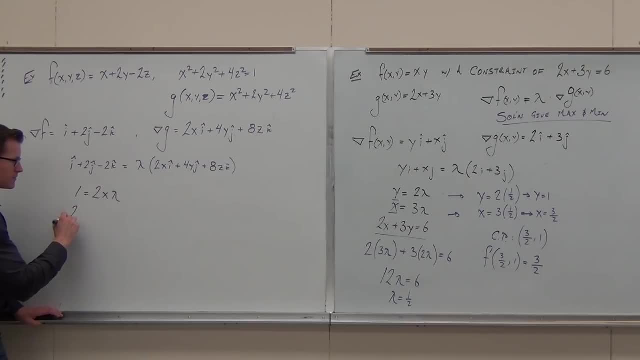 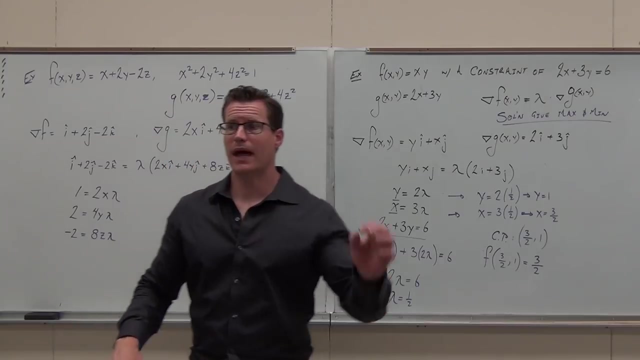 Someone else? come on quickly. What's the next one? 2. Perfect And lastly 2.. Yeah, fantastic. Now the last one I want. I want you to write out the constraint. Whatever the constraint is, that's your last equation. 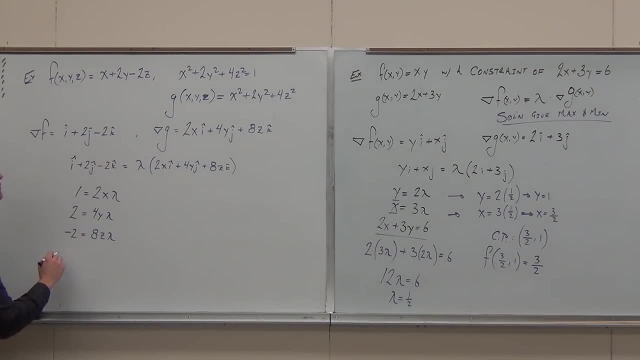 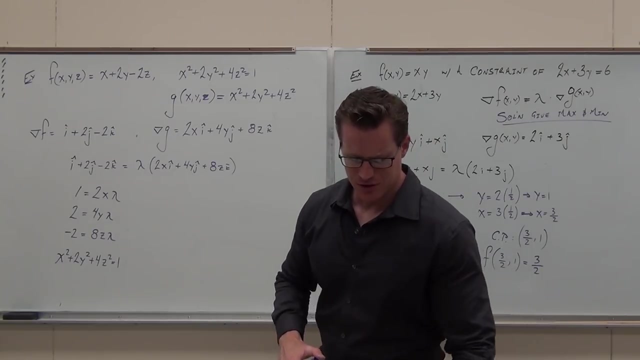 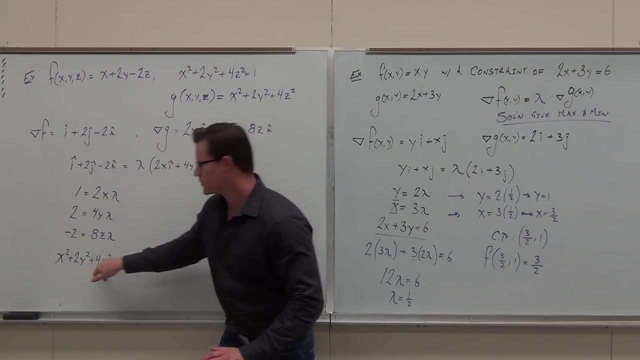 That's an important one. You've got to satisfy that. Okay, let's work on that. It's called the Hey, how about this? Do you guys see a way to take these three equations and use them in this one? Do you guys see a way to do that? 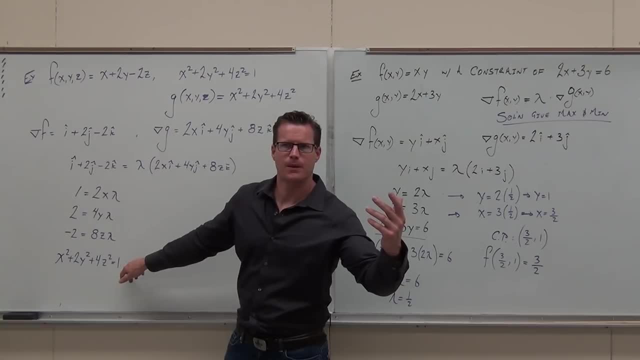 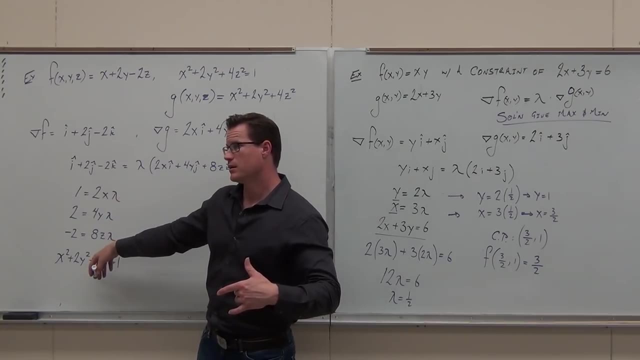 How would you do it? Come on, what would you do? Sulfur, Sulfur, what Mn-option? If I sulfur lambda, I'm not going to have any place to plug it in If I solve for x and y like here. 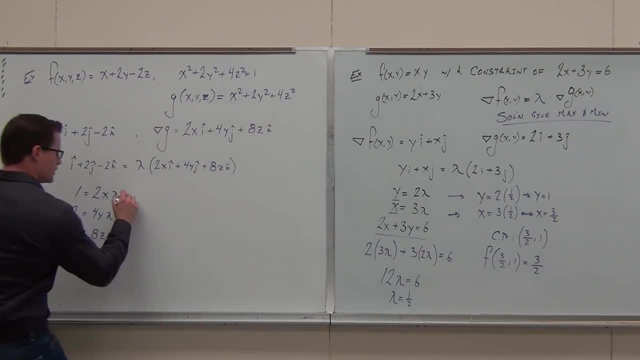 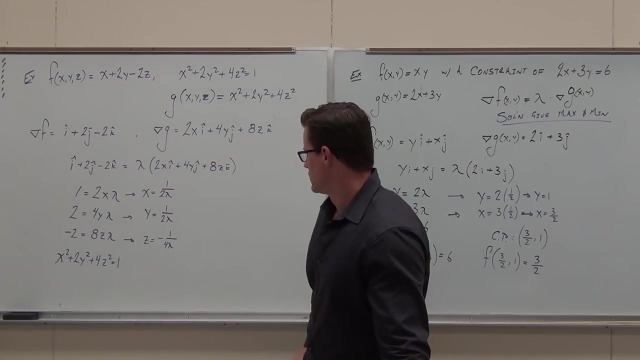 I have some places to plug it in. Let's try that. Can you double-check my work? I get 1 over 2 lambda, 1 over 2 lambda and 1 over negative. 1 fourth lambda. Do you guys get the same thing I got? 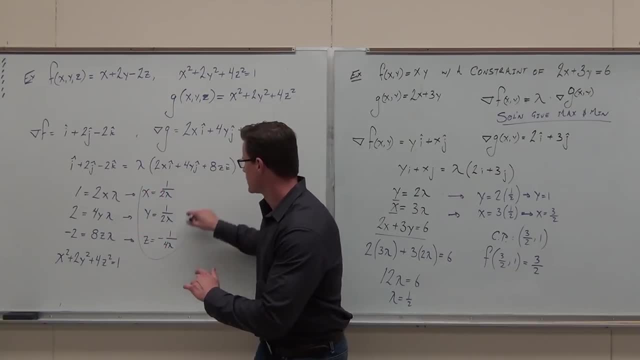 Hey, now that we have these variables and a place to plug them in, do that? Take these variables, substitute what they're equal to into that equation? What you're doing here is you're finding the one value of lambda that's going to create a level curve that has 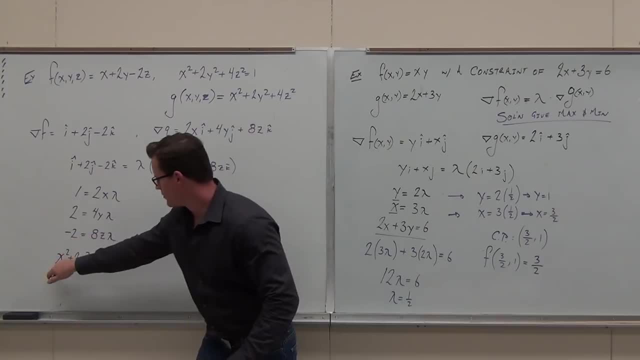 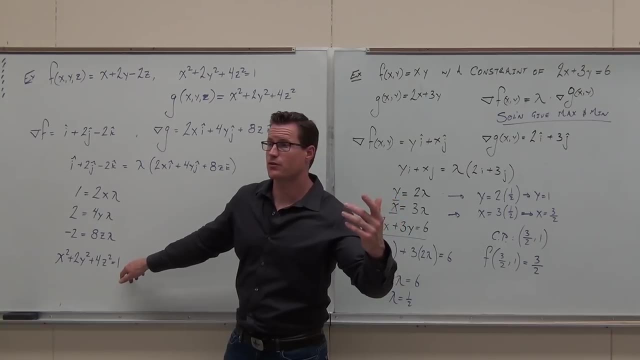 Do you guys see a way to take these three equations and use them in this one? Do you guys see a way to do that? How would you do it? Come on, what would you do? Solve for what? If I solve for lambda, I'm not going to have any place to plug it in. 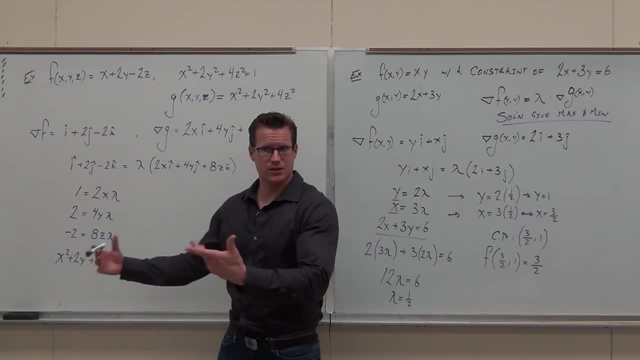 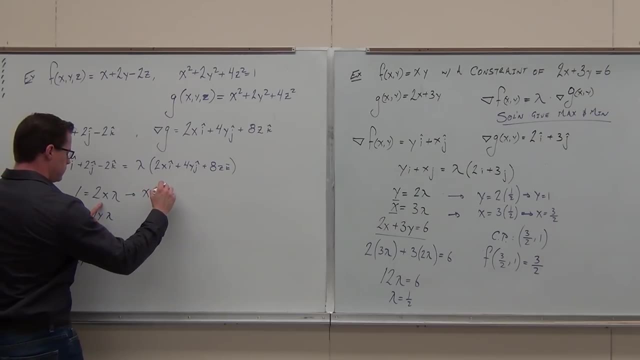 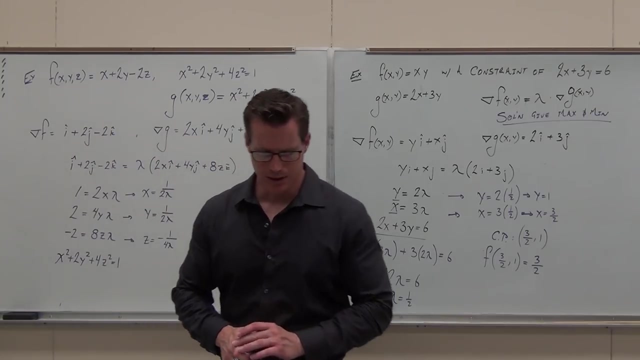 Right for x and y, like here. I have some places to plug it in. Let's try that. Can you double check my work? I get 1 over 2 lambda, 1 over 2 lambda and 1 over negative, 1 fourth lambda. 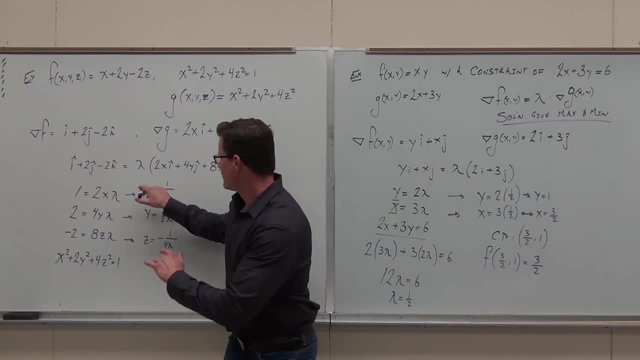 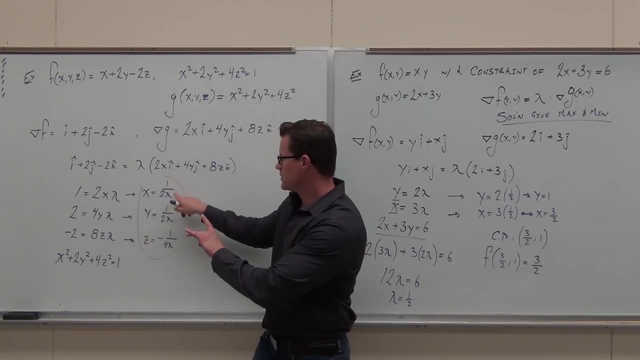 Do you guys get the same thing I got? Hey, now that we have these variables and a place to plug them in, do that: Take these variables, substitute what they're equal to into that equation. What you're doing here is you're finding the one value of lambda. 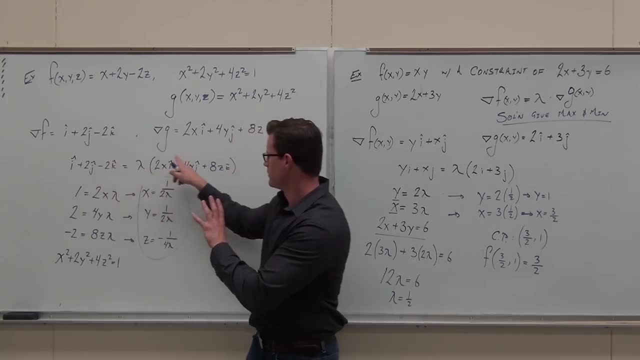 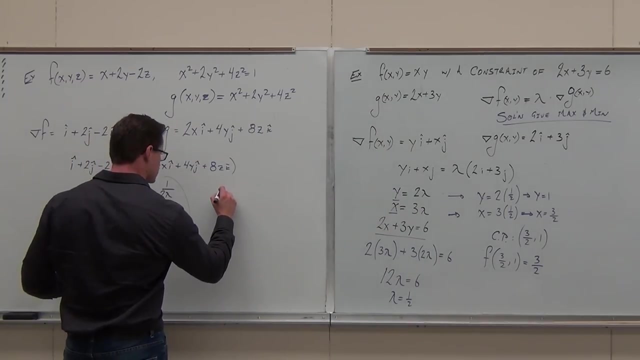 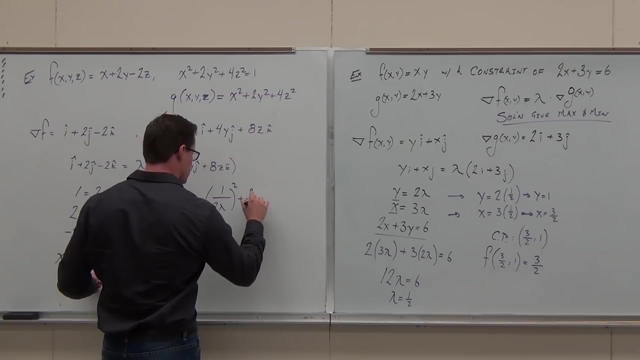 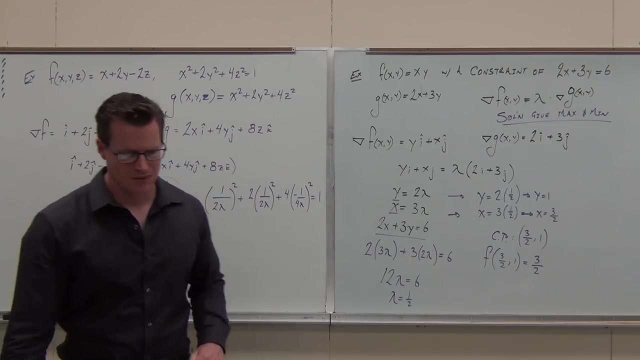 that's going to create a level curve that has well lambda, that creates the same, That's normal for two different level curves and where that point exists, that's the max or min. Well, we can simplify that. We can simplify that. 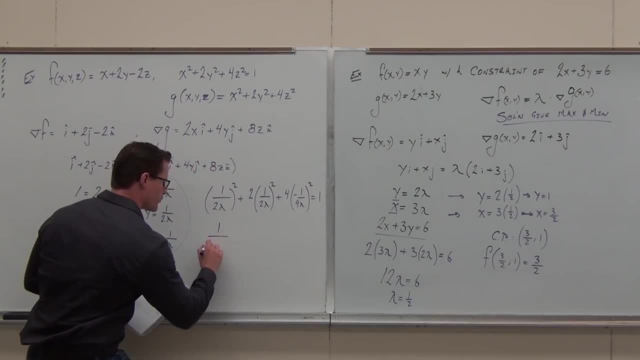 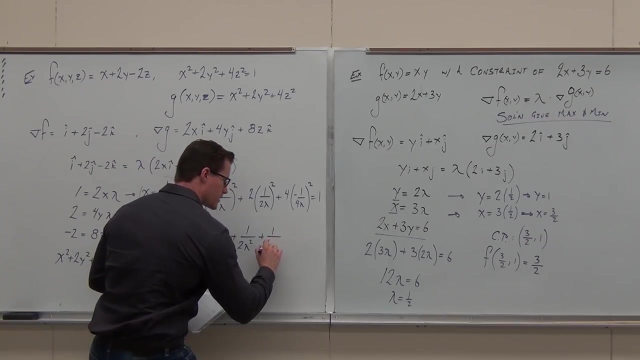 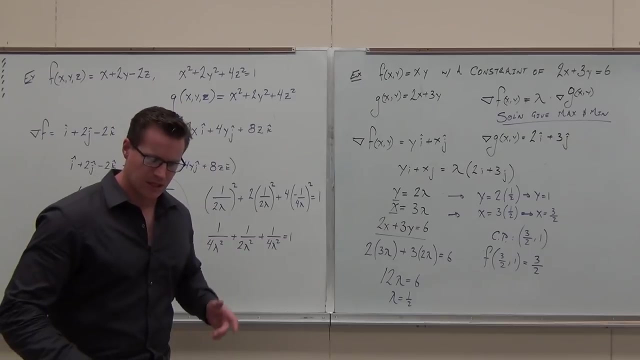 We can simplify it. So if we simplify this, what I got was 1 over 4 lambda squared plus 1 over 2 lambda squared, plus another 1 over 4 lambda squared Head nod if you're okay with that. so far, for real. 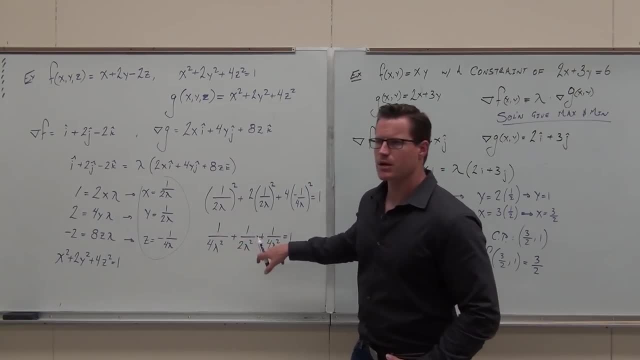 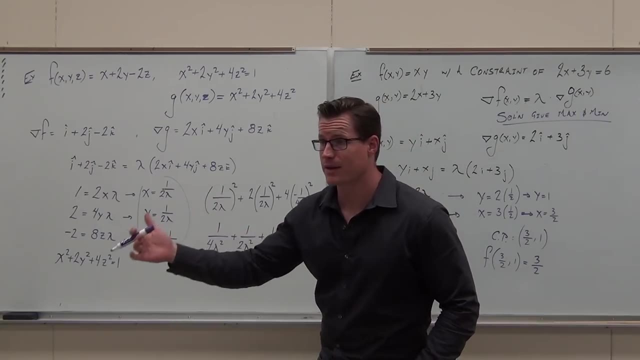 Substitution, Put it in there. Hey, how would you solve that? Come on quick, We've got to move kind of quickly on this. one Common denominator. Okay, sure, Common denominator, whatever. Multiply everything by the LCD. 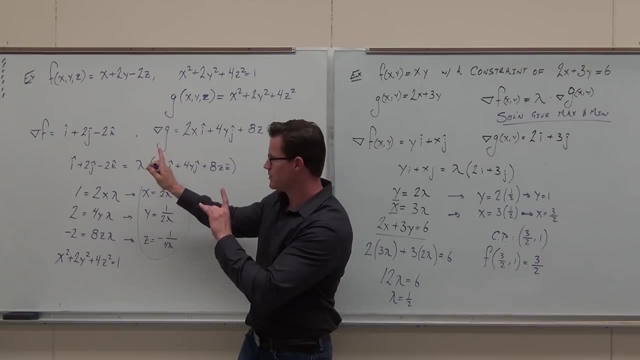 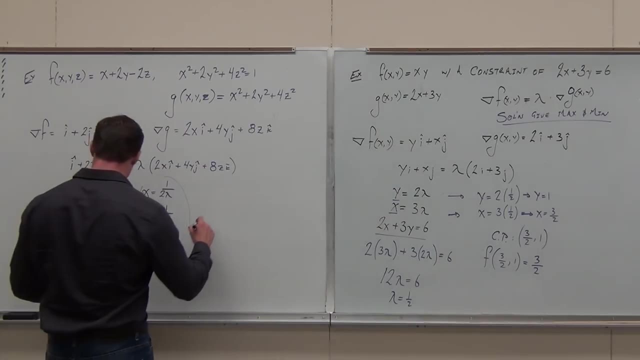 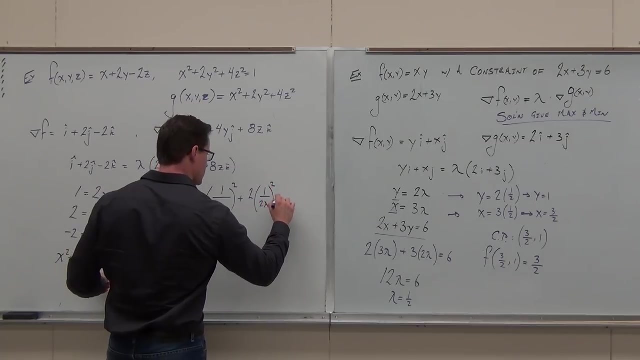 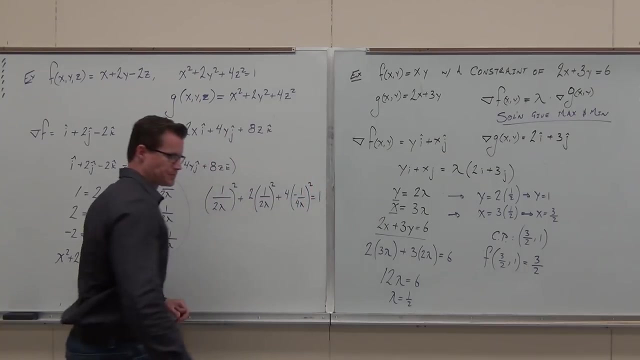 well, lambda that creates the same normal for two different level curves And where that point exists, that's the maximum end And we can simplify it. So if we simplify this, what I got was 1 over 4 lambda squared plus 1 over 2 lambda squared. 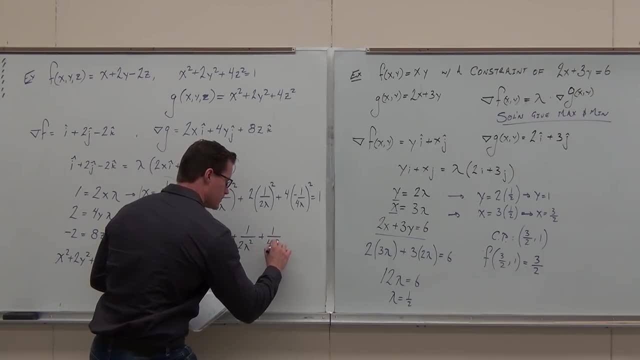 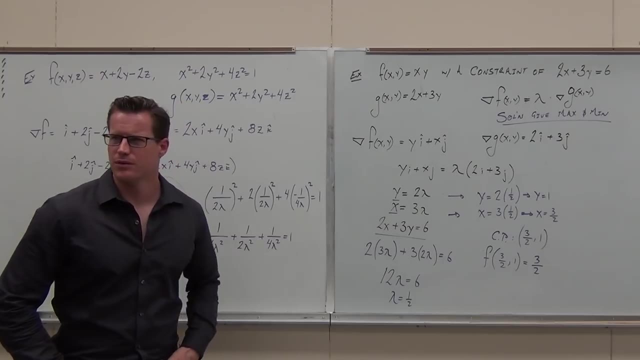 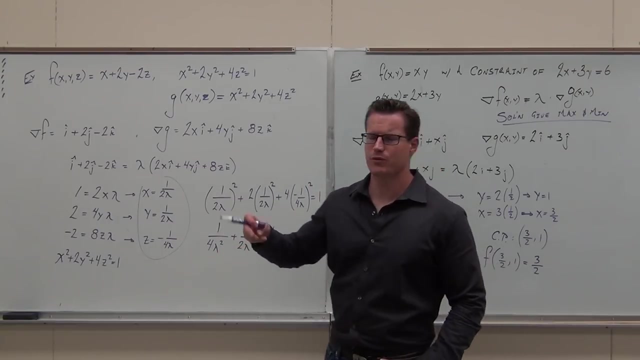 plus another 1 over 4 lambda squared Head on. if you're okay with that, so far For real Substitution, Put it in there. Hey, how would you solve that? Come on quickly, We've got to move kind of quickly on this one. 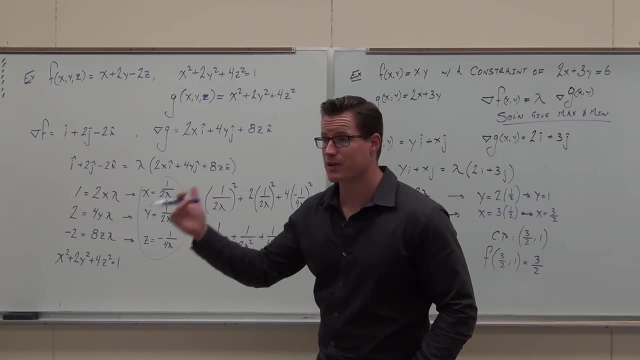 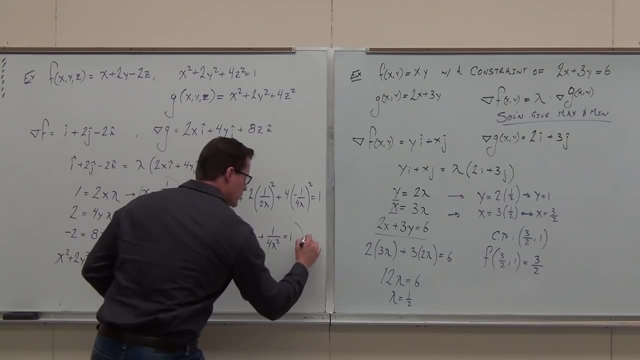 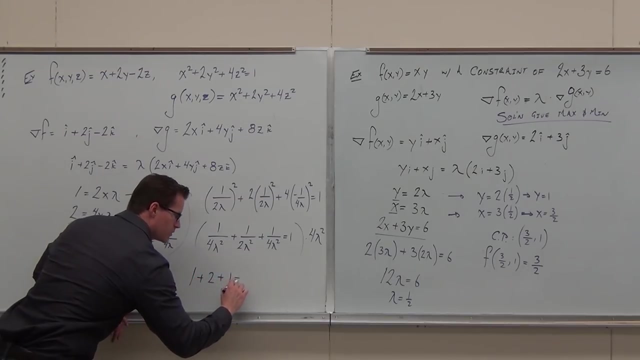 Common denominator. Okay, sure, Common denominator. whatever Multiply everything by the LCD, It doesn't matter. If we multiply everything by 4 lambda squared, then we get 1 plus 2 plus 1 equals 4 lambda squared. So that means that that side adds to 4.. 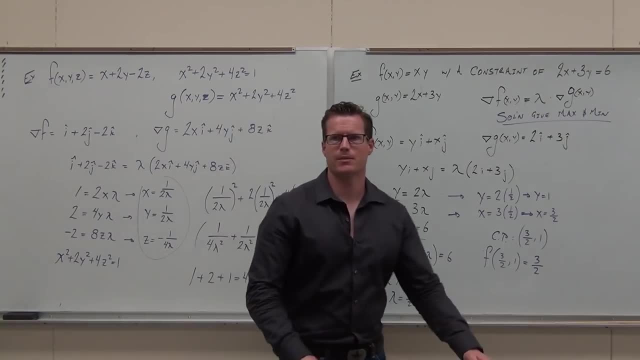 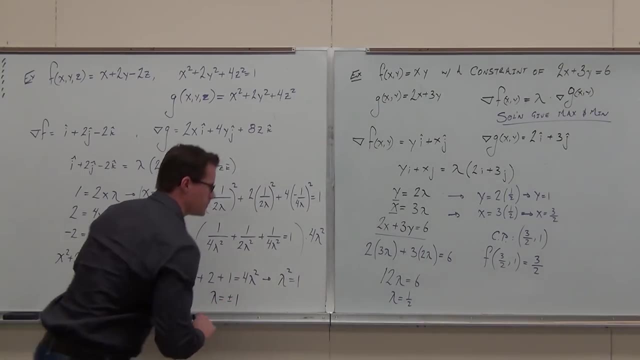 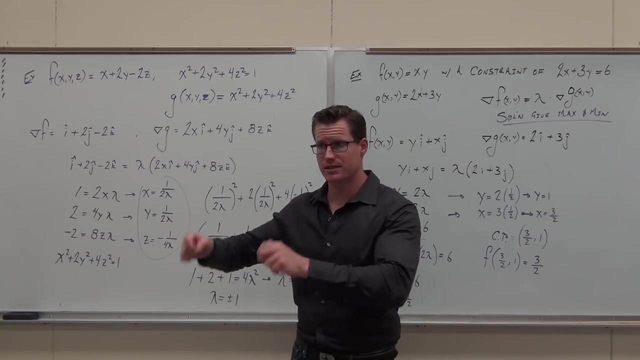 Lambda squared equals 1. Everybody, please. how much is lambda equal to? What is it Close enough? Good, we get 2.. Hey, hey, do we have something that maps us back from lambdas to x, y and z values? 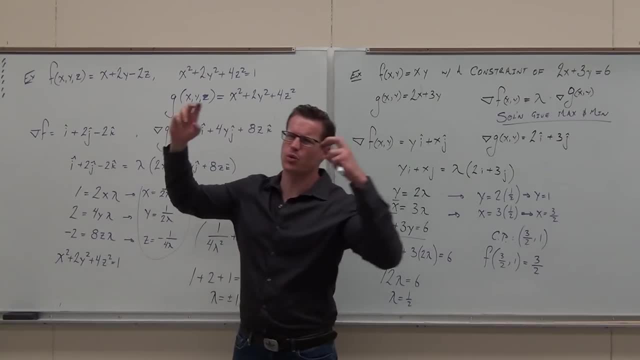 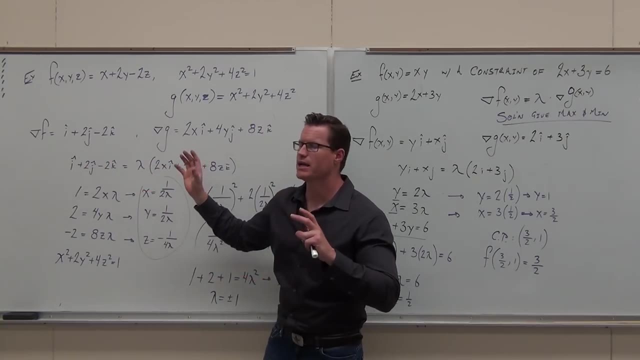 So the whole idea is gradients, yeah, Set them sort of equal. Lagrange multiplier says they're scalar multiples. That's what that is. Set component for component, Component for component, equal. Try it any way you can, any way you can to solve for lambda. 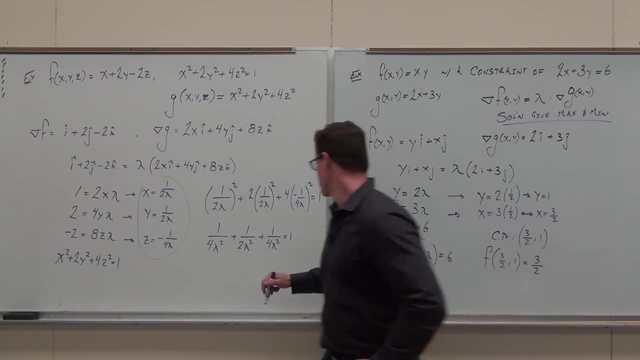 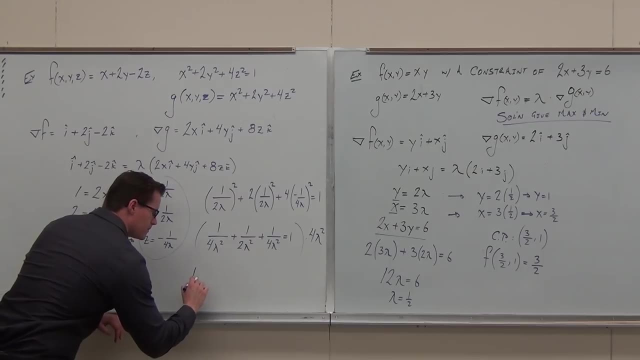 Doesn't matter. If we multiply everything by 4 lambda squared, then we get 1 plus 2 plus 1 equals 4 lambda squared. Well, that means that that side adds to 4. Lambda squared equals 1. Everybody please. 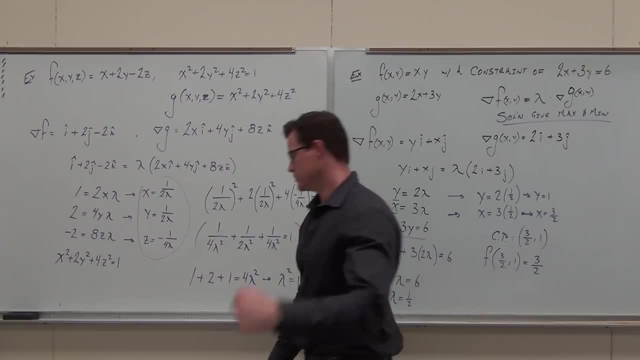 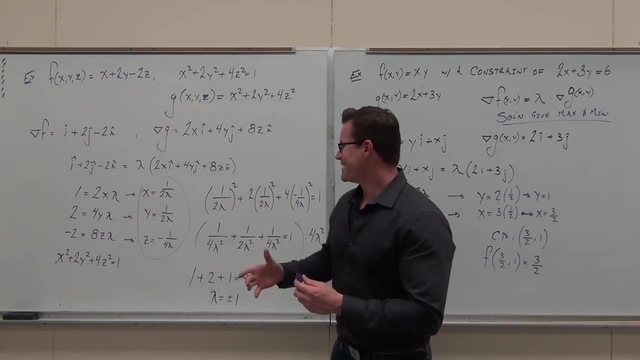 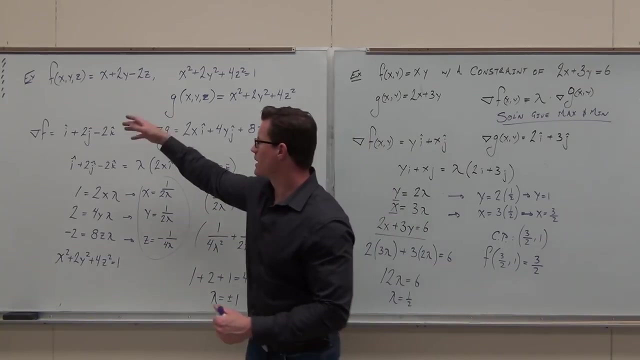 How much is lambda equal to? What is it Close enough? Good, We get 2.. Hey, hey, do we have something that maps us back from lambdas to x, y and z values? So the whole idea is gradients, yeah. 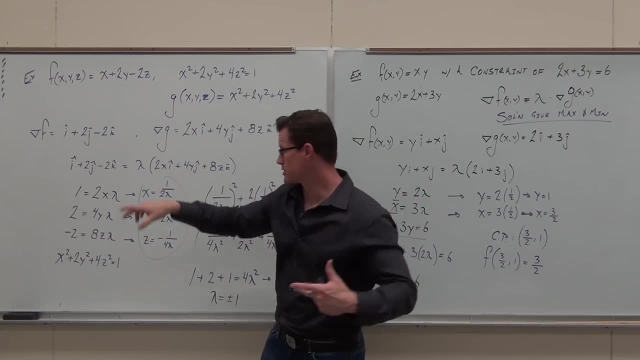 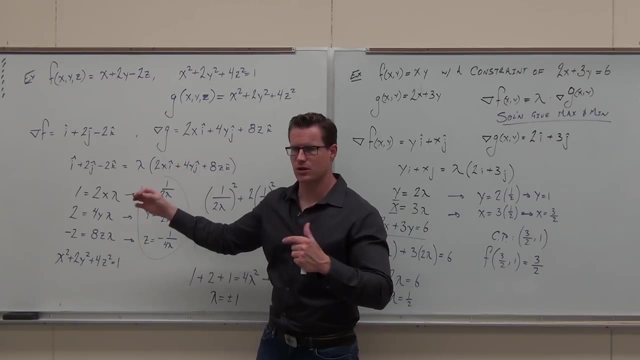 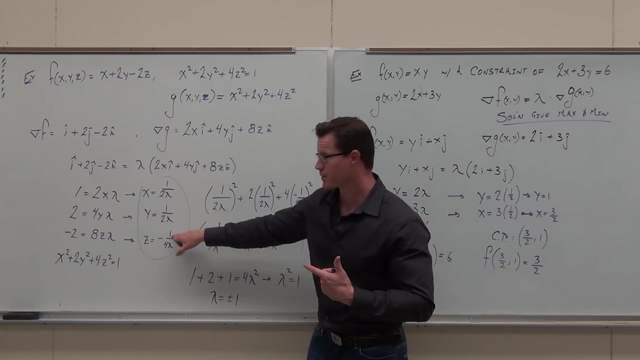 Set them sort of equal Lagrange multiplier says they're scalar multiples. That's what that is. Set component for component equal. Try it any way you can, Any way you can To solve for lambda. Then reverse substitute. So once we find our lambda we can plug in each 1 and negative 1 to all 3 of these components. 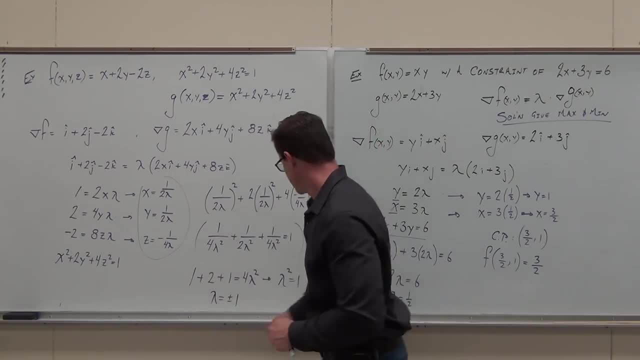 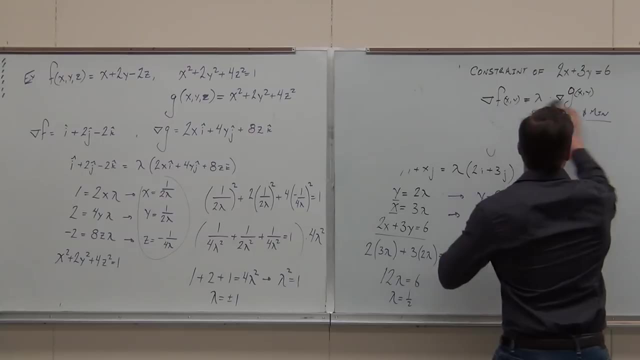 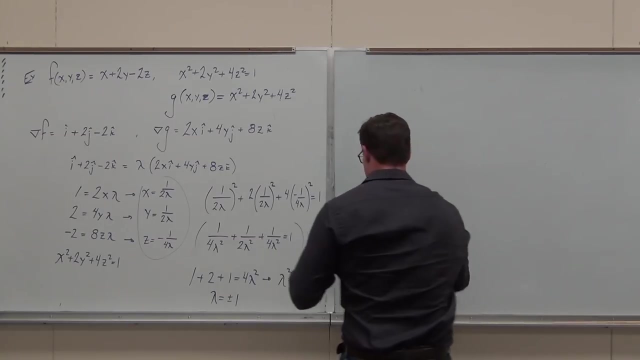 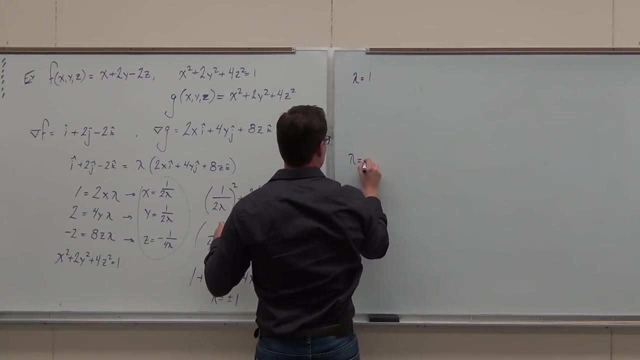 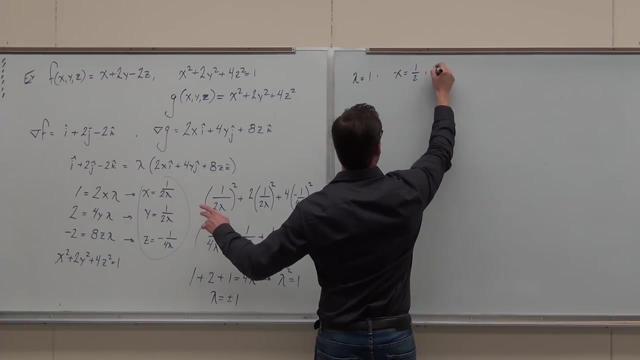 and figure out what that point is. Do it, Go ahead, Try it. used weight, Let's say Clara said we can feel it's just a CBSA-type step-backiat. We don't get the healed very easily, exactly, You don't get the correct data set, like at 10, and you can't punch it back. 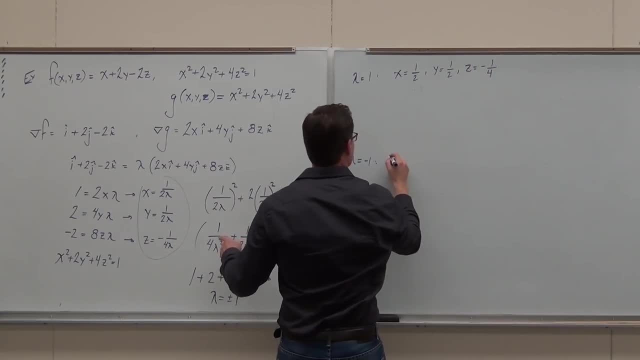 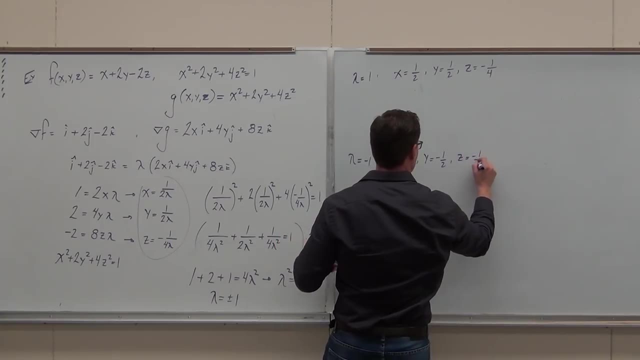 Instead, you have to go to the table and you have to. goodness, If you get a canopies and- and quick thing, get that. we're still out of here, But those would be faster. Say: we have canopies left over and y left over. 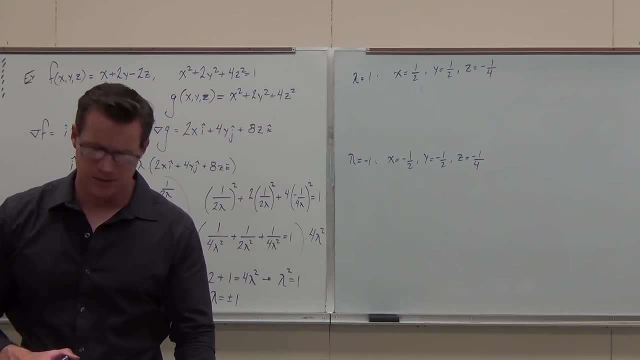 You don't have to fix that, Dramatize it, Dramatize it. That's just realize you got to do that And you have to be bit stressed. Same things that I got Now. here's what we said before. 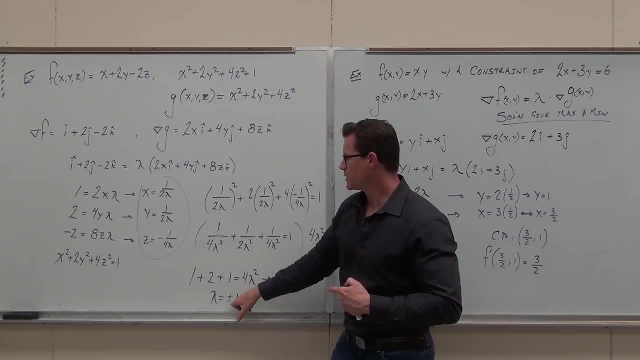 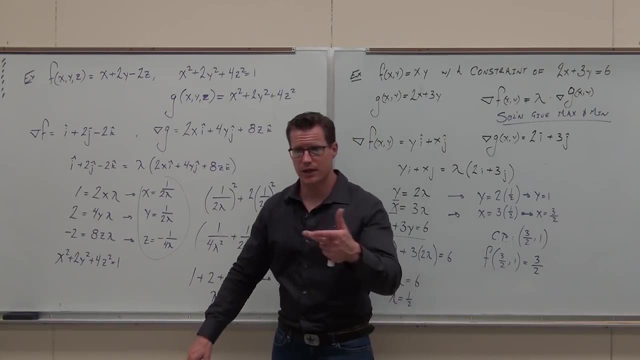 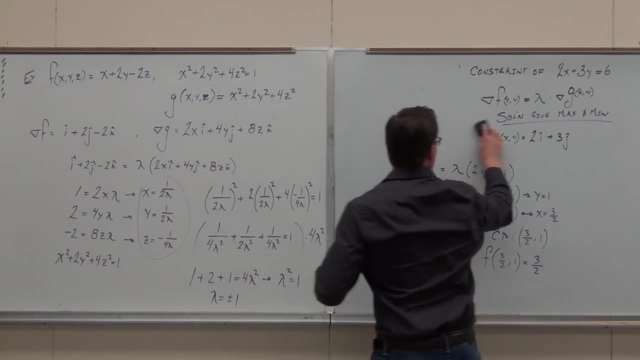 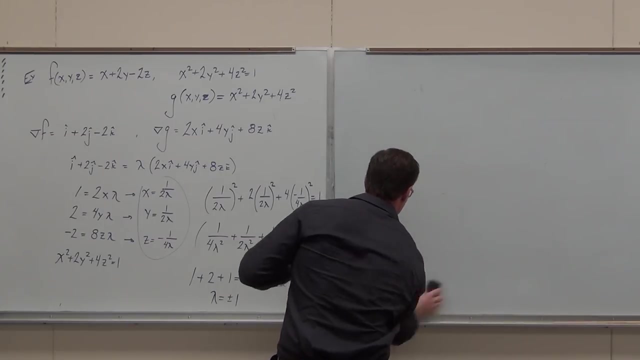 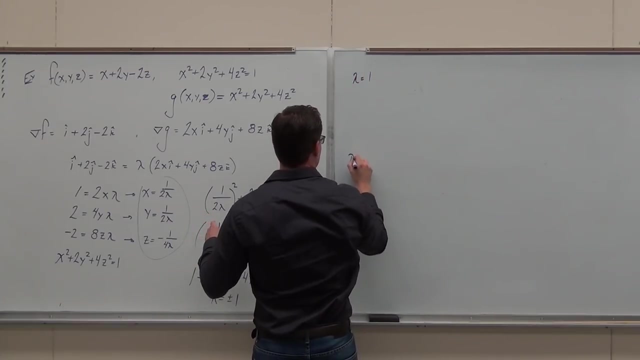 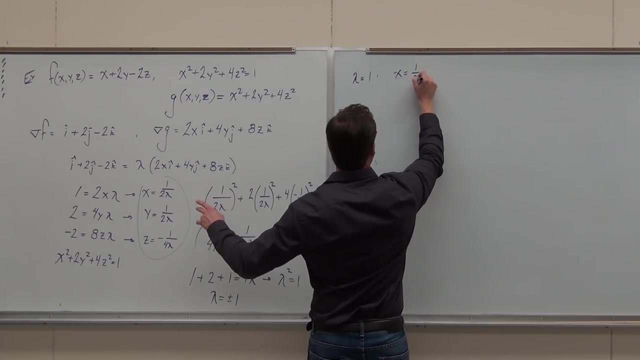 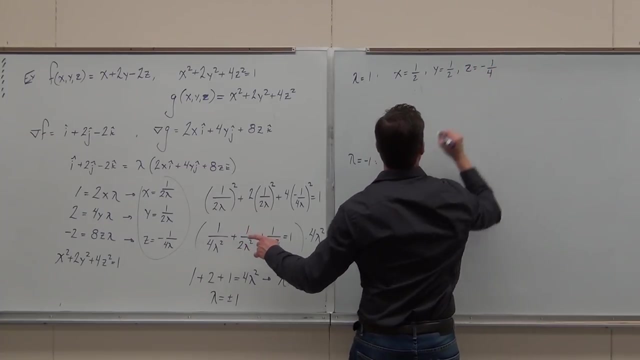 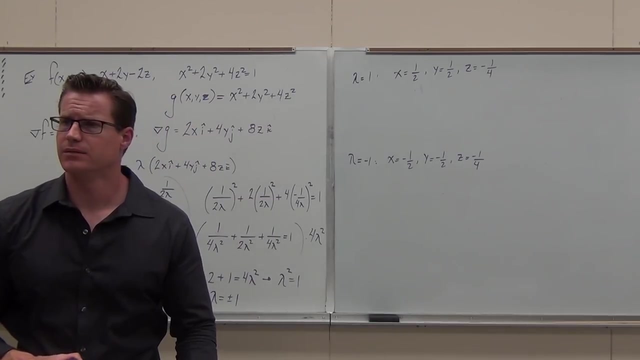 Then reverse substitute. So once we find our lambda, we can plug in each 1 and negative 1 to all three of these components and figure out what that point is. Do it, Go ahead, Try it, So we get the same things that I got. 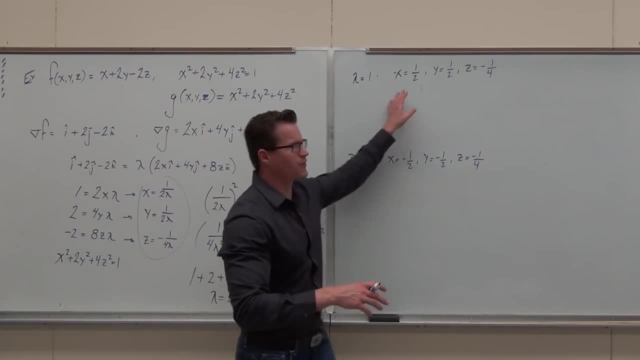 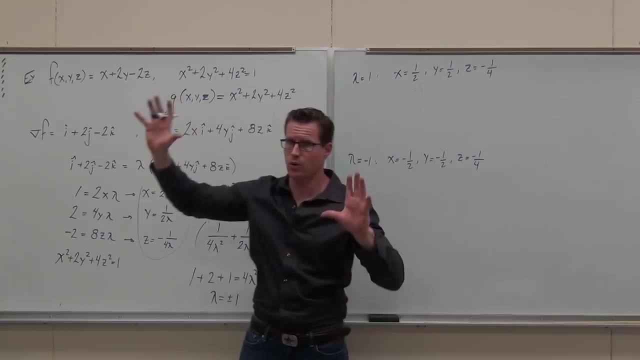 Now here's what we said before. What we said was at that point: verify, that's one single point. x, y, z. one single point for that function, Head nod, yes, no, It also satisfies this thing. That was the whole key here. 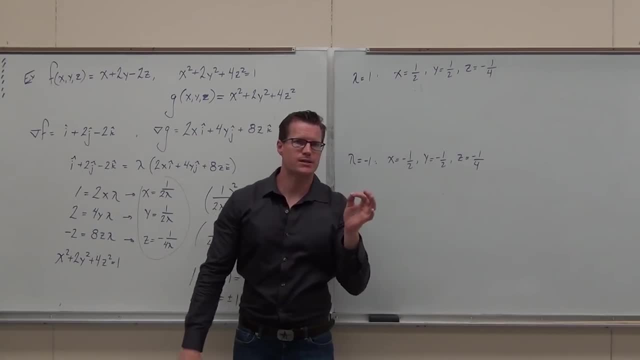 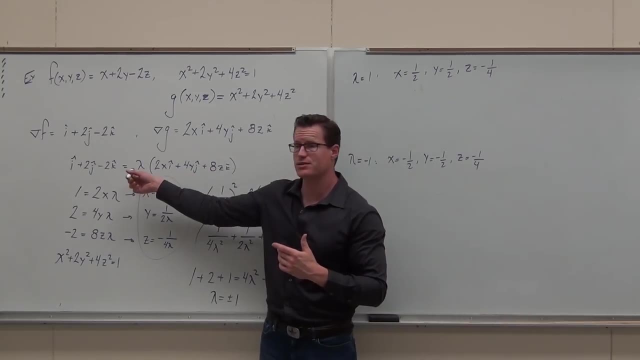 So we have one point, We have two points. One of these is going to be the max, One of these is going to be the min. Maxima and minima are found at solutions to this. That was the statement I made earlier. 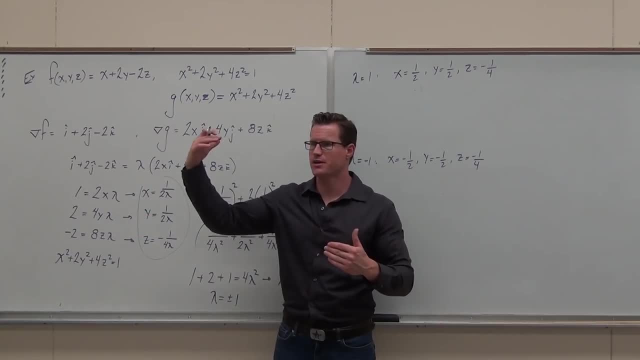 So what we're finding are maxima and minima. Whatever the highest value is, that's our max. Whatever the minimum value is, that's our min. How do you figure out which one's the biggest one and which one's the smallest one? 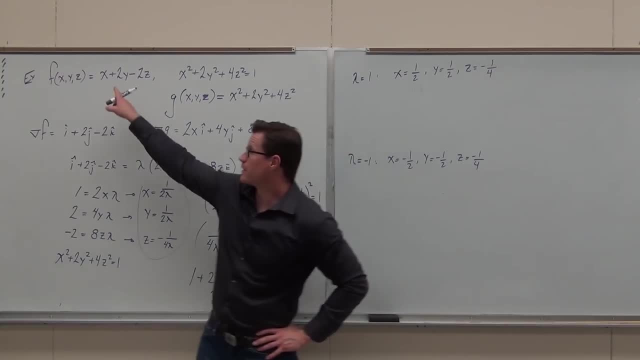 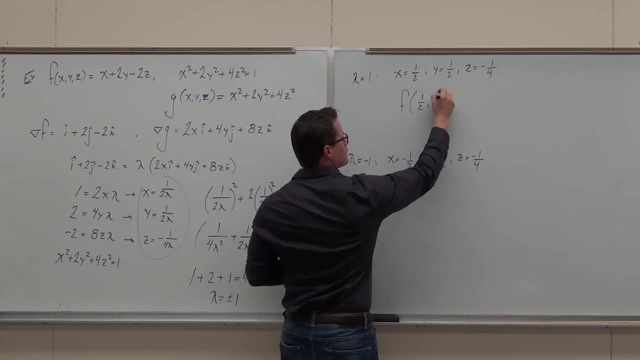 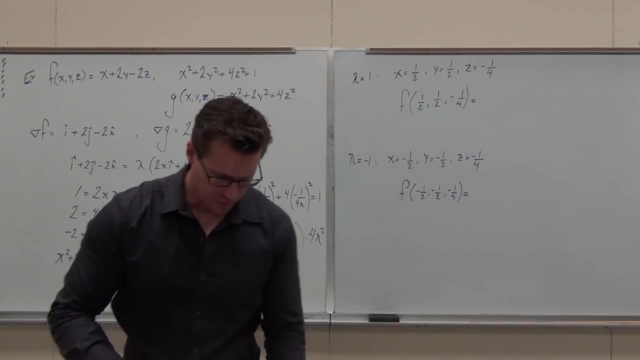 Plug it in. Plug it into where? Plug it into the original Right there, Plug it in right there. So if we plug it into that f of this, F of that, Plug them in. I've already done it for you. 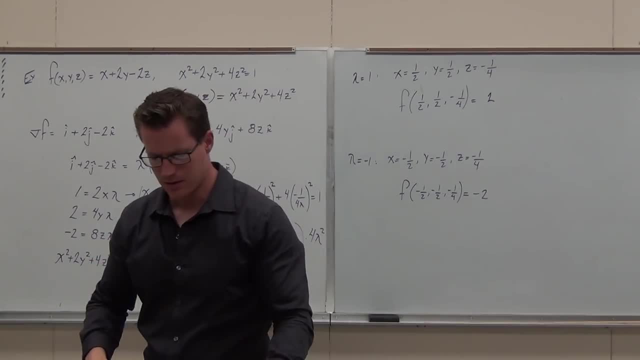 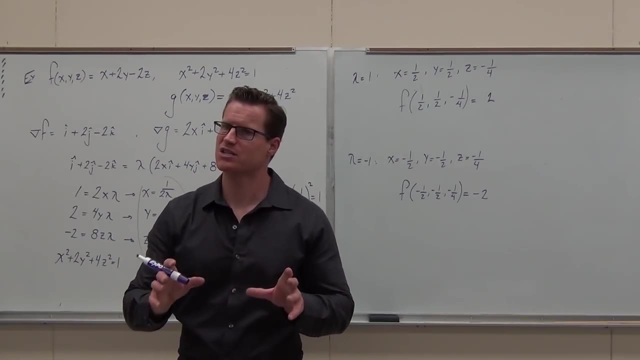 2 and negative 2.. If you can double check me, I think I got those ones right. Hey, that's kind of cool right? There's no checking, There's no guesswork. What's the maximum value? What's the maximum value of this function based on the fact that we have to satisfy that constraint? 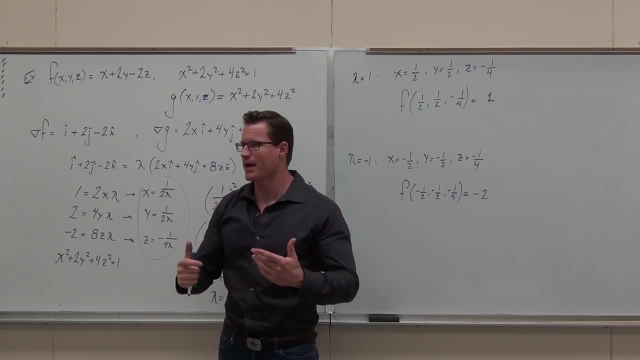 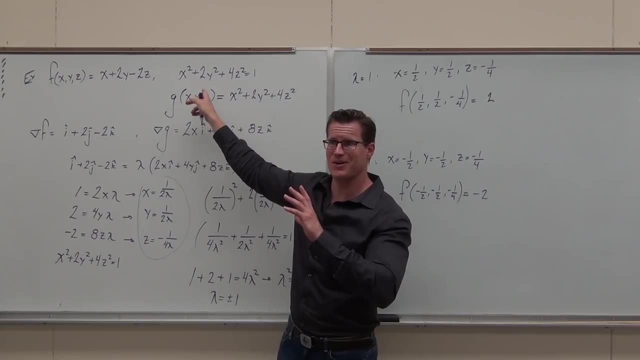 What's the maximum value? 2. Yeah, That's called a constrained maximum. It's the highest that surface gets, but based on the fact that we've got to satisfy that, That's kind of cool right. So this is the max. 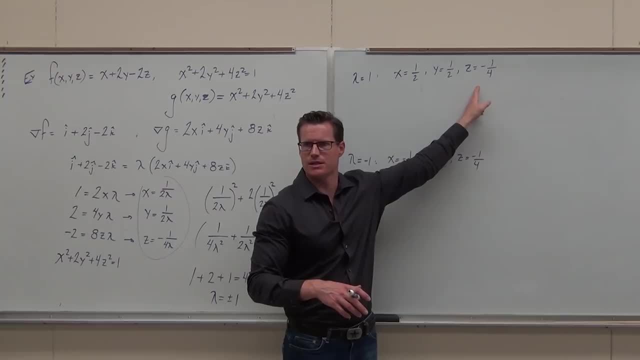 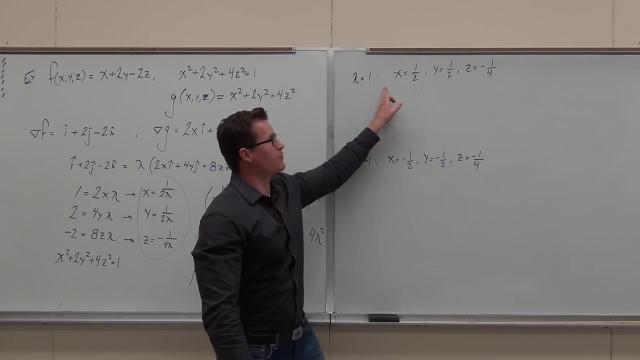 What we said was at that point: verify. that's one single point: X, Y, Z. one single point for that function. head nod, yes, no, It also satisfies this thing. That was the whole key here. So we have one point. 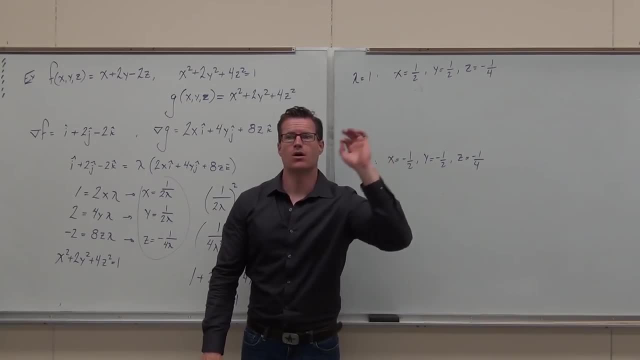 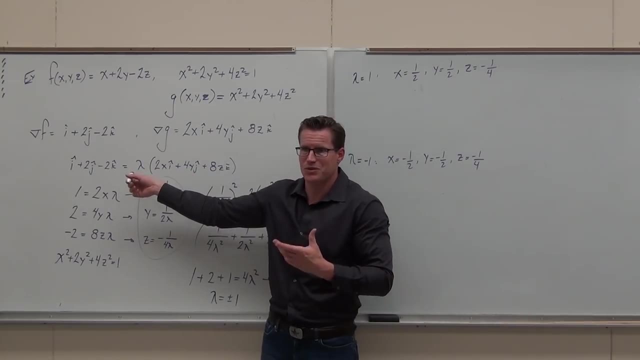 We have two points. One of these is going to be the max, One of these is going to be the min. Maxima and minima are found at solutions to this. That was the statement I made earlier. So what we're finding are maxima and minima. 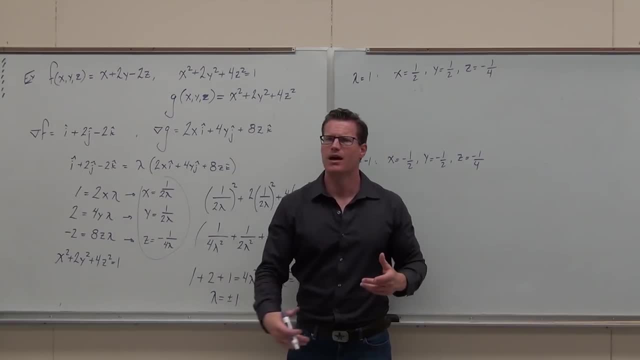 Whatever the highest value is, that's our max. Whatever the minimum value is, that's our min. How do you figure out which one's the biggest one and which one's the smallest one? Plug it into where? Plug it into the original. 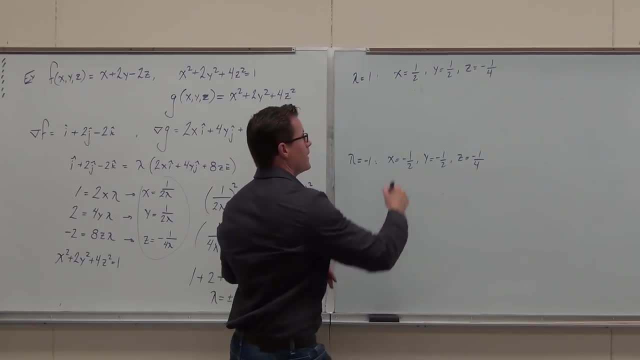 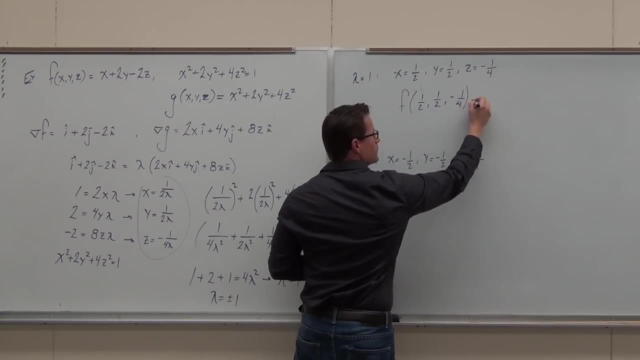 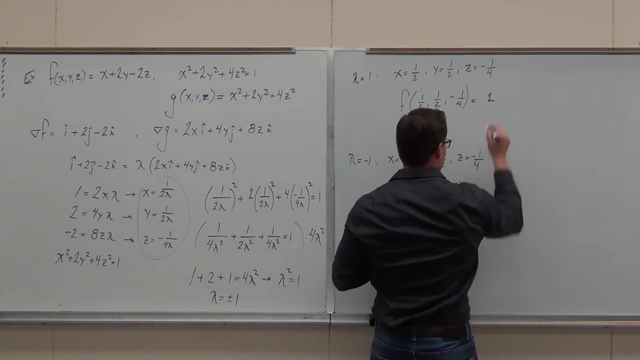 Right there. Plug it in right there. So if we plug it into that F of this F of that, plug them in. I've already done it for you. 2 and negative 2.. If you can double check me, I think I got those ones right. 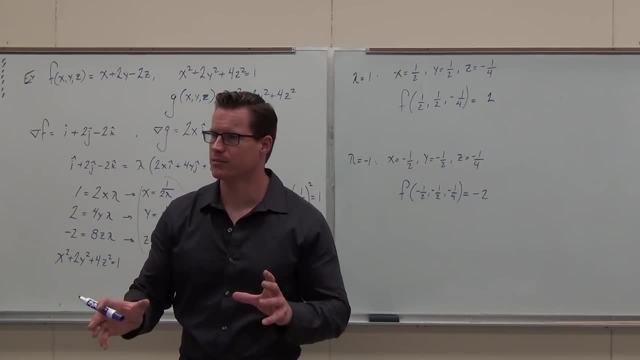 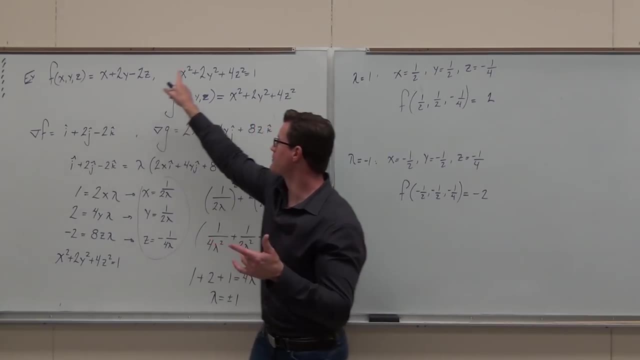 Hey, that's kind of cool, right, There's no checking, There's no guesswork. What's the maximum value? What's the maximum value of this function, based on the fact that we have to satisfy that constraint? What's the maximum value? 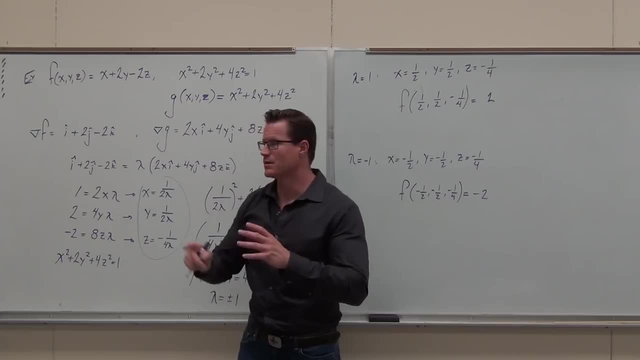 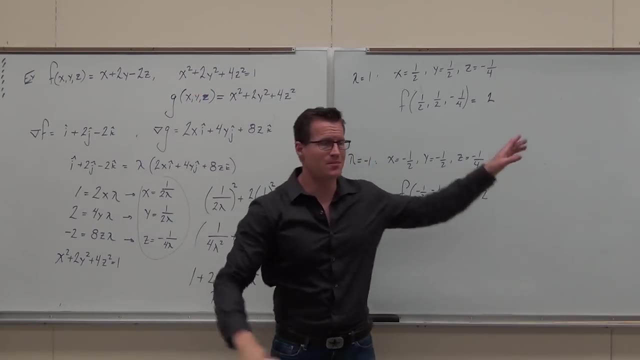 2. Yeah, that's called a constraint maximum. It's the highest that surface gets, but based on the fact that we've got to satisfy that, That's kind of cool right. So this is the max and this is the min. 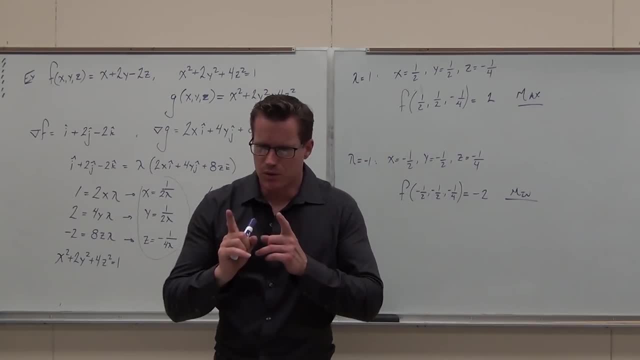 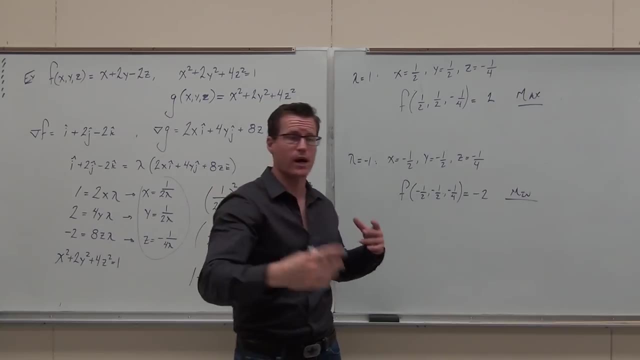 That's the idea. These are the two values. we have those scalar multiple normals where we create that point that we bounce off One level curve bounces off another one. We happen twice. One of them's the high point, one of them's the low point. 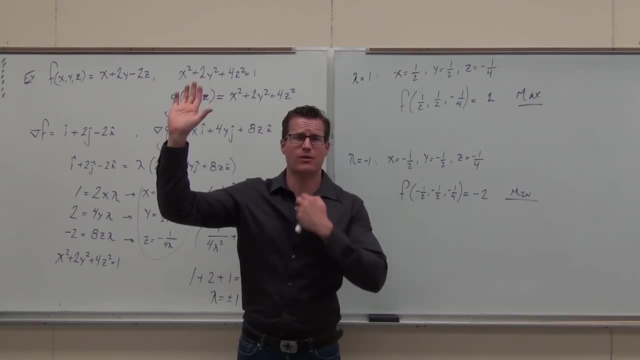 Pretty neat, huh. So, fans, if you understand, I'll tell you what We have. one more really hard problem. It's hard only because of the substitutions. Obviously, gradient's pretty easy, right Gradient's pretty easy, This is pretty easy. but doing this 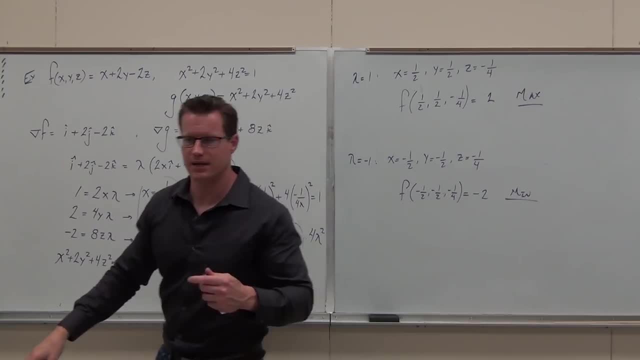 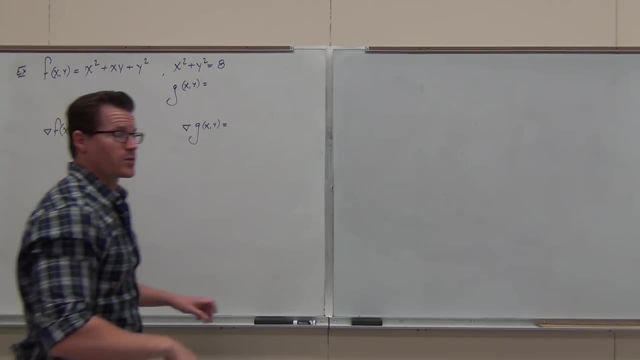 the system's going to be kind of tough, So we're going to try that next time. So, as I said, a hard problem, hard problem. We did one really easy. We did one with three variables. Now we got one really hard. 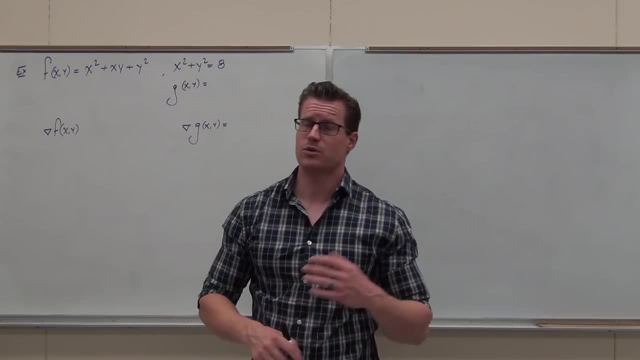 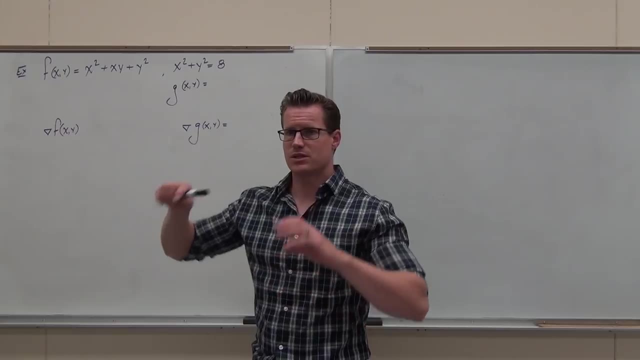 The thing that's going to make it hard is the algebra, The algebra behind it. If you recall, we're working on constrained optimization, Those Lagrange multipliers, And the idea was: take level curves, find normal level curves. it's gradient. 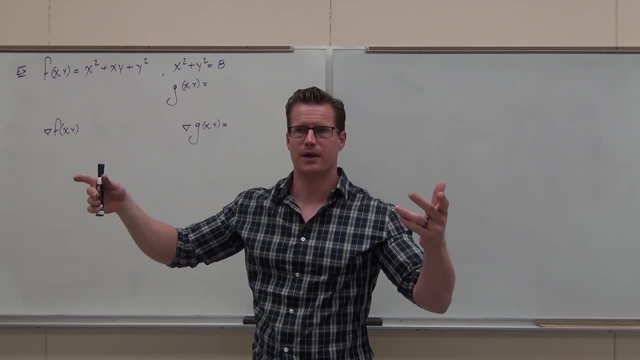 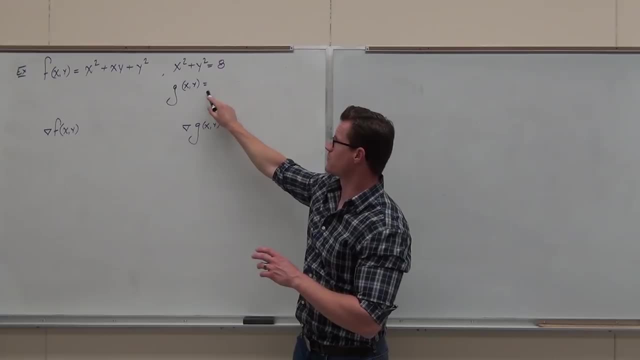 They have to be scalar, multiples, if we're going to share a common normal. That was the plan. So when we're given these two functions- okay, here's your surface, here's your level curve- we must create a surface for that to be a level curve of. 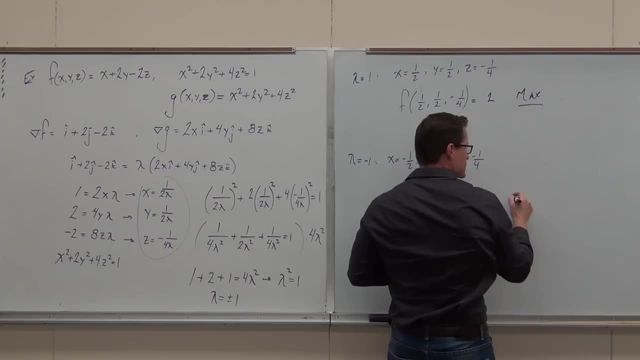 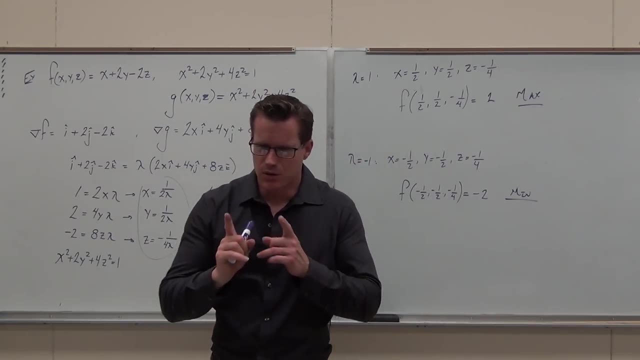 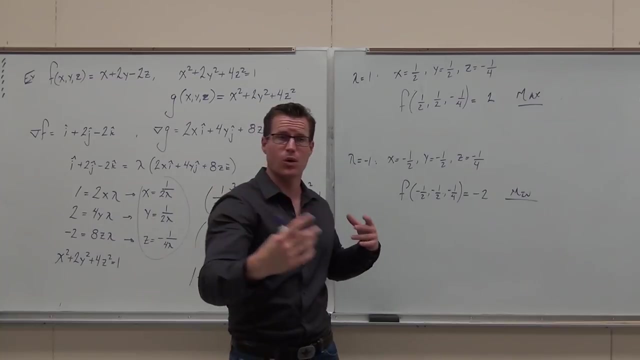 And this is the min. That's the idea. These are the two values where we have those scalar multiple normals, where we create that point that we bounce off One level curve bounces off another one, We happen twice. One of them is the high point. 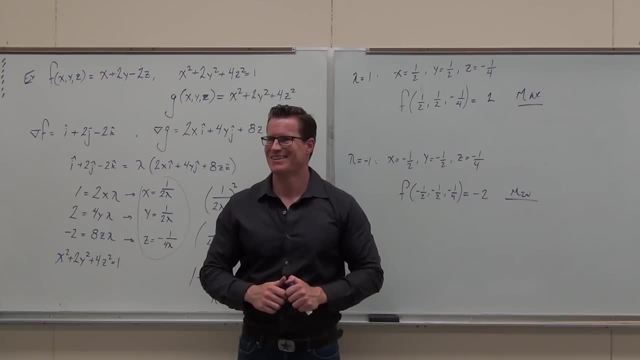 One of them is the low point. Pretty neat, huh. So, fans, if you understand, I'll tell you what We have one more really hard problem. It's hard only because of the substitutions. Obviously, gradient's pretty easy right. 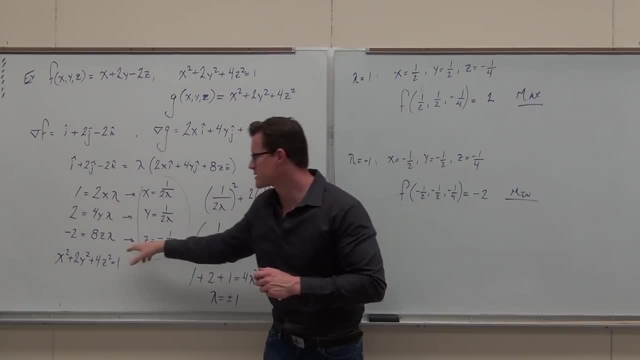 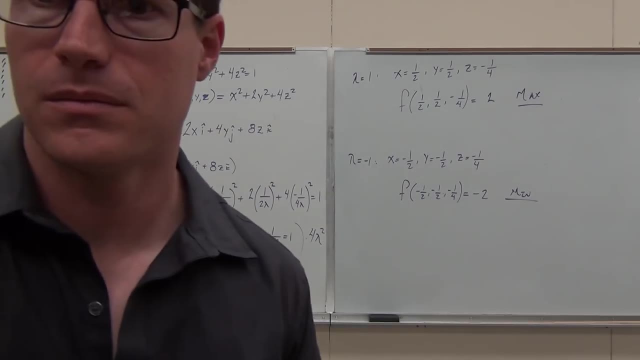 Gradient's pretty easy, This is pretty easy. But doing this the systems can be kind of tough, So we're going to try that next time. So, as I said, a hard problem, Hard problem, We did one really easy. 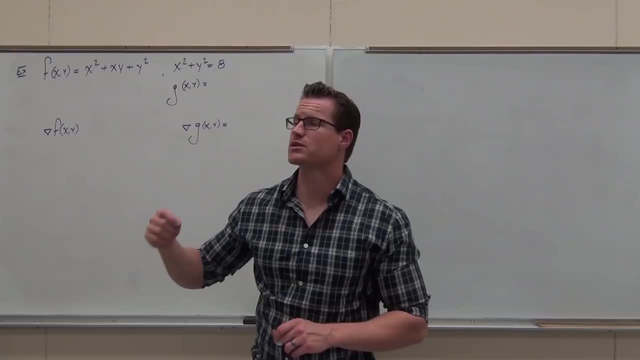 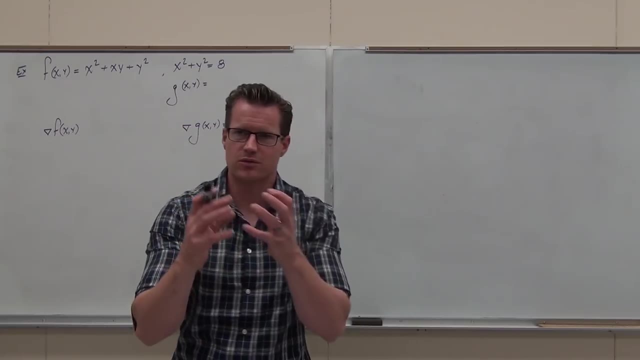 We did one with three variables. Now we got one really hard. The thing that's going to make it hard is the algebra behind it. If you recall, we're working on constrained optimization- Those Lagrange multipliers- And the idea was: take level curves, find normals to level curves. 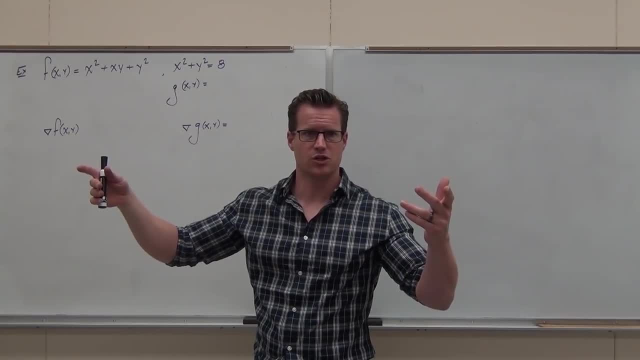 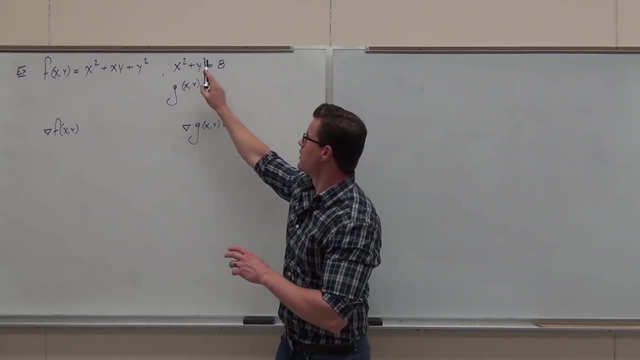 It's gradient. They have to be scalar multiples if we're going to share a common normal. That was the plan. So when we're given these two functions, okay, here's your surface, here's your level curve- we must create a surface for that to be a level curve. 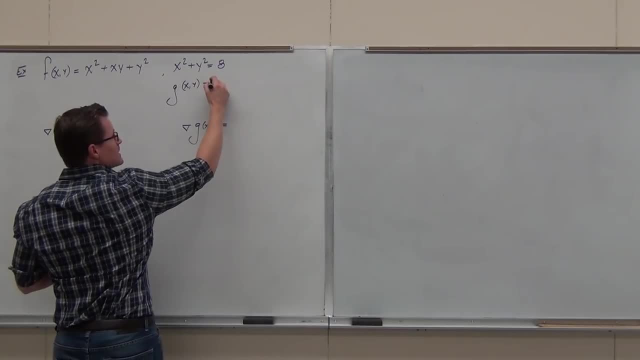 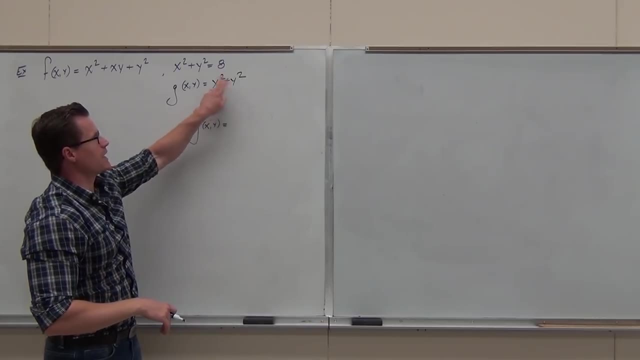 For that to be a level curve of that's basically just take your variables. Good, That's the surface And you can verify it. If I set this equal to 8, I get that specific level curve. that is on that surface heading. 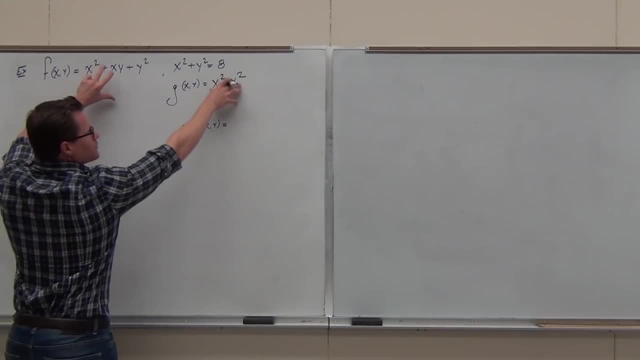 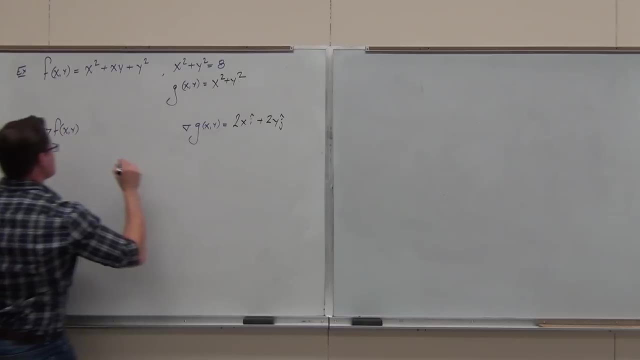 on the two ways around, that one After that we find the gradient of both of these surfaces. This is 2xi plus 2yj. This is 2x Plus yi. plus what 2x? Yeah, we can do it that way. 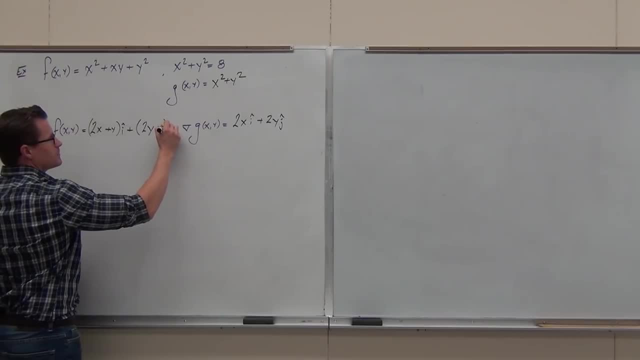 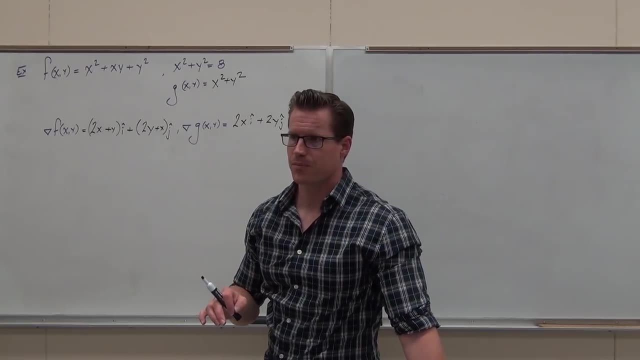 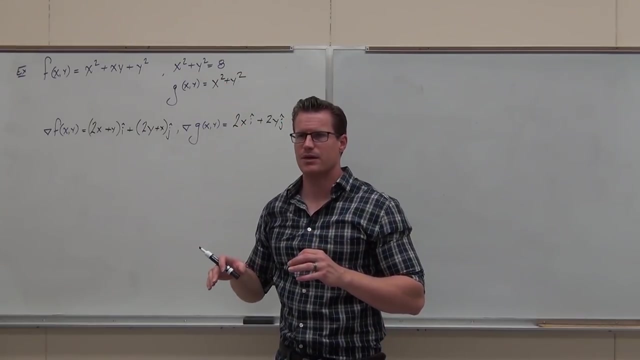 J. Those are the two gradients, Those are the two normals to those level curves. so those surfaces, Are you following me? Which means it's a normal to that specific level curve And we're saying that we want to find the points where these things are scalar multiples. 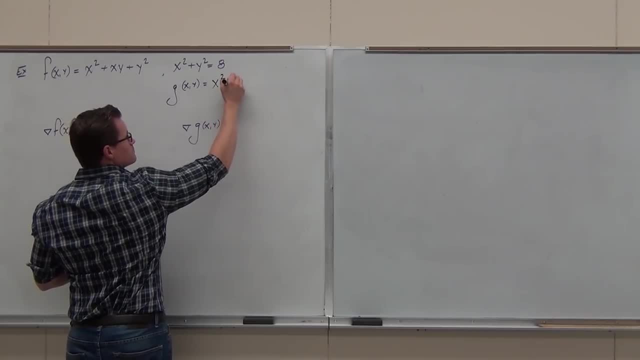 That's basically just take your variables. Good, So we're going to do that next time. So, we're going to do that next time. So we're going to do that next time. Good, That's the surface and you can verify it. 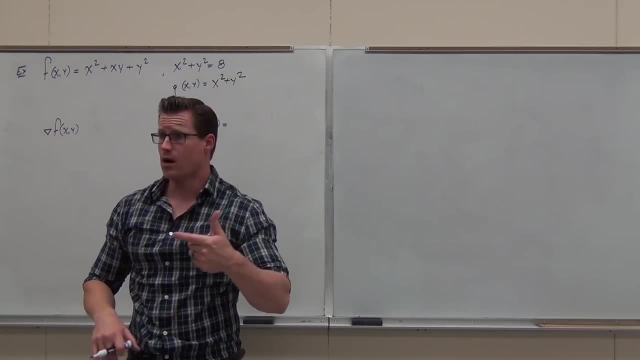 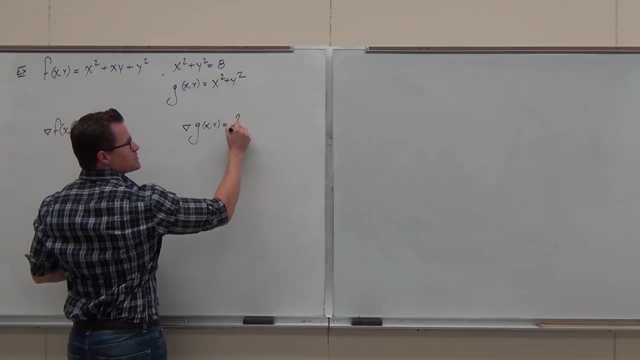 If I set this equal to eight, I get that specific level curve that is on that surface, heading on the two ways around that one. After that we find the gradient of both of these surfaces. This is 2xi plus 2yj. 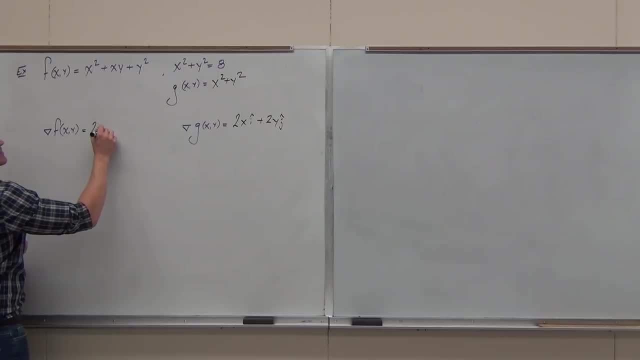 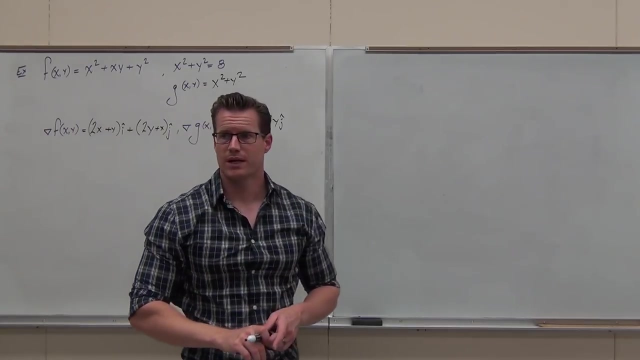 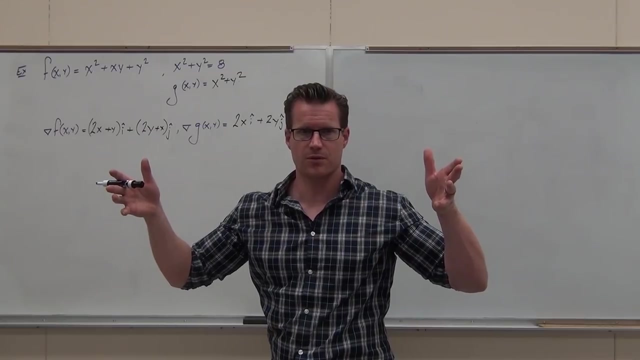 This is 2xi plus what 2x. Yeah, we can do that, We can do that way. J. Those are the two gradients, Those are the two normals to those level curves. so those surfaces, Are you following me? 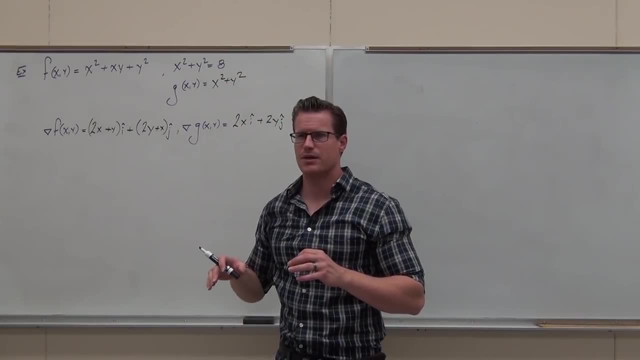 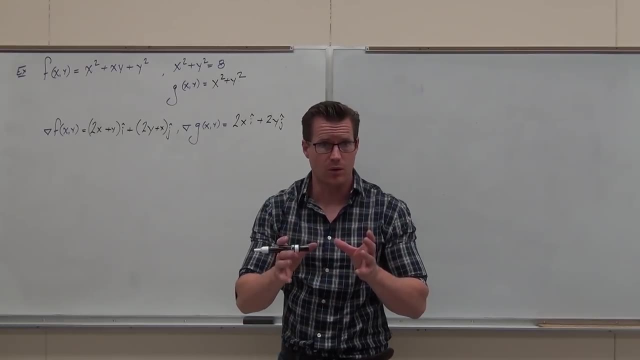 Which means it's a normal to that specific level curve. and we're saying that we want to find the points where these things are scalar multiples. That's why we set the lambda, some constant that we don't know, but we do know at the points we're looking for, where the level curves bounce off each other, they will have normals. 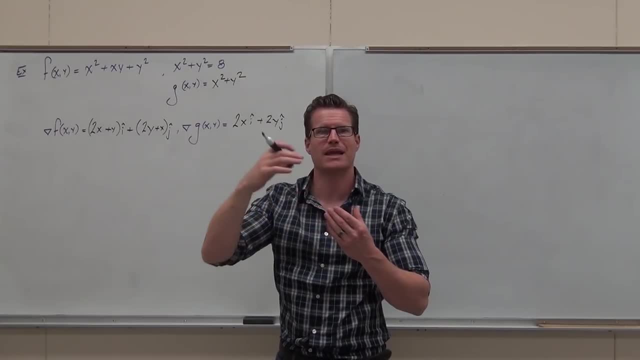 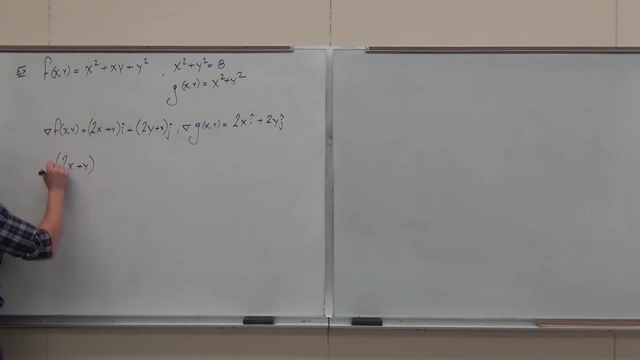 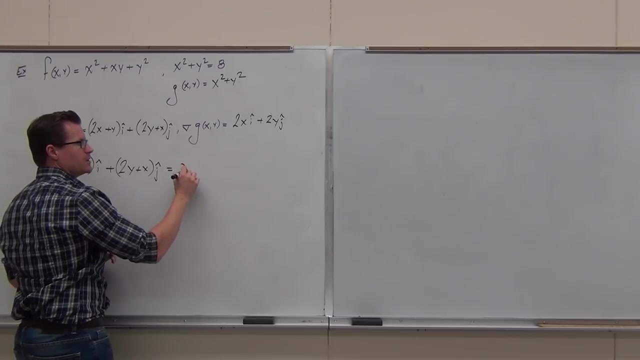 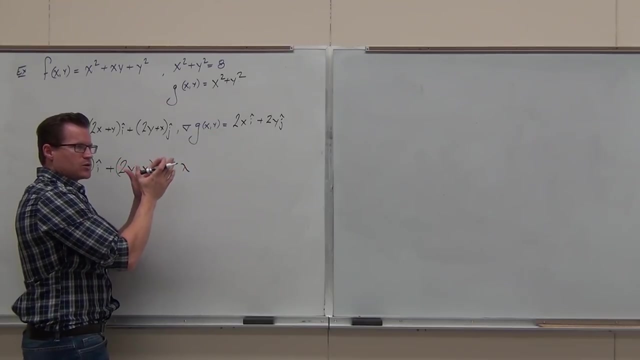 that are scalar multiples. So we force it to happen by finding the lambda, the scalar multiple that makes it happen. Okay, well, that means that 2x plus yi plus 2y plus xj equals lambda Some. these must be scalar multiples for us to have a common tangent, common normal. 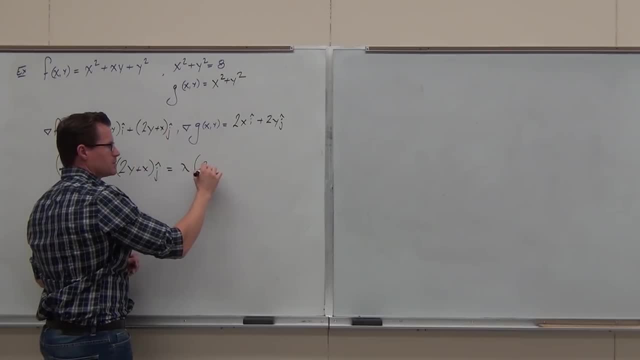 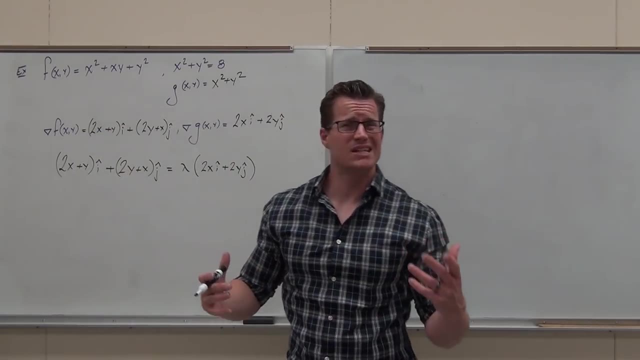 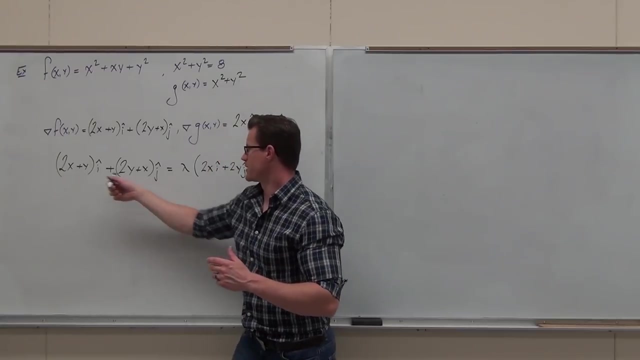 or force those level curves to bounce off each other. That's the main part. That's actually the easy part. I'm going to show fans if you see where all this stuff is coming from. Now. the idea is, if I have one vector- verified vector equal to a scalar multiple. 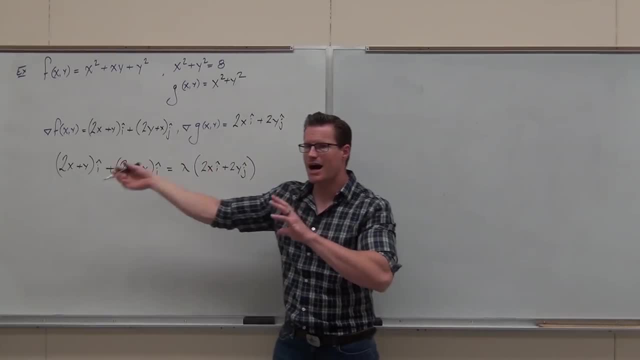 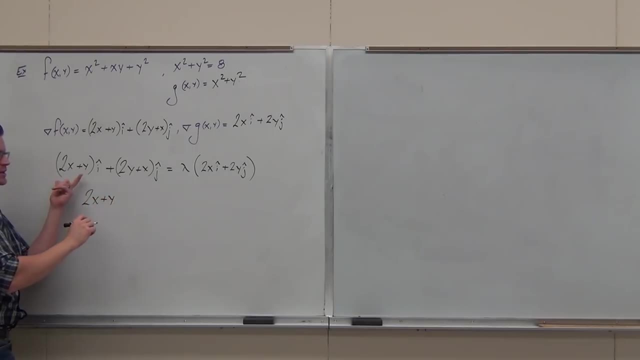 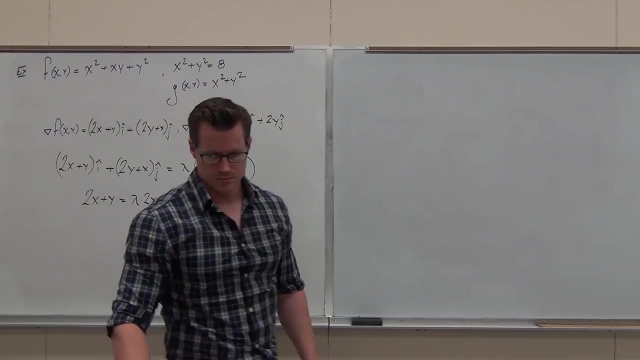 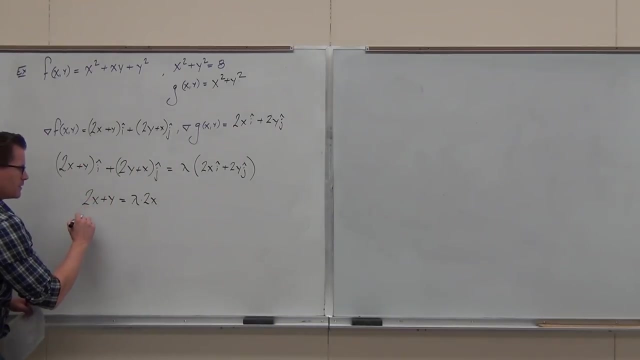 of another vector, the components of those vectors- i and j, have to be equal. so I know that 2x plus y must equal lambda times 2x. Does that make sense to you? I also know that 2y plus x has to equal lambda times 2y. 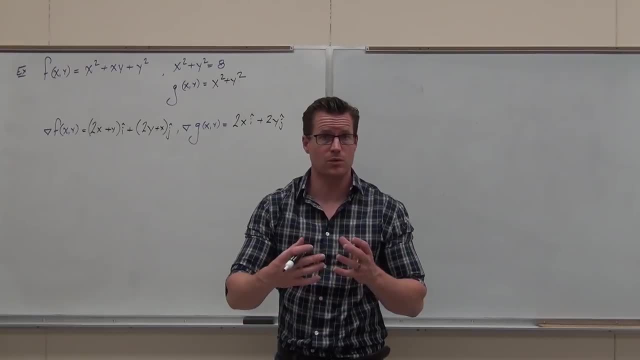 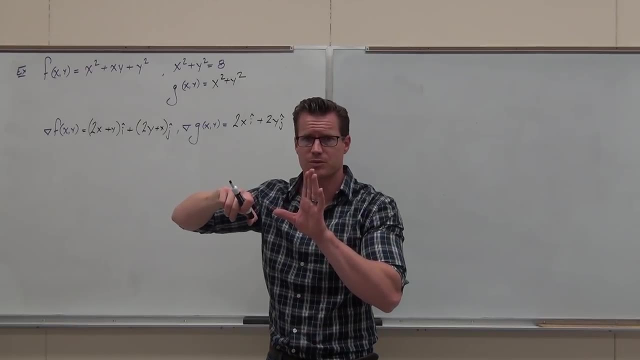 That's why we set them equal to lambda- Some constant that we don't know, but we do know at the points we're looking for, where the level curves bounce off each other, they will have normals that are scalar multiples. So we force it to happen by finding the lambda, the scalar multiple that makes it happen. 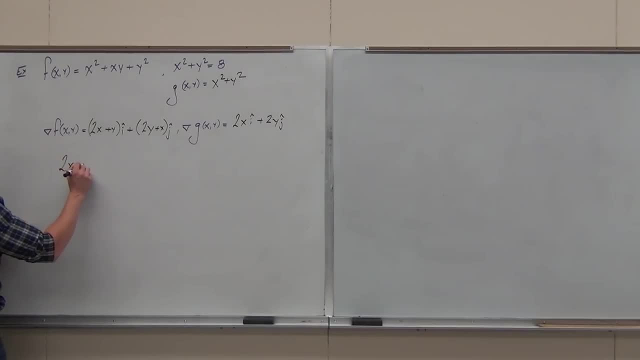 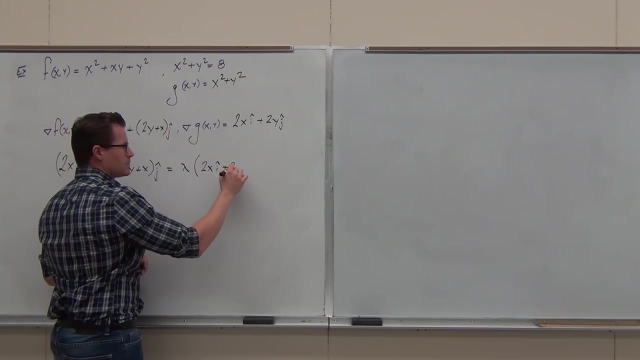 Okay, well, that means that 2x plus yi plus 2y plus xj equals lambda. These must be scalar multiples for us to have A common tangent. common normal will force those level curves to bounce off each other. That's the main part. 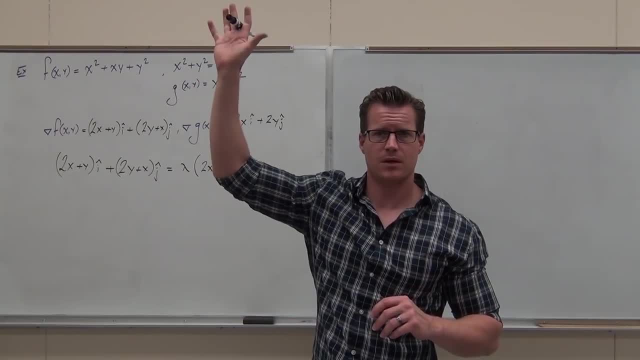 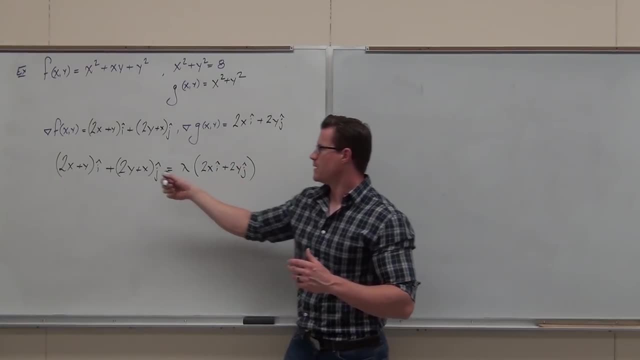 That's actually the easy part. I'm going to show fans if you see where all this stuff is coming from. Now, the idea is, if I have one vector, verified vector equal to a scalar multiple of another vector, the components of those vectors- i and j- have to be equal. 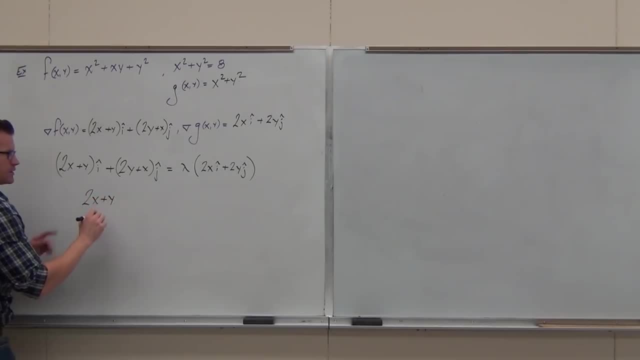 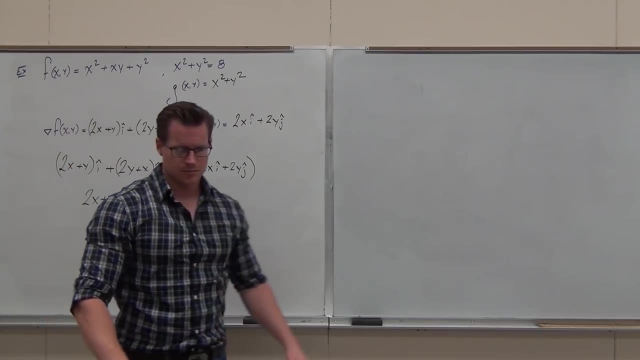 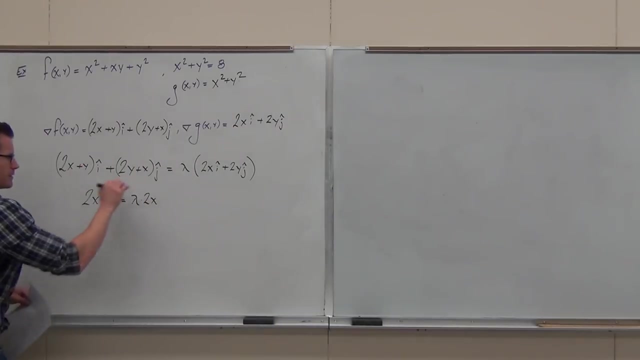 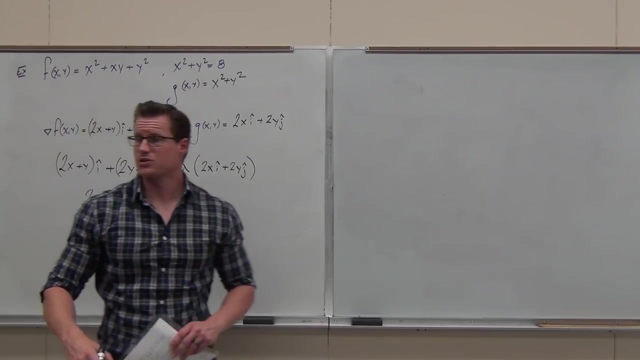 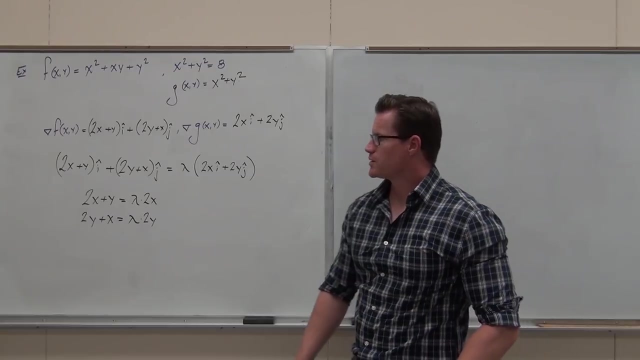 So I know that 2x plus y must equal lambda times 2x. Does that make sense to you? I also know that 2y plus x has to equal lambda times 2y. Those things have to be there. What I've told you pretty much this whole time is write these down. 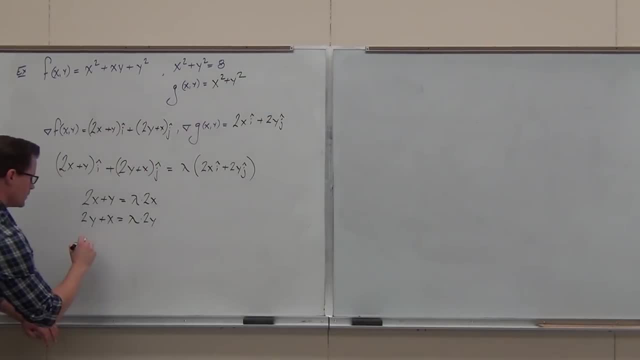 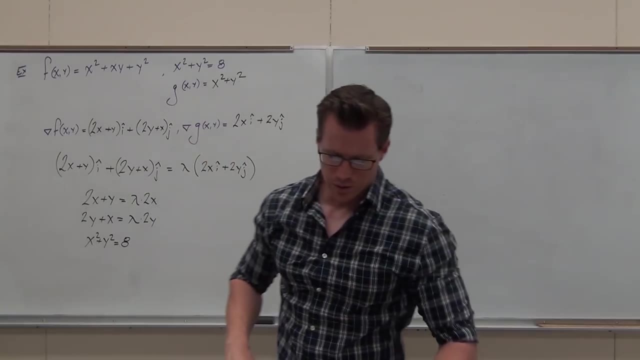 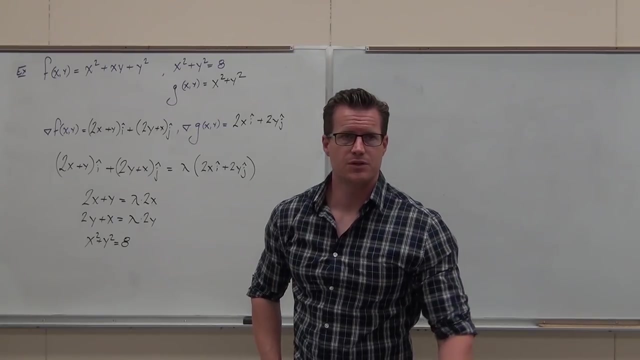 Write down your constraint. The whole goal in life for you in this section, is to solve lambda. I've given you two ways and there are two different ways to do it. I'm going to give you this third one. It's a third way to do it. 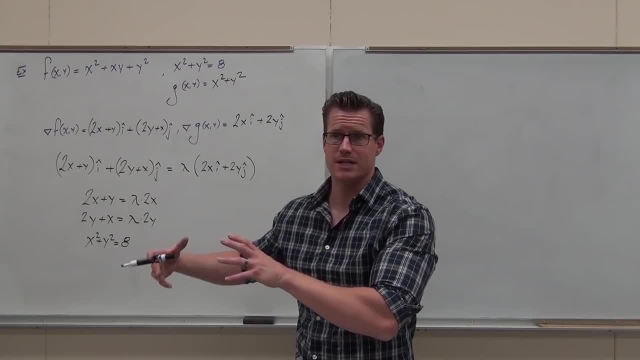 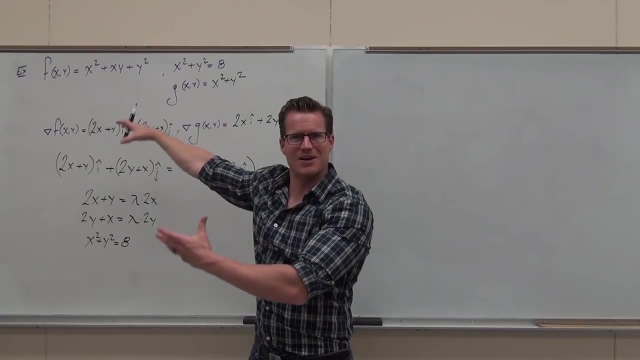 I've given you three completely different examples to show you three different techniques. This one's not going to be that easy. There's a lot of algebra behind it. This was the easy part. Do you understand the idea behind this? That's pretty cool, right. 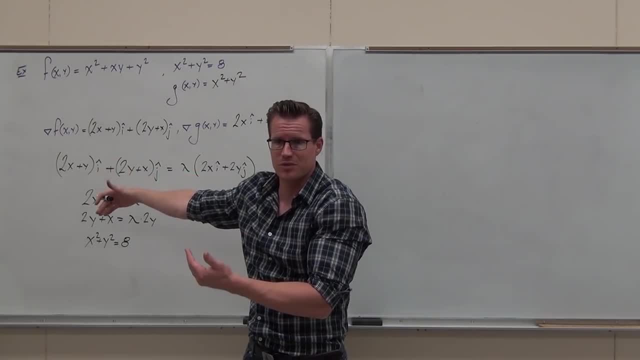 We're setting gradients equal to each other by a scalar multiple. It's called the Lagrange multiplier. That's pretty much it. Our goal is to find that and then substitute back in to solve this thing. So we're going to do that. 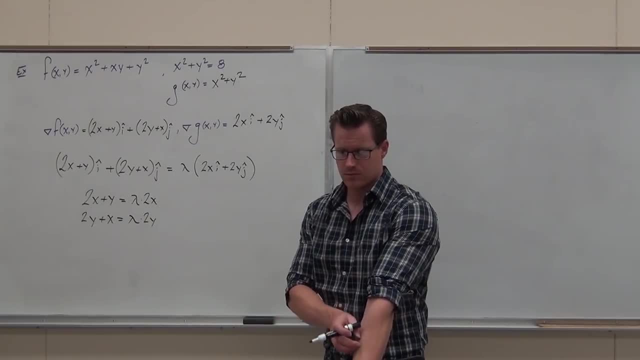 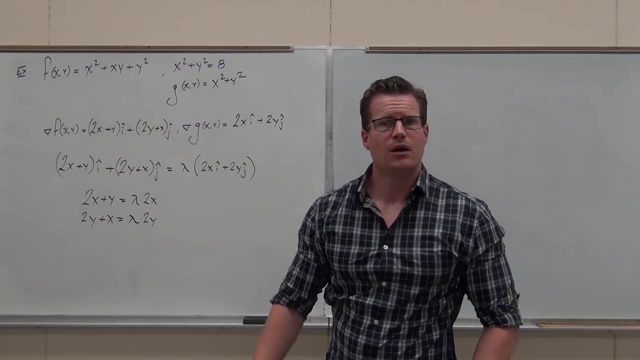 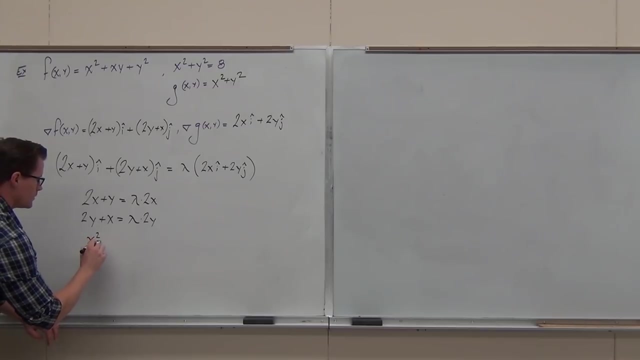 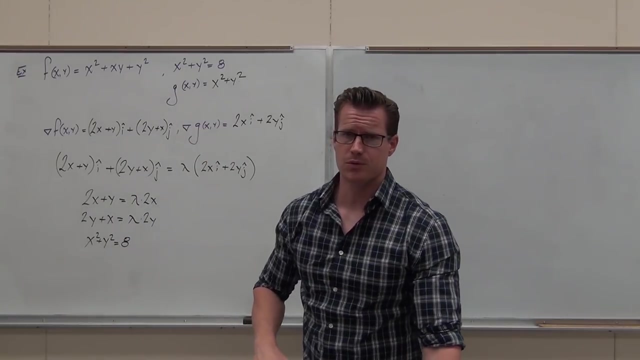 Those things have to be there. What I told you, what I've told you pretty much this whole time, is: write these down, Write down your constructions, Write down your constraint. The whole goal in life for you in this section, is to solve lambda. 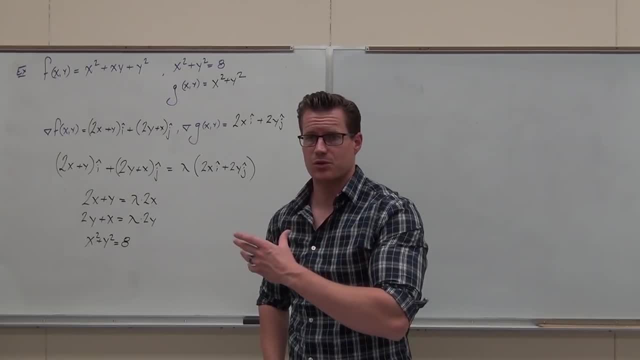 I've given you two ways and there are two different ways to do it. I'm going to give you this third one. It's a third way to do it. I've given you three completely different examples to show you three different techniques. 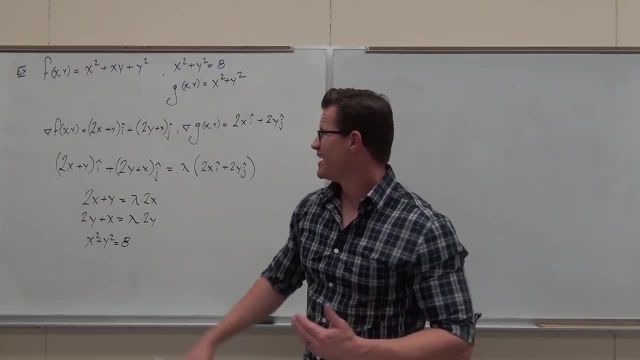 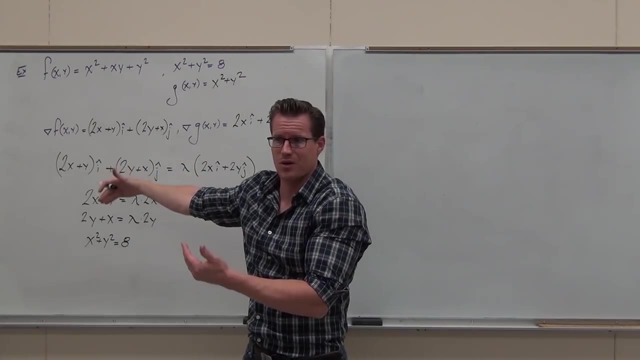 This one's not going to be that easy. There's a lot of algebra behind it. This was the easy part. Do you understand the idea behind this? That's pretty cool. right? We're setting gradients equal to a scalar multiple. It's called the Lagrange multiplier. 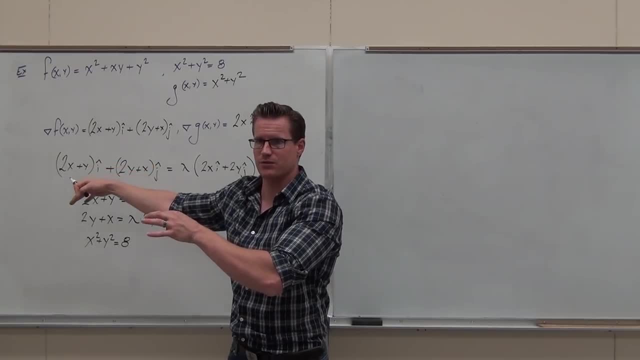 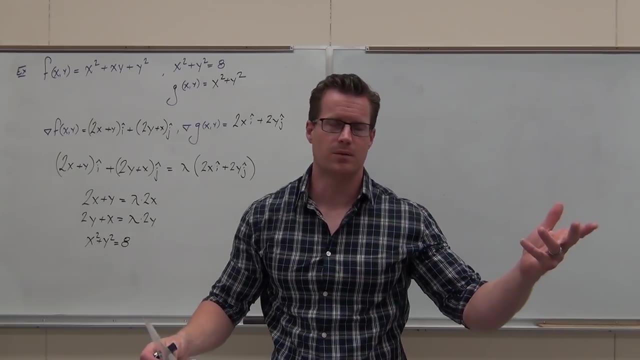 That's pretty much it. Our goal is to find that and then substitute back in to solve this thing. So we're going to do that, We're going to go very quickly. It's all algebra. The algebra in calculus, as you know, is the hard part. 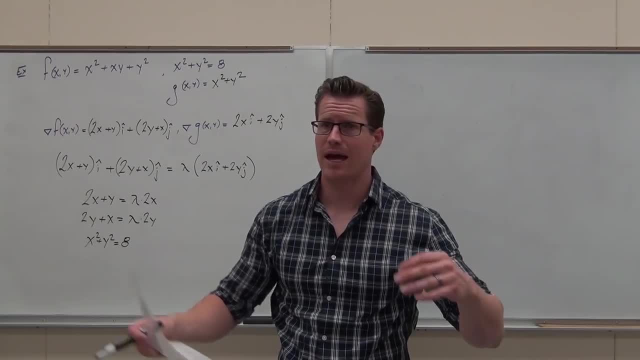 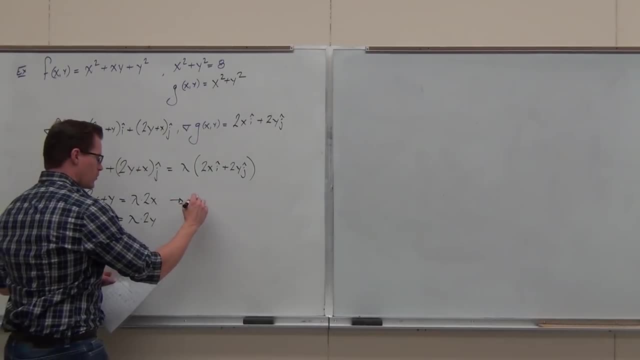 So I'm going to show you how to do it. I'm going to go fast, though. I'm not going to ask for a lot of comments or feedback. I'm just going to show you the technique here. So the technique, This one, I would solve for y. 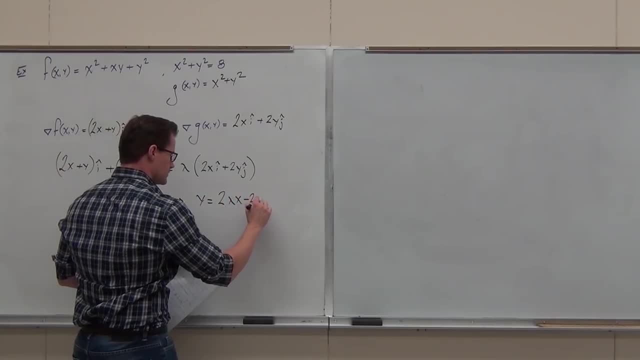 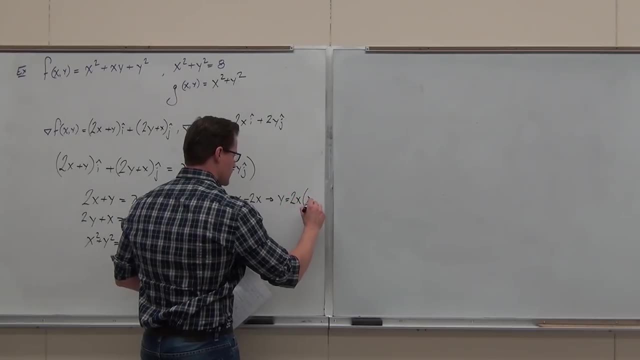 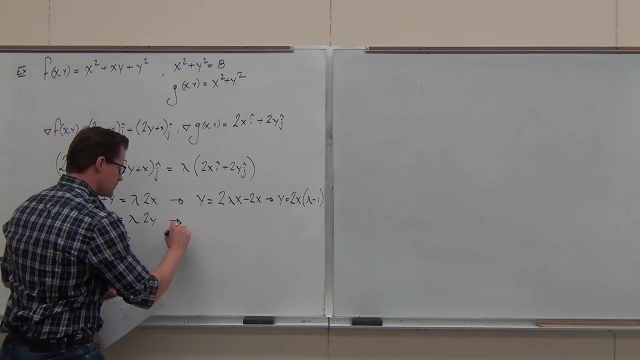 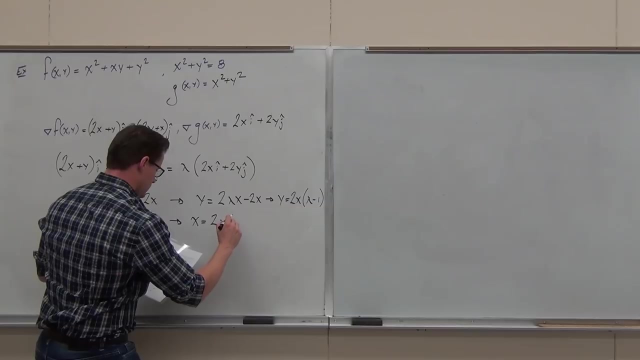 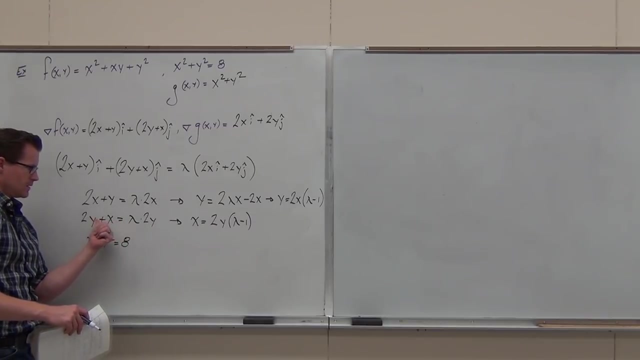 And I'm going to factor out 2x. So we get y equals 2x lambda minus 1.. This one I'm going to solve for x. If we do that, we get what we get. We get this: Solve for x: subtract the 2y factor in the same version. 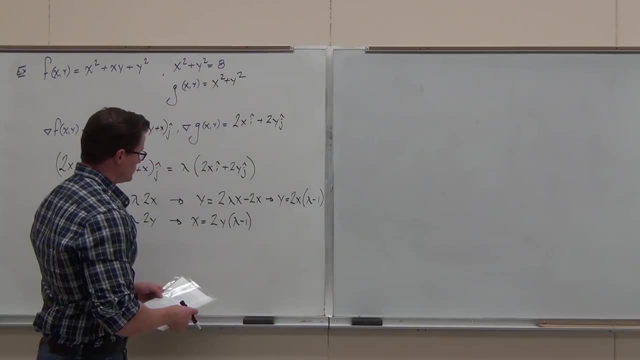 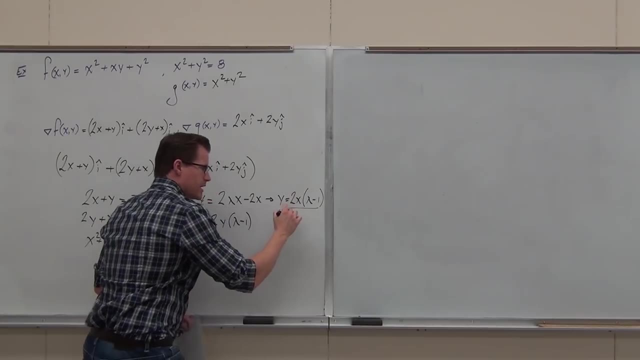 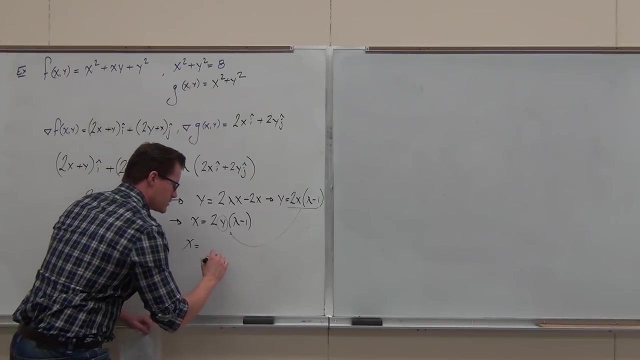 You guys understand the algebra on that one Now. now I have to get rid of one of these variables, It doesn't matter which, But I'm going to take this and substitute in for the y here. So x equals 2 times 2x lambda minus 1.. 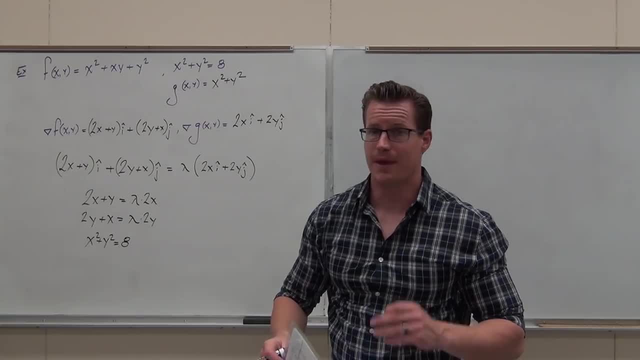 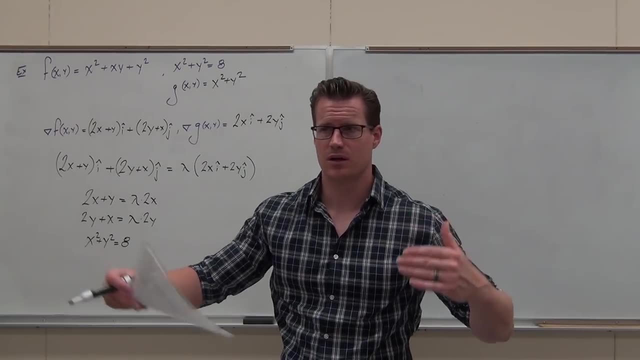 We're going to go very quickly. It's all algebra. The algebra in calculus, as you know, is the hard part, So I'm going to show you how to do it. I'm going to go fast, though I'm not going to ask for a lot of comments or feedback. 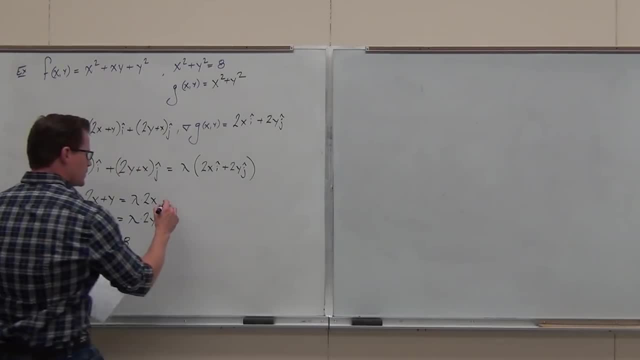 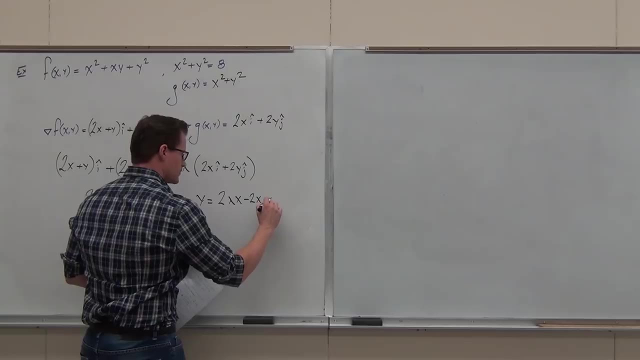 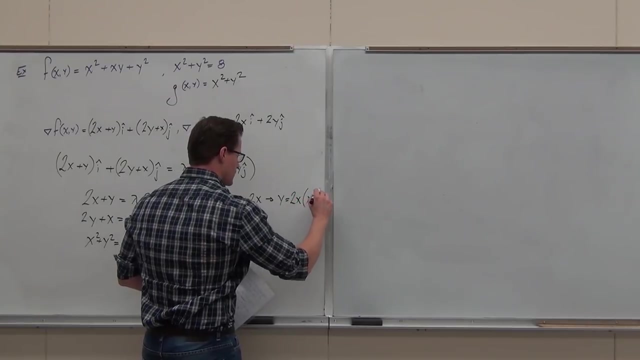 I'm just going to show you the technique here. So the technique, This one I would solve for y, And I'm going to factor out 2x, So we get y equals 2x lambda minus 1.. This one I'm going to solve for x. 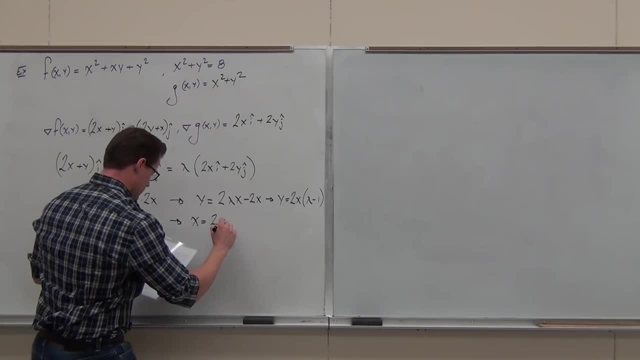 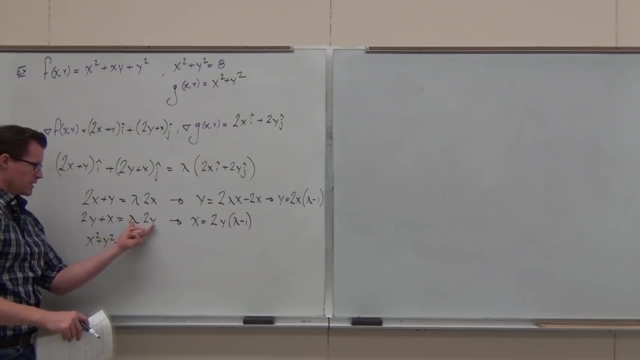 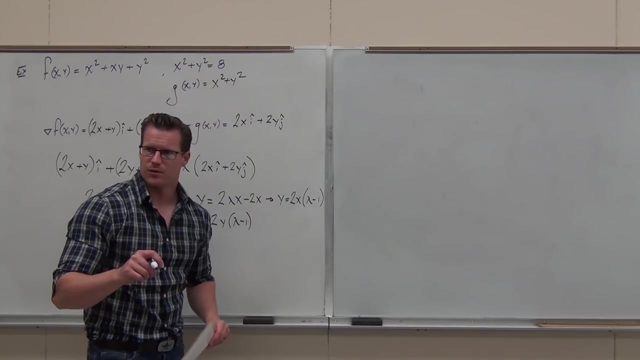 If we do that, we get this Solve for x subtract the 2y factor in the same version. You guys understand the algebra on that one. Now I have to get rid of one of these variables, It doesn't matter which. 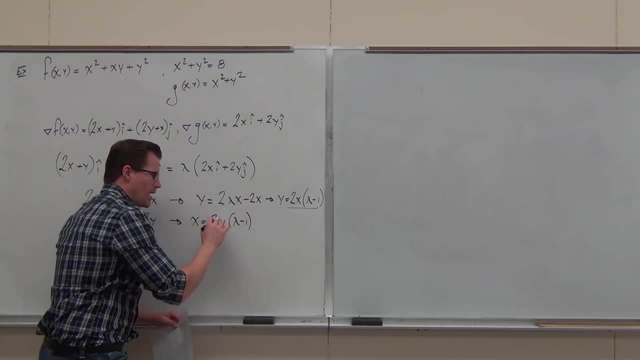 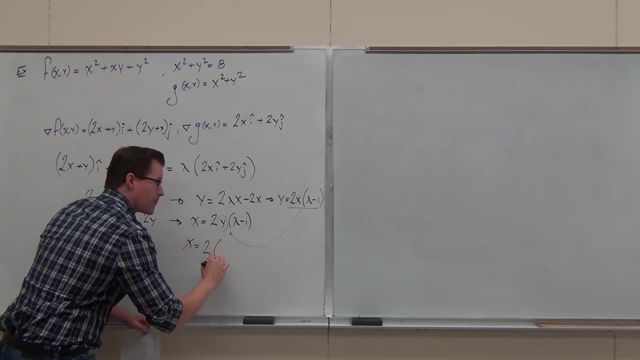 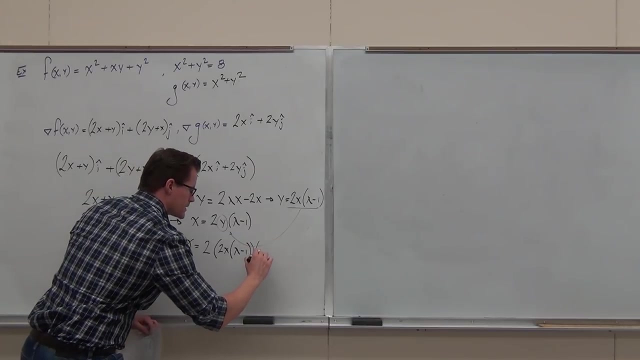 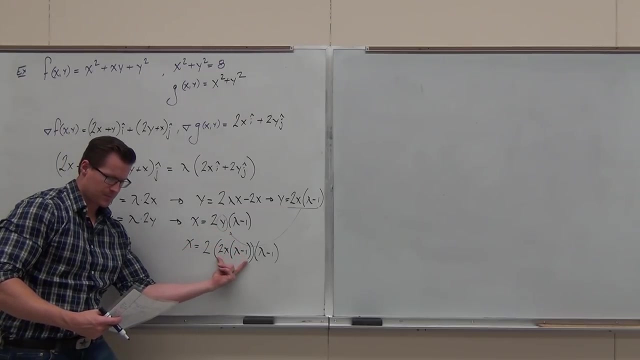 But I'm going to take this and substitute in for the y here. So x equals 2 times 2x. lambda minus 1 times lambda minus 1.. Here's the 2.. Here's the y. Here's the lambda minus 1.. 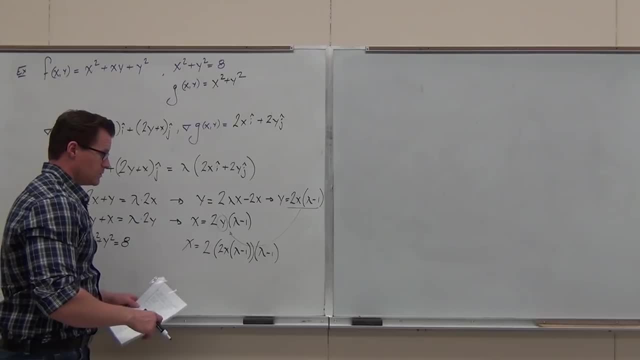 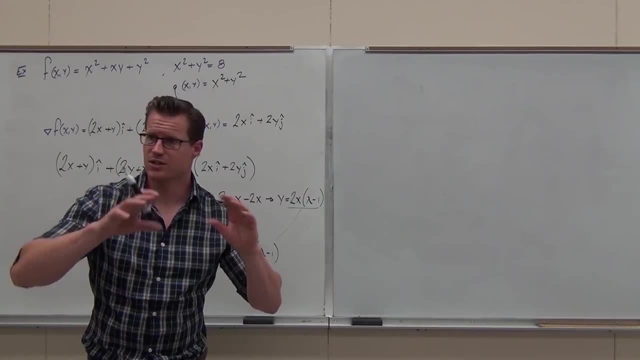 Can you follow that Okay? So what we're going to do, Since we have one variable now, I'm going to distribute, I'm going to get 0 on one side And I'm going to use the zero product property to figure out some values here. 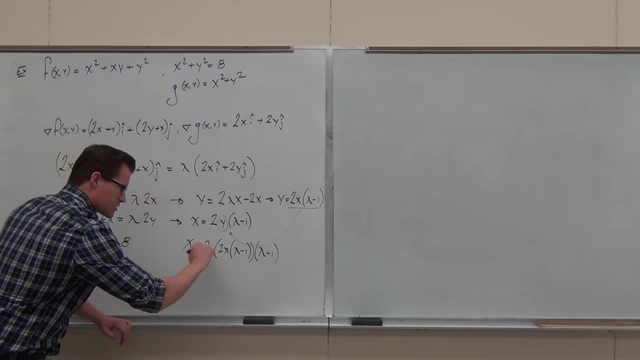 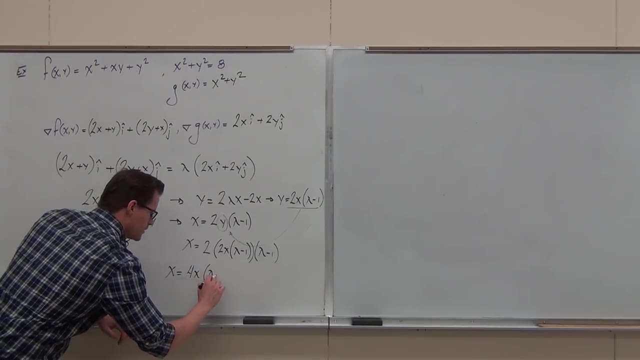 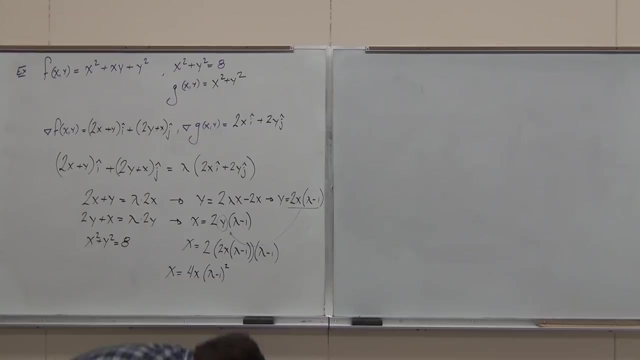 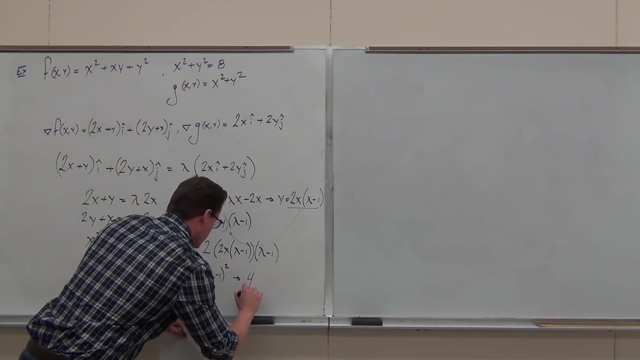 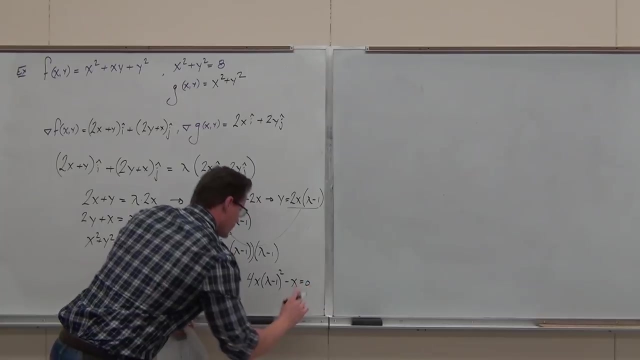 So let's go ahead and let's at least distribute this. So I have 4x lambda minus 1 squared And if I move everything to one side, we're going to have this 4x lambda minus 1 squared. minus x equals 0.. 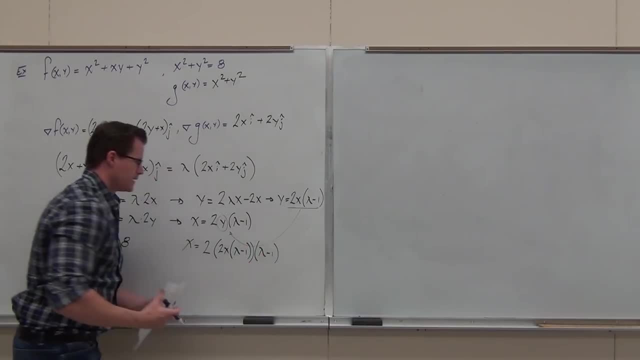 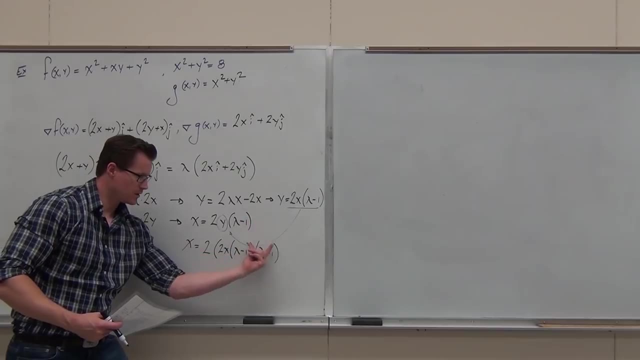 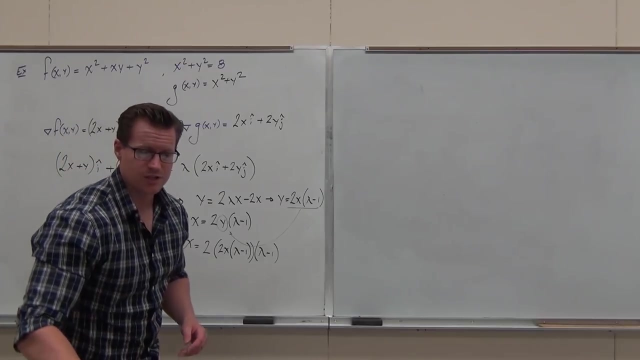 Here's the 2, here's the y, here's the lambda minus 1.. Can you follow that? Okay, So what we're going to do, since we have one variable now, I'm going to distribute. I'm going to get 0 on one side and I'm going 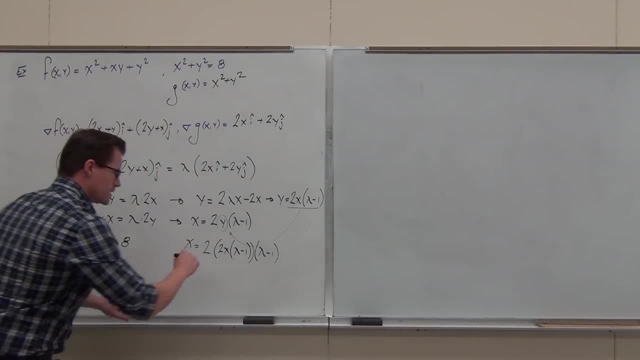 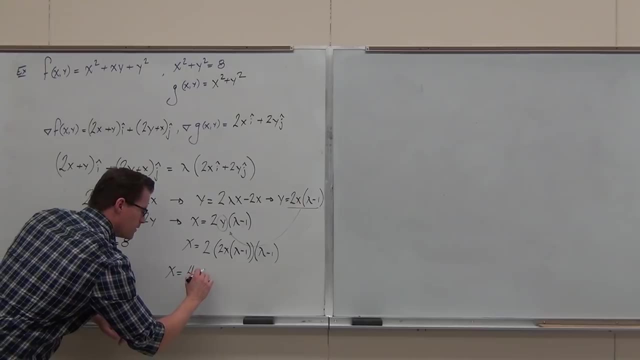 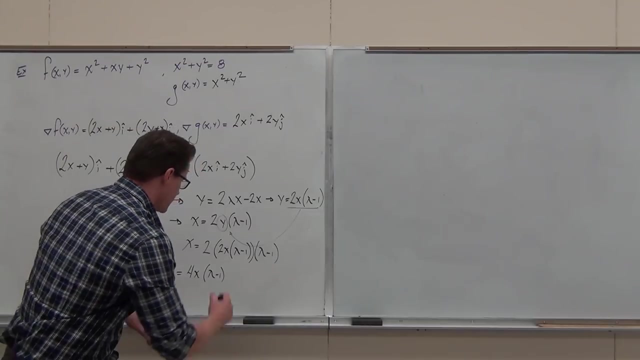 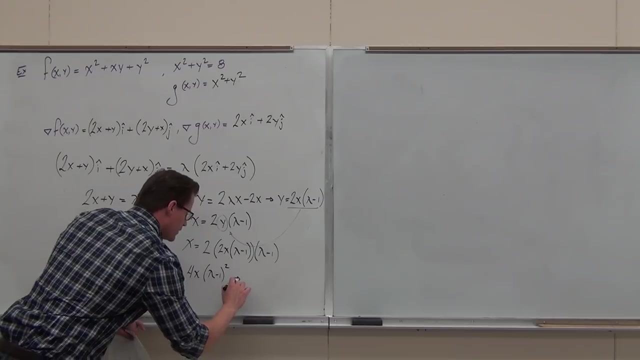 to use the zero product property to figure out some values here. So let's go ahead and let's, let's, let's at least distribute this. So I have 4x lambda- oops, lambda- minus 1 squared, And if I move everything to one side, we're going to have this: 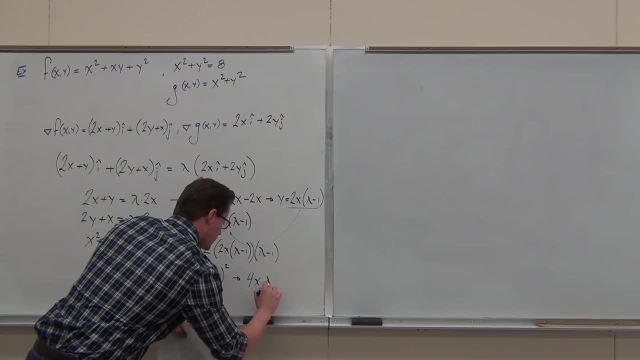 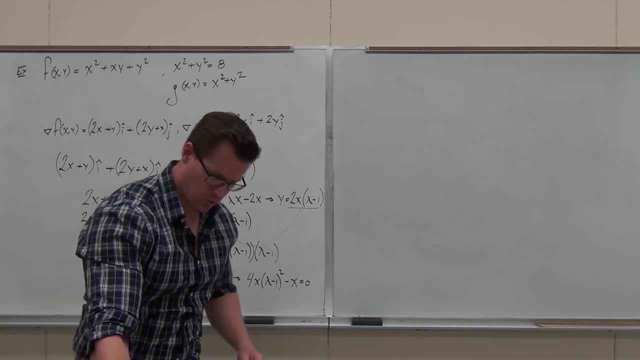 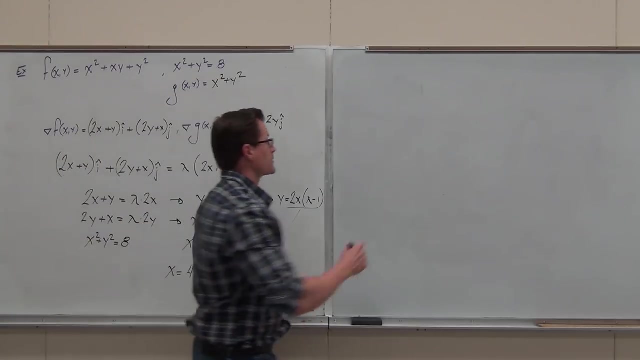 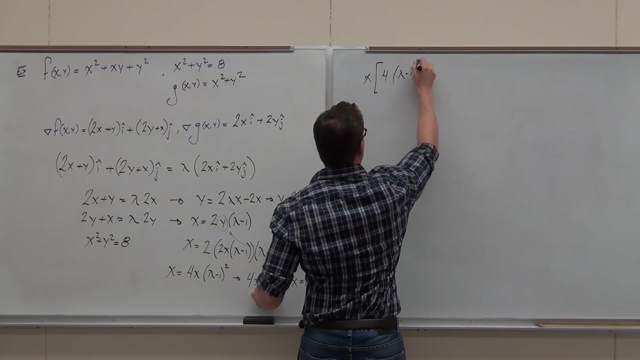 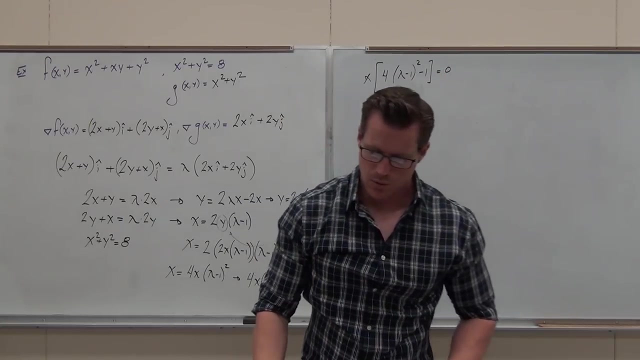 4x lambda minus 1. squared minus x equals 0, and that's the key. That's what I want. If I factor out the x, if I factor out the x, we're left with that. Listen, I do want to move fast, but I don't want to leave you behind algebraically. 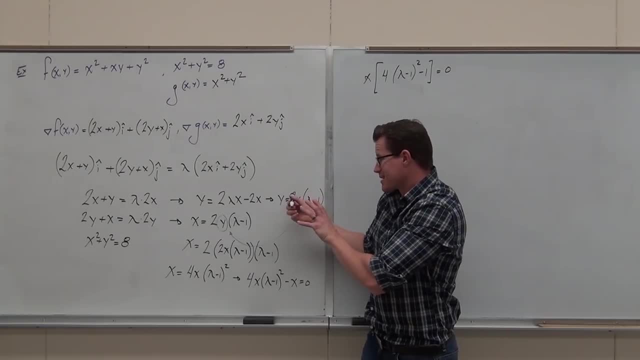 Are you guys okay on the? it's a horrible substitution, but it's kind of a basic substitution. Solving for y substitute in after you solve for x, You guys get that. Hey, that's fine, That's fine. 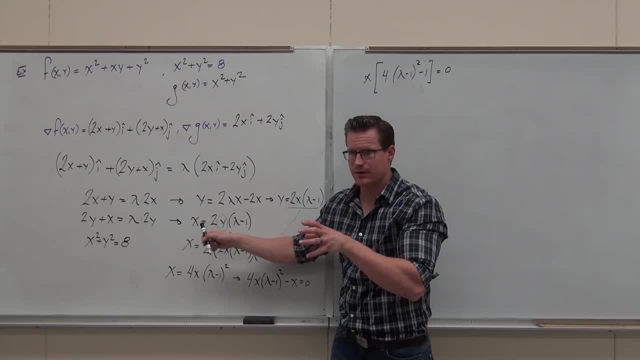 That's the system. You can do it. Our goal is to solve lambda. That's what I want. Now. I still have some x's in here, so I'm going to get everything on one side. I'm going to distribute. 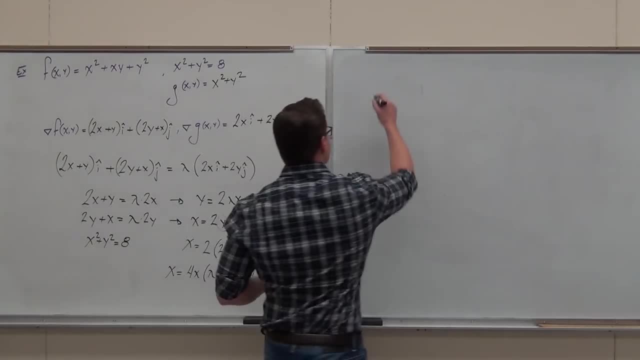 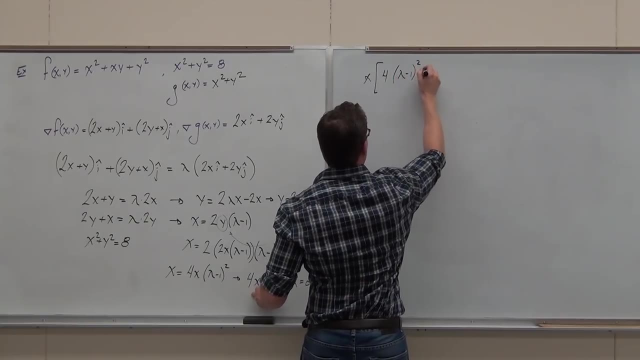 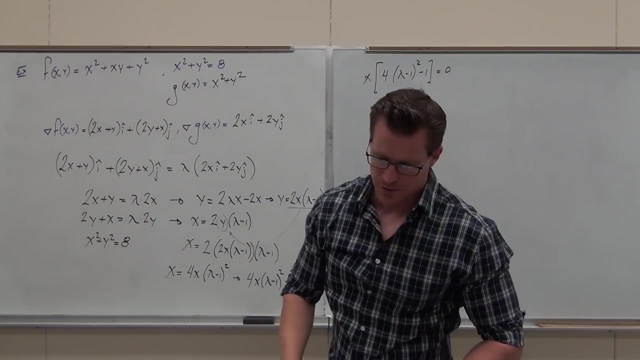 And that's the key. That's what I want. If I factor out the x, If I factor out the x, we're left with that. Listen, I do want to move fast, But I don't want to leave you behind algebraically. 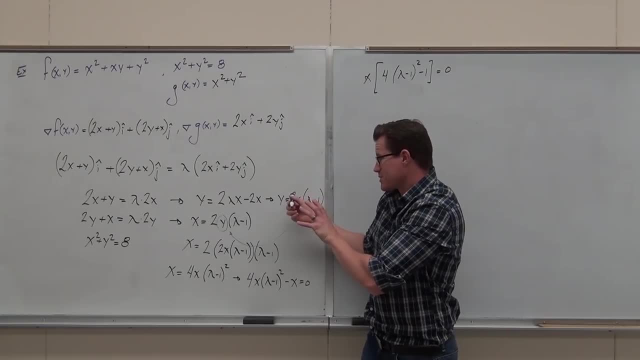 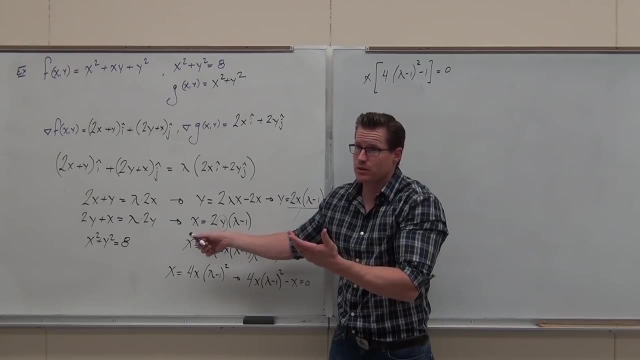 Are you guys okay on the? It's a horrible substitution, But it's kind of a basic substitution. Solving for y substitute in After you solve for x, You guys get that. Hey, that's a system, You can do it. 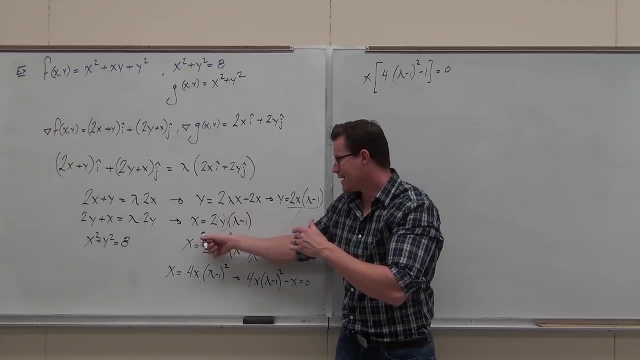 Our goal is to solve lambda. That's what I want. Now. I still have some x's in here, So I'm going to get everything on one side. I'm going to distribute. I'm going to get everything on one side. 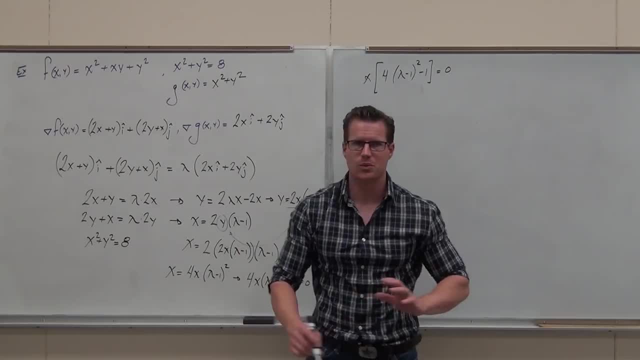 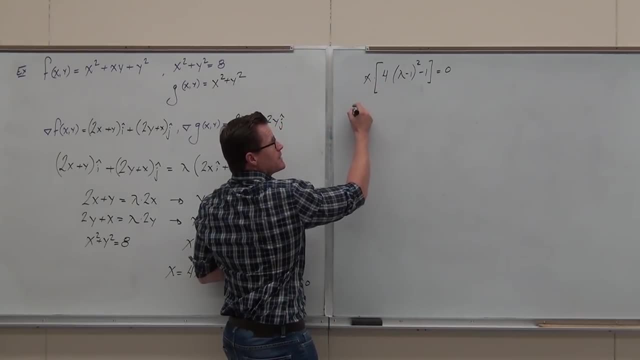 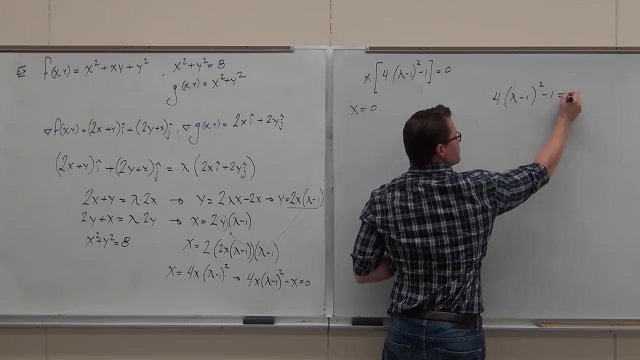 So 4x lambda minus 1, squared minus x. I'm going to factor the x away Now because that's a product, And this is a product of two things equal to 0.. I know we have two cases: Either x equals 0 or 4 lambda minus 1, squared minus 1 equals 0.. 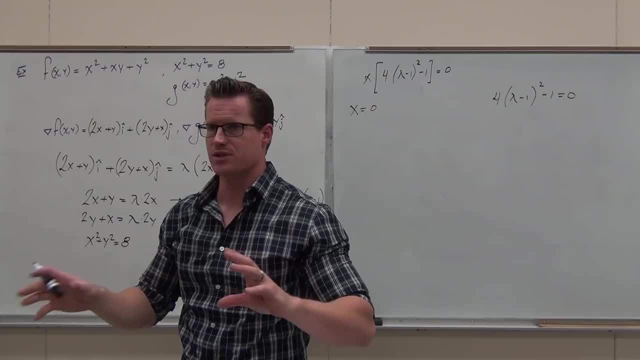 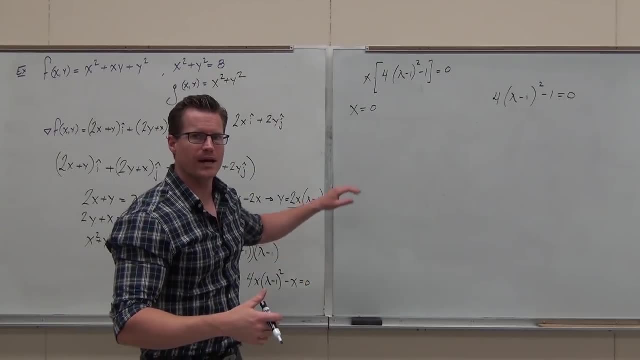 That's got to be the case. One of those two things has to be the case for us to get this equal to 0. Does that make sense? Now, here's the issue. I want to backtrack with this one, so you understand that this is irrelevant. 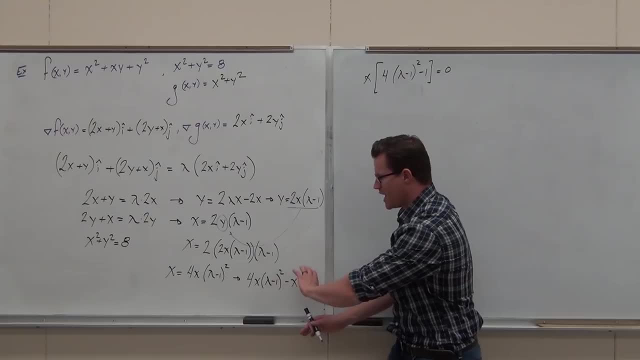 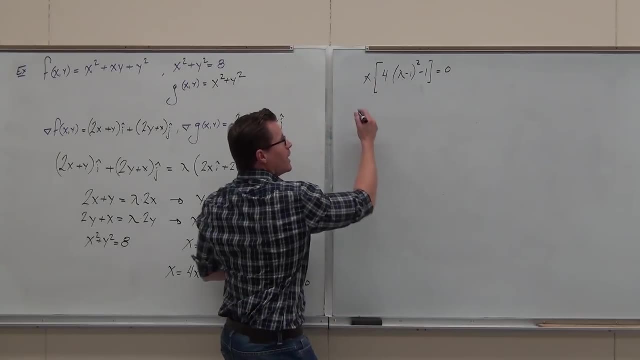 I'm going to get everything on one side, so 4x lambda minus 1, squared minus x. I'm going to factor the x away Now, because that's a product and this is a product of two things equal to 0, I know. 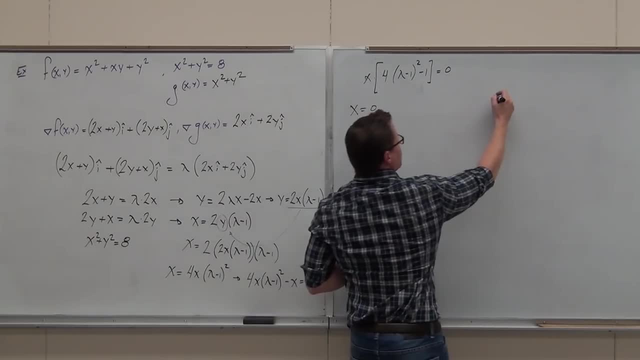 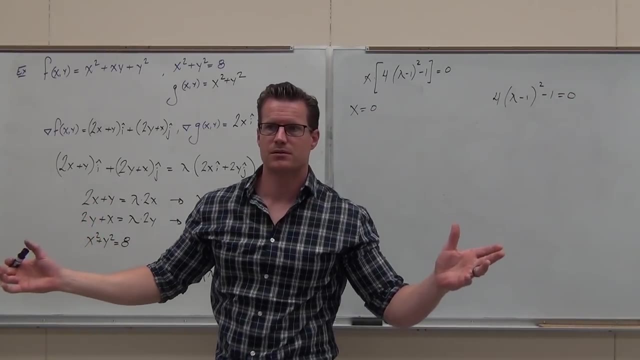 we have two cases: either x equals 0 or 4 lambda minus 1, squared minus 1 equals 0. That's got to be true. That's got to be the case. One of those two things has to be the case for us to get this equal to 0.. 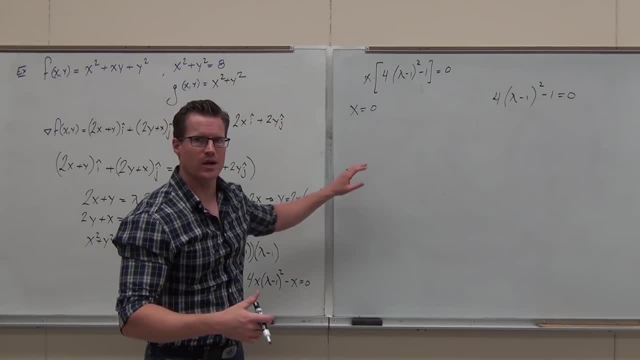 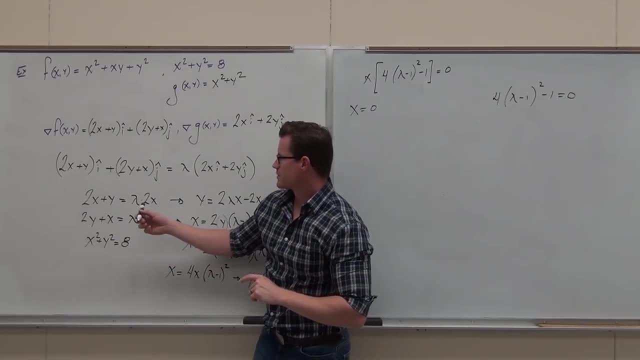 Does that make sense? Now, here's the issue. I want to backtrack with this one, so you understand that this is irrelevant. Here's why: If I let x equal 0,, if I let x equal 0, then 0 and 0 means y would also equal 0.. 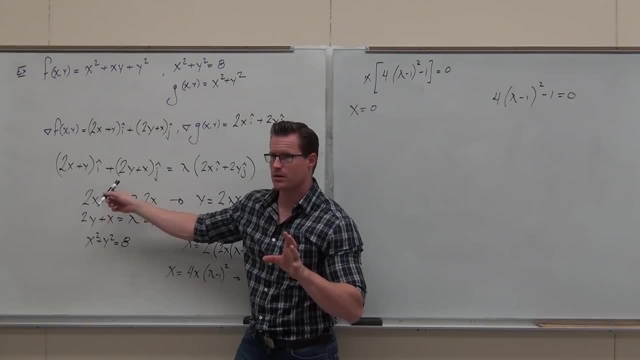 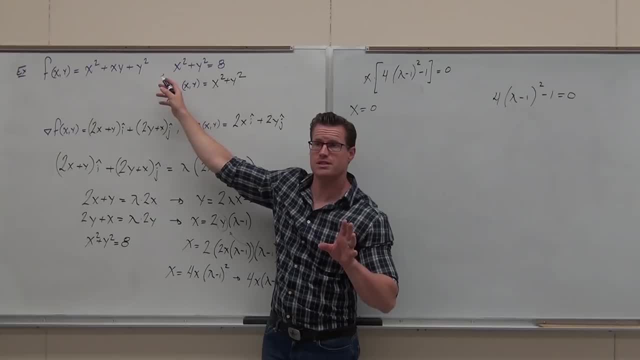 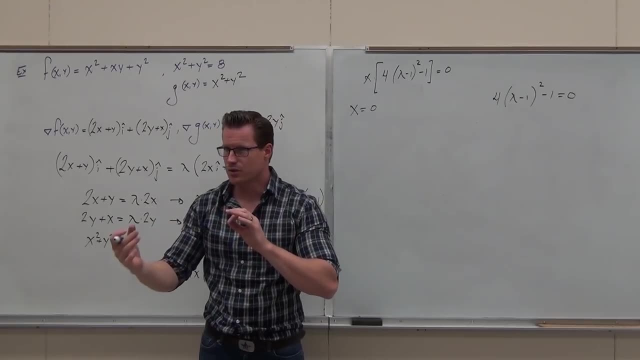 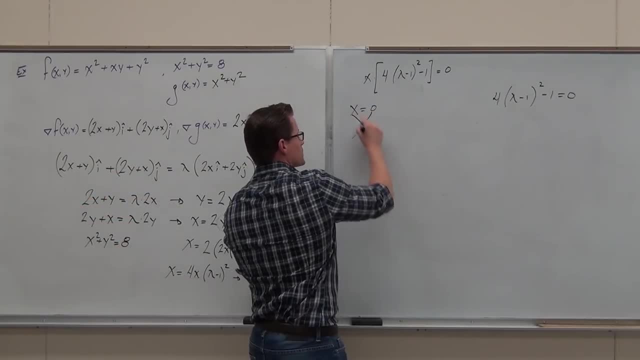 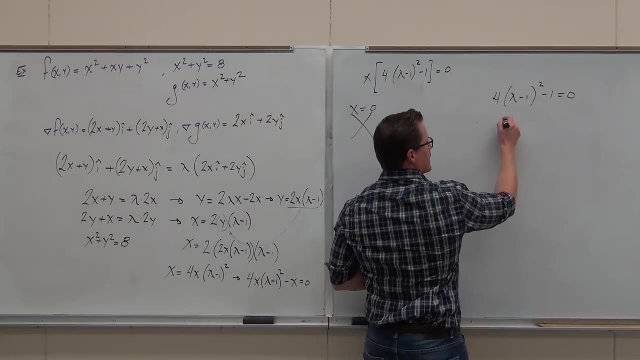 Plug in: x equals 0, y is also 0, you go: uh no, This one is no good, This guy, I told you from the beginning: solve for lambda. You have to solve for lambda. If we do, we have lambda minus 1 squared equals positive 1. fourth: 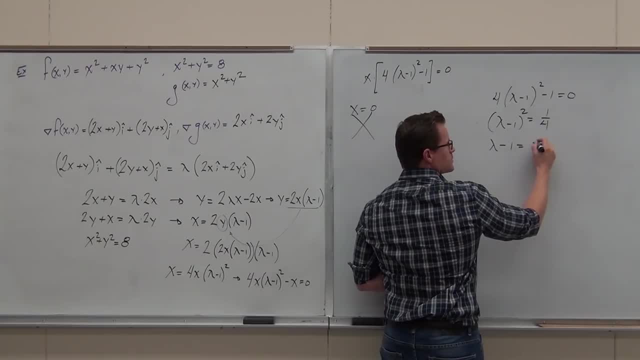 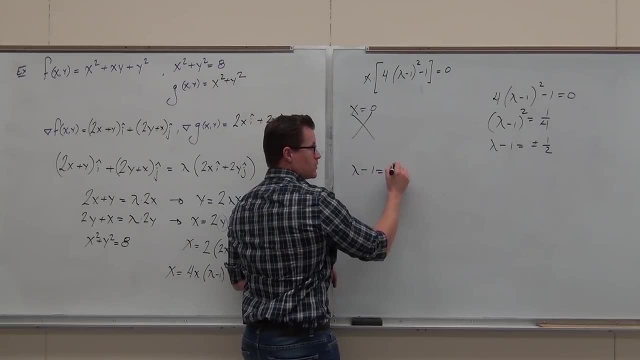 If we take a square root, we get lambda minus 1.. equals plus or minus 1 half. if we take this and separate it, lambda minus 1 equals 1 half and lambda minus 1 equals negative 1 half. if we add 1, we get 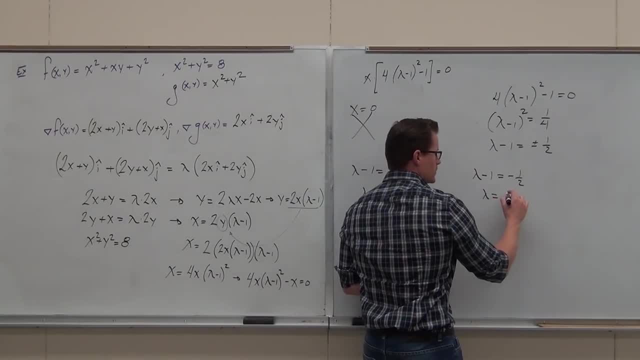 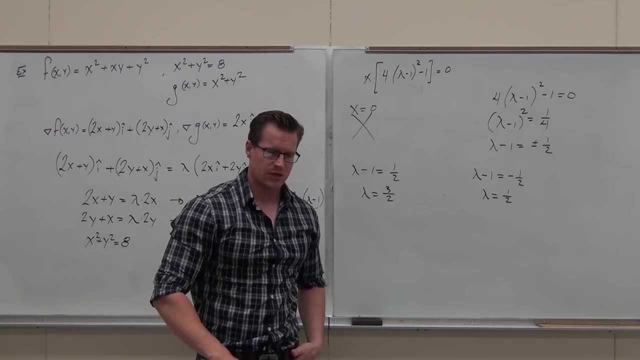 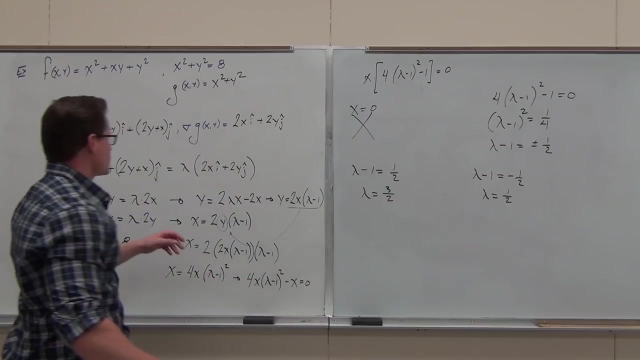 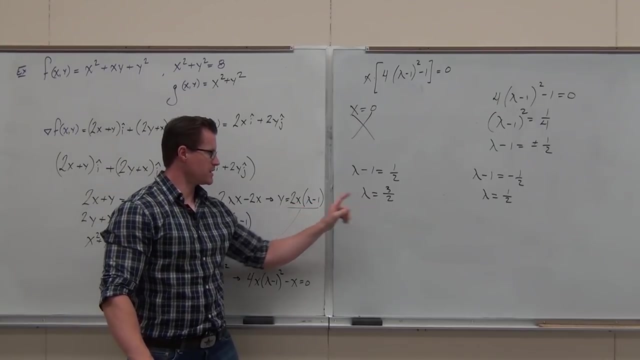 lambda equals 3 halves and we get lambda equals 1 half. you guys okay with that? okay now? now, since we have something that gives us X is something that relates X's to Y's, we're going to take each of these and plug them in for lambda. it's going to give us a as an equation, so let's use 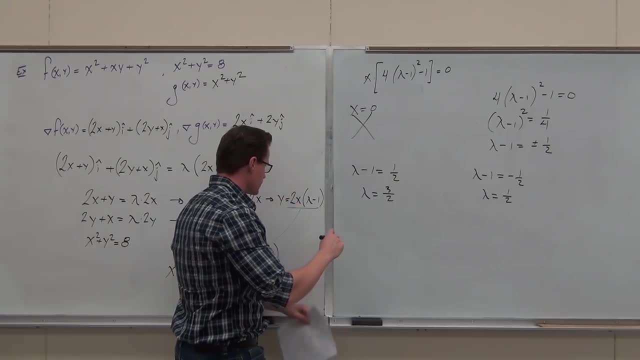 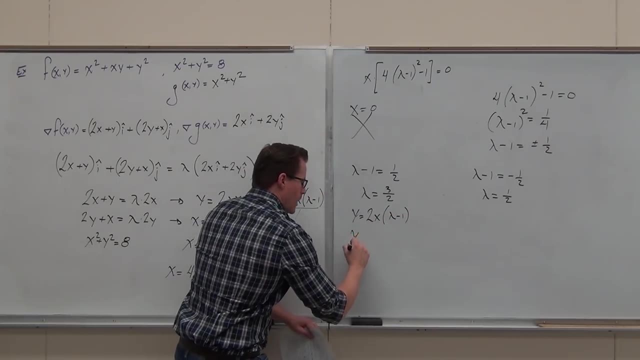 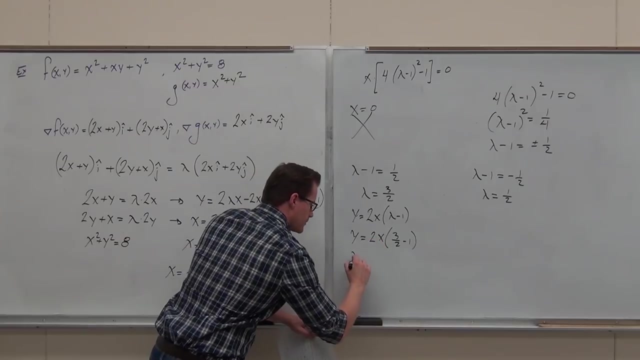 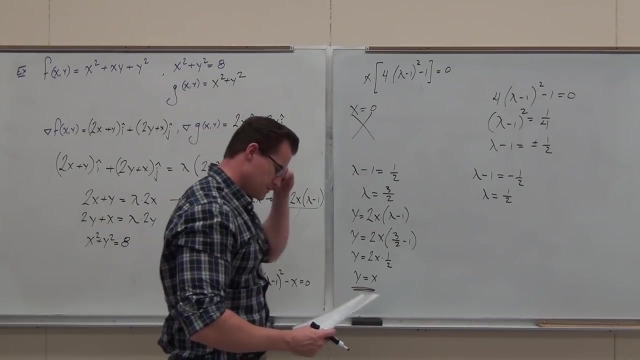 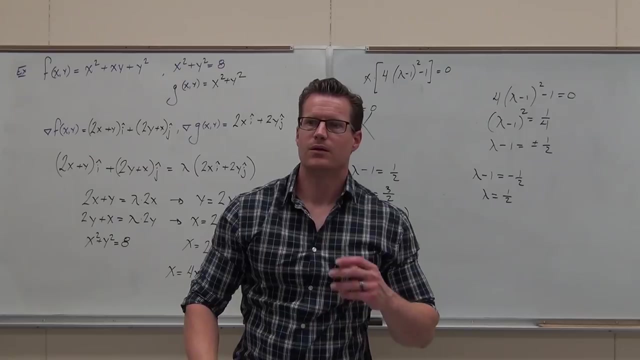 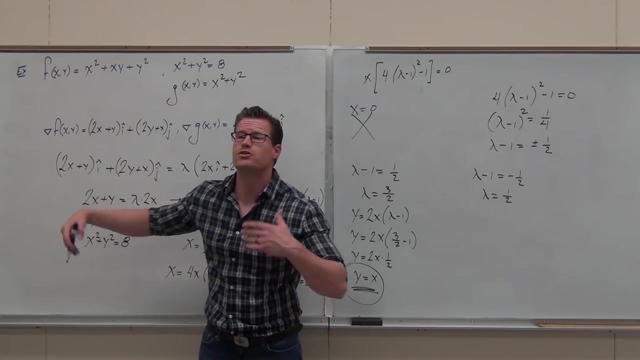 let's use this one: Y equals 2x. 3 halves minus 1, that's 1 half. Y equals X. this is where it's going to get fun. what that does? that gives you a substitution to plug into this constraint. so we've done all this work to find a substitution to plug into that. 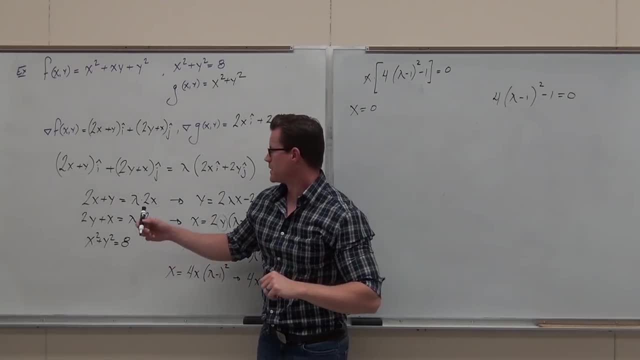 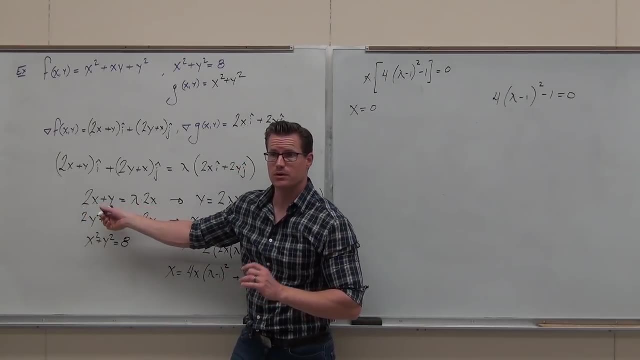 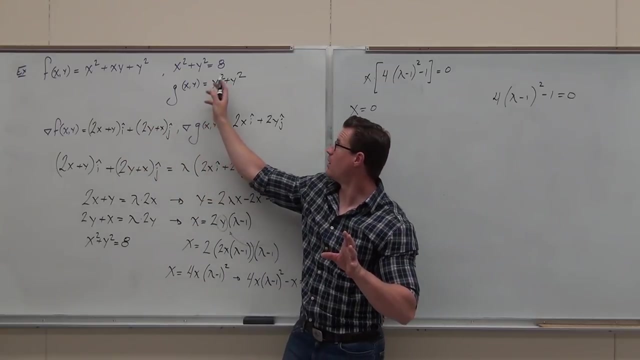 Here's why: If I let x equal 0, then 0 and 0 means y would also equal 0. Do you see that Then x equals 0 and y equals 0.. Is that on our constraint? No, Because 0 plus 0 does not equal 8.. 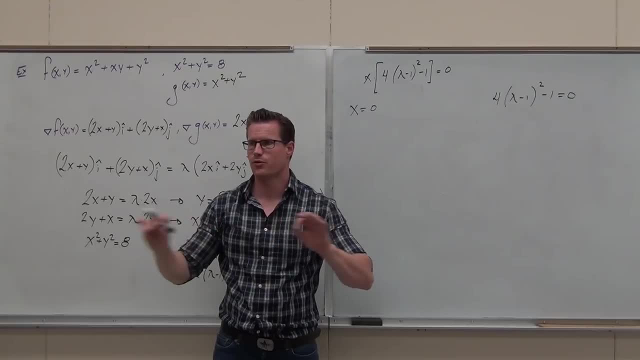 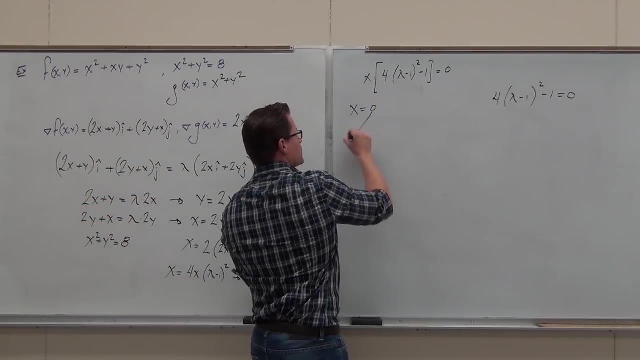 So x equals 0.. x equals 0 does not lead anywhere. for us, It's an invalid solution because it's not on our constraint. Plug in: x equals 0.. y is also 0.. You go no, This one is no good. 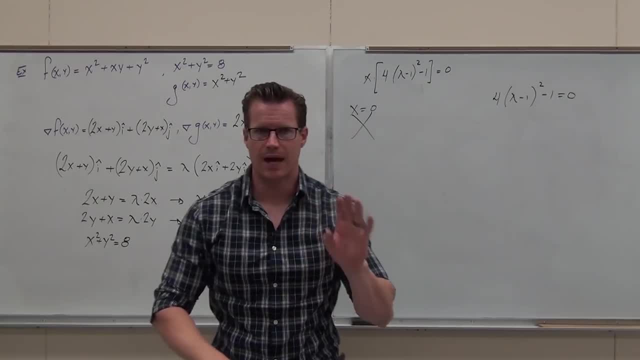 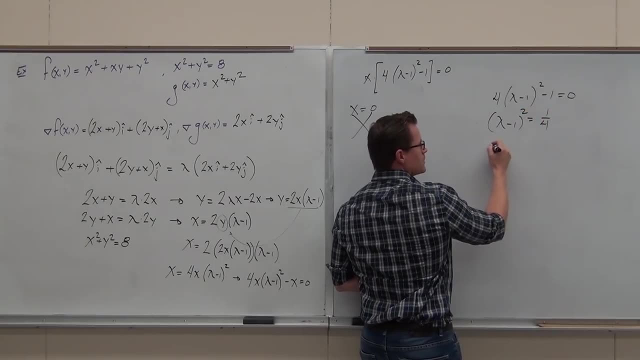 This guy. I told you from the beginning: solve for lambda. You have to solve for lambda. If we do, we have lambda minus 1 squared equals positive 1. fourth, If we take a square root, we get lambda minus 1 equals plus or minus 1 half. 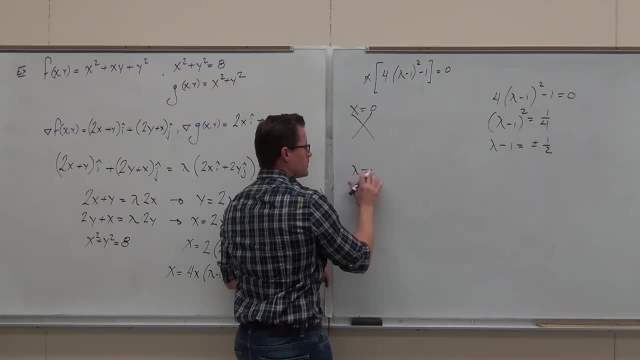 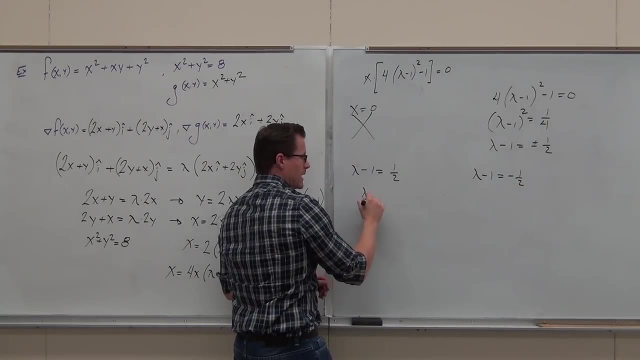 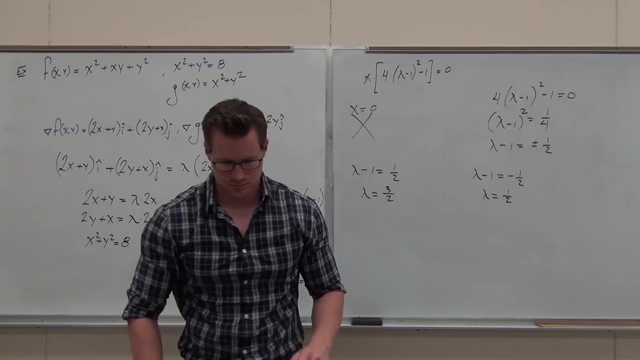 If we take this and separate it, we get lambda minus 1 equals 1 half and lambda minus 1 equals negative 1 half. If we add 1, we get lambda equals 3 halves and we get lambda equals 1 half. 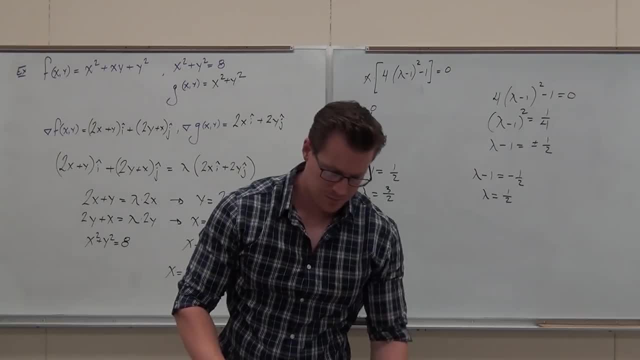 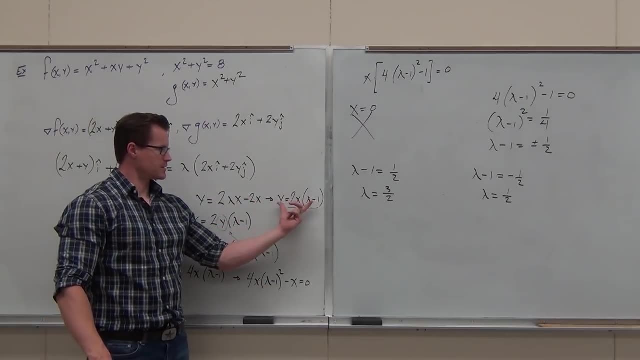 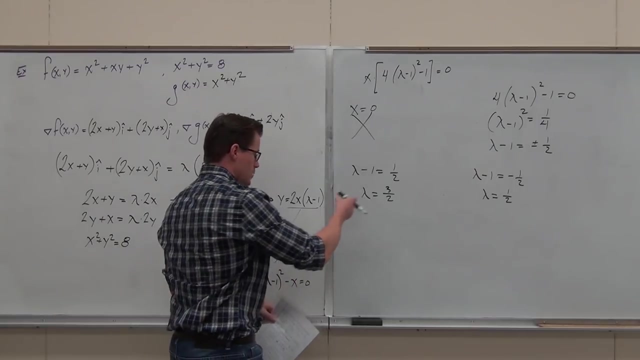 You guys okay with that? Okay Now. now, since we have something that gives us x's, something that relates x's to y's, we're going to take each of these and plug them in for lambda. It's going to give us an equation. 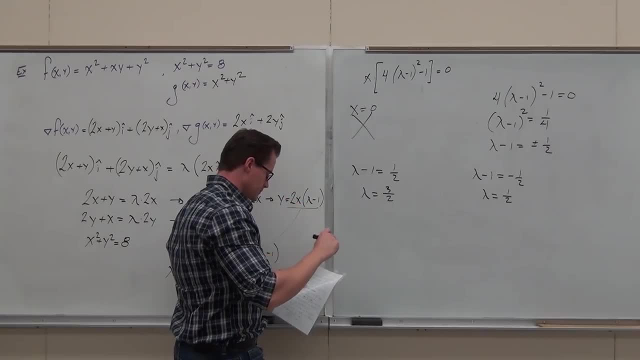 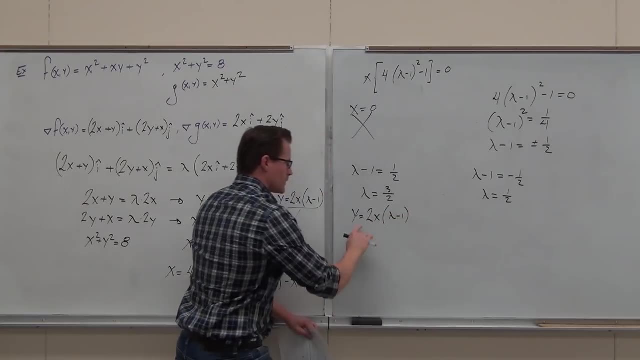 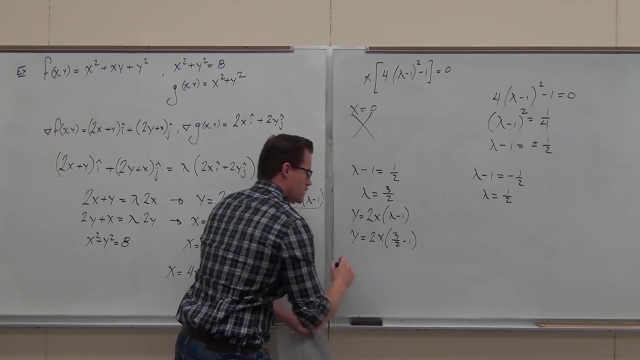 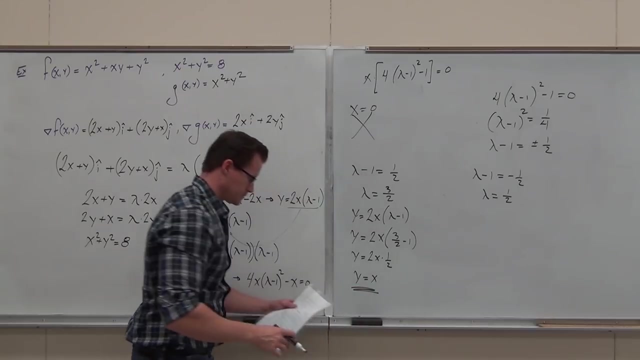 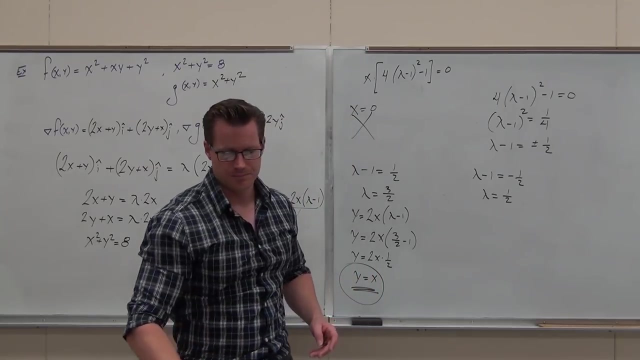 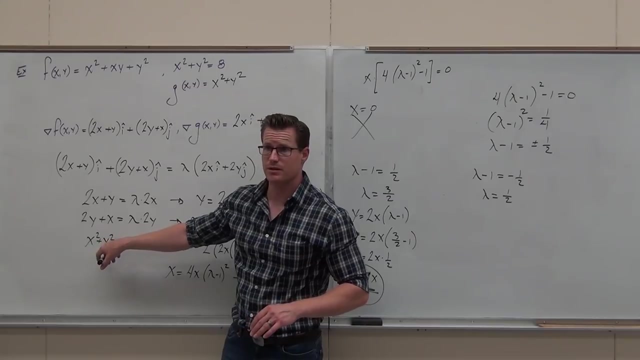 So let's use this one: y equals 2x, 3 halves minus 1.. That's 1 half y equals x. This is where it's going to get fun. What that does? that gives you a substitution to plug into this constraint. 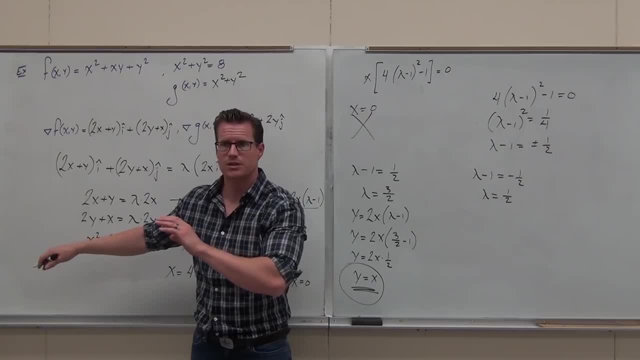 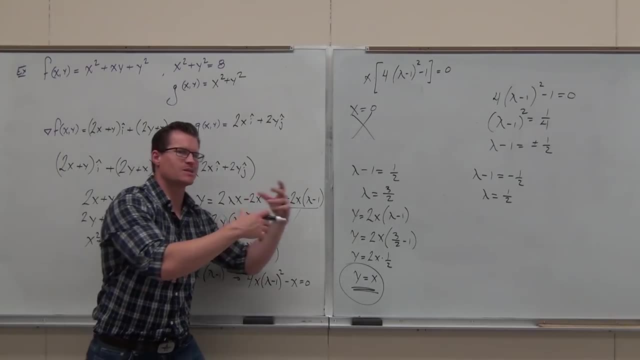 So we did all this work to find a substitution to plug into that constraint. So we go: yeah, find lambda great, Plug it in. What it tells you is not an actual value of x. It tells you a substitution for x or y. 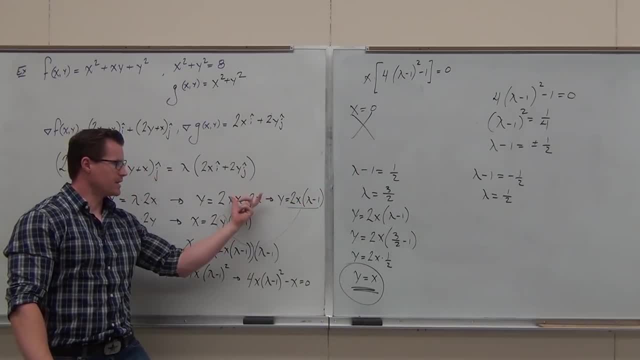 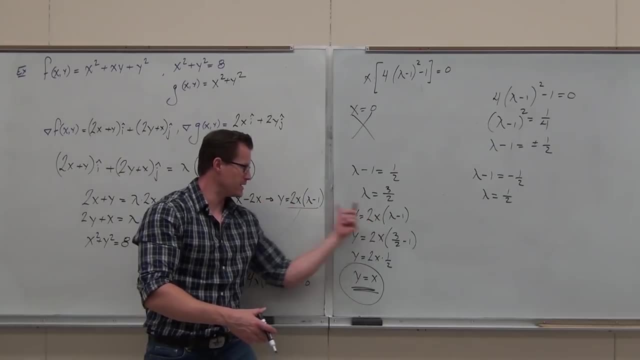 constraint. so go, if I'm the grave, plug it in. what it tells you is not an actual value of X. it tells you a substitution for x or y. this is yeah, plug it. plug it in here. that's exactly we did. it's great here this, like there. plug it in its. 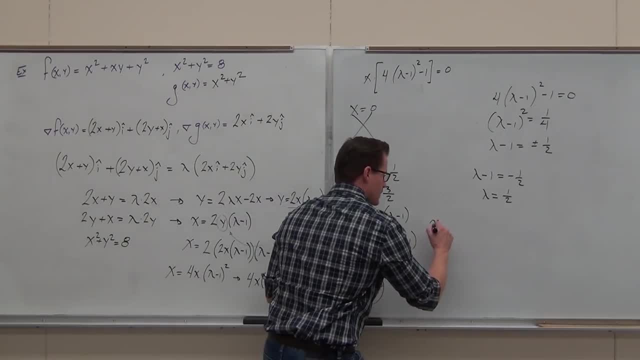 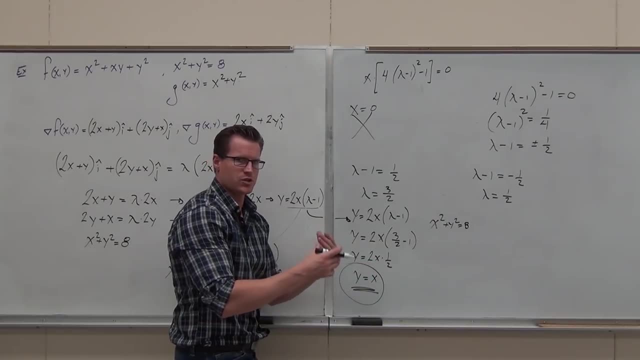 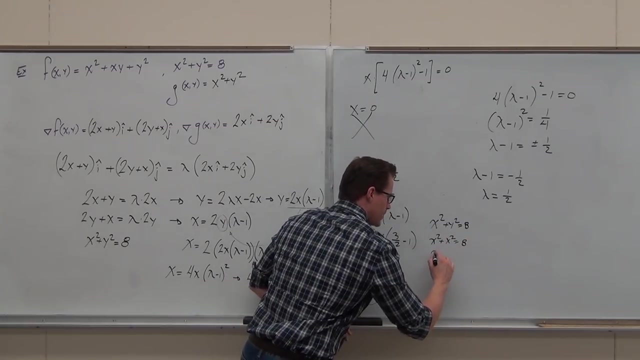 tongue you: Y equals X. now we take that and we said: whatever you want, choose X equals wire wipe was exit. I'm behind, want to pick the right answer. that I mean because I'm only going to let this rule rule. there says like a mode: I'm going to choose y equals x, then x squared plus x squared equals 8, 2x squared equals 8, x equals plus or minus 2.. 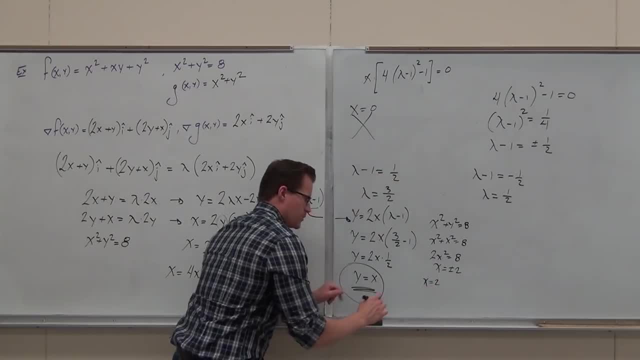 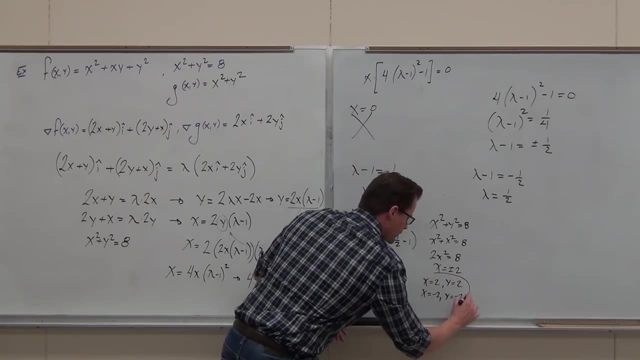 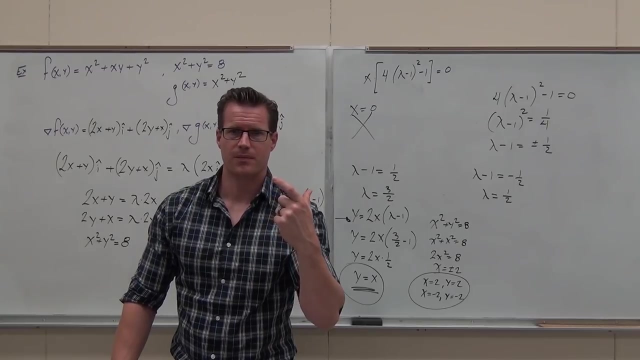 If x equals 2, then y equals 2.. If x equals negative 2, then y equals negative 2.. Those right, there are two points that will be either a maxima or minima. That's the plan. How much time do we got? 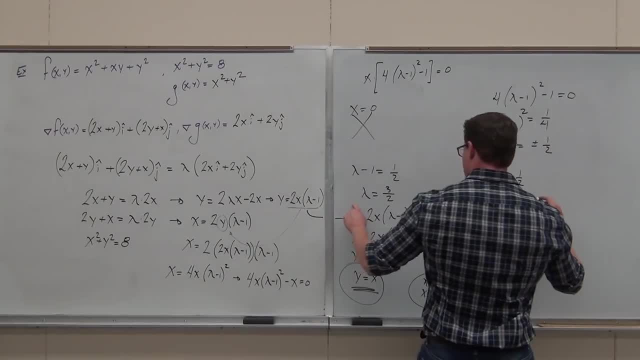 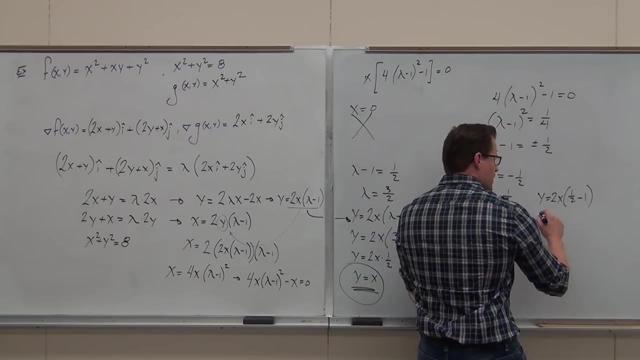 Four minutes left. Okay, We're going to do another one If I do the same thing. here. we got y equals 2x. now we're going to have 1 half minus 1.. All right, Well, that means that y equals 2x times negative 1 half. 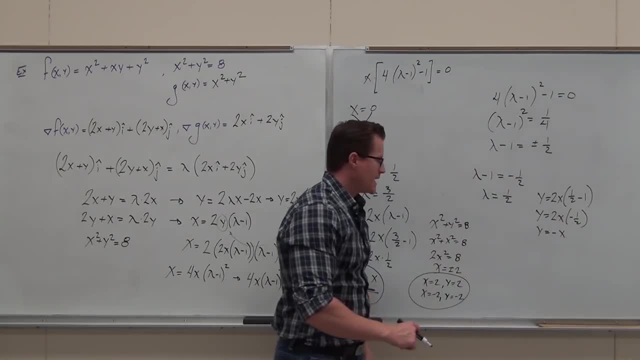 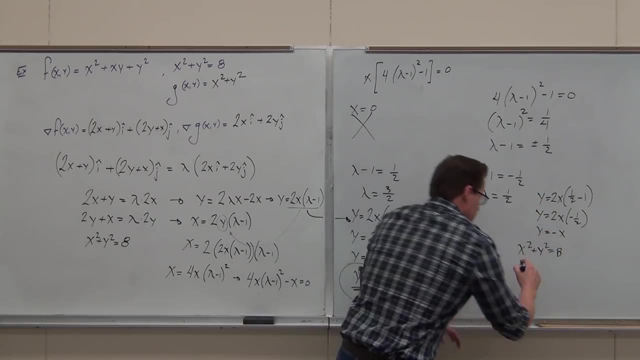 Well, that means that y equals negative x. However, if I take that and plug it in, x squared plus y squared equals 8, when I square a negative I get a positive. So it's still going to be: x squared plus y squared equals 8.. 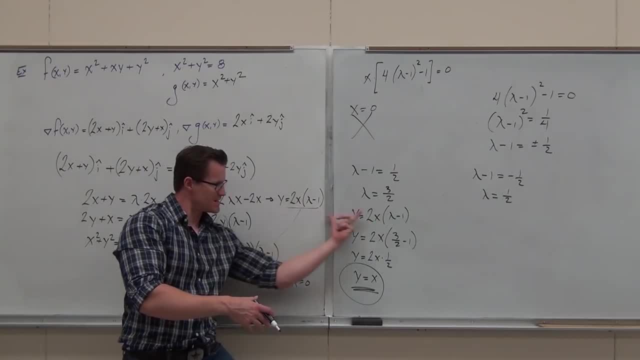 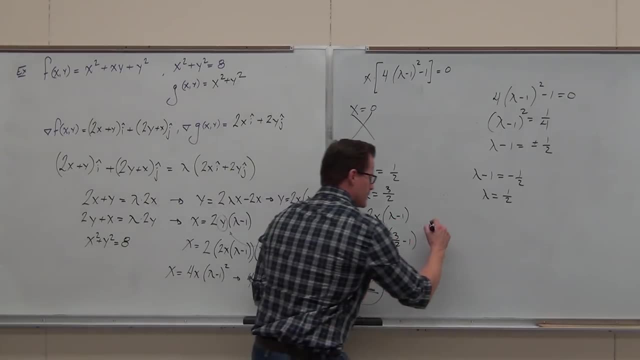 It says: yeah, plug it in here. That's exactly what we did. It's right here, This, Right there, Plug it in. It's telling you: y equals x. Now we take that and we substitute Whatever you want. 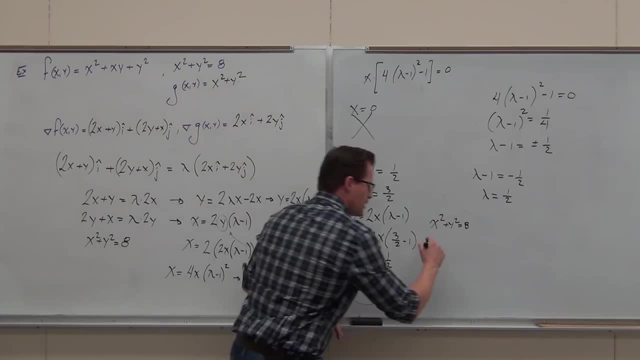 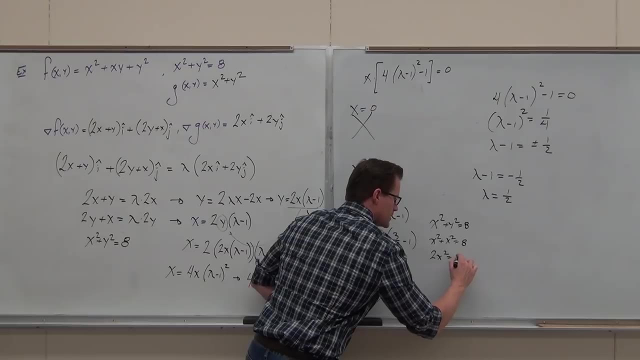 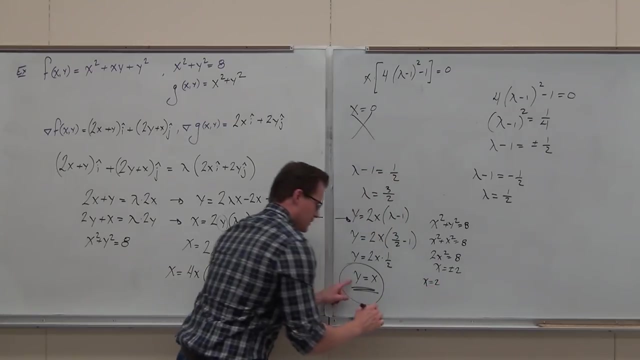 Choose x equals y or y equals x. I don't care, I'm going to choose y equals x, Then x squared plus x squared equals 8.. 2x squared equals 8.. x equals plus or minus 2.. If x equals 2, then y equals 2.. 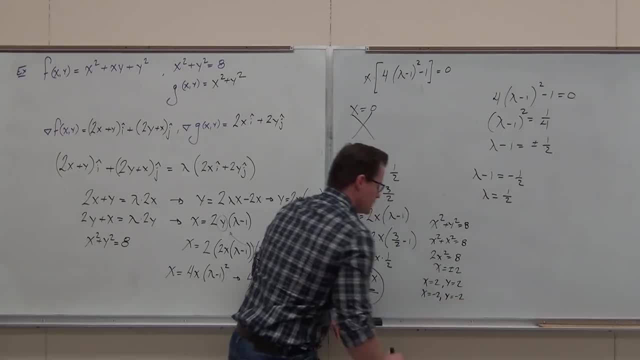 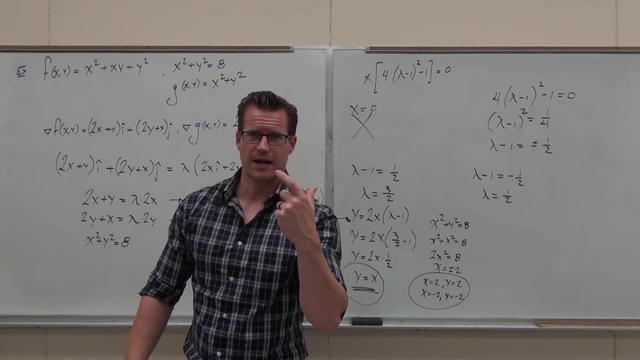 If x equals negative 2, then y equals negative 2.. Those right. there are two points that will be either a maxima or a minima. That's the plan. How much time do we got Four minutes left. OK, We're going to do another one. 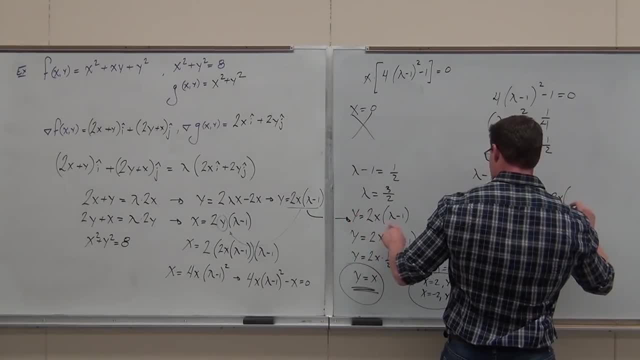 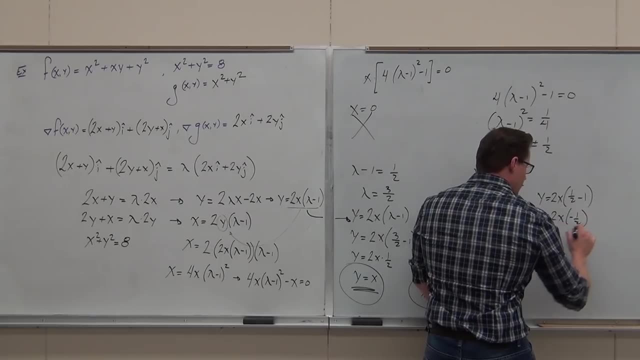 If I do the same thing here, we got y equals 2x. Now we're going to have 1 half minus 1.. All right, Well, that means that y equals 2x times negative 1 half. Well, that means that y equals negative x. 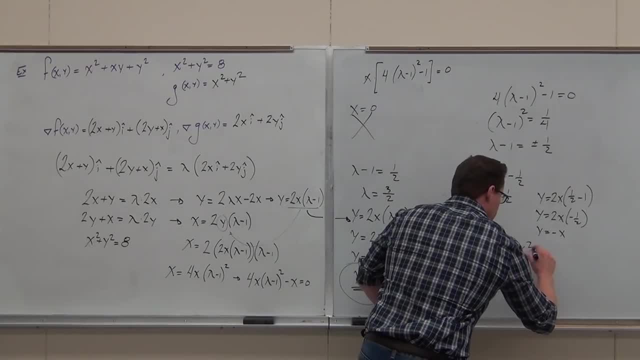 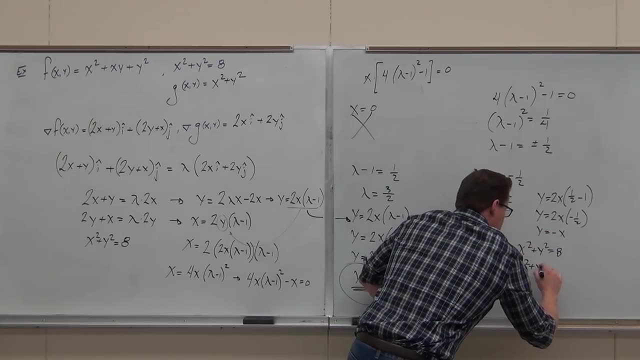 However, if I take that and plug it in, x squared plus y squared equals 8.. When I square a negative, I get a positive. So it's still going to be: x squared plus y squared equals 8.. It's going to be sorry. x squared plus x squared equals 8.. 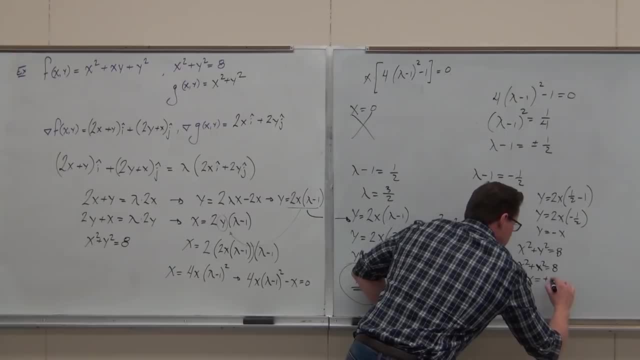 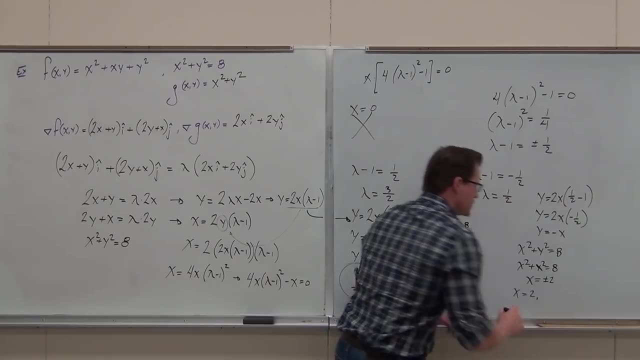 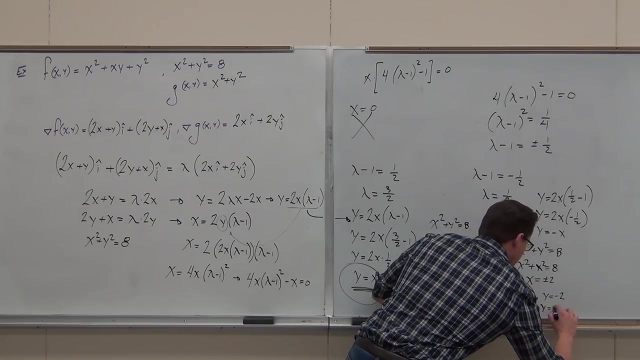 It's going to give the same thing: x equals plus 2 or minus 2.. However, if you go back to what we used for that, If x equals positive 2, y is the opposite sign, And if x equals negative 2,, then y is the opposite sign. 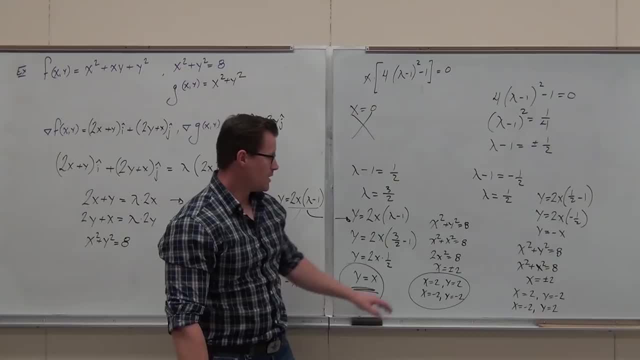 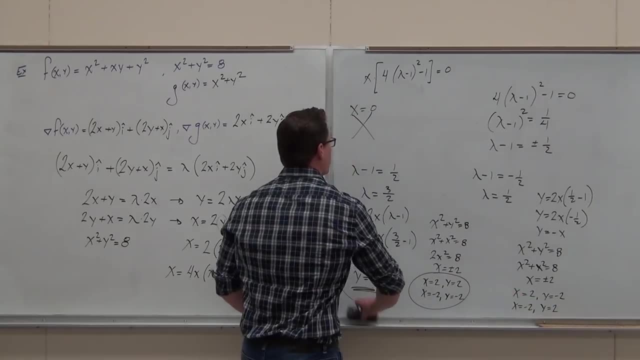 That's what that says. So we get some points that look awfully similar. We get the point 2, 2, negative, 2, negative 2.. 2, negative, 2, negative, 2, 2.. So out of those four points- I'm going to write them up here- 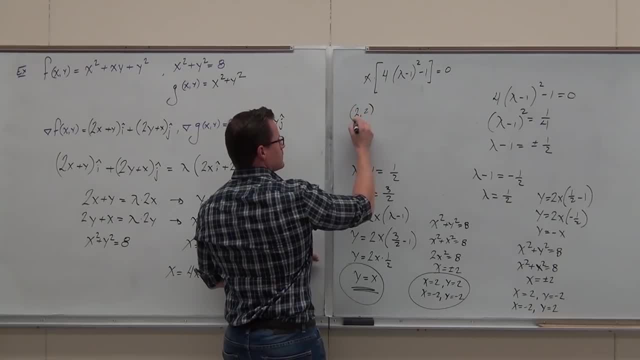 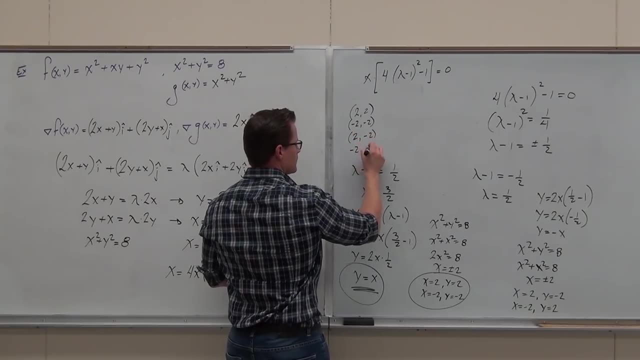 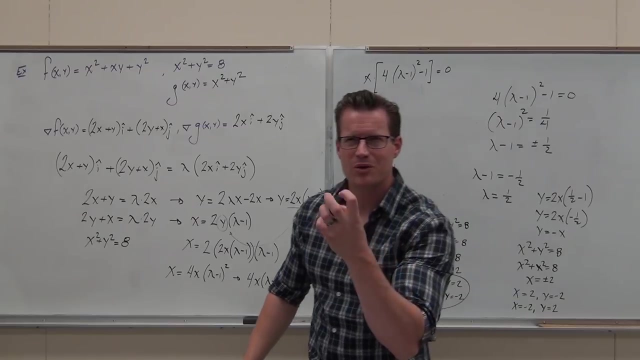 Out of those four points. You tell me this and then we'll be done. Out of those four points, how do you check them? Where do you put them to see which one's the biggest and which one's the smallest? Where do you do it? 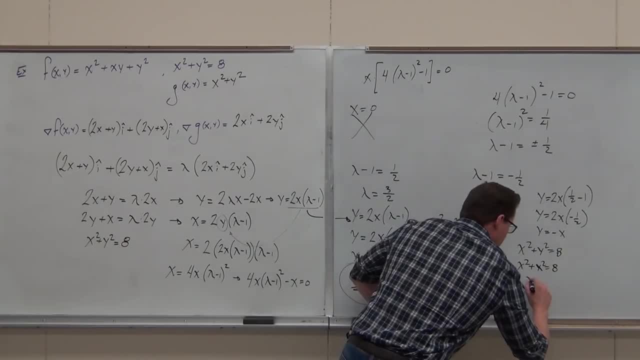 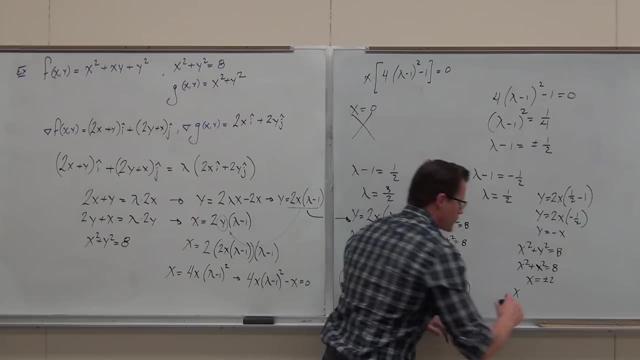 It's going to be sorry. x squared plus x squared equals 8.. It's going to give the same things: x equals plus 2 or minus 2.. However, if you go back to what we used for that, if x equals positive 2, y is the opposite sign. 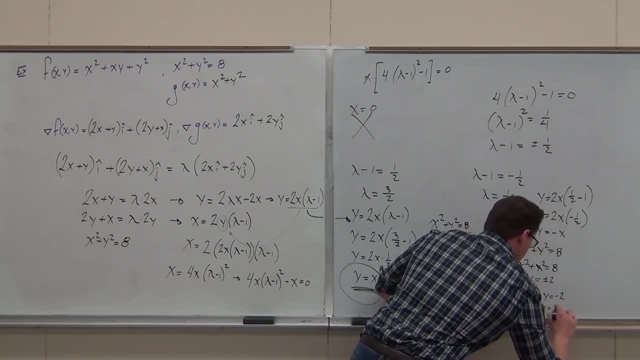 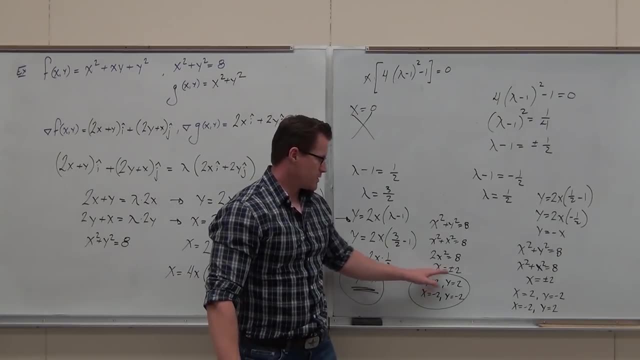 And if x equals negative 2, then y is the opposite sign. That's what that says. So we get some points that look awfully similar. We get the point 2, 2, negative, 2, negative 2.. 2, negative 2, negative 2, 2.. 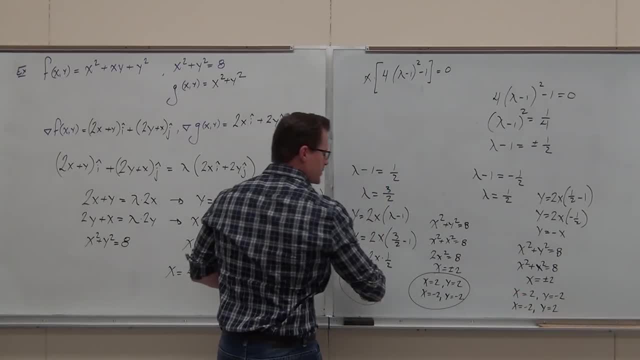 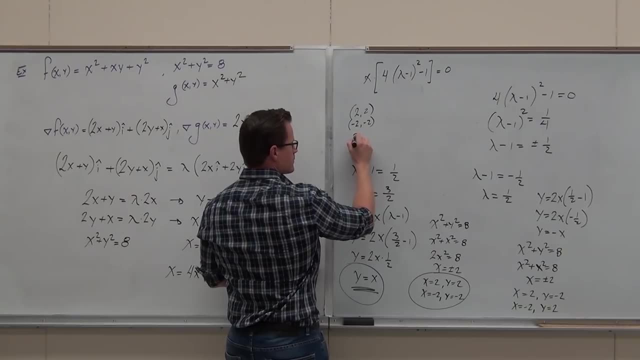 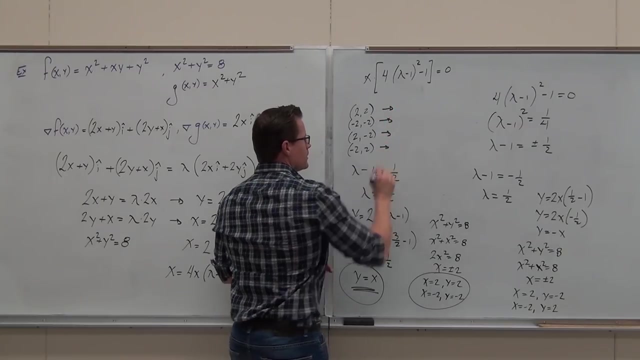 So, out of those four points, I'm going to write them up here. Out of those four points, you tell me this and then we'll be done. Out of those four points, how do you check them? Where do you put them to see which one's the biggest and which one's the smallest? 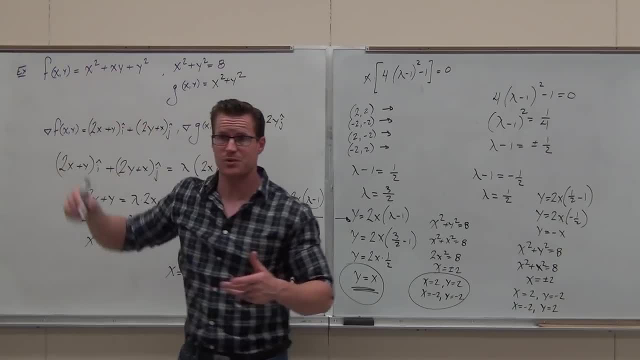 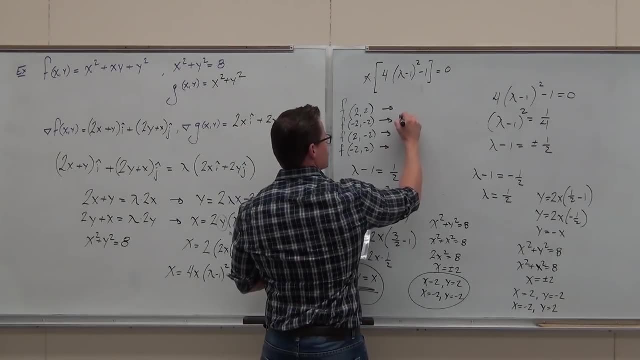 Where do you do it? You put them right there to see which is the biggest and smallest. So we're going to evaluate f of all those. We're going to look at f of all those things. You can try it on your own. 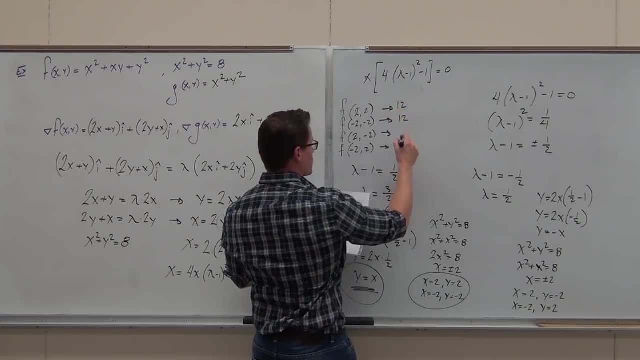 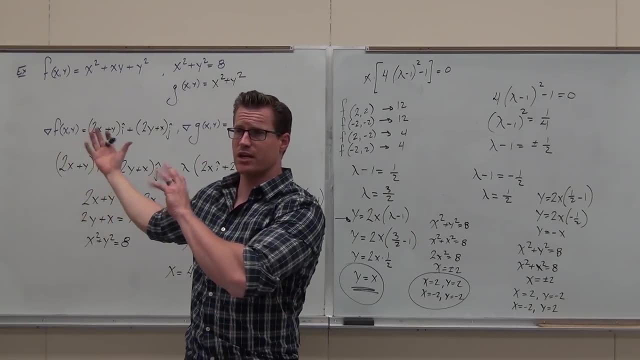 This one is 12.. This one's also 12.. The nature of the square: This one's 4.. This is also 4.. Hey, what's the maximum value we attain out of this constrained optimization problem? We learned earlier that these have to create maximum or minimum. 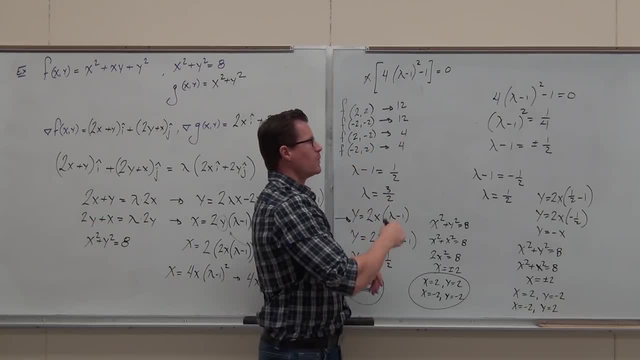 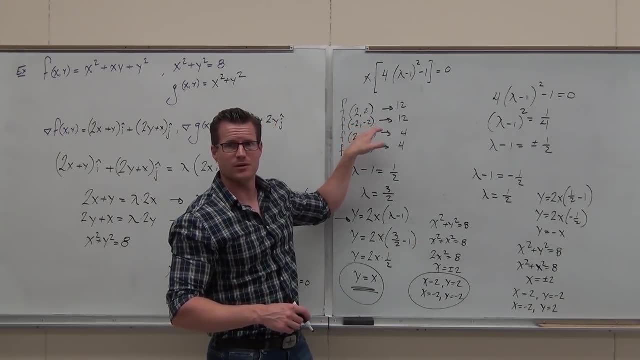 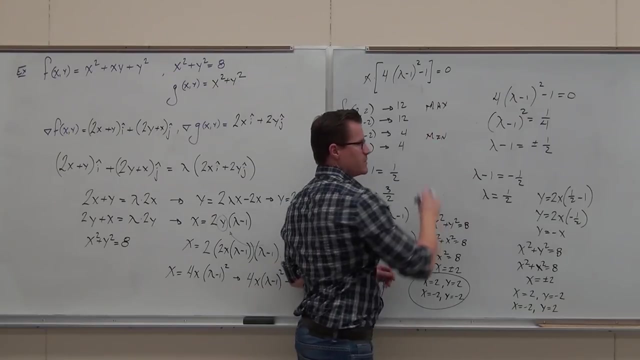 That's what they do. All maximum and minimum will occur at these values with our lambda. What's our max value? Where does it occur? Two different points. That's our max- Constrained maximum. That's our min- Constrained minimum. 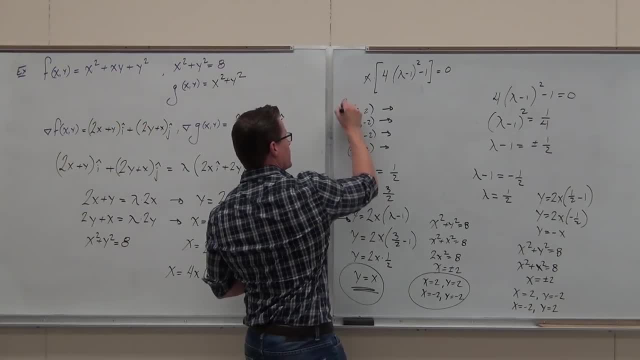 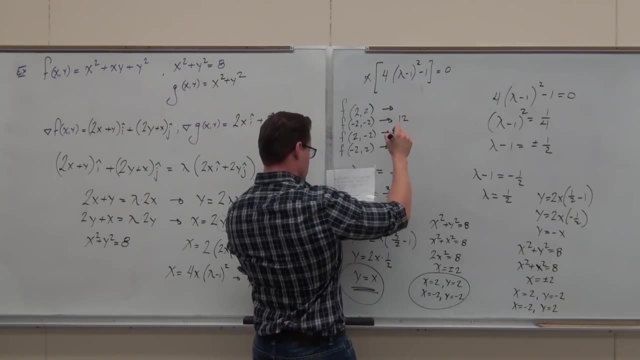 You put them right there to see which is the biggest and smallest. So we're going to evaluate f of all those things. You can try it on your own. This one is 12.. This one's also 12, the nature of the square. 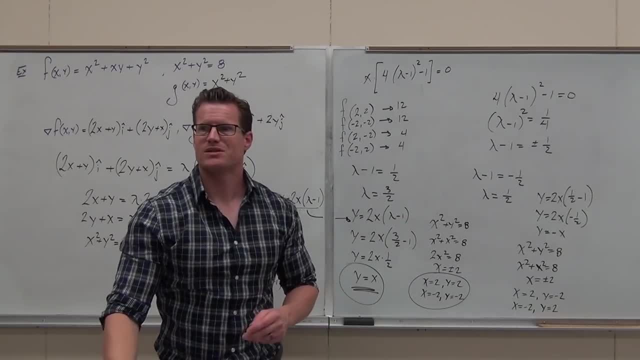 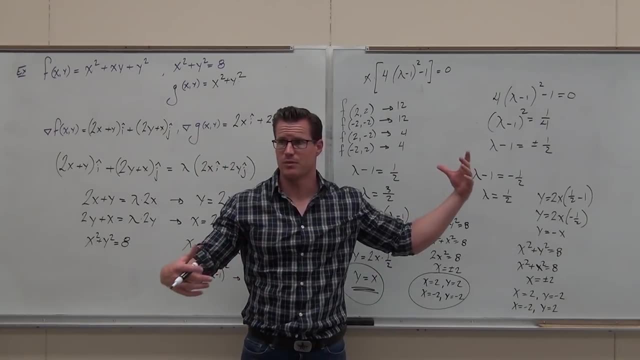 This one's 4.. This is also 4.. Hey, what's the maximum value we attain out of this constrained optimization problem? We learned earlier that these have to create maximum or minimum. That's what they do All. maximum and minimum will occur at these values with our lambda. 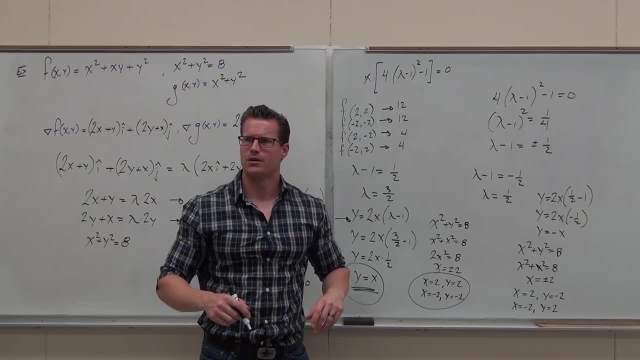 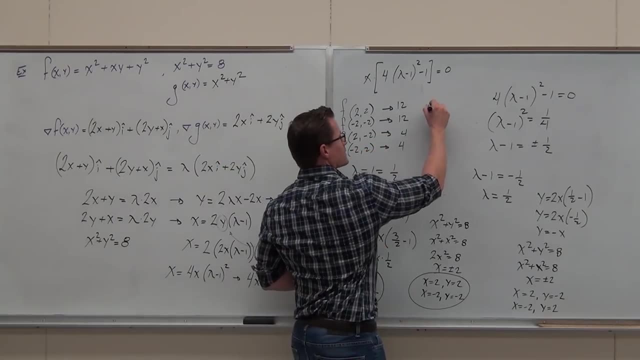 What's our max value? Where does it occur? Two different points. What's our minimum value? Where does it occur? Two different points. That's our max- constrained maximum. That's our min- constrained minimum. I know the algebra's fast. You might want to go through it a couple times on your own, but that's the idea.